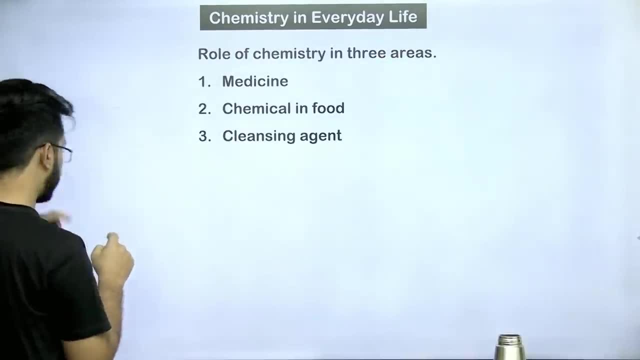 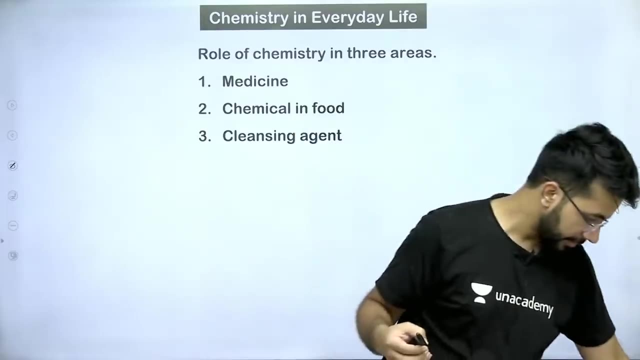 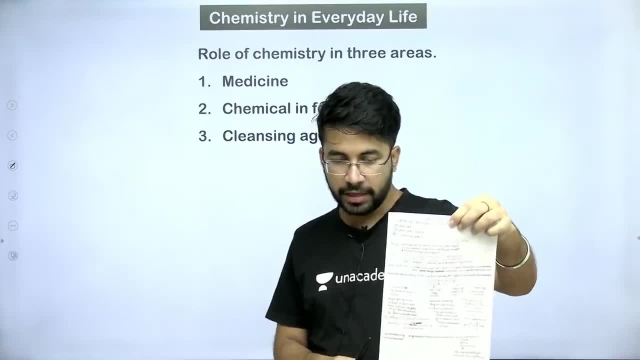 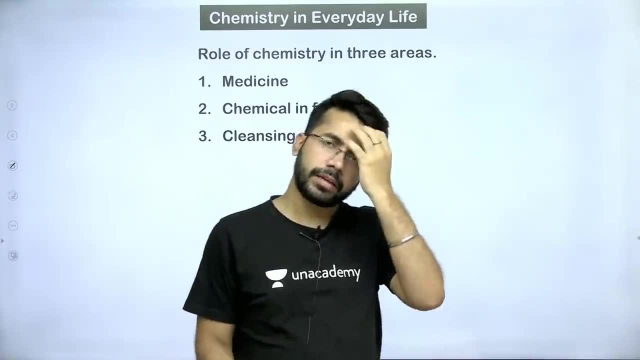 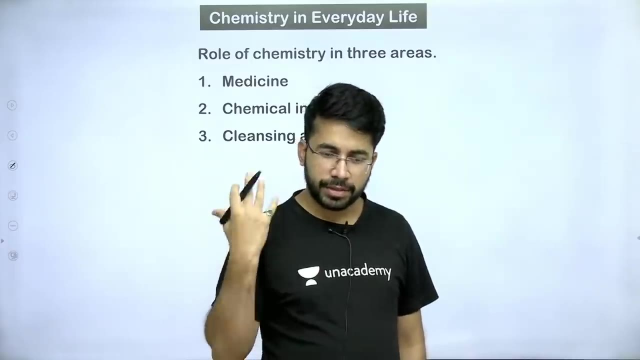 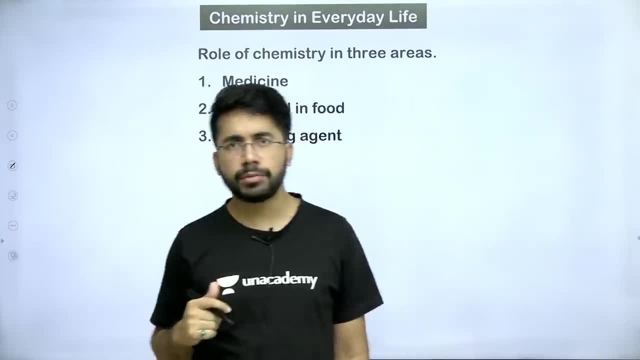 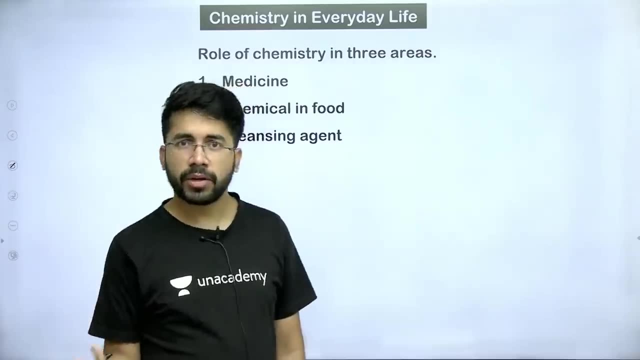 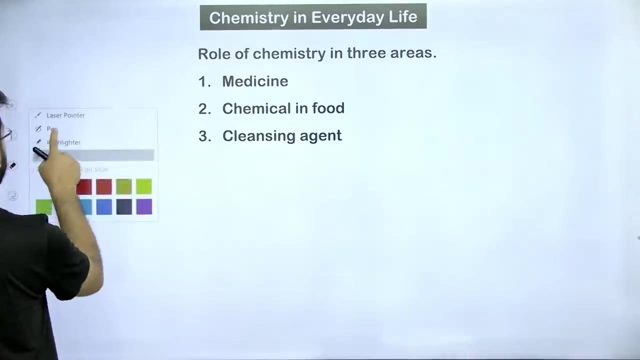 What is it? What is it? cad safari, cad safari. You must be watching this. What is it? Toppers Telegram channel. I put the chemistry, they put the physics and I have been putting bio for many days. Come, my friends, let's talk about the cleansing agent. What is the cleansing agent? then understand what is the cleansing agent. 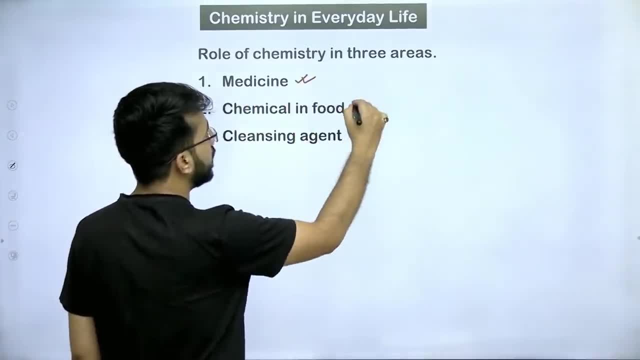 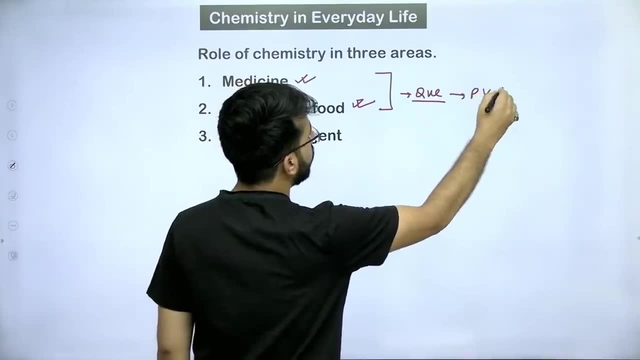 First of all, the medicine questions actually come from both these parts. If I talk about the questions that have come so far, I will talk about BYQ. So from these two parts only p by q is here. A soap and detergent comes in the cleansing agent. 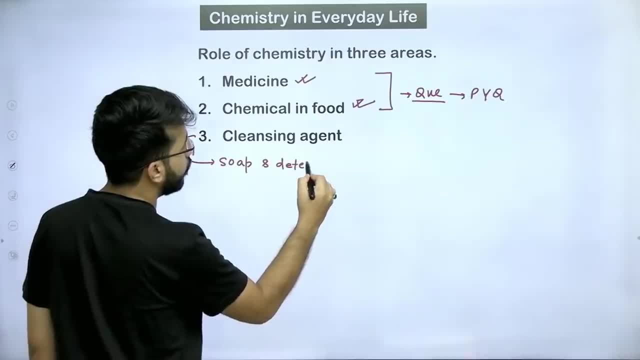 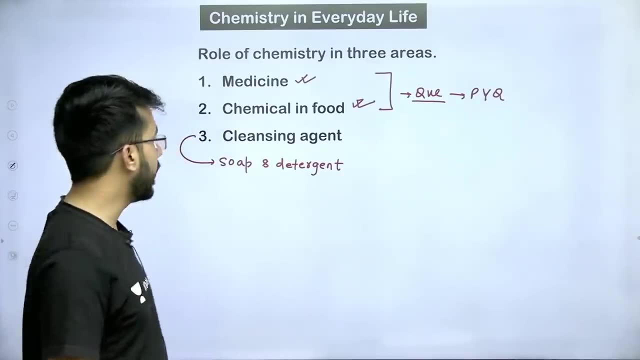 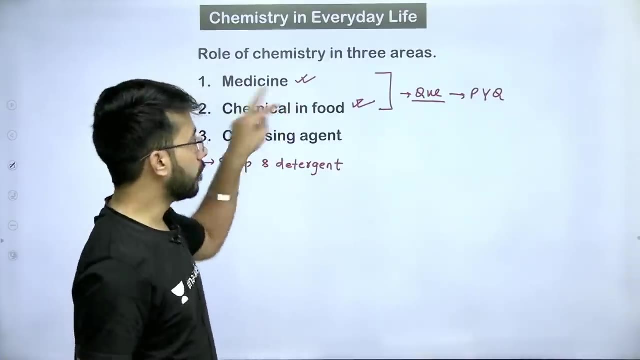 A soap and detergent comes in the cleansing agent and soap and detergent have not come to the question yet So far. I will give his short notes and I will study them both. I will give his notes and I will study them both, because the question comes from here. 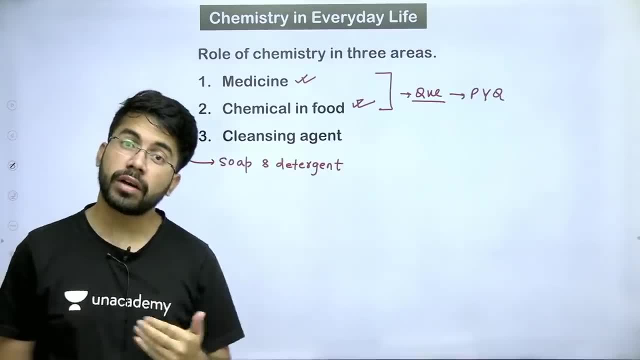 Because this chapter is the part of detergent. here is a description of the body water. Now I will give you an example. Why did this chapter come from here? It also comes in hydrogen, soft water, hard water, so that's why it is covered from there. 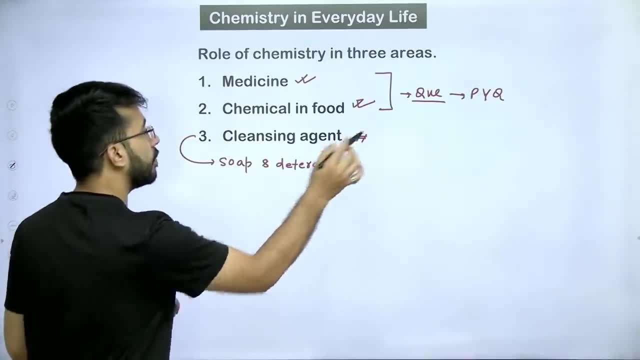 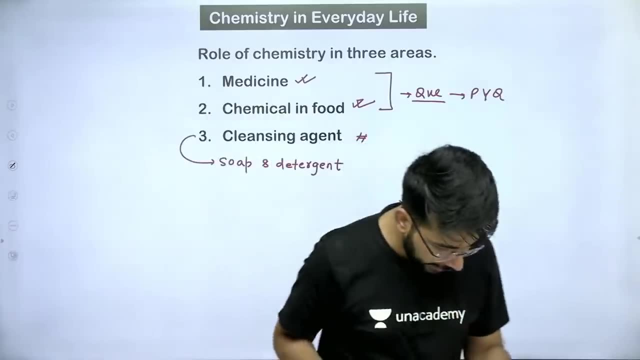 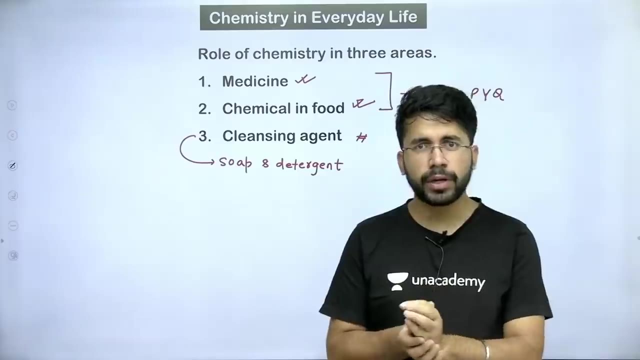 Means. this cleansing agent part will be covered in the hydrogen chapter. So next is medicine and chemical in food. The audio and video are clear so far. Ether lecture has already come. You can see it in my special classes. Diodonium has also been done. 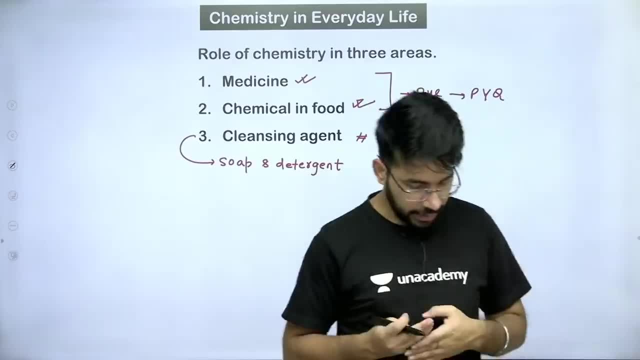 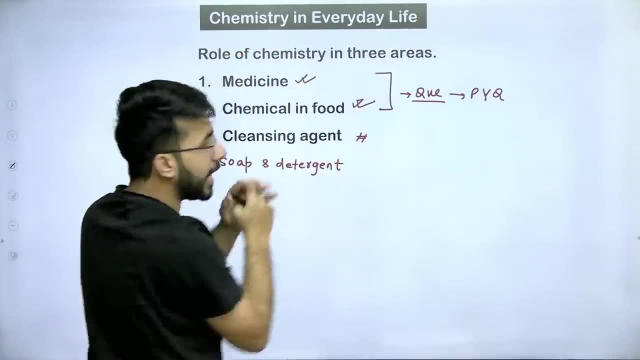 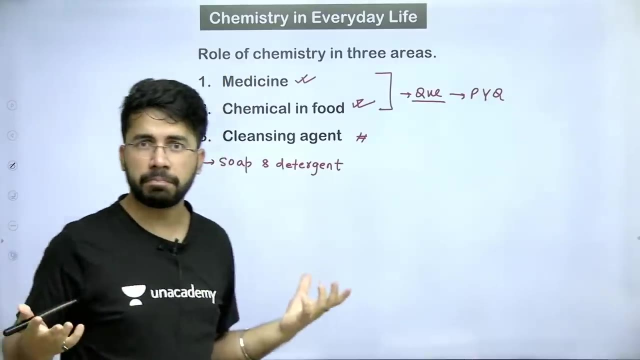 Let's go next Next. Good morning. So, my friends, rule of chemistry in three areas. Actually, we are going to study the use of our chemistry in daily life. So what is the use of our chemistry in daily life? So first of all, let's come to chemistry in medicine. 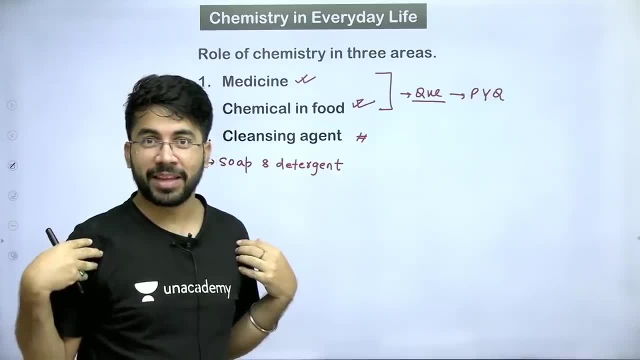 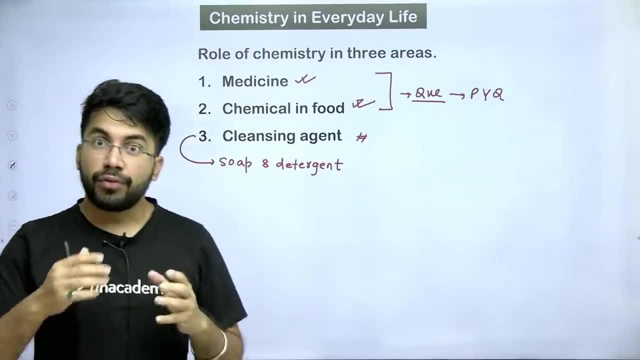 Means your biology is incomplete without chemistry. So, son, chemistry is always needed, Right? So, my friends, we are going to study chemistry in medicine as well, To increase the shelf life of food. Like you must have seen that there is a product. 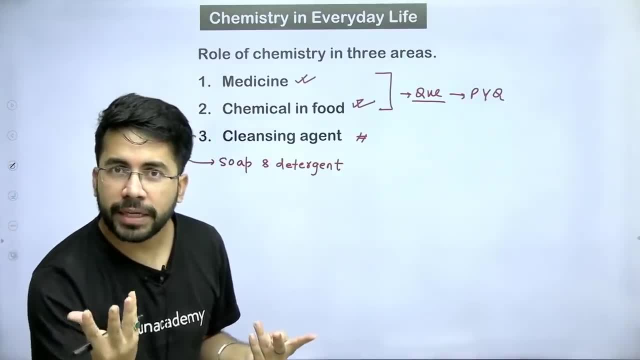 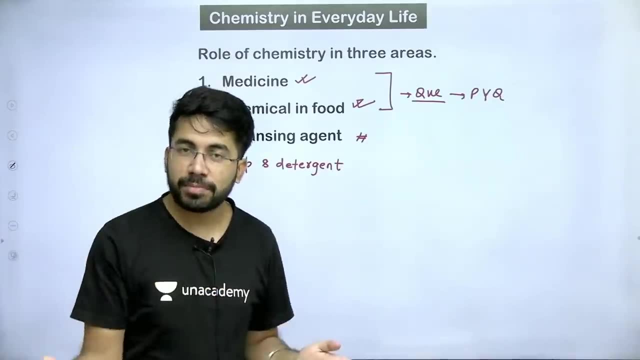 Like nowadays, food comes automatic, ready-made food. Like a few days ago I went to the mall So there was a pot there Which we can use for six months. Means by adding some chemical in it. it has been preserved for six months. 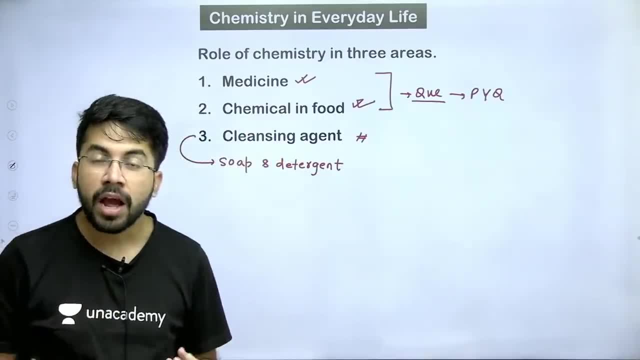 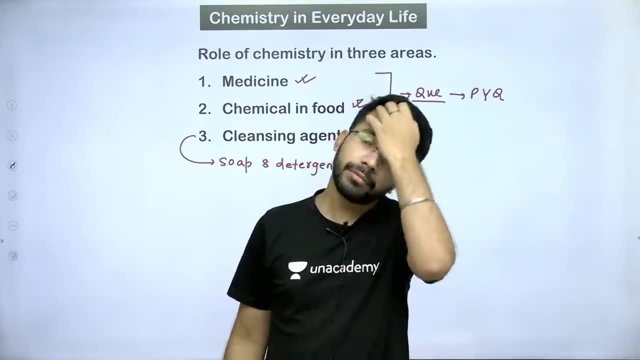 So all those things from which food is preserved, Artificial sweetening agent. When sweets are added, then artificial sweetening agent is added in it So that it is artificial Means more sweet. We add a color, friends, Like rose-colored rose. 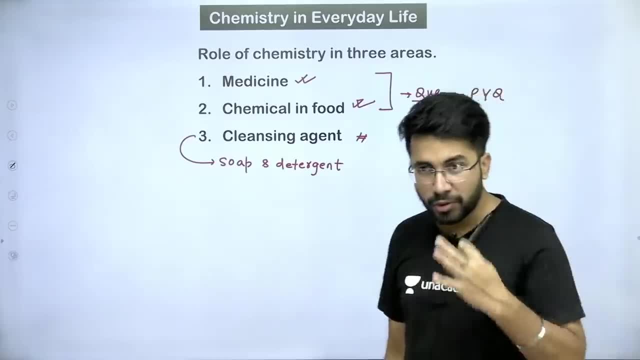 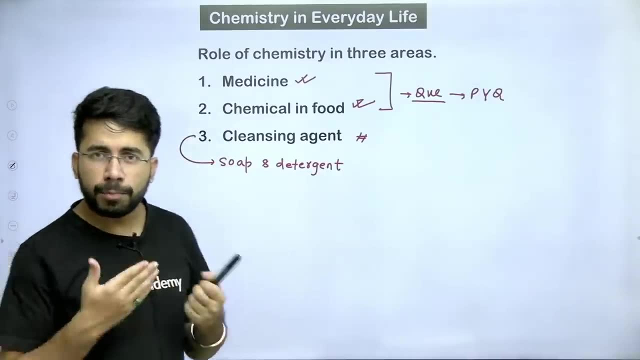 It does not come like that Which we call Rajbhog Or we call Balushahi, So it does not come in itself. We add color in it. It is a chemical. So all those things To preserve food, To increase sweetening in food, 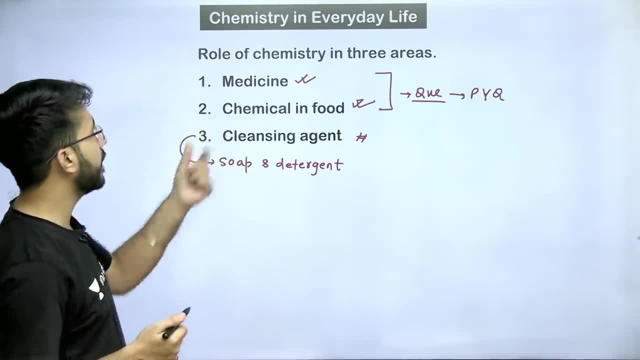 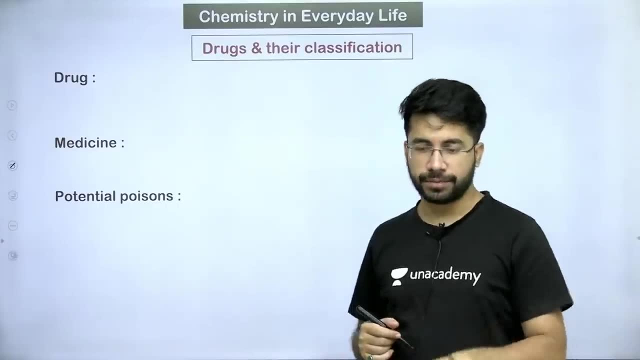 To change the color of food. We will use all these chemicals in food. Let's use it First of all. let's study the part of medicine, Drug and their classification. First of all, let's study Drug and their classification. 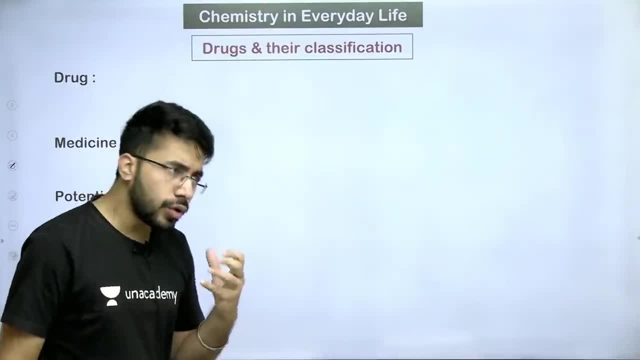 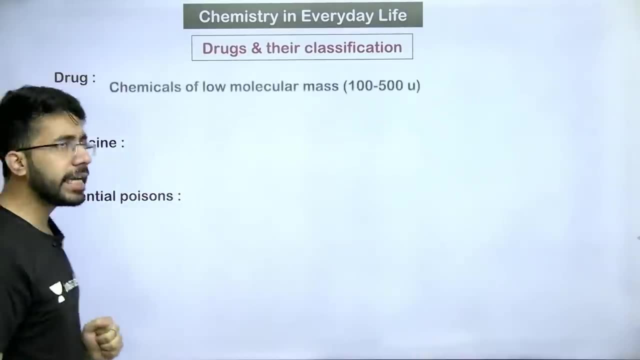 What is a drug? What is a drug? So drug is a chemical substance whose molecular mass is low. First of all, we will understand that drug is a chemical substance whose molecular mass is low. Very true, Chemical is of low molecular mass. 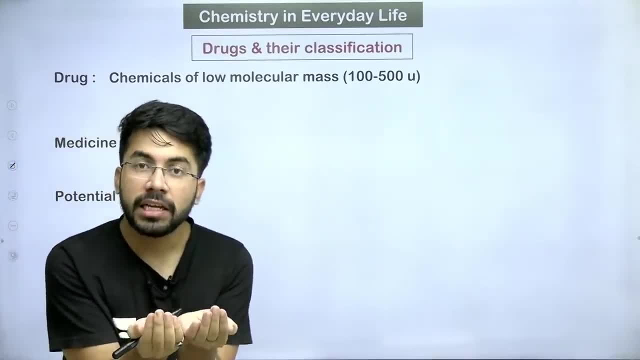 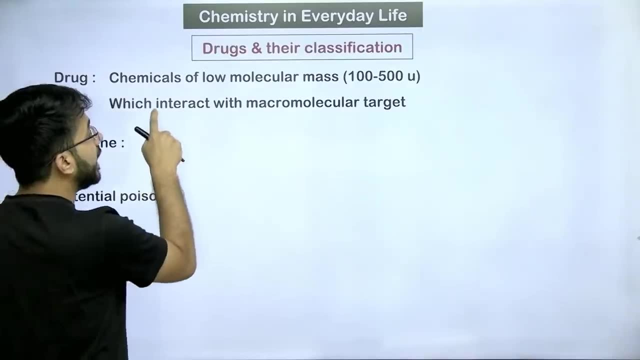 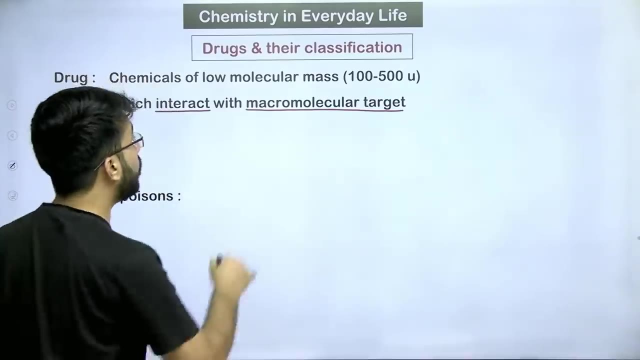 It may be of low molecular mass, But it attacks big targets. What does it mean? It may be of low molecular mass, But it will interact with macromolecular targets. Ok, It may be of low molecular mass, But it will interact with large molecules. 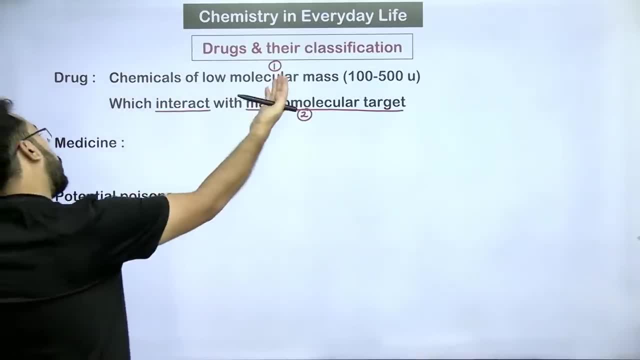 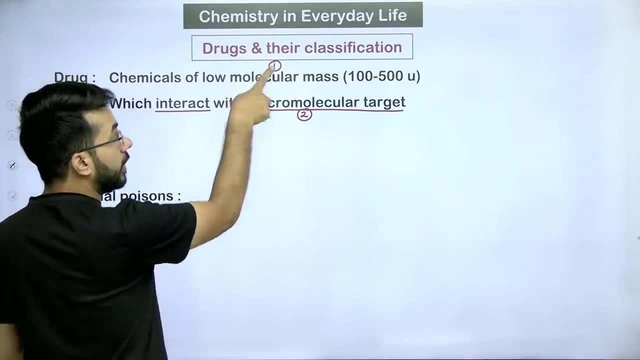 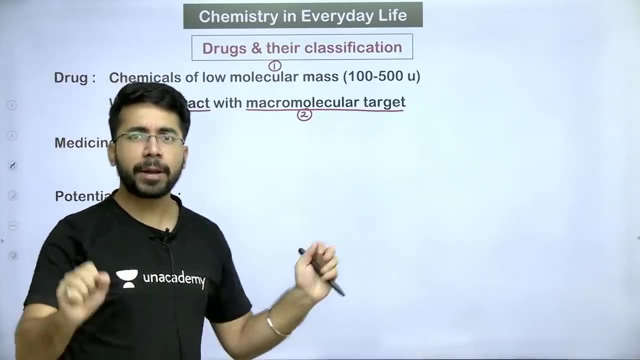 Ok, Good. So chemicals of low molecular mass, Which is interacting with macromolecular targets? Ok, These two will interact With their interaction. If your body is getting relief, If there is any problem in your body, You took any drug. 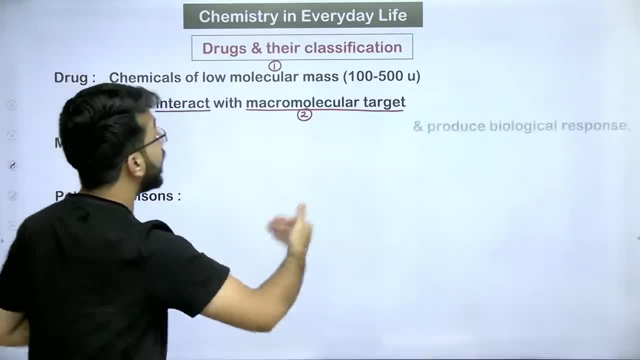 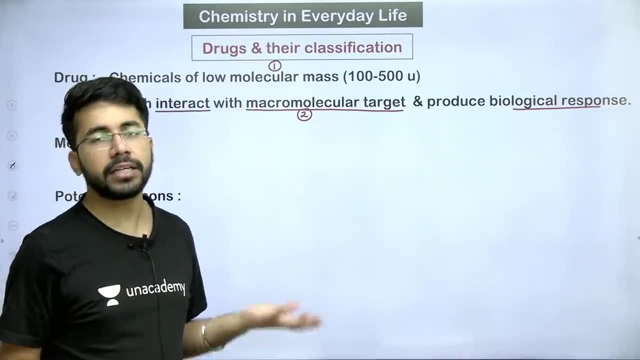 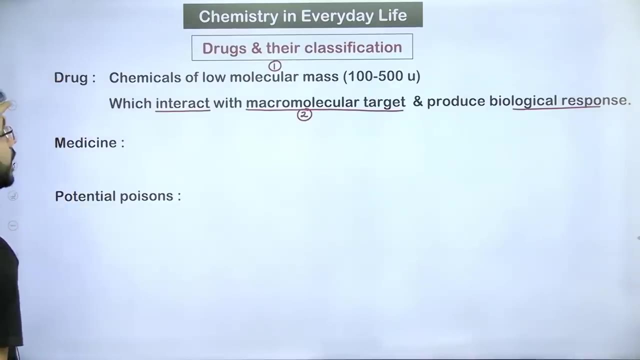 Interacted with that problem And the problem got benefit. The therapeutic effect Which produces biological response, Which produces healing in your body, That is called a drug. Ok, When will we call drug medicine? We will call drug medicine when that biological response has come in your body. 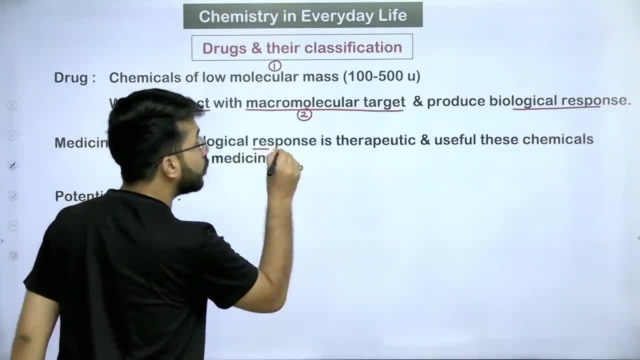 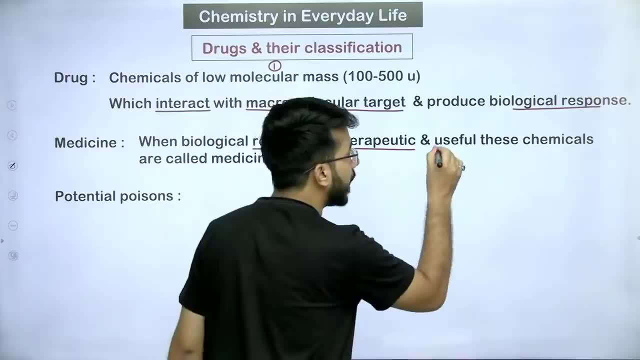 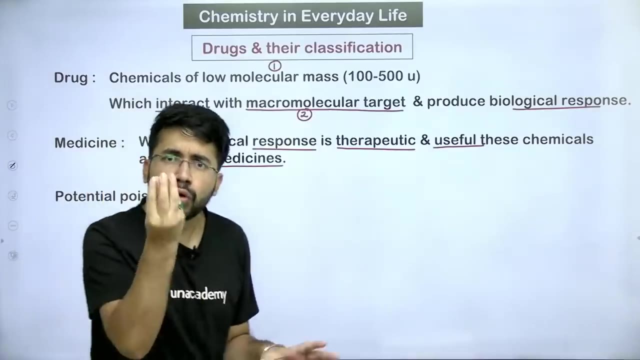 If that response is therapeutic, If that response is therapeutic And it is useful for your body, It is beneficial for your body. Then what do we call it? We call it medicine. Understood What is drug? It is a chemical of small molecular mass. 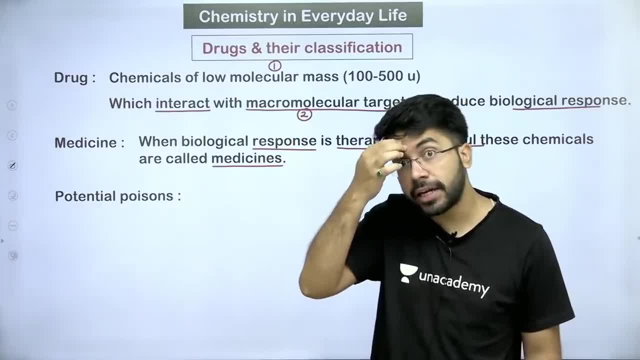 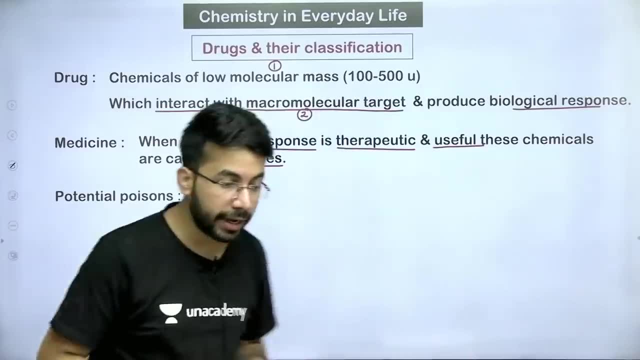 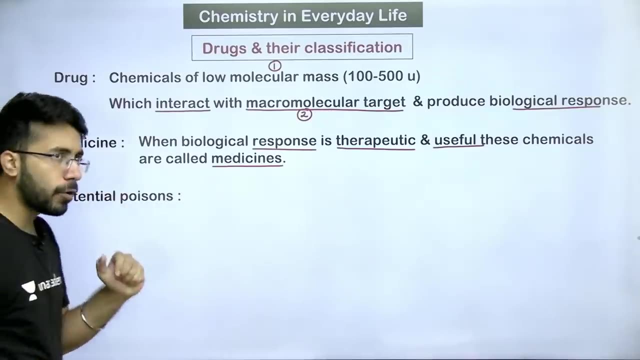 Which will interact with big macromolecules And biological response will produce a response in your body. If that response is therapeutic. If the response is therapeutic, Then only it is called as medicine. Now, what is the term potential poison? So if medicine 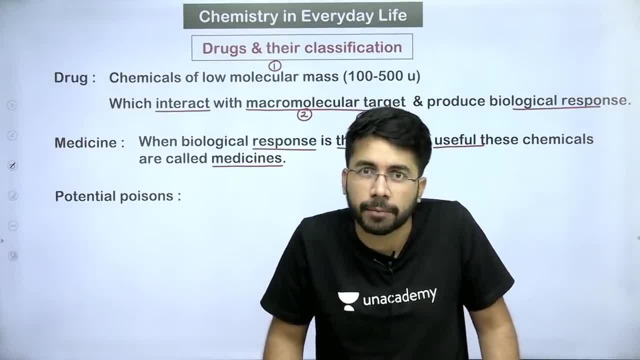 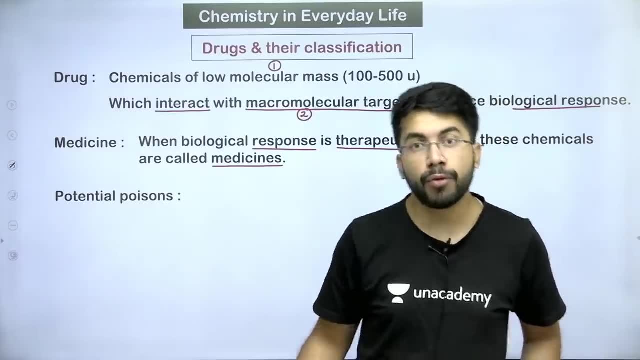 Like the doctor said, You have to take one medicine in the morning, in the evening and in the afternoon. If you take two in the morning, in the evening and in the afternoon Instead of three, you took an overdose. Then it will work as a poison. 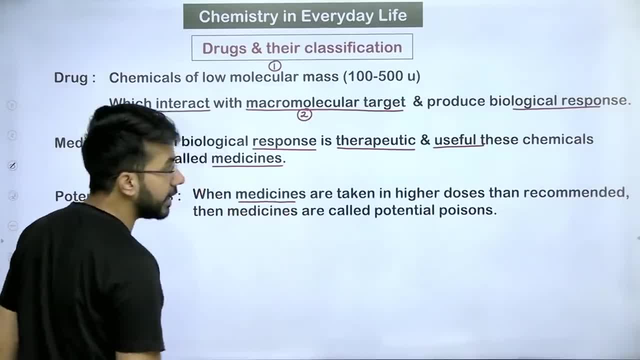 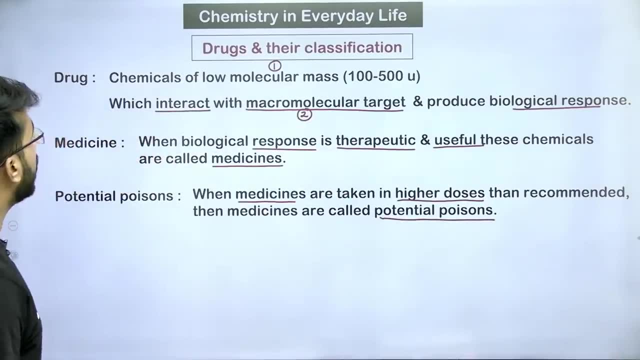 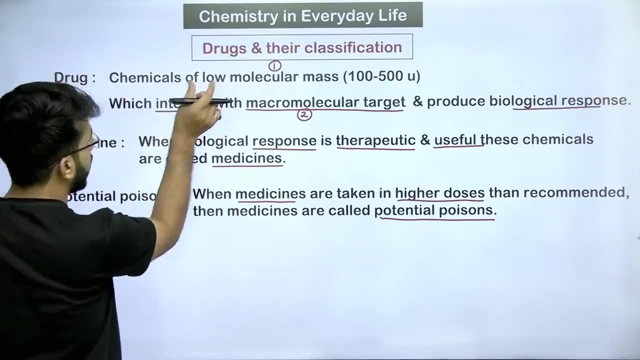 This thing: If medicine, If medicine, If you take it in higher doses, Then it becomes potential poison. Okay, This is drug, This is medicine And this is potential poison: Small molecular mass Which interact with big macromolecules. 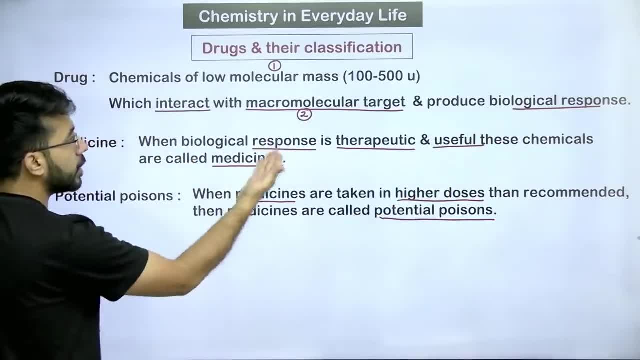 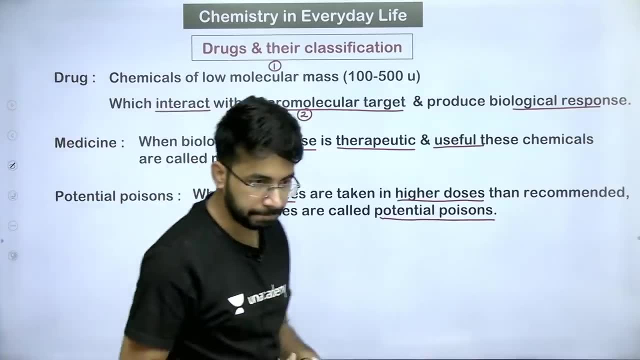 And produce biological response. If response is therapeutic and useful, Then it is medicine, But if you take medicine in higher doses, Then it becomes potential poison. Okay, Very simple. This is very simple definition. Let's go Now, when this is done. 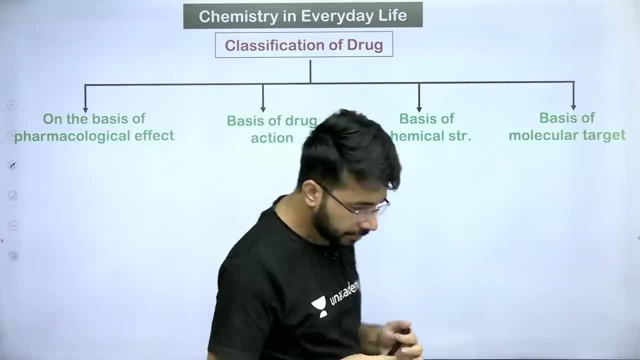 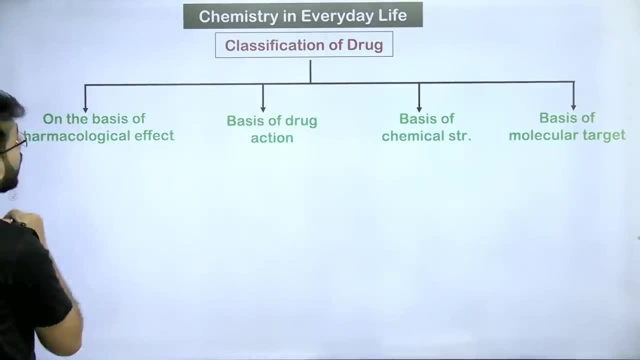 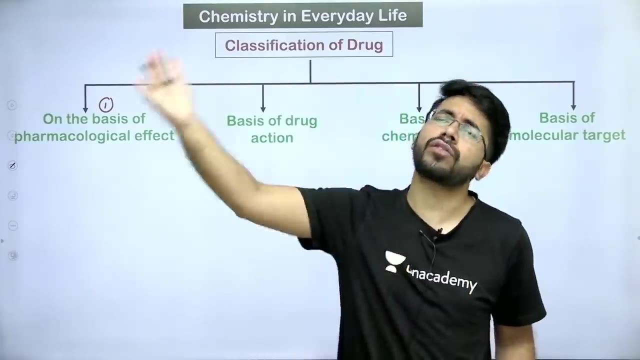 Next is my friend, Let's do the classification of the drug. That in what part this drug is classified? First of all, On the basis of pharmacological effect. On the basis of pharmacological effect Means you must have seen That there are many painkillers in the market. 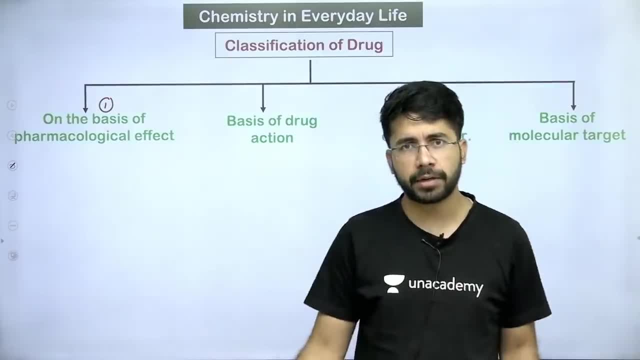 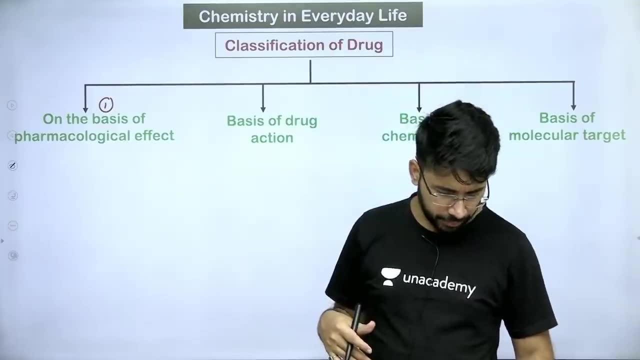 There is a range of medicines Which work in painkillers, Like for fever. There is a wide range of medicines Like if you go to the market to buy anything- anti-acid, If you go to the market to buy anti-acid. 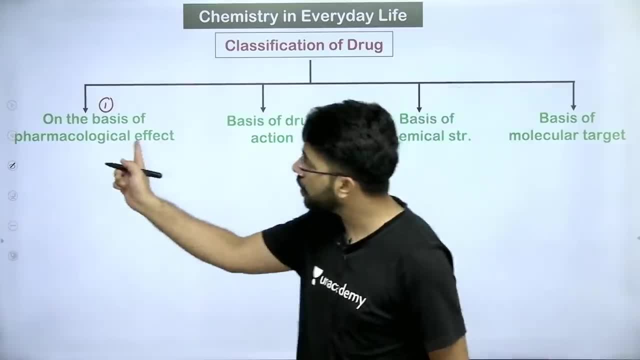 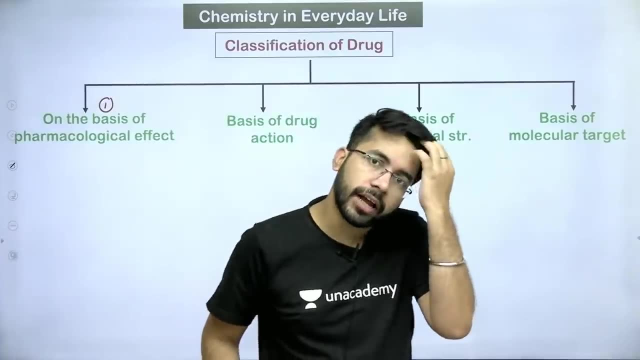 Then also you get a range of anti-acids Right. So pharmacological effect: This is very useful for doctors, Because you will go to the doctor If you have a headache, Then they will give you a medicine, If they have a lot of medicines. 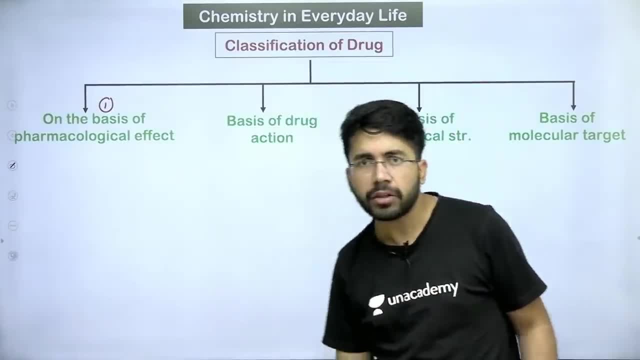 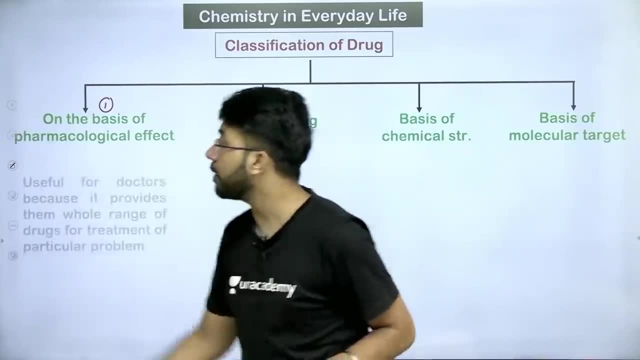 Then they will give you one of them. If they have a leg pain, Then they have a lot of medicines. There is a range of medicines. They will recommend you one of them. So this is very useful for doctors. It is useful for doctors. 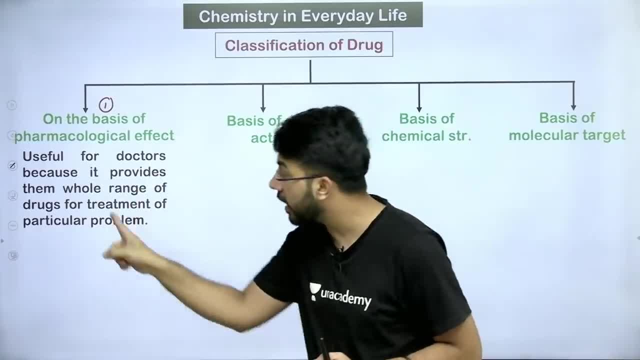 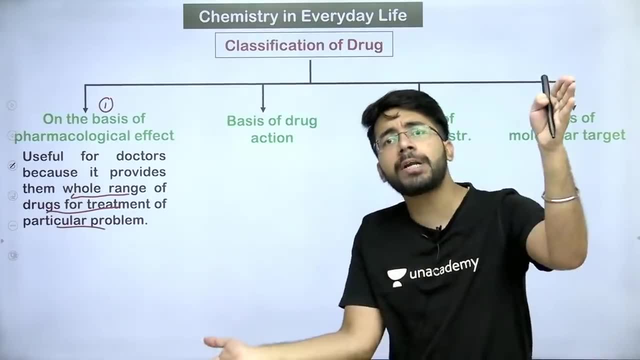 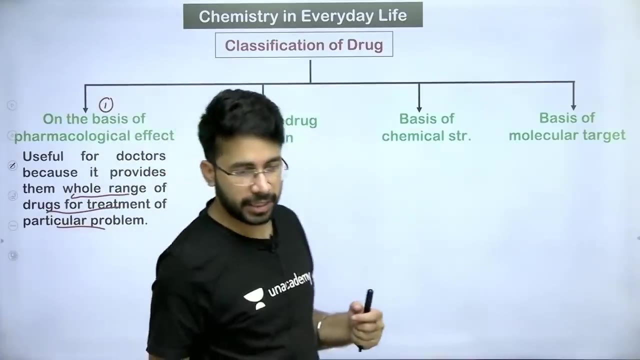 Why? Because it provides doctors Whole range of drugs for treatment of a particular problem, Means it has provided a lot of painkillers. It is very useful for doctors Which painkiller should be given in headache, Which painkiller should be given in leg pain. 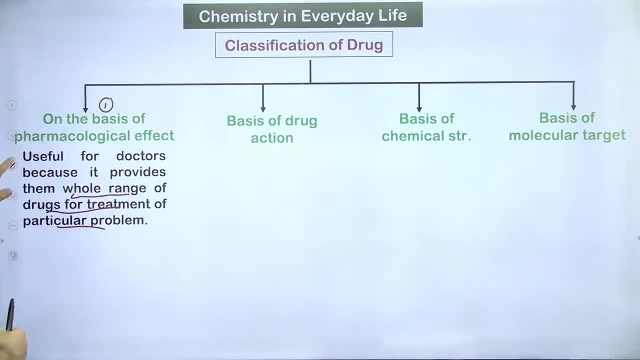 Right. So here, whole range of, Whole range of pharmacological, Pharmacological, Whole range of. What do you get? One second Yes, Here, Oh man, What is happening? You get whole range of drug, Right, Whole range of drug. 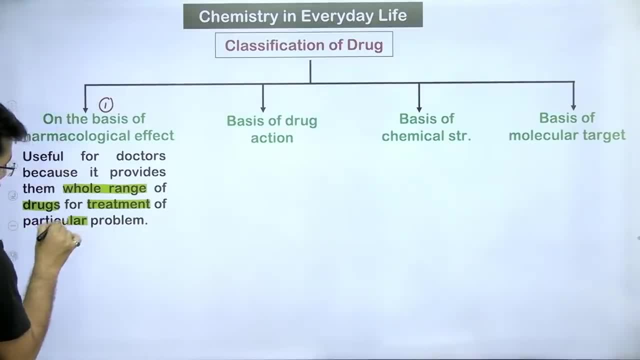 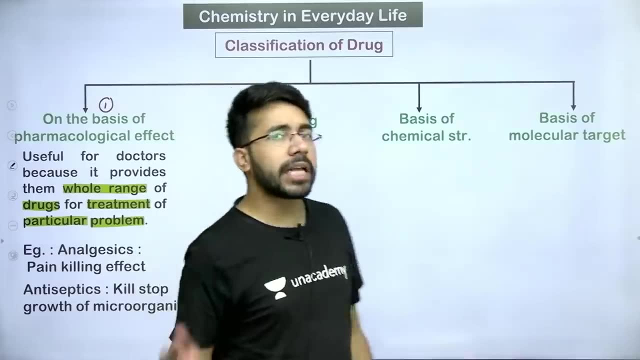 For whom? For the treatment of a particular problem. For the treatment of a particular problem. Let's go Next In example. Like you have analgesics, What is analgesics? Painkillers? Right Now It is called antiseptic. 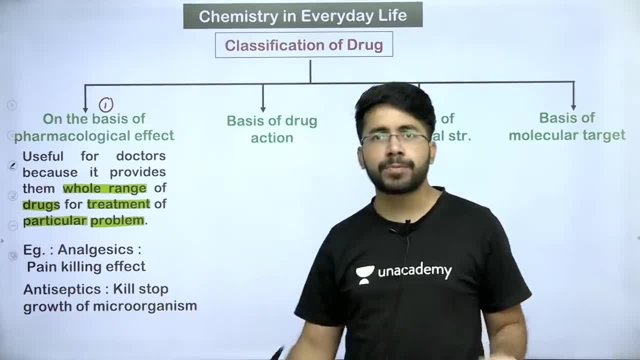 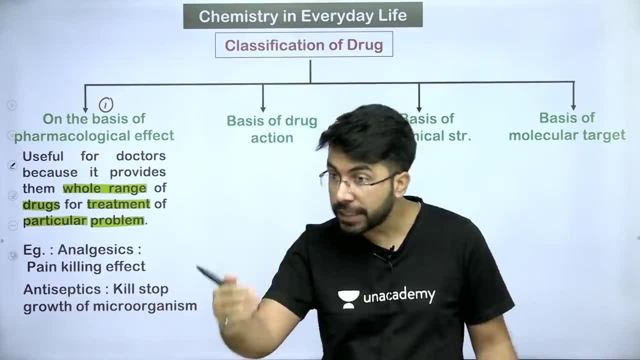 So antiseptic is that which kills your microorganisms. So, like analgesics, So painkillers- There are a lot of painkillers And doctor according to himself, According to the symptoms of the patient, That medicine is given to him. 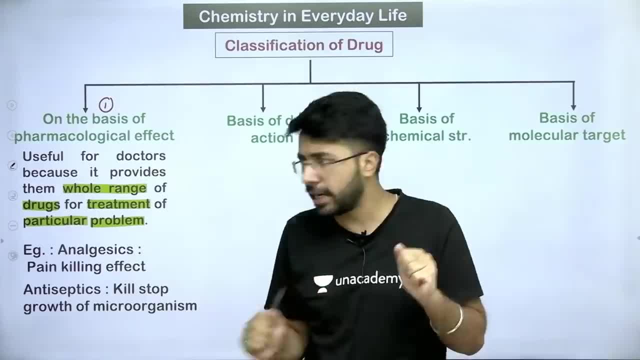 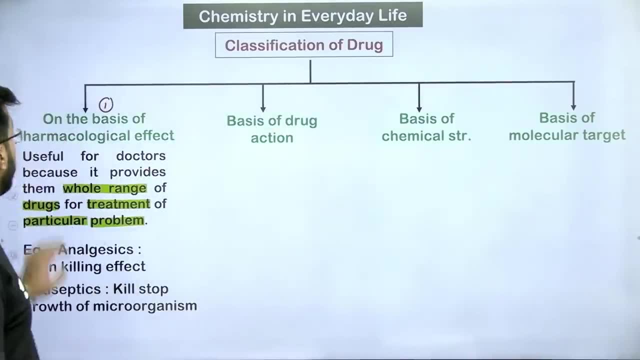 So you will get a lot of range of analgesics. You will get a range of antiseptic. It is beneficial for the doctor. Okay, On the basis of drug. On the basis of drug. On the basis of action on drug. 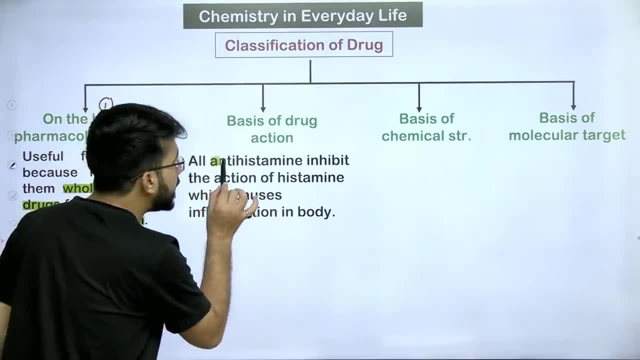 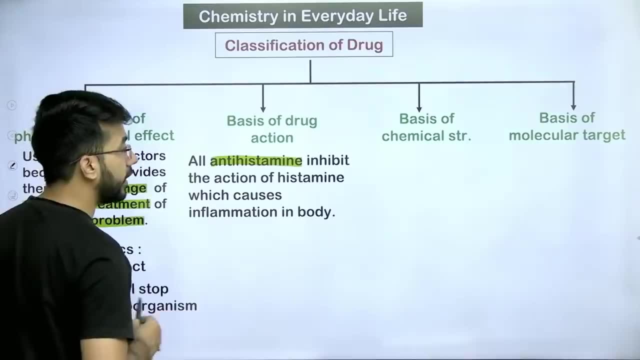 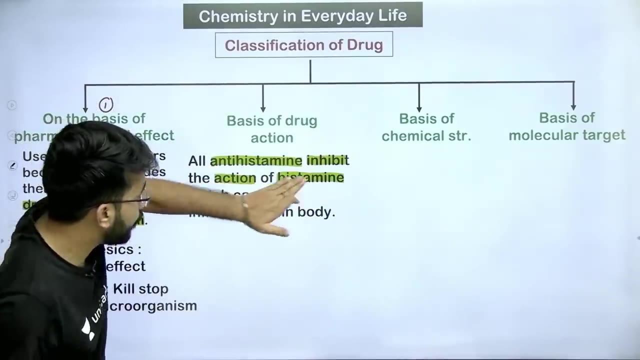 Come. It is said that all antihistamine. Now we will study about histamine and anti-histamine in detail. What do all antihistamine do? It stops the action of histamine. Antihistamine inhibits the action of histamine. And what does histamine do? Inflammation in the body. It causes inflammation in the body. What are histamines in the body? It will cause inflammation in the body. It will cause swelling in the body. swelling will come. When swelling comes, then, my friend, we give antihistamine. What does it do? 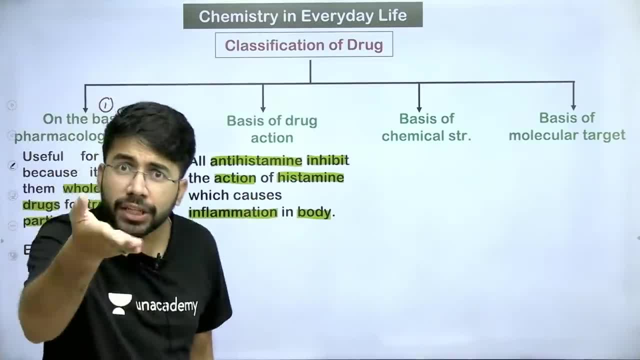 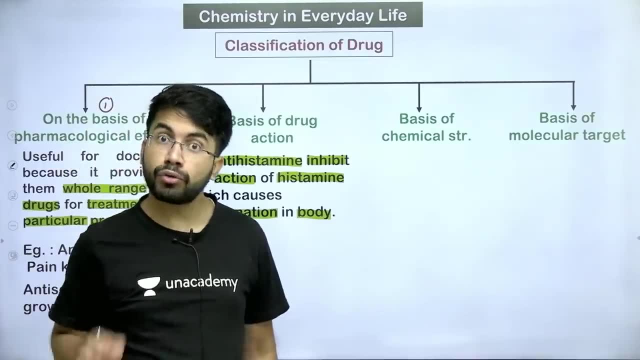 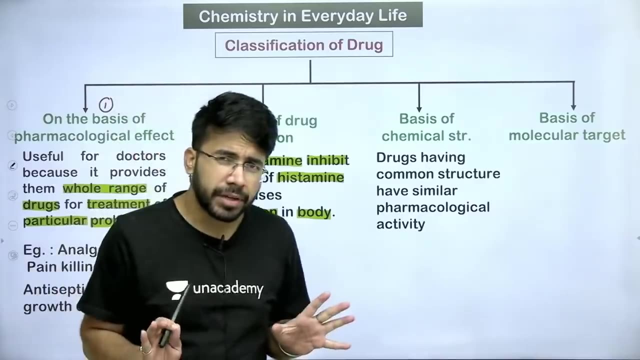 It stops the action of histamine. So on the basis of action, the classification of the drug has been done. One chemical is such that it is causing inflammation and swelling and the other chemical is such that it is reverting it. On the basis of chemical structure, it has been seen that generally the same structure 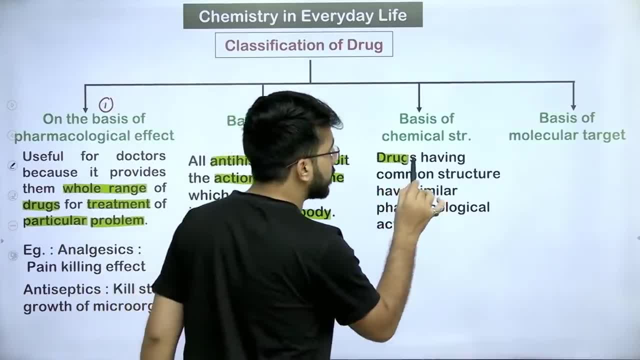 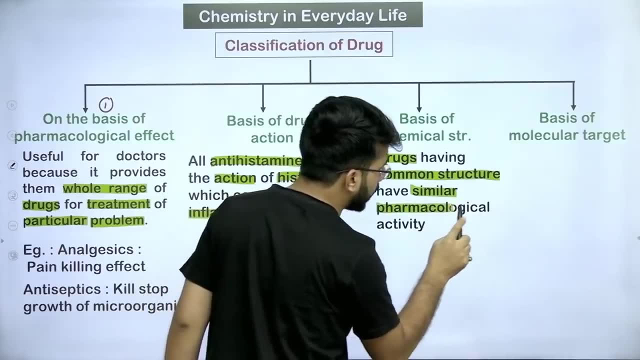 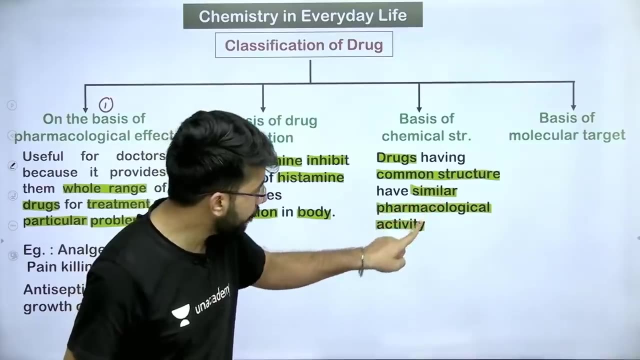 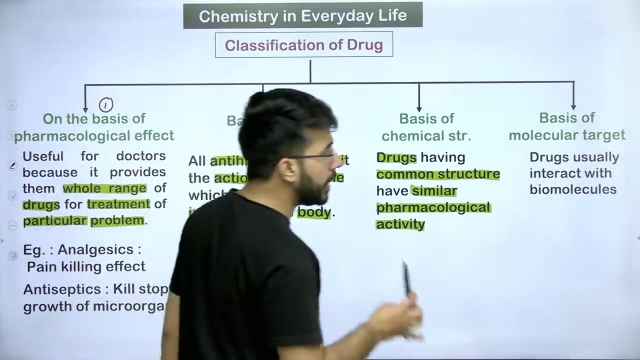 chemical has been seen that such drugs which have a common structure, They have similar pharmacological activity. Understand: such drugs which have a common structure, they have similar pharmacological activity. Next, now let's come to the basis of the molecular target Drugs usually, 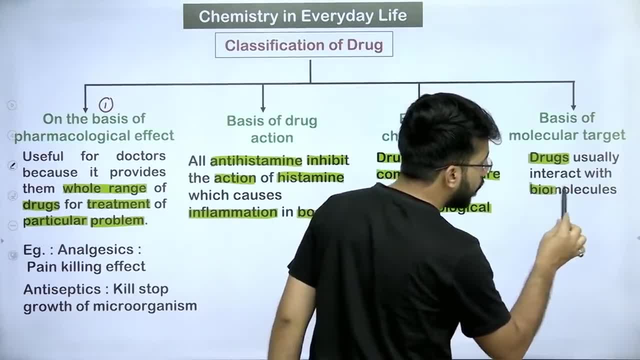 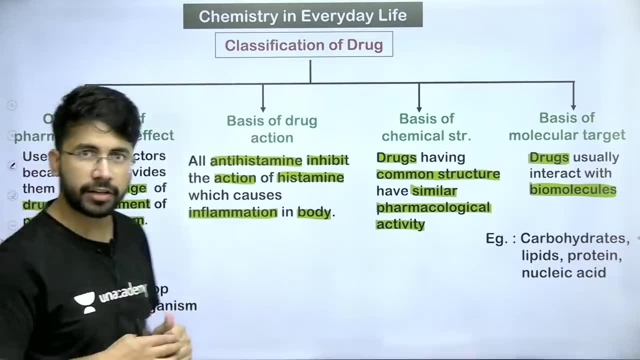 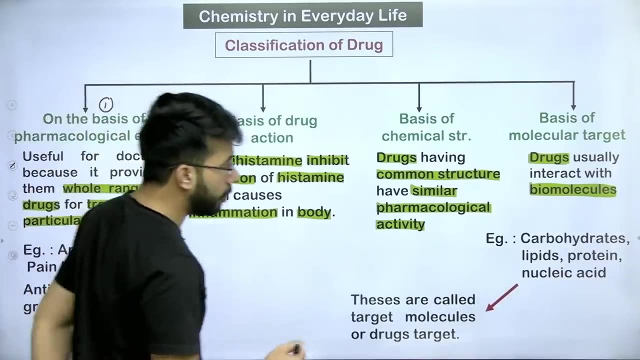 interact with biomolecules. There are biomolecules in your body: Carbohydrates, lipids, proteins, nuclear acid. So all these drugs interact with carbohydrates. Example: this is the example of biomolecules. this is the example of biomolecules. Okay, these are the biomolecules. 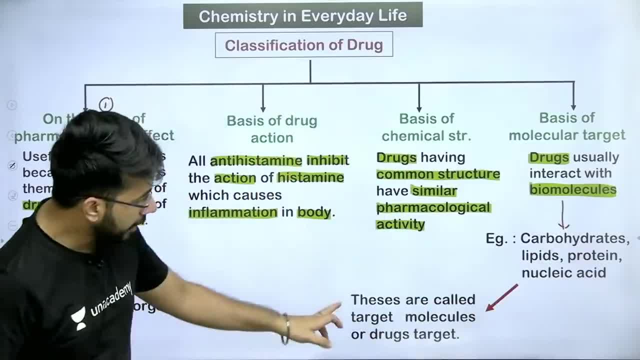 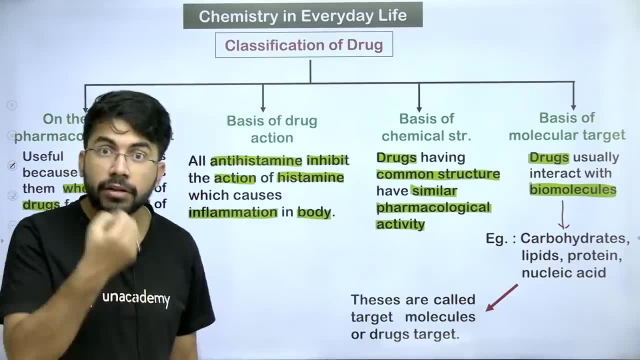 the example of carbohydrates in front of you: lipid, protein, nucleic acid- and these are called target molecule and drug target. The drug is on the target. when you inhale it, take some medicine, you intake it, not inhale, you intake it, so friends will intake it and it interacts with it. 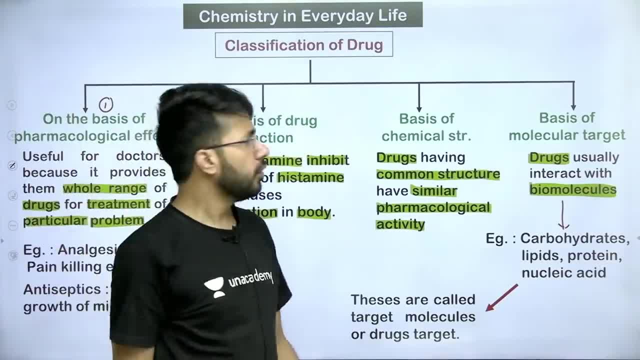 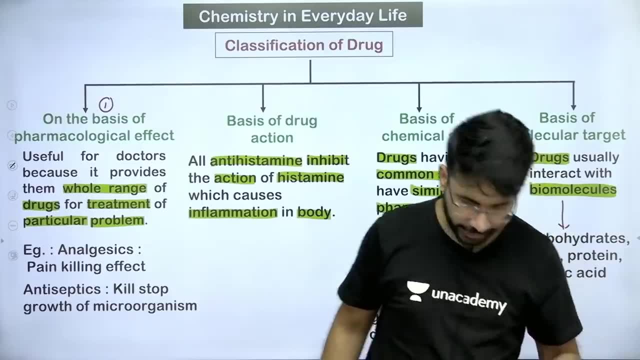 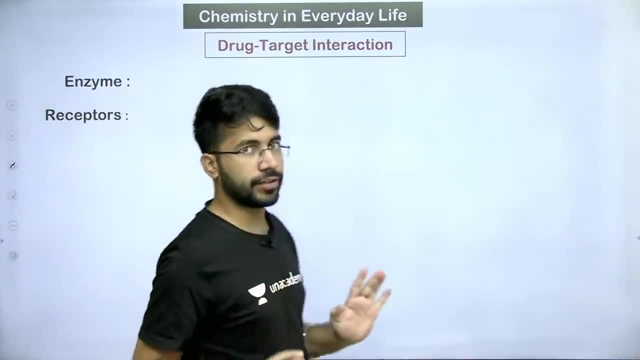 And So this is a small classification, it does not become a question. but if there is a classification then you have to know. You have to know the classification. Now come, your main actually starts from here. Drug target interaction: Mainly. your main starts here. 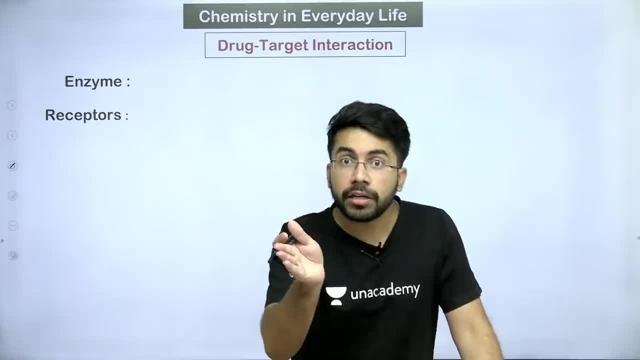 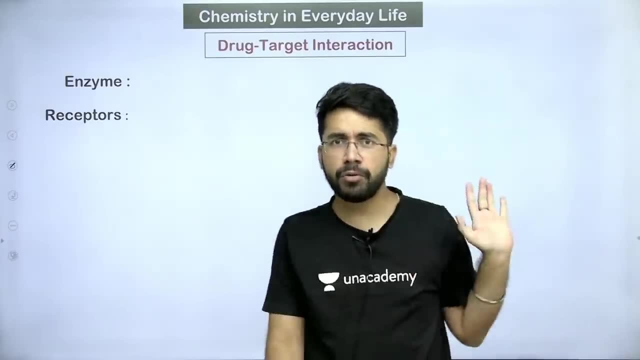 Come. First of all, let's understand how the drug interacts with the target molecule. Just now, we learned who the drug will interact with With the biomolecule. When you take the drug, who will it interact with With the biomolecule? 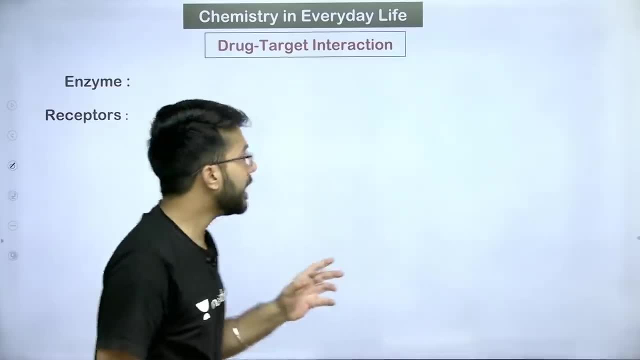 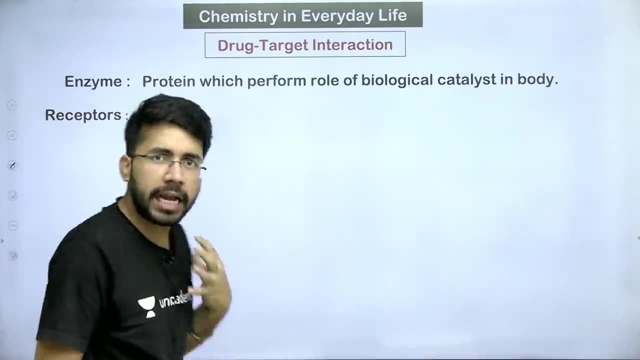 How will it interact? We are going to learn that Understand. we have two definitions. First of all, what is enzyme? Enzyme is actually a protein. There is a protein in your body. What does it do? It acts as a biological catalyst. 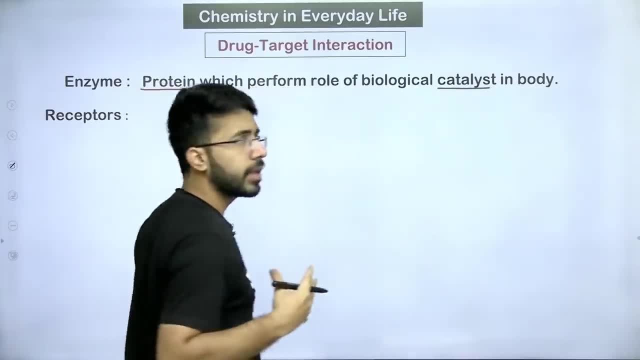 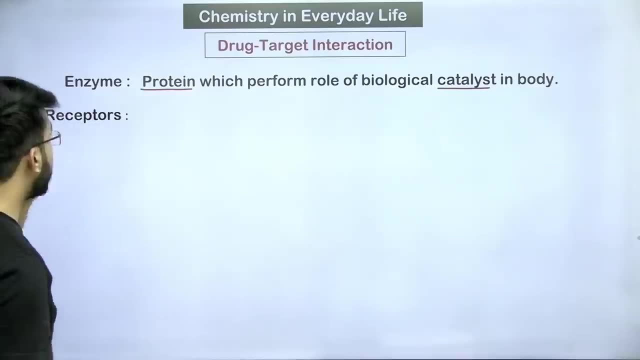 Actually, the enzyme acts as a catalyst. All the reactions that are happening in your body it does that. It acts as a catalyst. Come Now: what is receptor? There is a communication system in your body. For example, the car is coming. 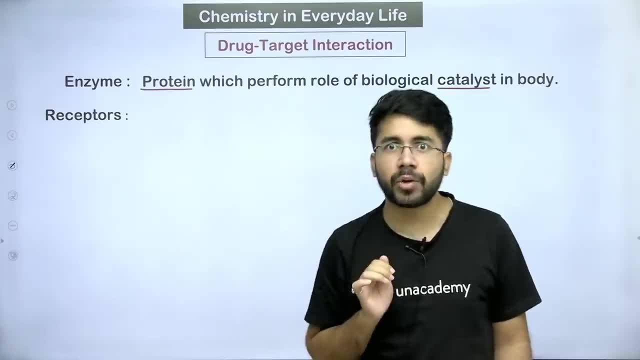 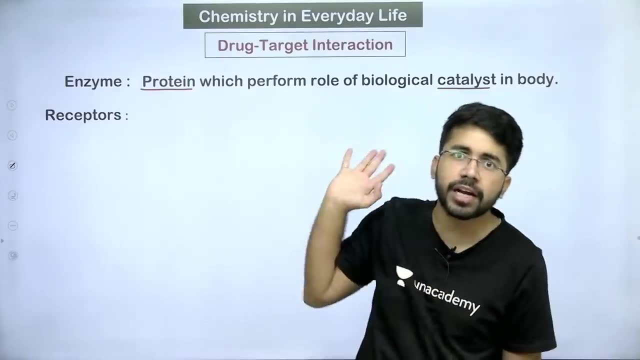 So we have to be on the side, Left side or right side. This message goes to the brain Somewhere. the communication system is running Like when you touch something hot, you quickly remove your hand. What is the message in our body? 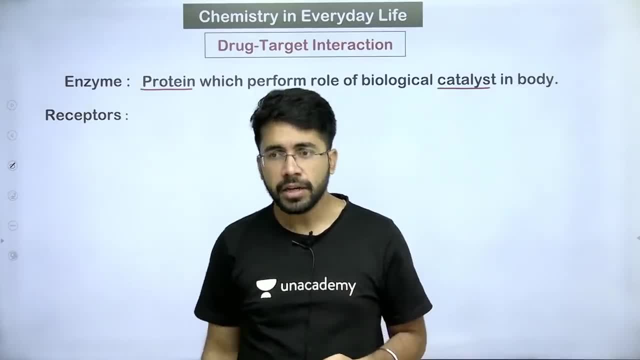 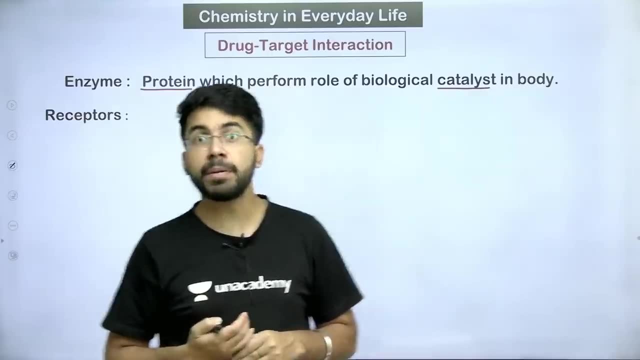 If you remove it from there, it will burn. Okay, You feel cold things, that it is cold. So the body gets the message, We get the message in the neurons, We get the message in the nervous system. So what is the message transfer system? 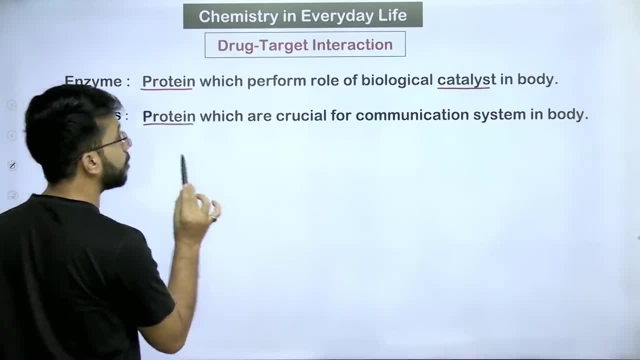 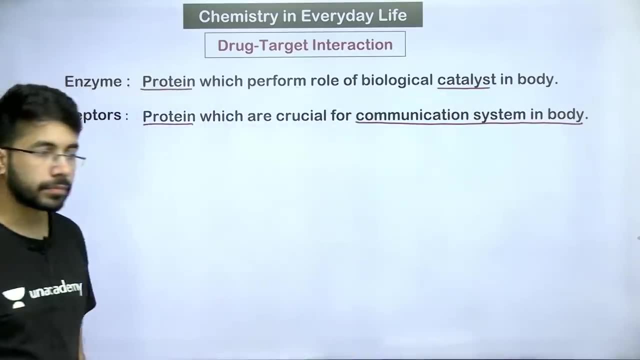 Who makes the communication system. Receptor is also our protein, Which takes care of the communication system in our body. It takes care of the communication system in our body. So if your receptors are weak, then let's see some people become thin. 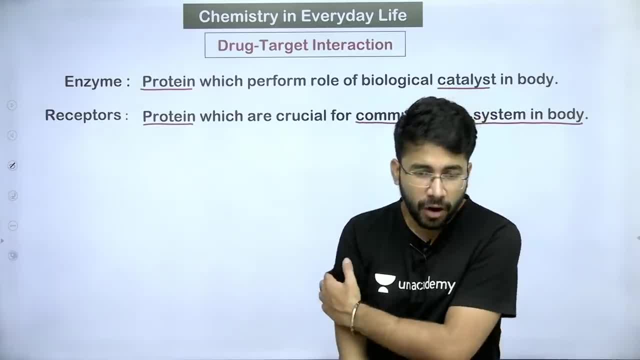 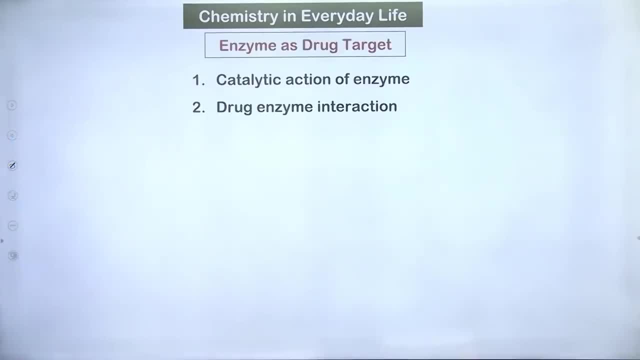 Because their receptors are weak. Okay, And who is the enzyme Which acts as a catalyst in your whole body? Any reaction will act as a catalyst in your whole body. Let's see Catalytic action of enzyme And the second one is drug action. 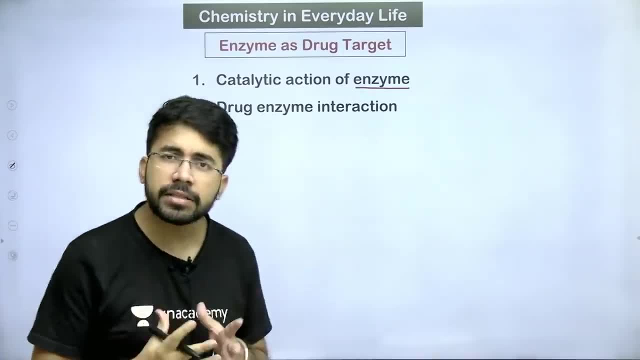 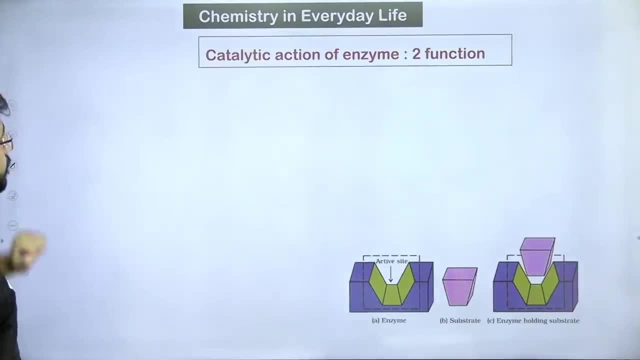 Drug enzyme interaction. First of all, let's understand. How does the catalytic interaction of the enzyme happen? How does the enzyme act as a catalyst? Let's see, Let's read one by one What happens. The enzyme we have. 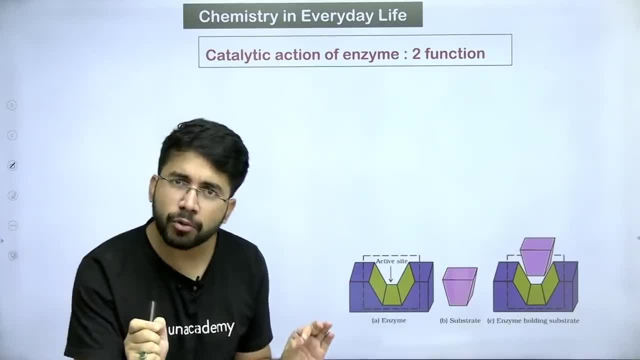 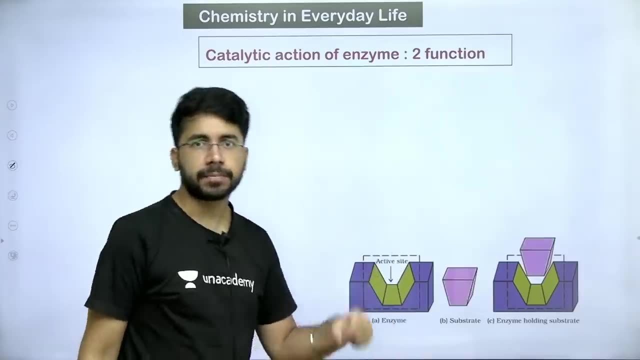 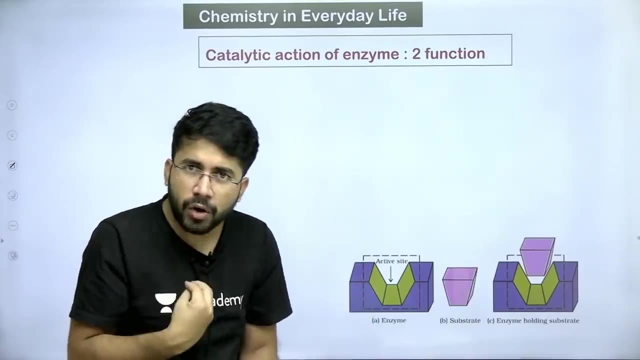 it has a special selective shape. The enzyme we have. it has a special selective shape. The enzyme we have. it has this empty shape. Okay, Now, what will it do in your body? It has to react with many molecules, For example, when you eat food. 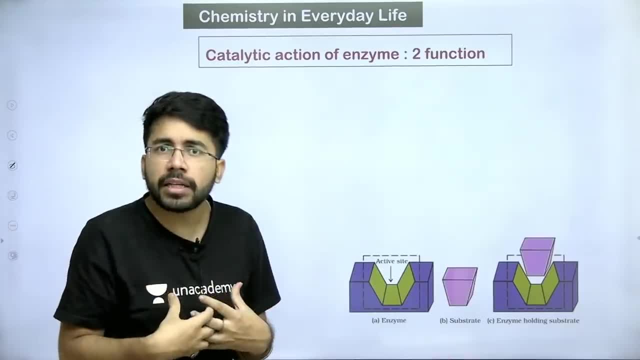 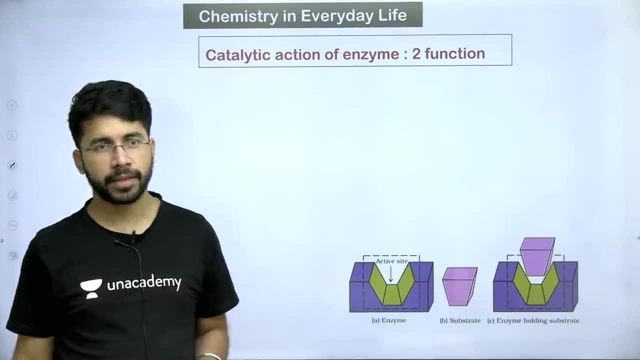 the acid inside helps to break the food. So it mixes the food and the acid So that the catalytic action becomes fast And your food gets digested. So see, this is the enzyme. There is an empty place in the enzyme. 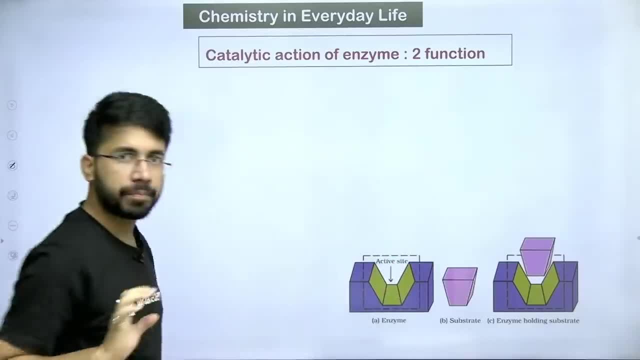 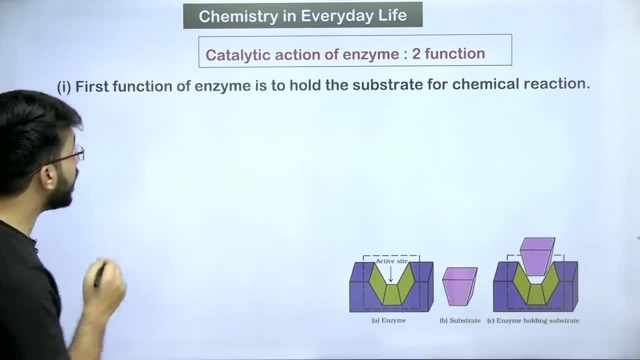 There is an active site Here. it will bring the substrate and make it sit. Understand, One by one, There are two functions in the catalytic action of the enzyme. What is the first function? It holds the substrate. There are enzymes in our body. 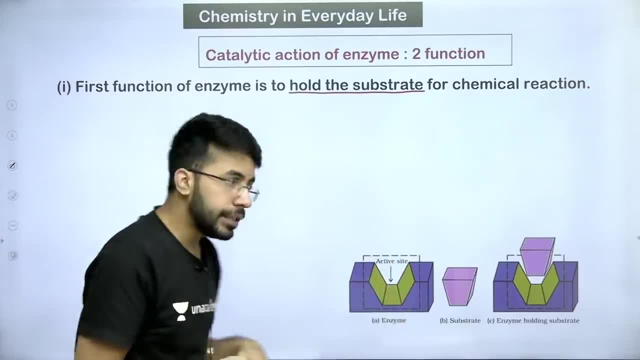 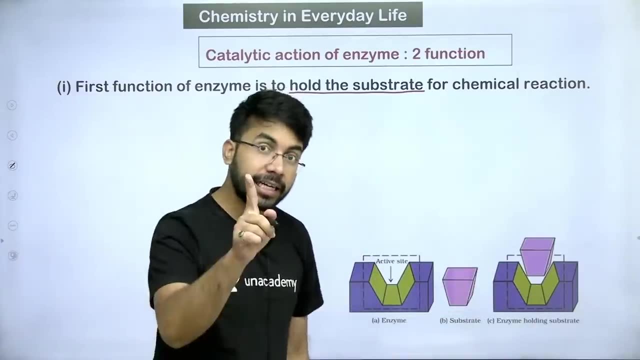 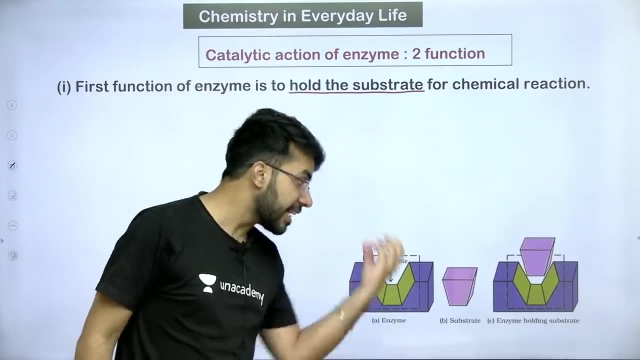 It has a special shape. It has a particular shape In which it holds the substrate. Now you have held the substrate here. Now see this: Every enzyme will hold different substrates Because every enzyme has a different shape. So only a special enzyme can give a special reaction. 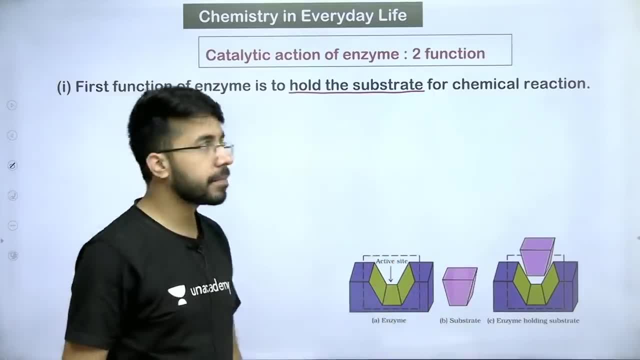 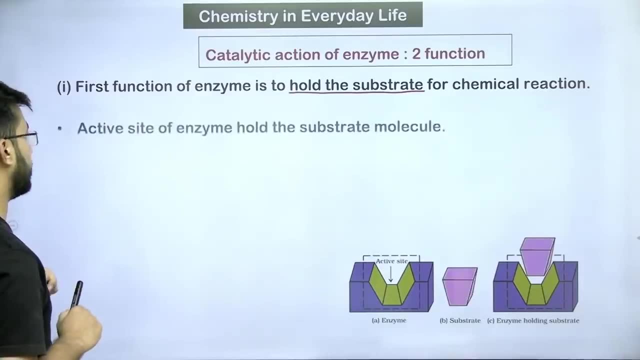 So different, different enzymes will come for every substrate. Let's go. The first thing is that it will hold the substrate, And where will it hold? It has an active site. It will hold in the active site. It holds the substrate in the active site. 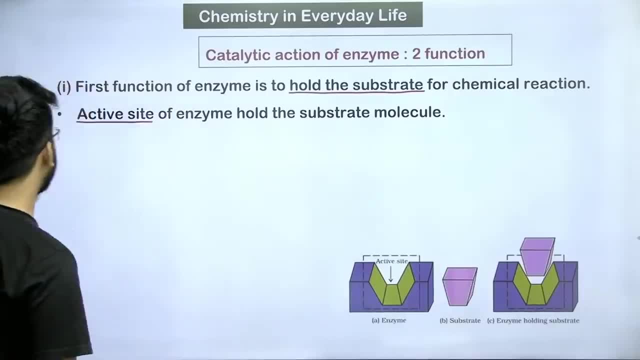 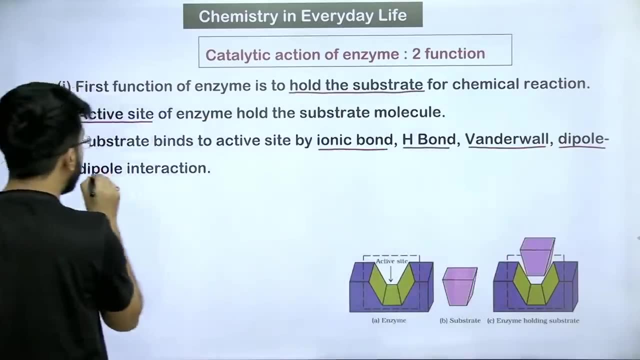 Which force of attraction does it hold? So there is H-bonding in it, There is ionic bonding in it. There is a wonderful force of attraction in it. There is a dipole-dipole interaction in it. It is holding it with this force of attraction. 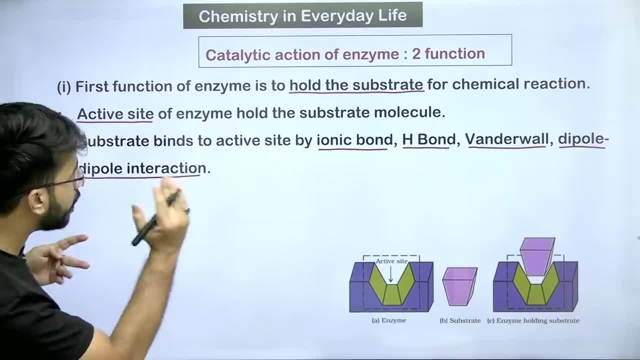 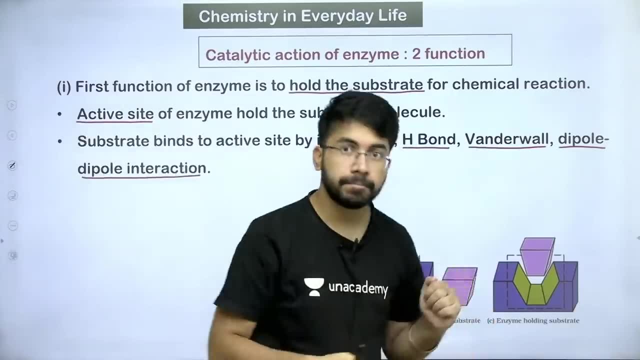 It is absolutely correct. Now come, There is ionic bonding, There is H-bonding, There is a wonderful: It is holding with dipole-dipole interaction. This is the first function, that it is holding the substrate. Now we have to do the reaction too. 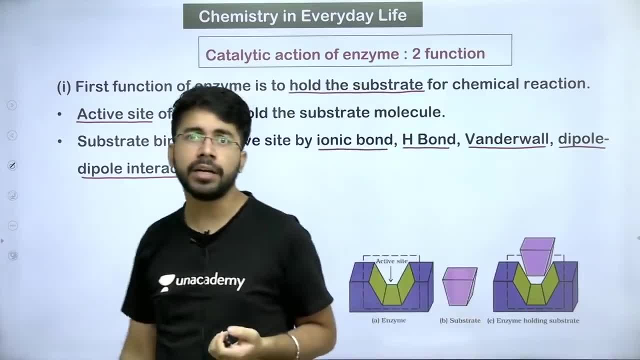 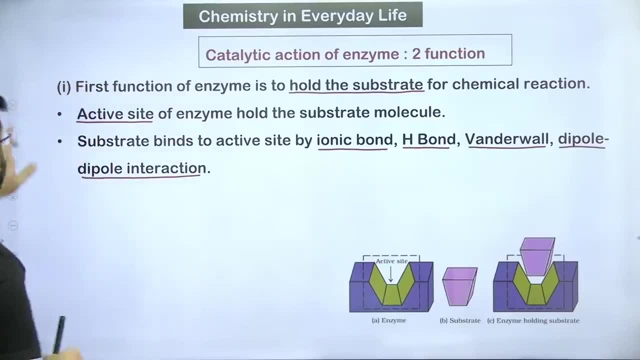 Now, what will happen? if we have to do the reaction, We will have to put a functional group in it from outside, Or we will have to put a chemical reagent from outside. Then it will do the reaction. So, my friends, the second function is: 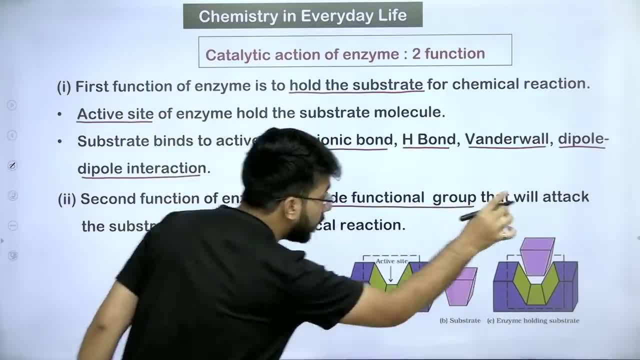 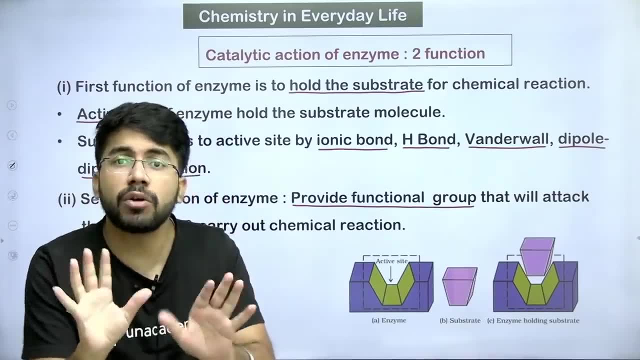 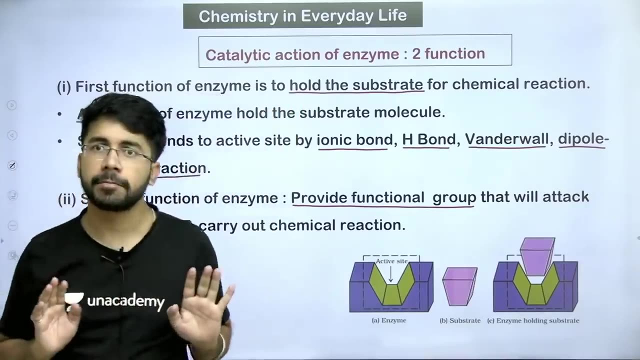 Provide functional group that will attack the substrate and carry out chemical reaction. Actually, we have a medium of enzyme, What is catalyst? We have a medium Where two reactant molecules come, They do the reaction And they make their product and leave. 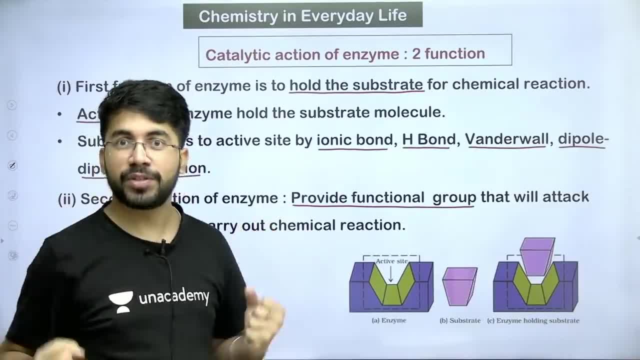 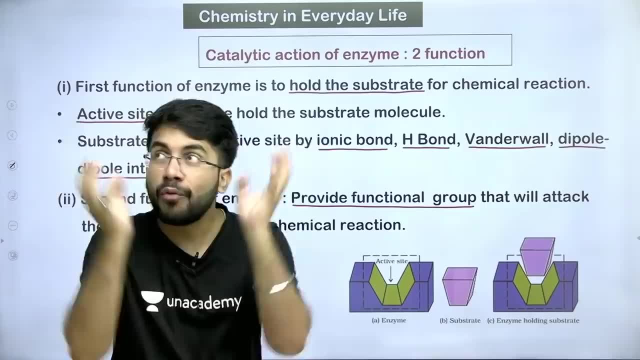 Like your restaurant, Like your OU rooms, Like your hotels, Like your many things Park. This is a medium, my friends. Two people come there, Two people come to the restaurant. One will talk and talk And will make their product and leave. 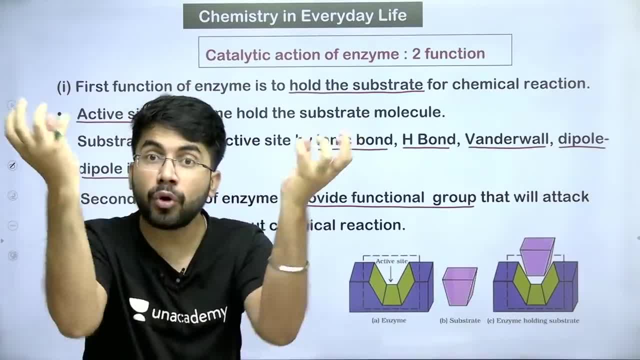 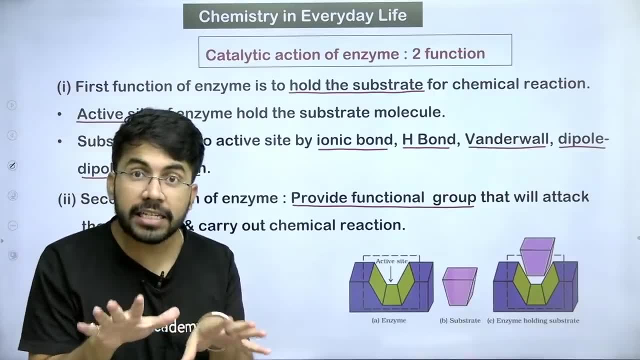 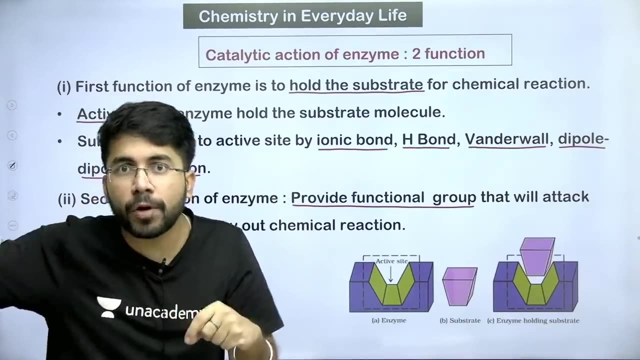 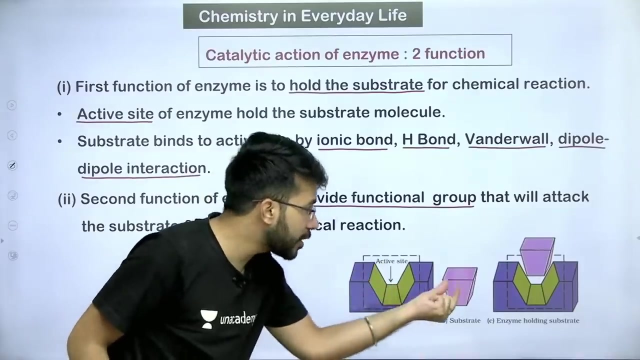 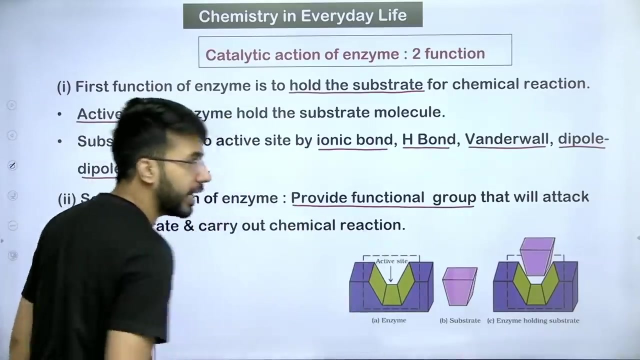 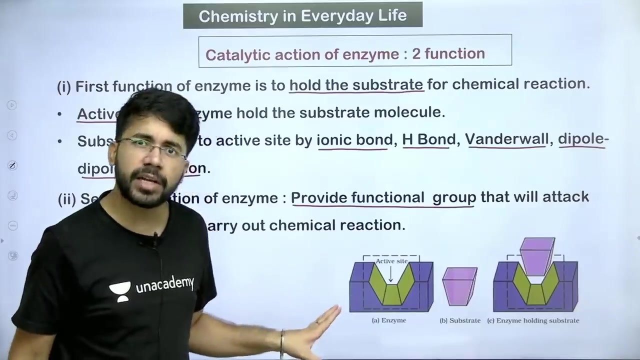 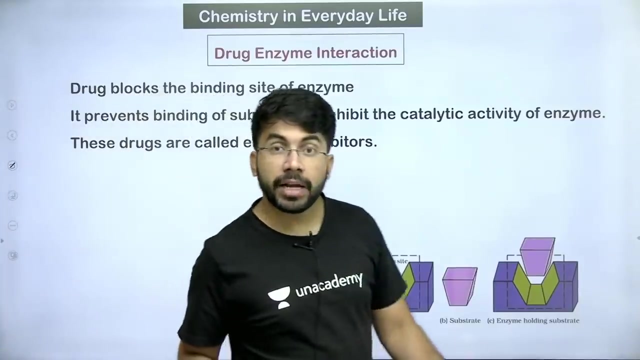 Restaurant was only a medium Where two reactant molecules come. They react, Make their product and leave. So catalyst, What is catalyst? We have a medium Where two people come, Two reactant molecules come, They both react. The catalyst also works the same way. it gives its own space. now the substrate will get stuck in this space. now the substrate will do the same thing. the other molecule will provide the functional group which will react with it and make the product. so how the enzyme is working as a catalyst, you understood now what happens. let's say the enzyme is in our body. 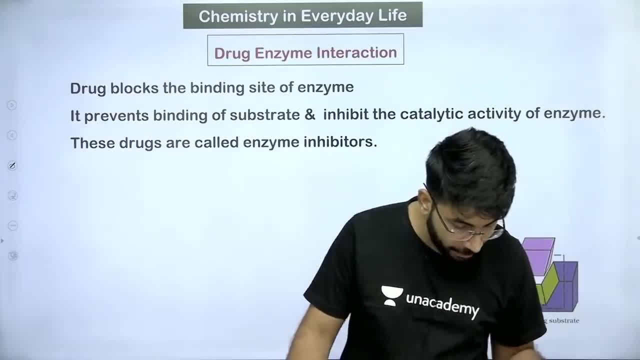 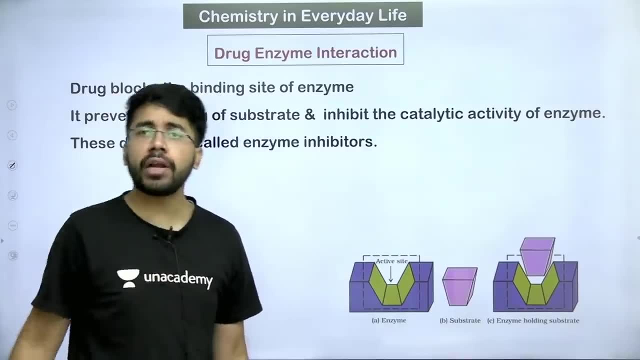 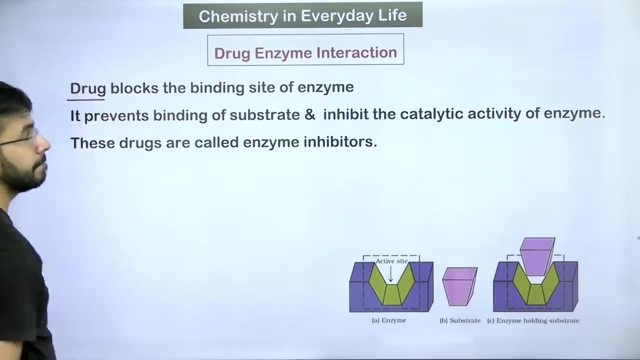 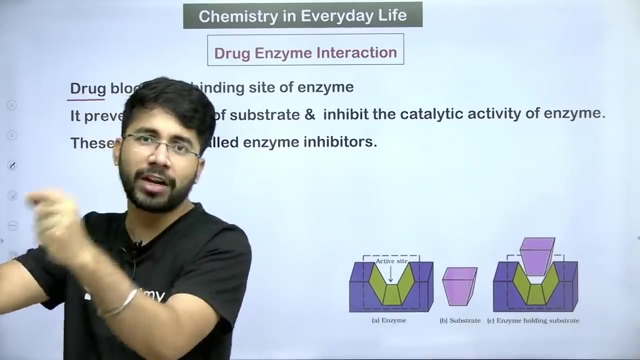 someone is doing the opposite reaction in our body. let's say, the enzyme is doing the opposite reaction in our body. okay, it is possible that the reaction it is doing here is harmful for our body. so what do we do? so we eat medicine for it as soon as we eat medicine. so what will it do? it will close that restaurant where two people are always coming meeting. the product is being made. that restaurant will have to be closed. only then the product will be made. 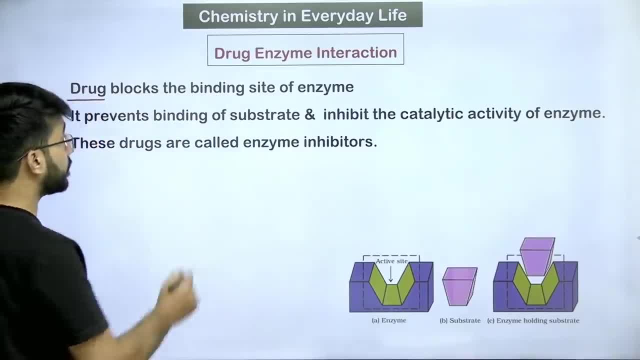 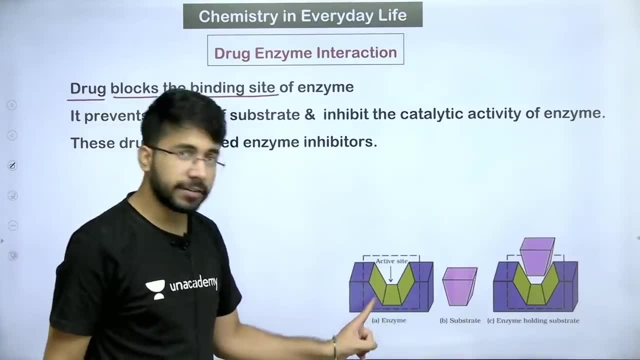 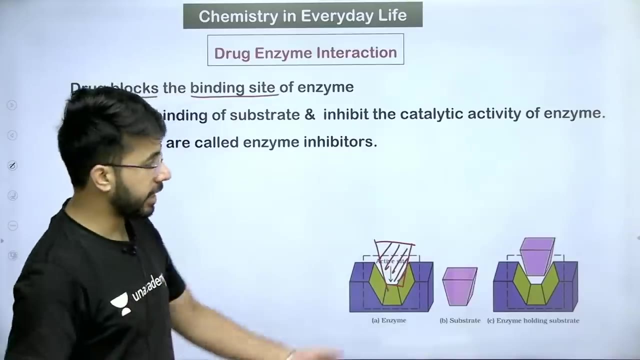 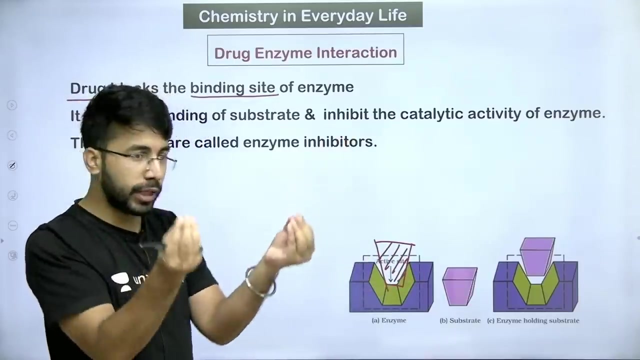 it will be closed. it will be closed. when we eat medicine, then that active site, that binding site, it blocks the medicine. what will it do? it will block it. it will come to this active site and sit itself. the drug itself will come and sit here. now, the substrate is not sitting. the substrate has not reached the restaurant. now, if the substrate has not reached the restaurant, then the other person will see that there is a drug sitting here. get out, get out, get out. we don't have, we don't have enough. 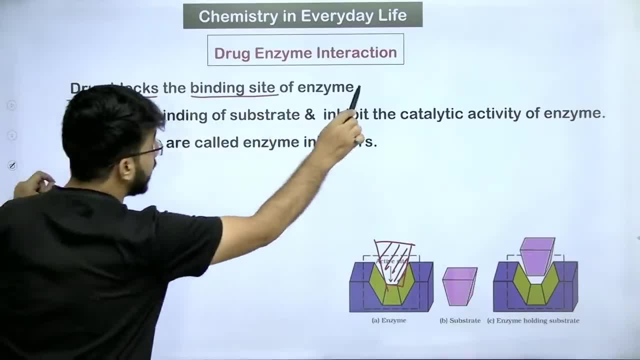 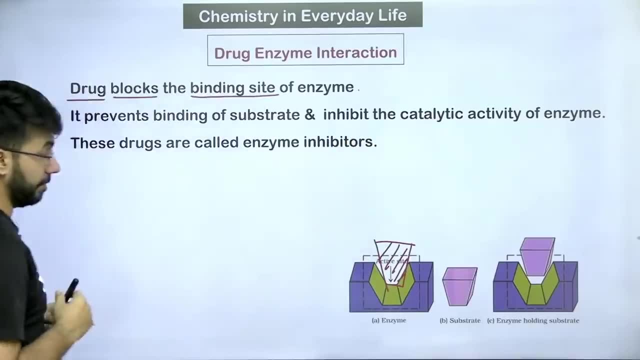 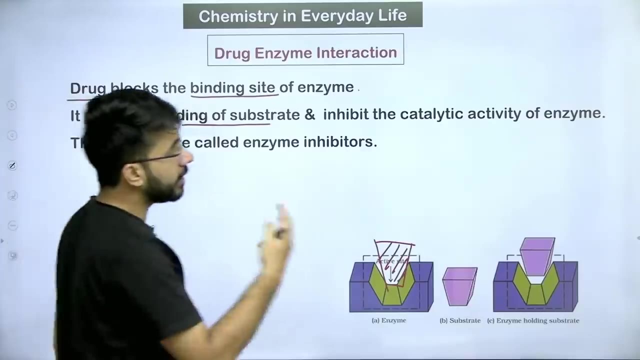 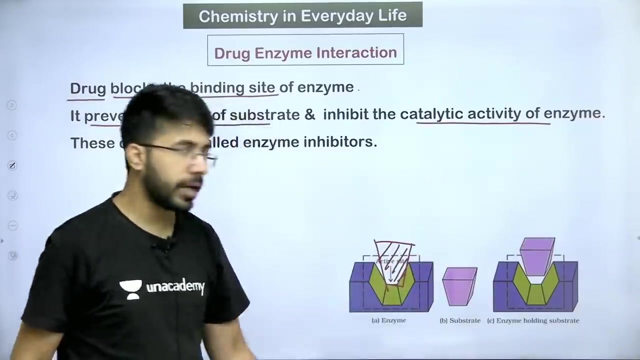 my friends, that's what happens. we cannot. that's what they will do. it prevents bindings. i will listen now. when the substrate does not come, when the functional group does not come, when there is no reaction, then theypy stop their work. 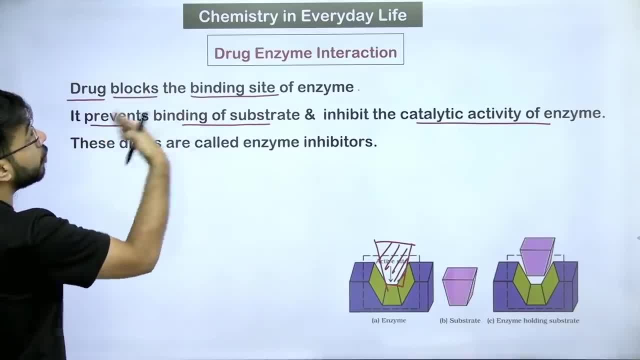 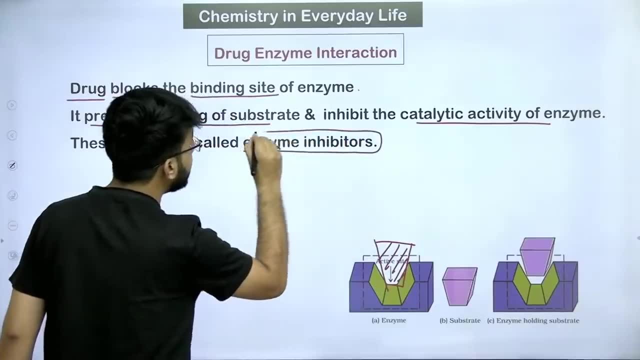 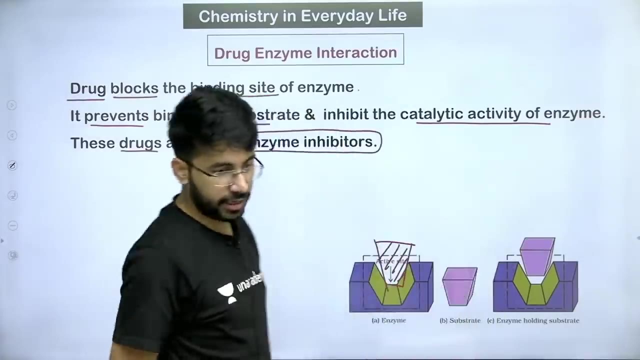 these drugs that is blocking that road. that is i. we are getting the restaurant closed. what is he doing? these drugs are blocking the. These drugs are called enzyme inhibitors. Enzyme inhibitors stopped the work of enzymes. Enzyme inhibitors stopped the work of enzymes. 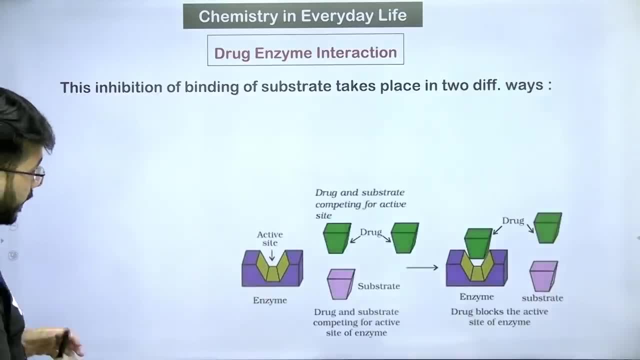 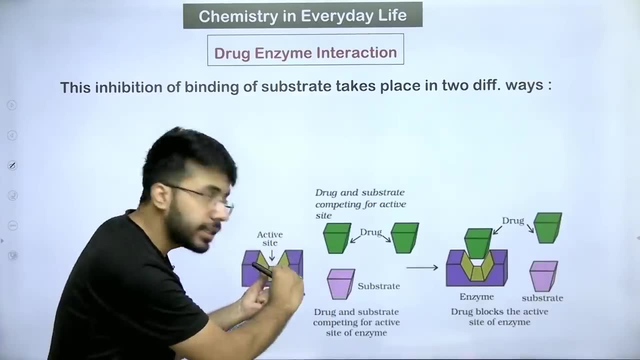 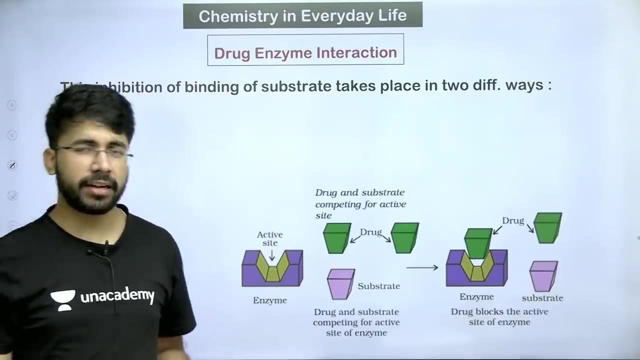 No problem. Now let's see. I have an enzyme, an active site. Now a substrate comes here, A functional group comes here, Both react, Makes a product, And this is wrong for some people. Now this is not seen by the drug. 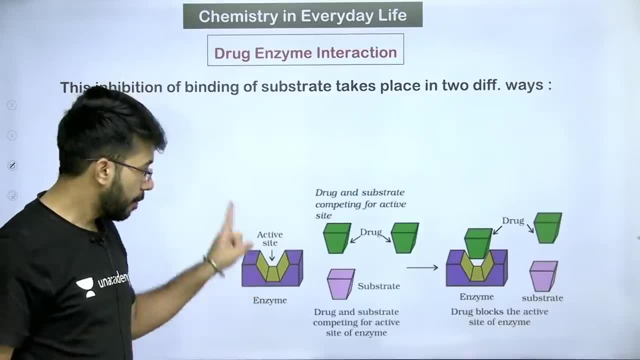 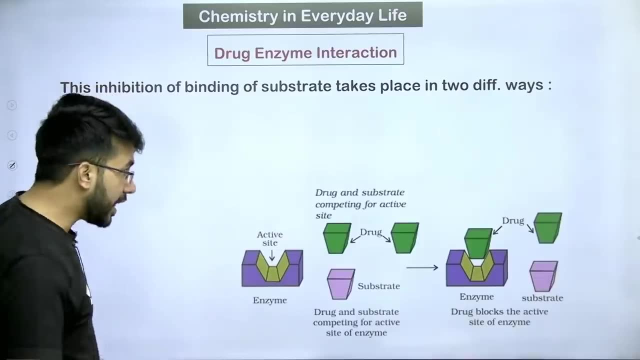 The drug says that it is enough. Two people are coming at the same place Making a product and going: Do one thing. You sit here yourself, Whoever comes, make a product from me first. So what happened? These two drugs will compete. 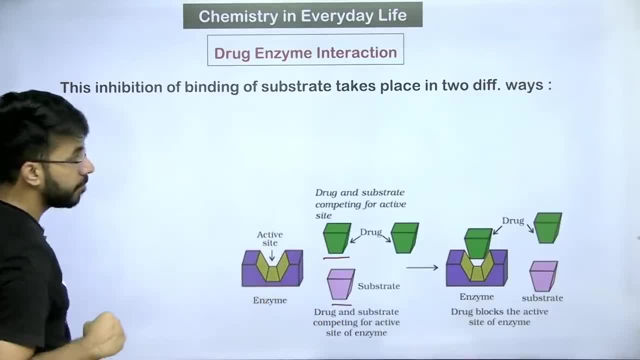 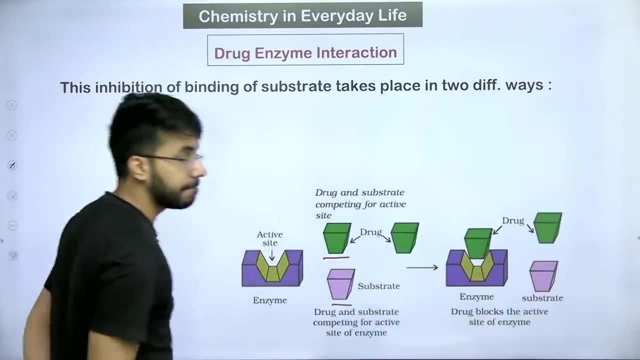 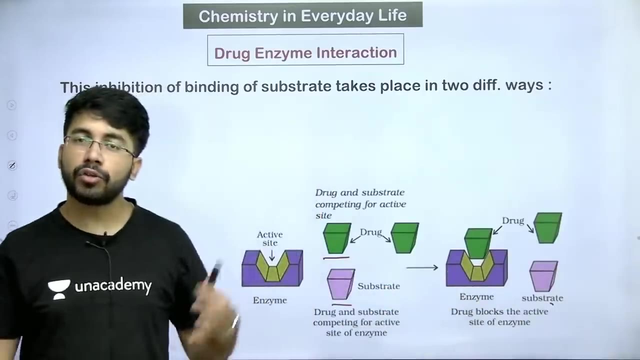 Substrate has to sit here too, Drug has to sit here too. Drug comes here much faster in this thing. So the drug came here and sat here. And poor substrate. So what happened? Substrate could not get medium, So two people could not get it. 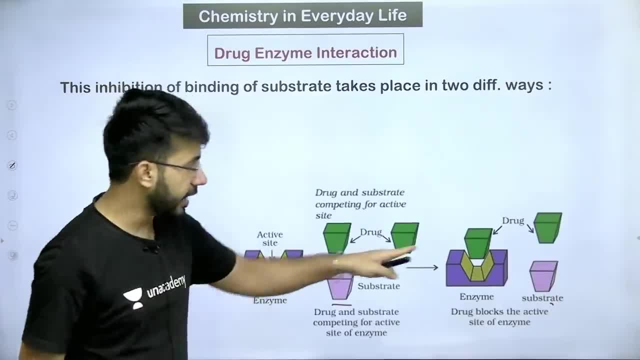 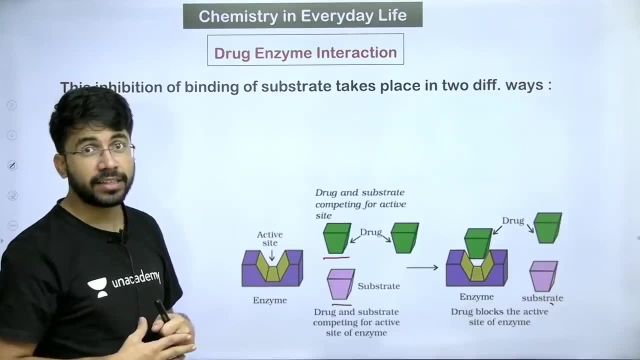 So the product could not be made. This is not a bajrang dal feeling, That brother. these two people do not want to get it. Substrate and functional group do not want to get it. So, my friend, what happened? Blocked. 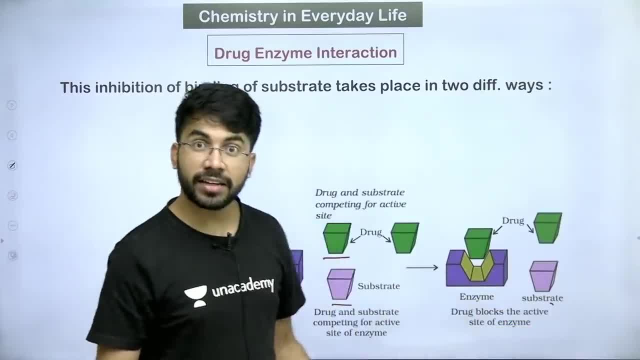 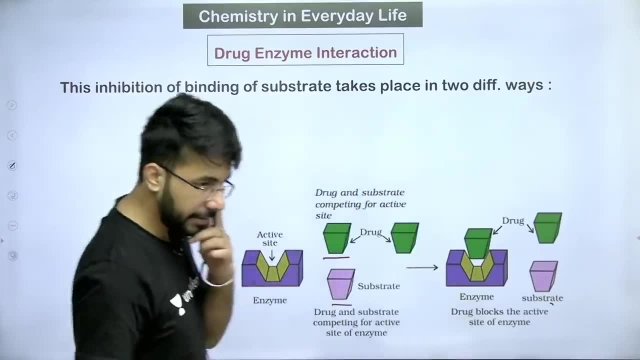 People are not coming from ahead. Come on, So take care of yourself. Okay, Medium See a little good medium Where there is no disturbance. Okay, Come on. So. the condition of binding of substrate takes place in two different ways. 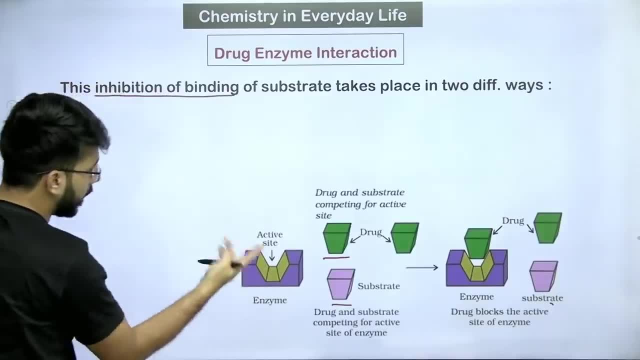 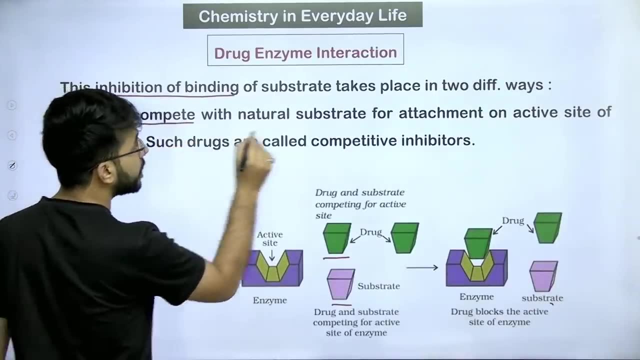 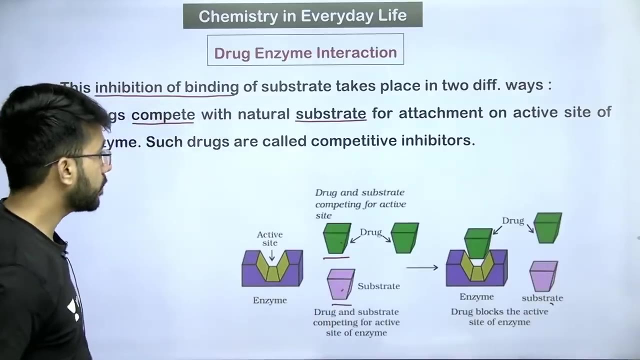 This is the drug. The drug which is binding of substrate, is doing it in two ways. What does it do first? What does it do first? This drug competes With whom? With the substrate Drug. competes with the substrate Drug. competes with the substrate. 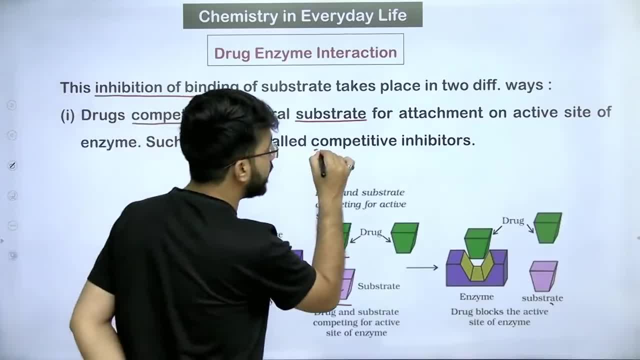 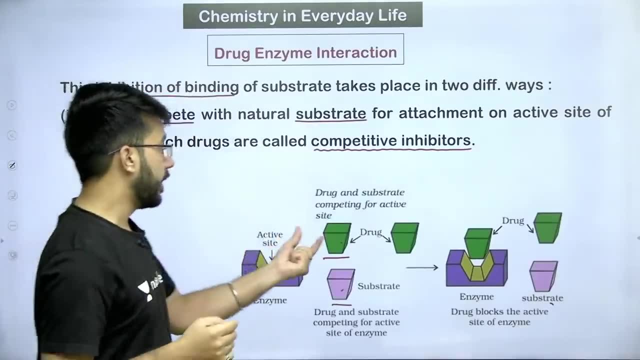 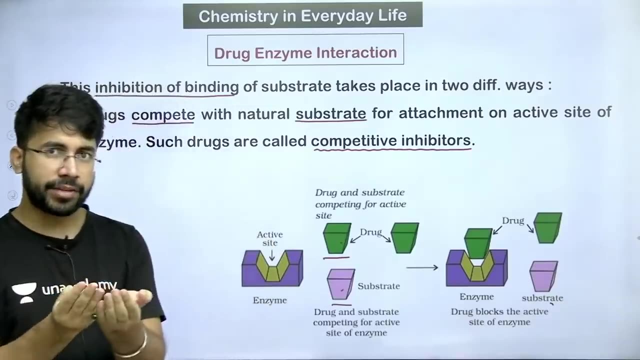 Okay, Such drugs are called competitive inhibitors. What happens, Actually? what happens? This drug is very clever. It knows that by going here, By going here In enzyme, Inside the enzyme, In the active site of the enzyme, There is going to be a milan of substrate and functional group. 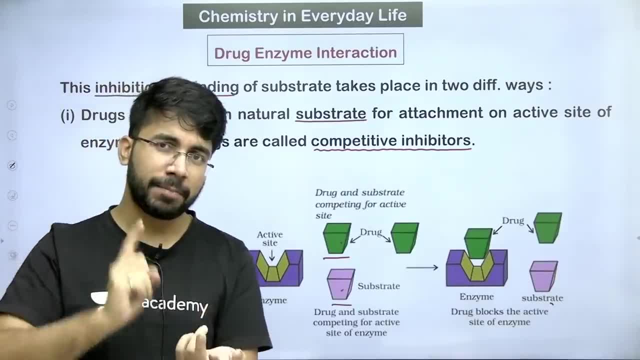 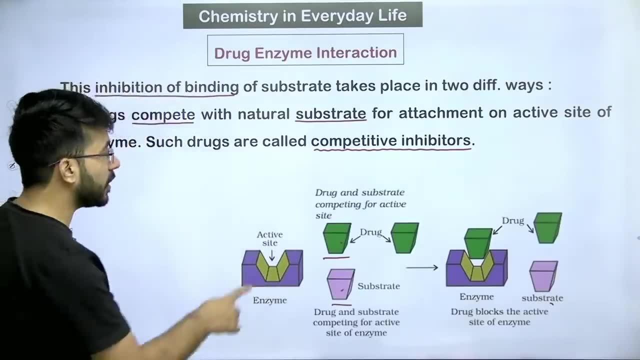 It says that if I reach before the substrate Then I will get the functional group. So it reached first in the circle of competition And reached first, It feels that it is a competitive inhibitor. It will reach first. No, no, no. 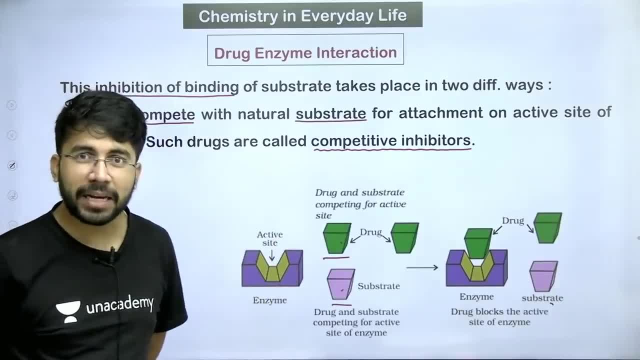 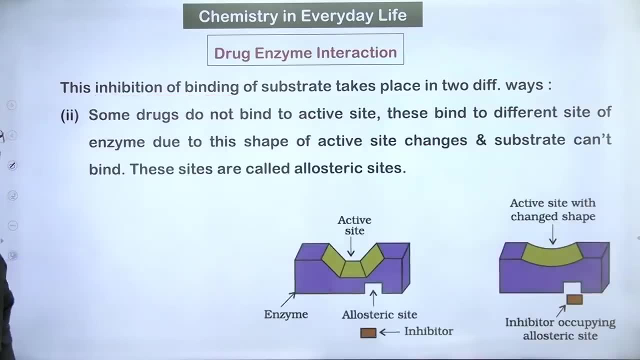 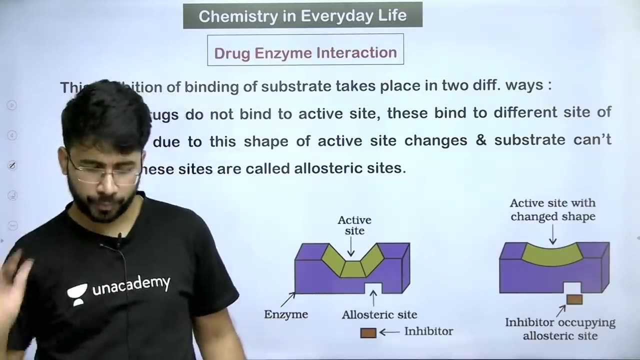 We are first, We are first. Okay, It reached first, And this drug reached first from the substrate. So Competitive inhibitors Second. There is one more way. One is to go and sit there yourself, Where there is an active site. 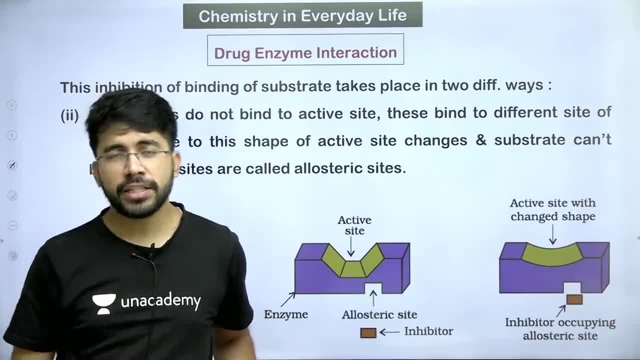 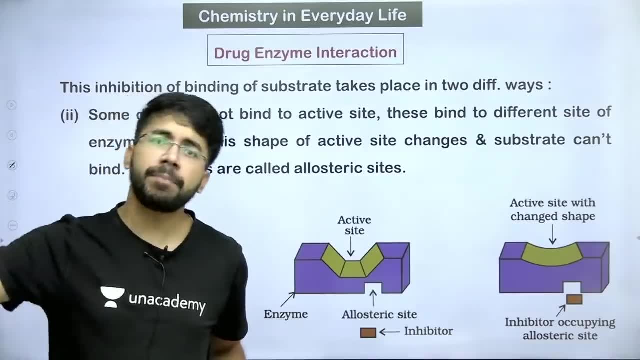 Or Waste the active site. Go and get water on the active site. Go and get a bottle of sauce on the active site. People could not sit there. Go and make a fuss there, Break the small bombs there And do that. 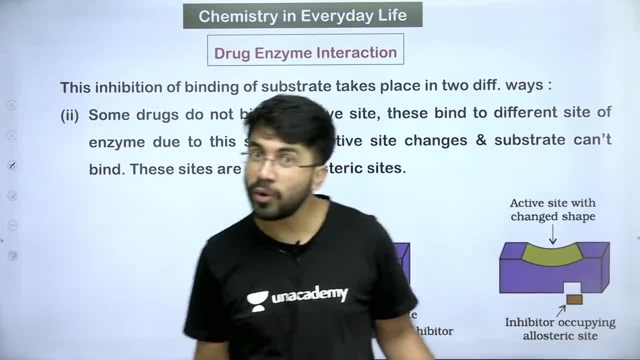 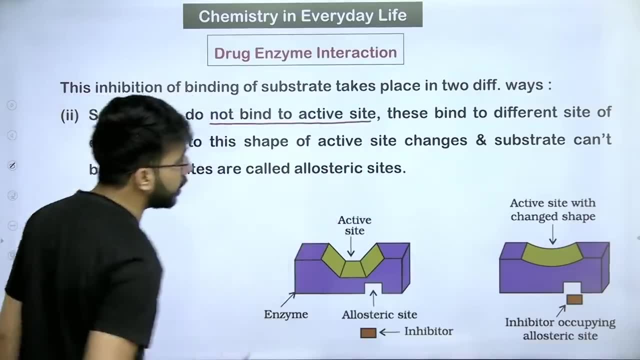 Terrorist attack happened, Something like that. Okay, So two people will not be able to meet there again. How will it happen? What is the second way? That, friends, Some drugs do not bind to the active site, Some drugs do not come on the active site. 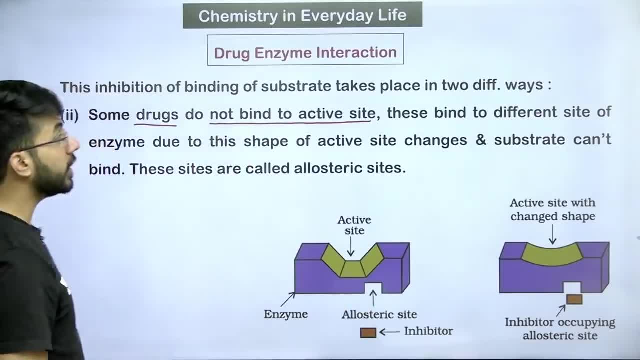 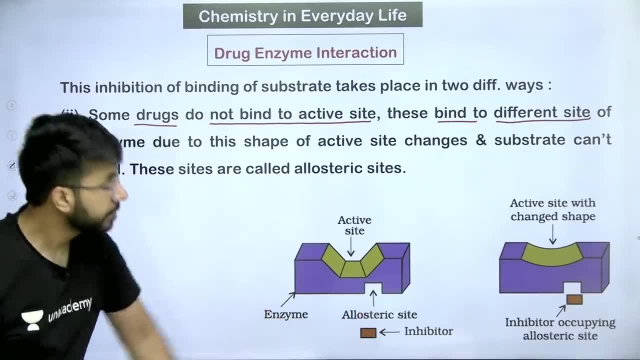 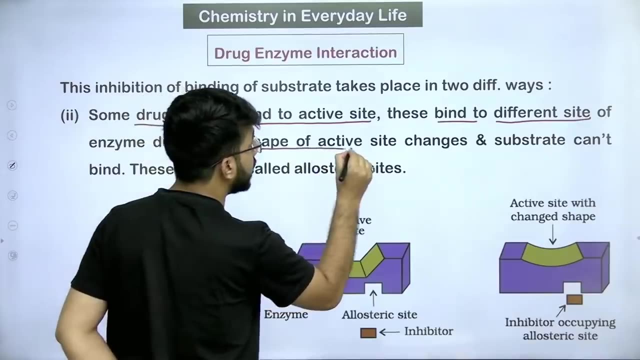 It goes somewhere else and attacks. What will happen? See, These bind to different sites. They bind, but they are on different sites. They are on different sites. Okay, And what is happening by binding on a different site? Shape of active site changes. 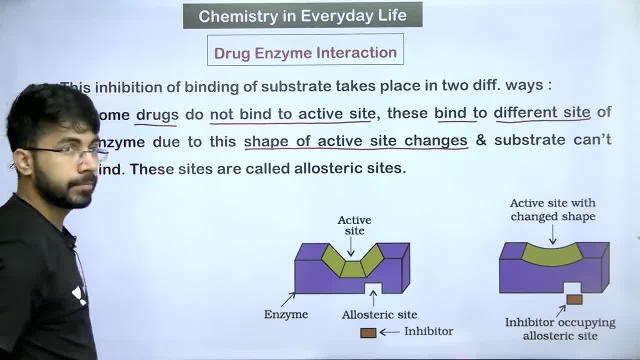 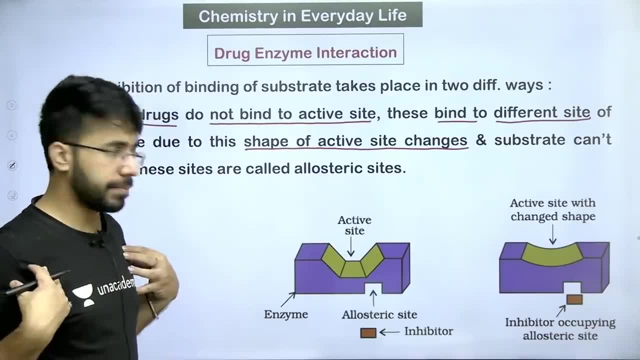 The shape of the active site changes. The drug is not sitting here now. It will sit in the competitive inhibitor. But what is happening now? It is saying that if it is not ours, then it will not belong to anyone. Okay, If it is not ours, then it will not belong to anyone. 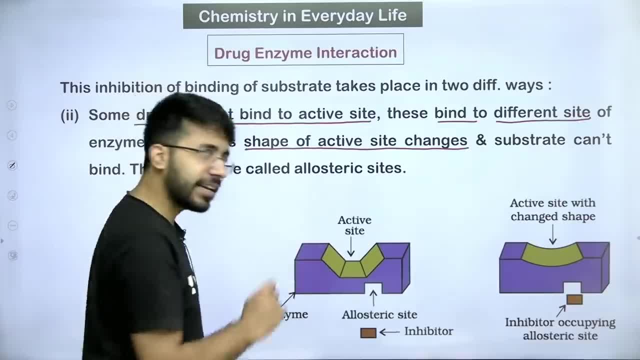 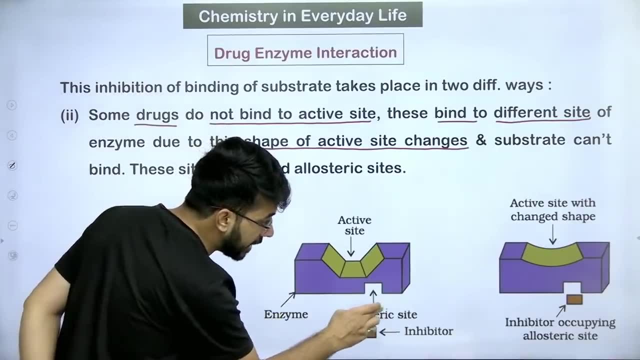 So that happened. It is not sitting there, It does not want to do anything, But it is telling others that we will change the shape and size. So what is happening? It goes here and sits in the allosteric site. It goes to the allosteric site and attacks. 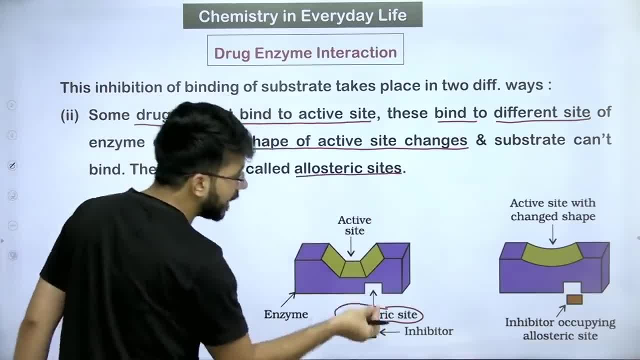 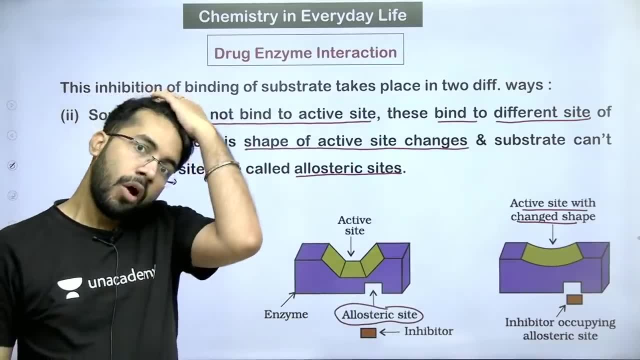 Okay, These sites are called allosteric site. It gets attached to the allosteric site And due to which the shape changes, Due to which the shape changes And the shape changes. What do we call this, Friends? The shape changes. 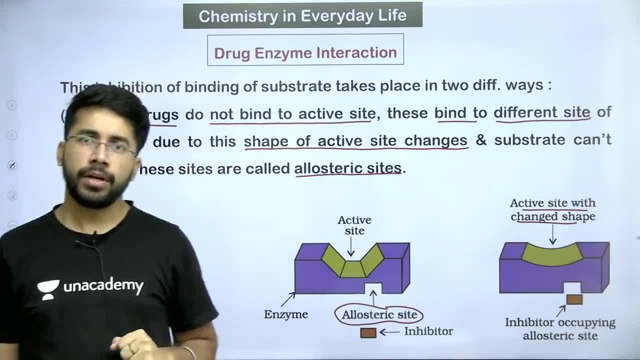 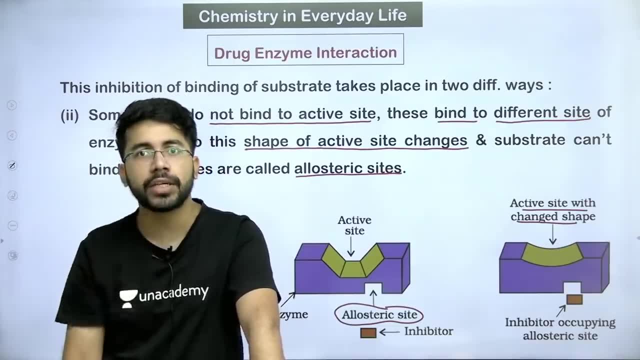 So the drug is working as an inhibitor in two ways. Drug One is to go and block the place yourself Or go to the allosteric site from the other place So that the place changes, The shape changes. And if the shape changes then the substrate will not be able to sit by itself. 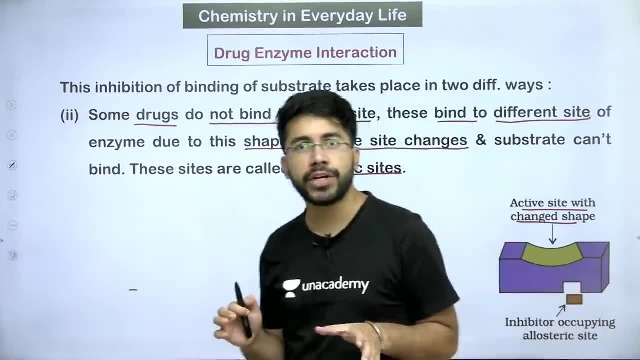 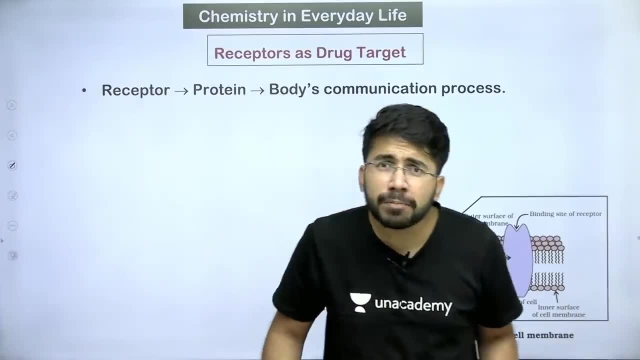 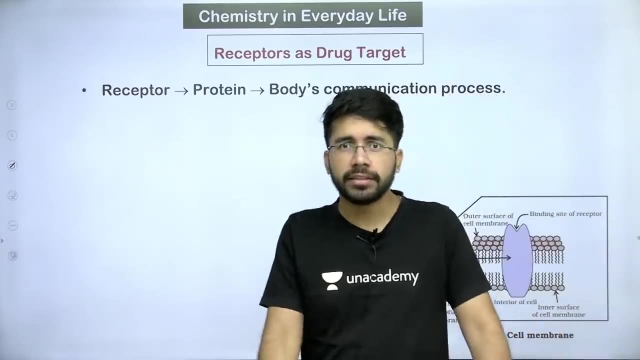 So you understood how drugs and enzymes interact inside the body. Okay, Now comes my friend Receptor as a drug target. Suppose you are studying science. Your receptor is not working. Your receptor has to do something else to the body. Suppose you have come into hypertension. 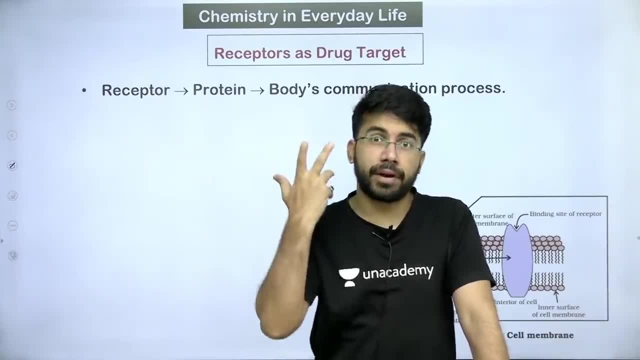 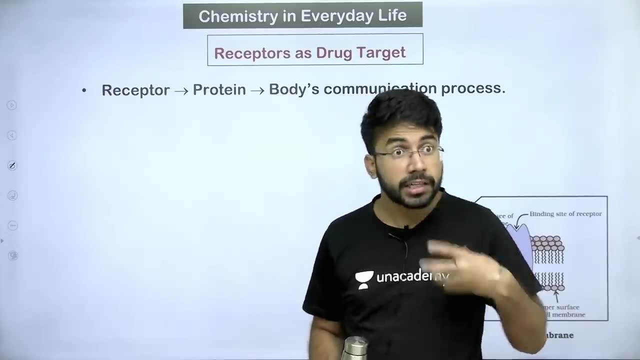 Where your receptor is working as an overactive. Many people have the problem of excitement. They get very scared when they see many things, So their receptor is working as an overactive. So even there we give drugs. So how does that drug interact with the receptor? 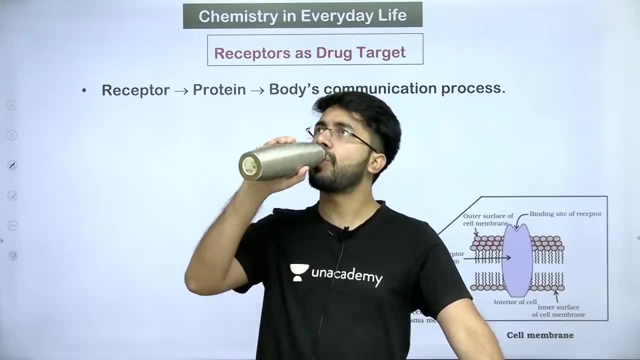 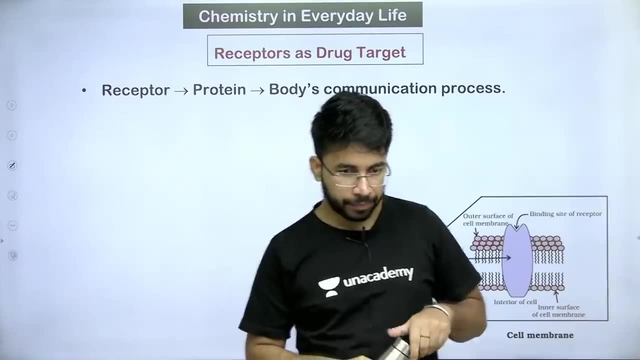 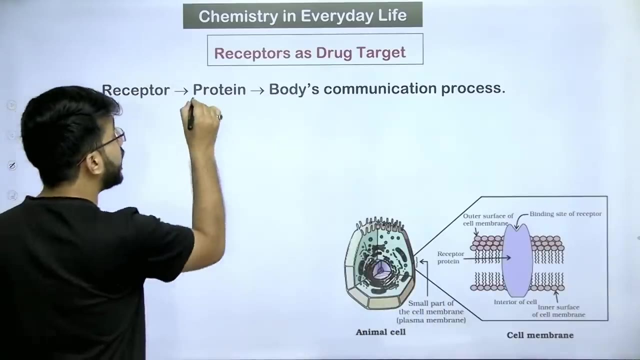 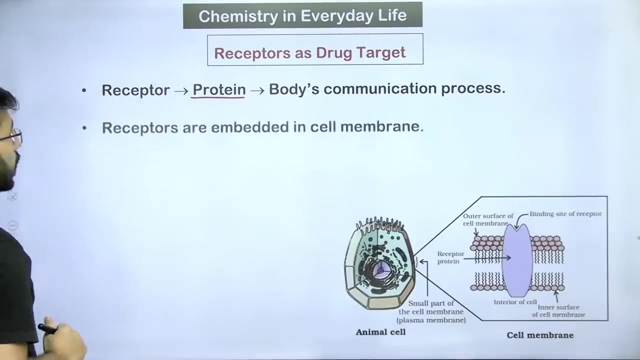 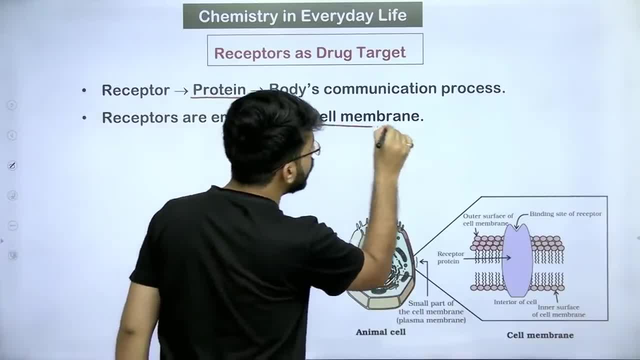 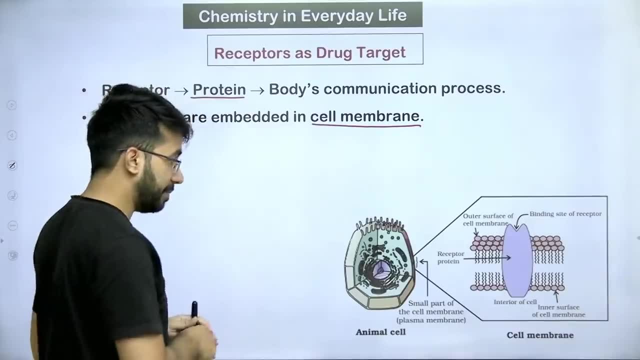 Receptors are embedded in the cell membrane, Our cell membrane. I have no idea about this, by the way, But still To study chemistry in everyday life, You have to get the idea We have animal cells. Okay, The receptor is inside this animal cell membrane. 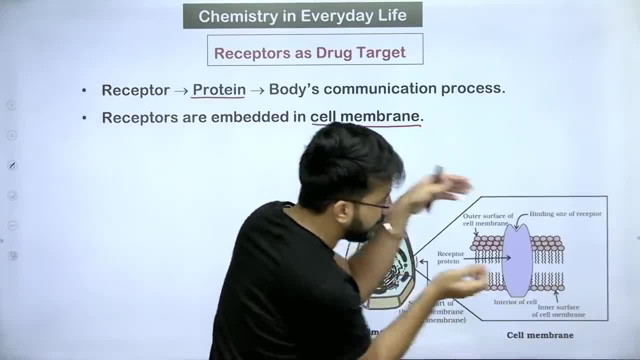 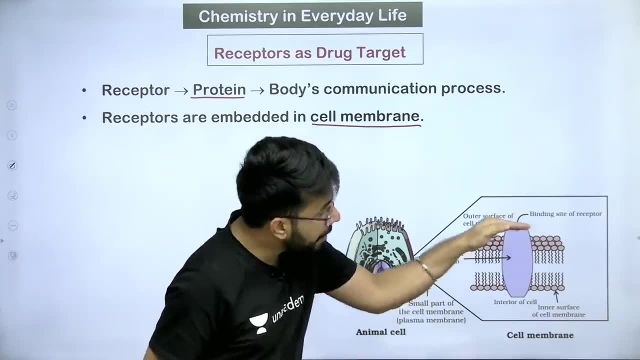 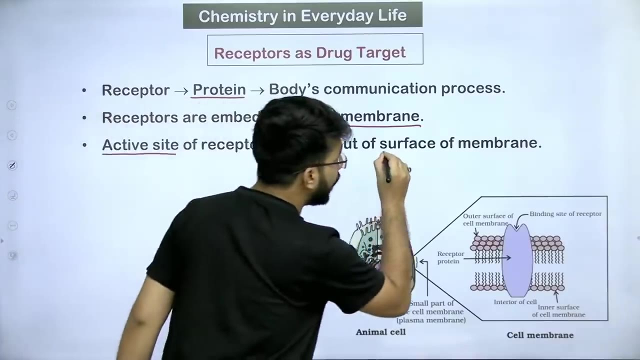 The receptor And its zoom view is shown here. The special thing about the receptor is The active site of the receptor Is coming out of the cell membrane. The binding site of the receptor, Or the active site of the receptor Is coming out of the surface of the cell membrane. 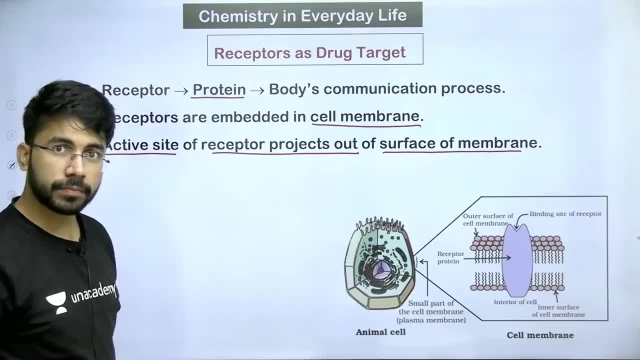 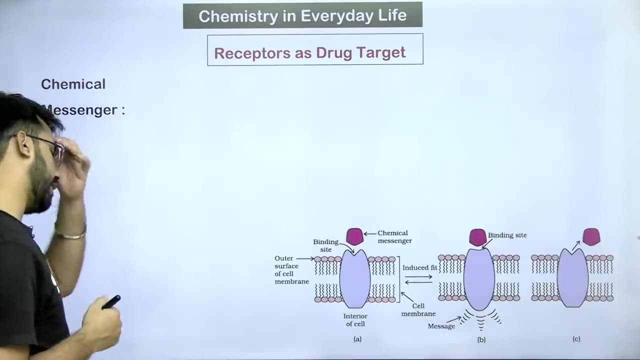 Projects out. Okay, Now understand. Here you can see the active site. That active site Is projecting out of the cell membrane. Now suppose a drug comes. Suppose a drug comes. Now what will the drug do? Okay, What is a chemical messenger? 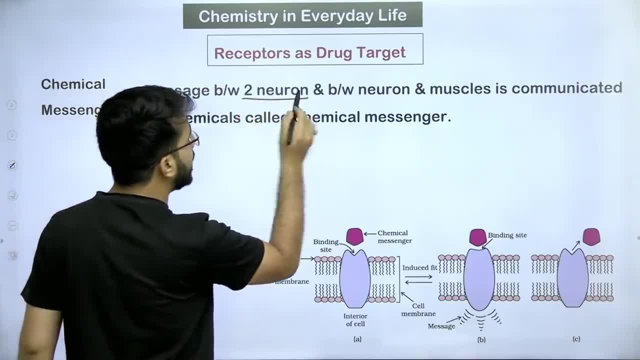 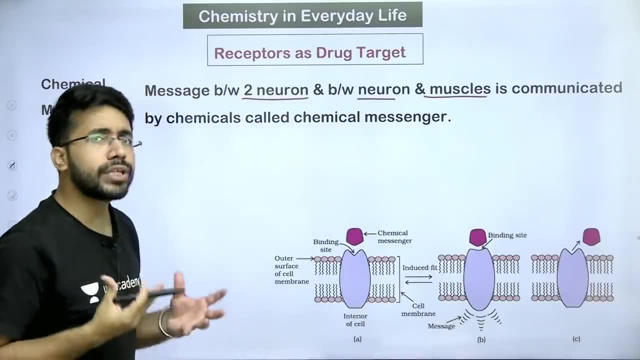 First of all, What is a chemical messenger? We have to transfer the message between two neurons, Or We have to transfer the message between the neuron and the muscle. For that There are some chemical requirements, And that is what we call a chemical messenger. 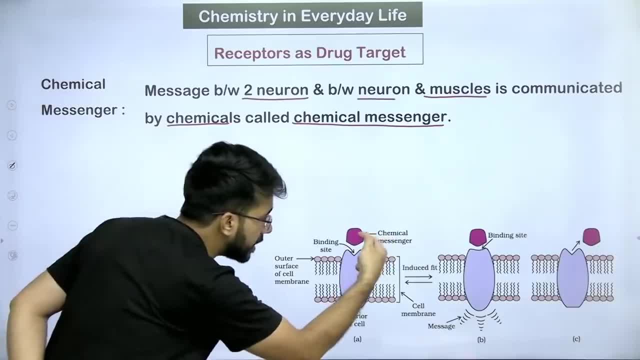 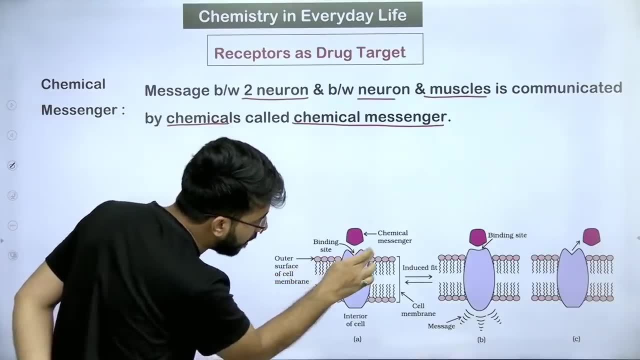 Okay, What does it do That? we are getting a chemical messenger in it. Why is a chemical messenger coming in the form of a drug? This is a binding site Which is projecting out of the cell membrane. Now the chemical messenger will be attached to it. 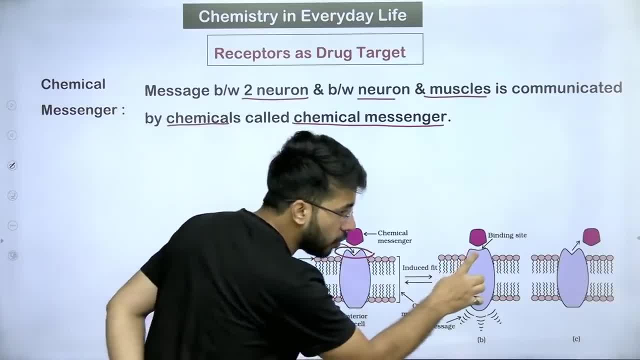 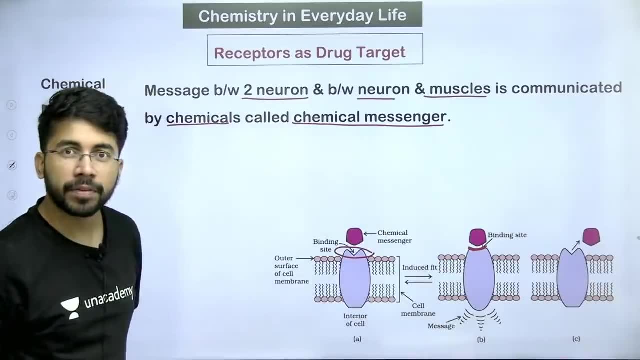 As soon as it is attached, My friend, As soon as it is attached, Its shape has been changed, Can you see, As soon as it is attached, Its shape has been changed And, because of this shape, changing The message which it had to signal. 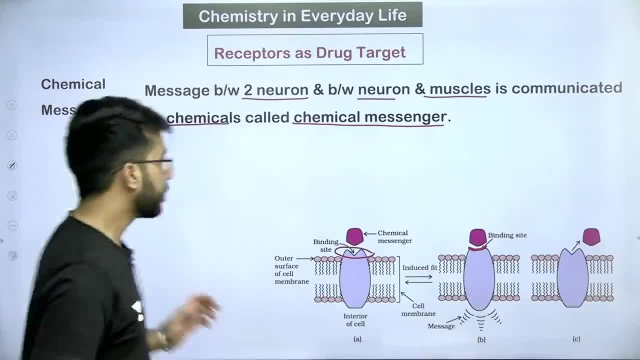 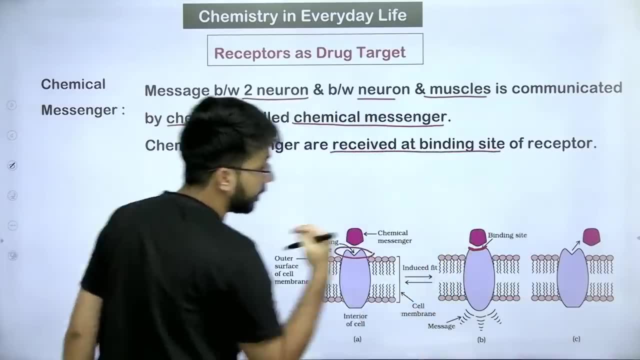 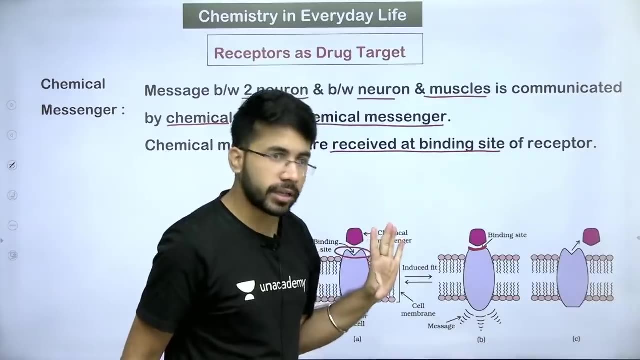 The message that was to be sent will be transferred Here. the chemical messengers are received at the binding site of the receptor. The chemical messengers have come at the binding site, Its shape has been changed and the message that was to be sent has been communicated. 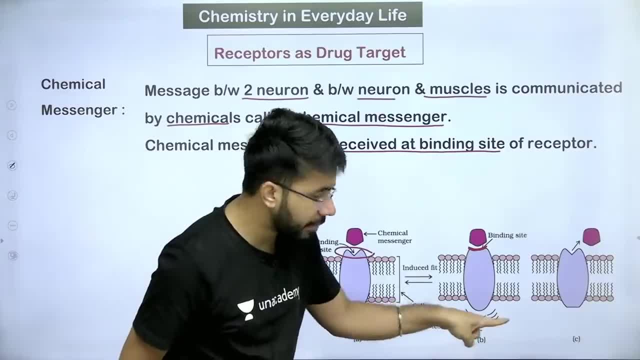 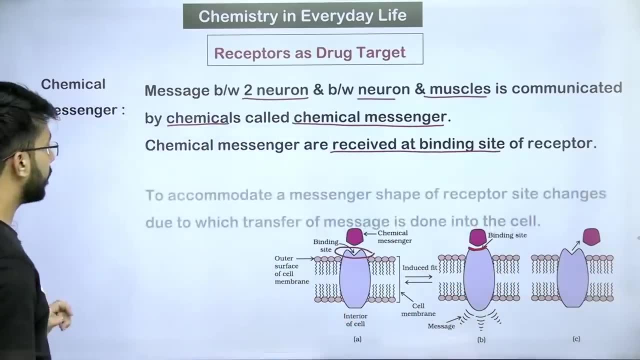 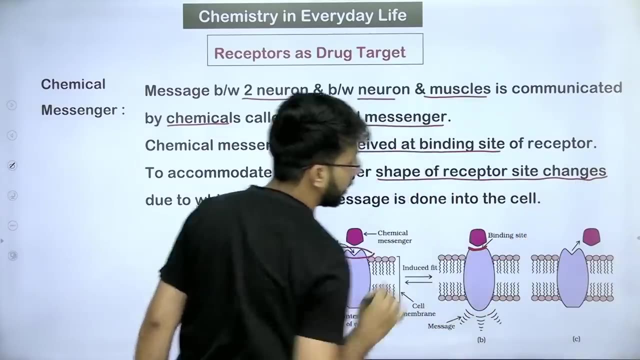 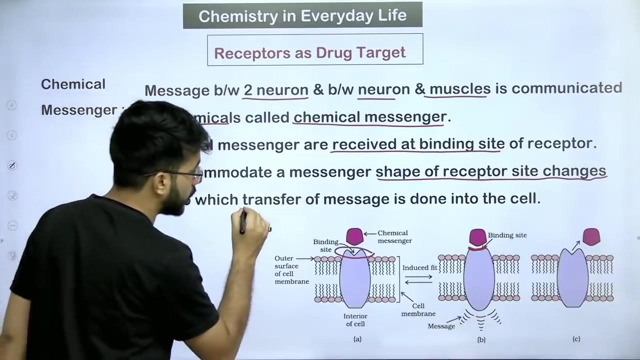 You can see, the message is being communicated. A tower-like symbol is being created here. Finally, the chemical messenger will be sent separately and the binding site will regain its position To accommodate a messenger. the shape of the receptor site changes. The shape of the receptor site changes, due to which transfer of message is done into the cell. 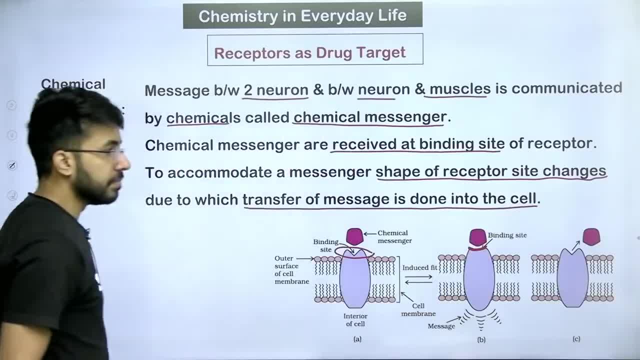 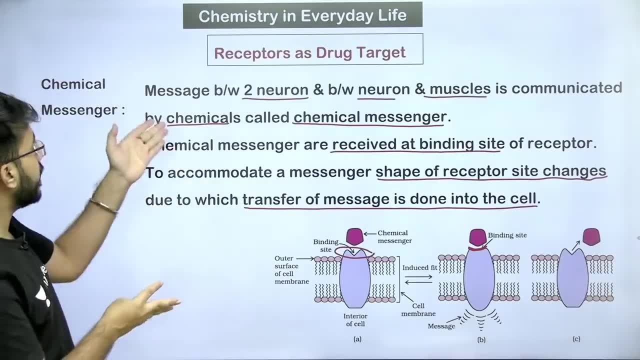 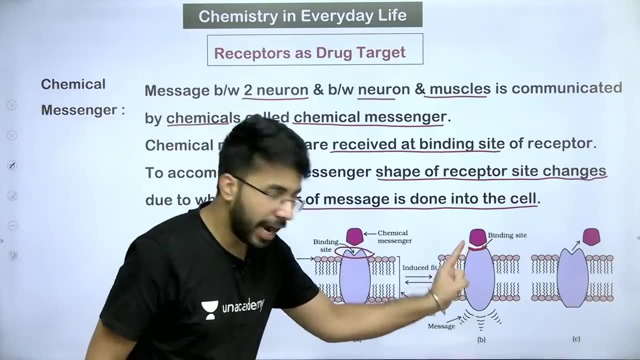 Because of this, the transfer of message is done in the cell. Message between two neurons, neuron and muscle, is communicated by chemicals called chemical messenger. Chemical messenger is received at the binding site, The shape of the receptor site changes and the message is transferred. 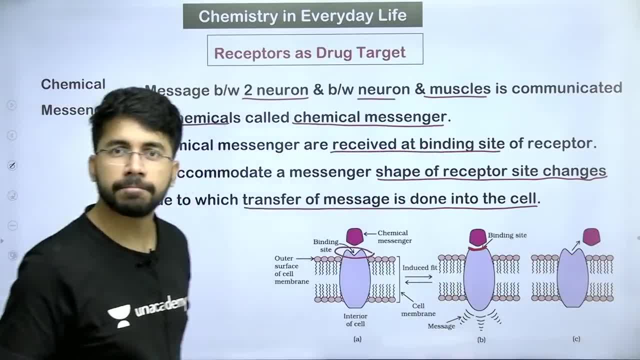 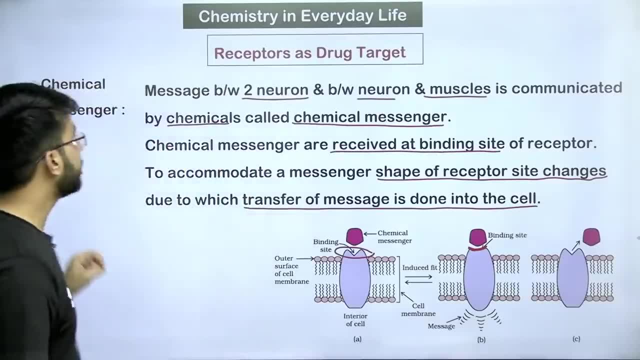 Again, the chemical messenger is sent separately and the shape of the receptor site is regained. So this is how the receptor and the drug target interact. Let's move on to the next topic: What is an agonist and what is an antagonist? 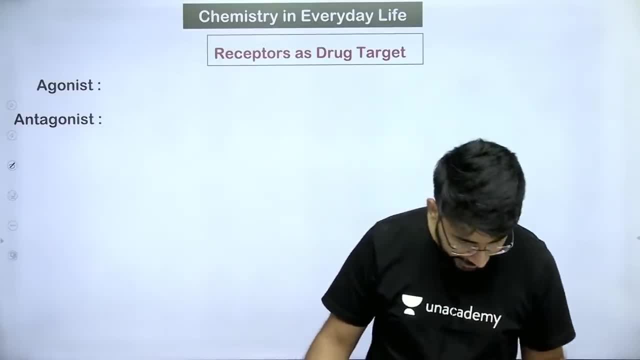 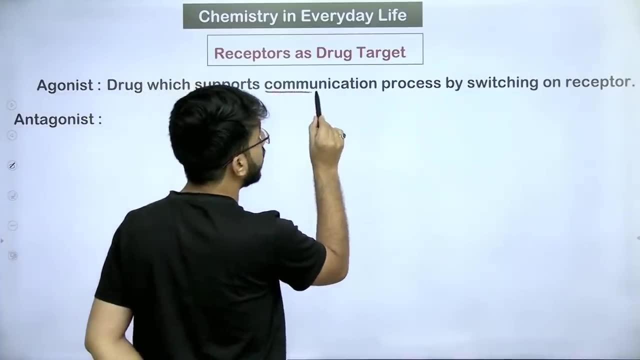 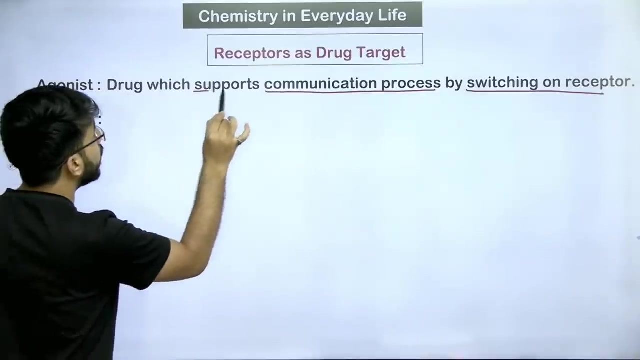 Does anyone know what an agonist is? Does anyone know what an agonist is? An agonist is a person who supports the communication system, Who supports the communication system. by switching on the receptor, He will start the receptor and support the communication system. 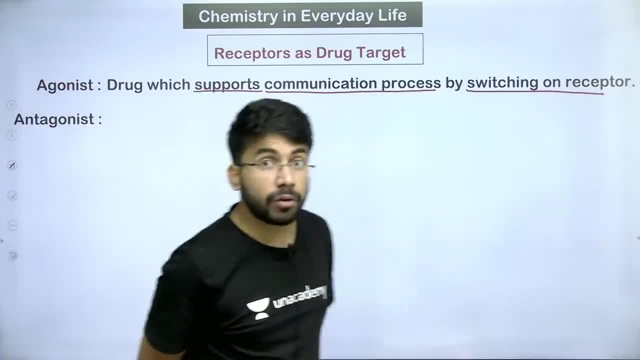 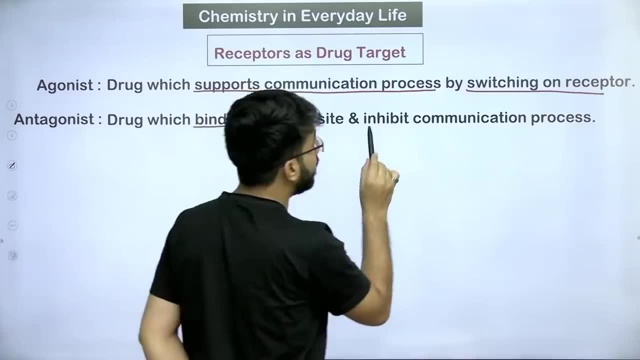 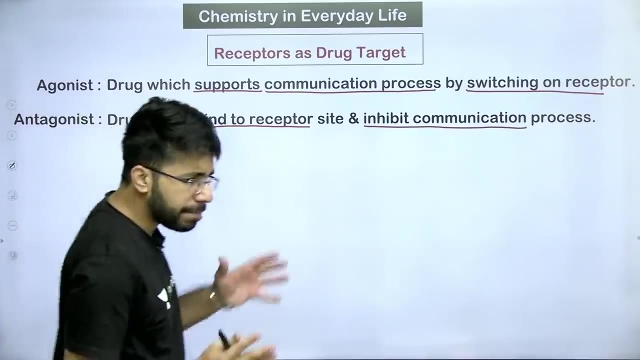 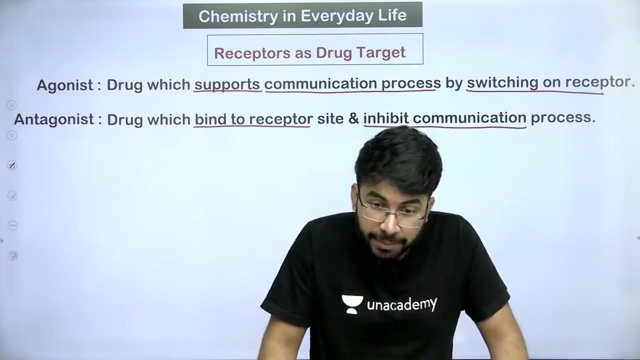 What is an agonist, my friend Antagonist is a drug in front of you which binds to the receptor and inhibits the communication, That which is bound to the receptor, The drug that is attached to the receptor. It sticks to the body and inhibits the communication system. 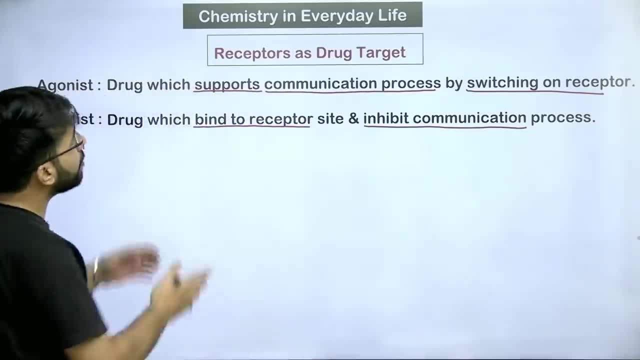 It will work the other way around: If you are lazy, then you will need an agonist because you have to support your communication system, And if you are a patient of overactive receptors, then you will need an antagonist because he reduces the receptors. 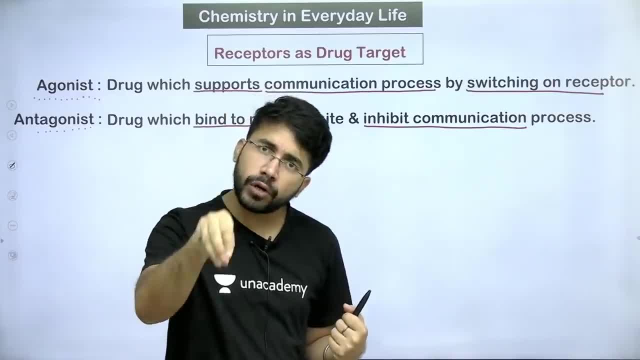 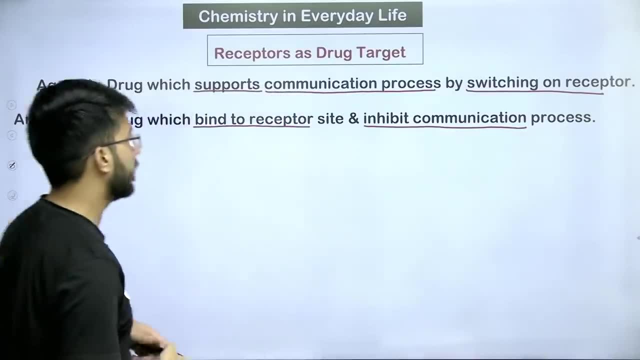 And it all happens through chemical messaging. Any drug that comes, it comes through the chemical messenger. The chemical messenger will provide its message that slow down. The chemical messenger will tell you to be fast. then you will start working fast. Let's move on to the next. 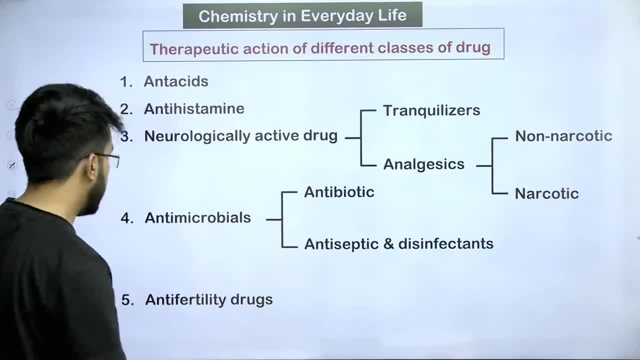 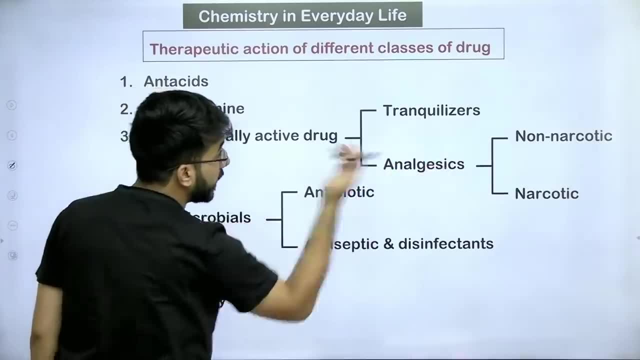 Now let's come to the therapeutic action of different class of drug. You have to read all these drugs: What is anti-acid, What is anti-histamine? What is tranquilizer? What is analgesics? What is antibiotic? What is antiseptic? 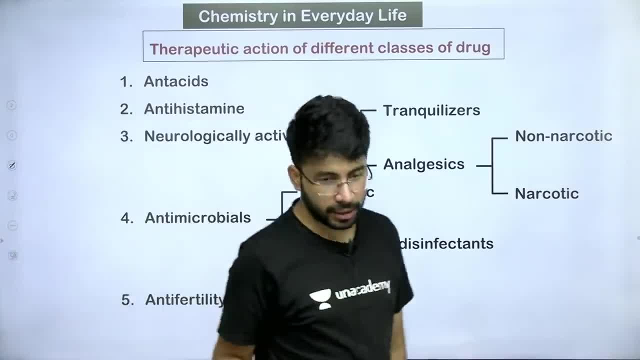 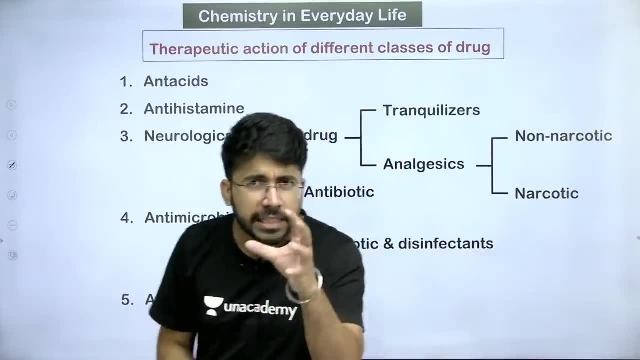 Disinfectant and anti-fertility drugs, Which are birth control pills. We have to read about all these Therapeutic action of different classes of drug. Let's go. What is anti-acid? What is anti-acid? Can you see this? 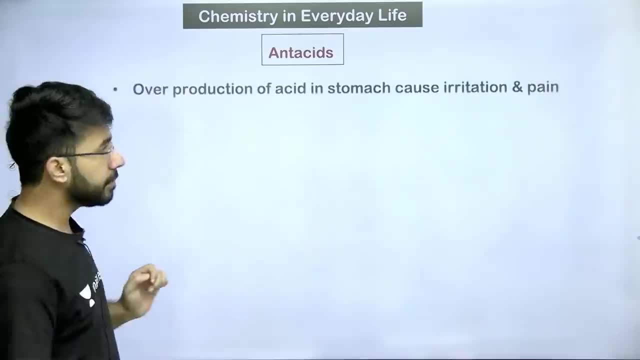 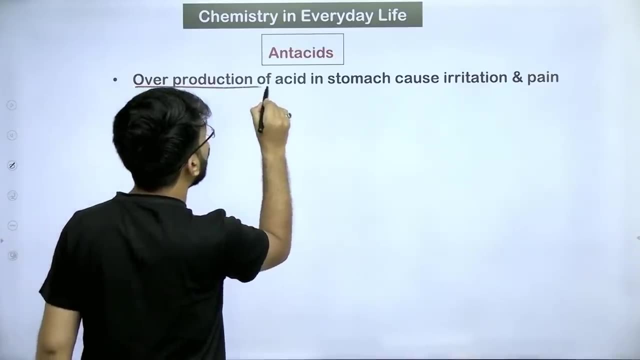 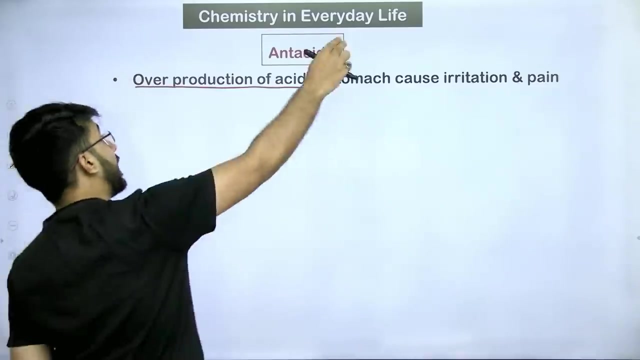 Acid is opposite to anti-acid. Let's move on to anti-acid. What is anti-acid Actually? what happens is overproduction of acid in our body causes irritation and pain. Right Anti-acid is given to prevent overproduction of acid. 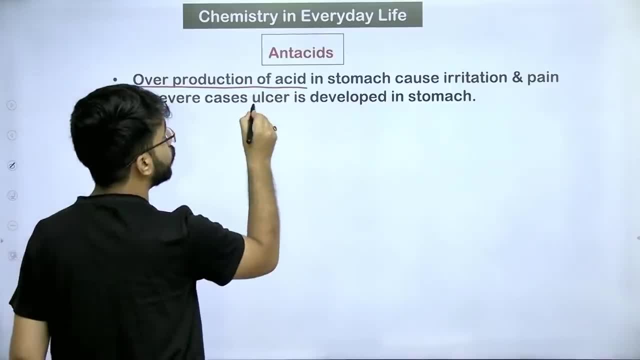 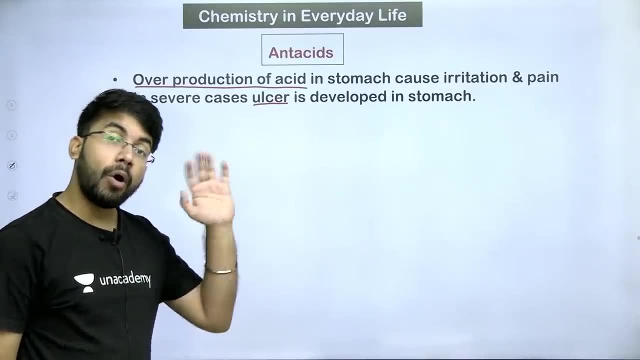 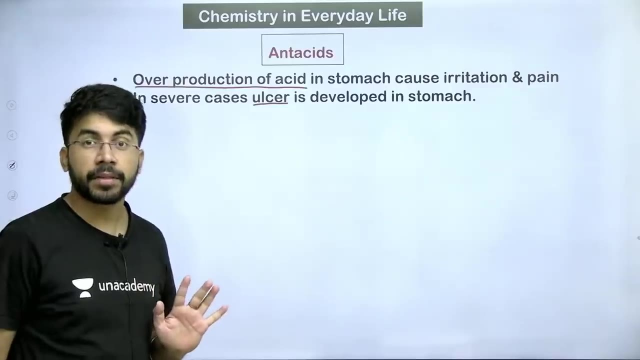 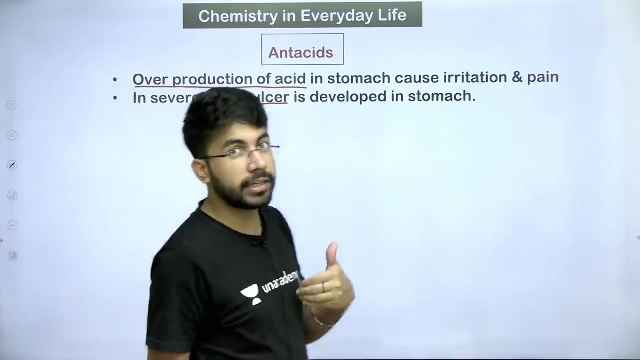 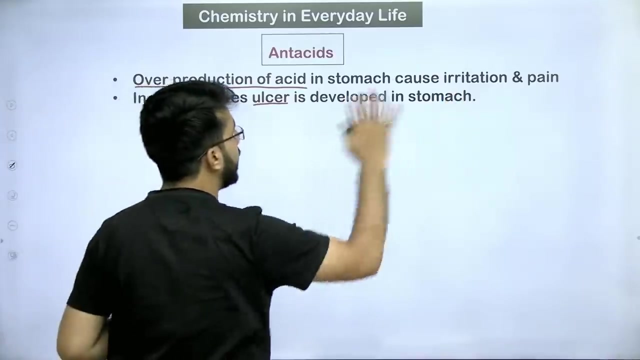 In severe cases, if too much acid is produced, then there is ulcer in the stomach. Right, If you have a very severe stomach disease, then what happens is that the affected part of the stomach has to be removed by cutting it off. it is such a dangerous disease so you have to have breakfast from time to time, drink water from time to time, save yourself from this. in terms of acidity, very small people take it, but it is a very big case. it is a very big case. okay, now, this is my friend. so overproduction of acid in the stomach causes irritation and pain. many times it has ulcers. there is also an ulcer in the stomach due to this. 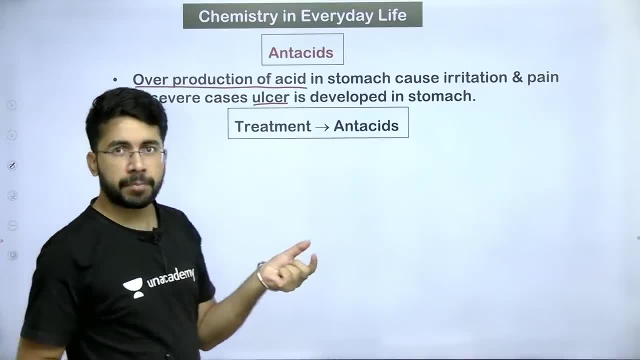 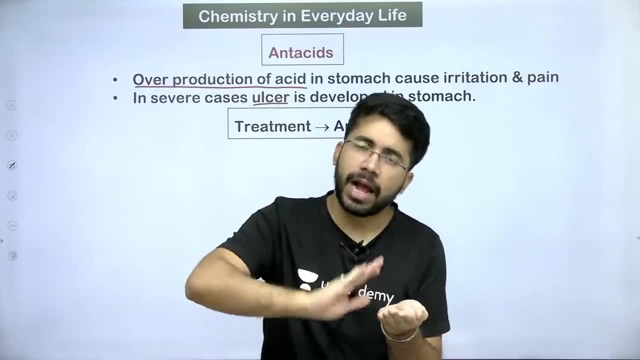 now I will tell you what is its treatment. so there are many anti-acids in the market, so anti-acid is its treatment. opposite to acid, you give base. anti-acid is base. what does that base do? it will neutralize the acid and base. your stomach will be fine. 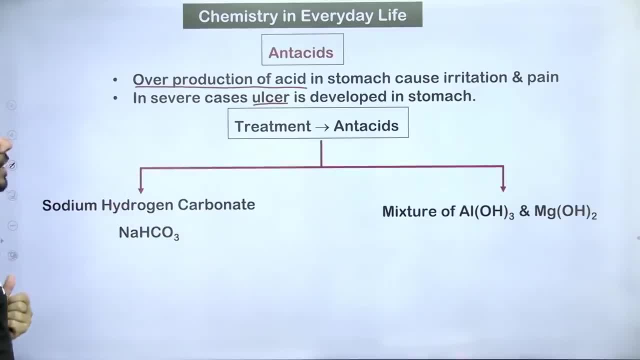 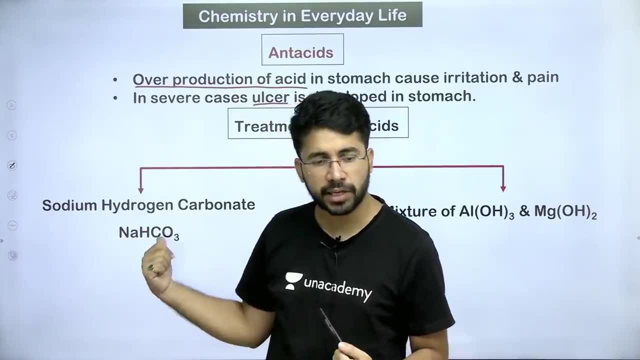 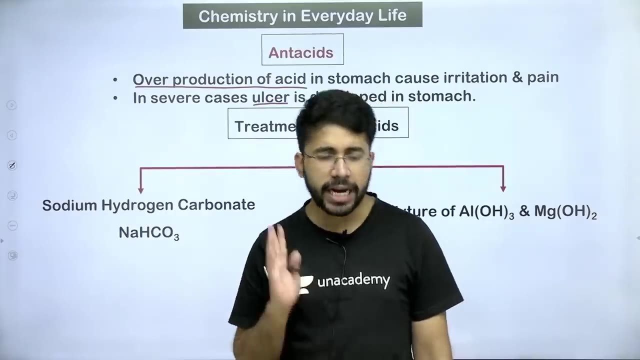 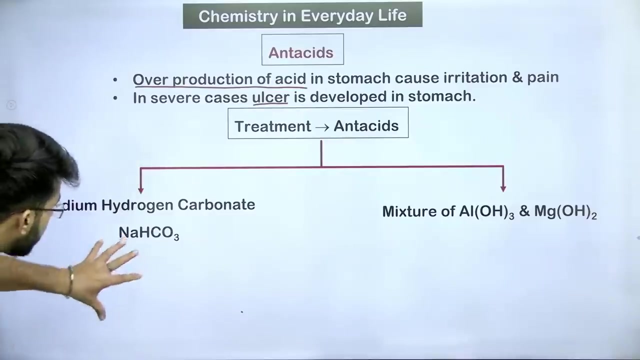 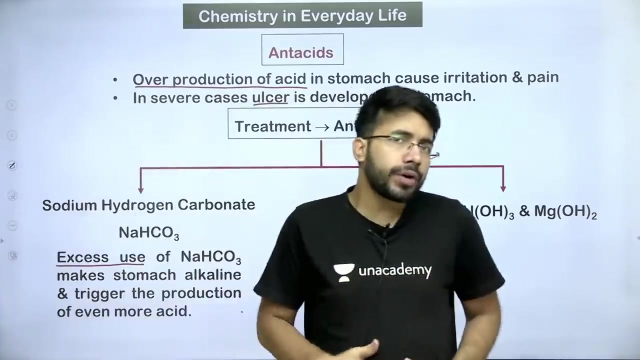 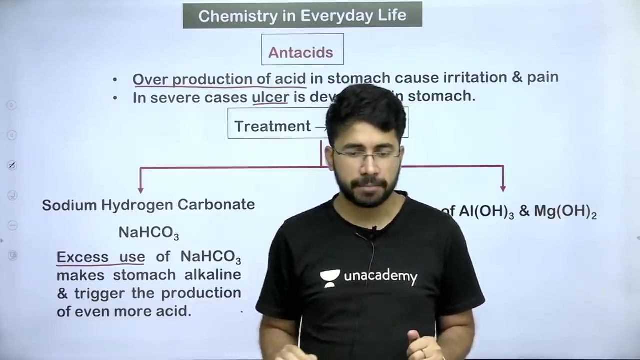 come, my friends. let's come here that anti-acid is of two types in the market. in the old days we used to use this sodium bicarbonate. this is also of basic nature- and nowadays we are using this mixture of aluminum hydroxide and magnesium hydroxide. these are both anti-acids. both will reduce the production of their acid, that is, it will reduce a little. now, what is this sodium bicarbonate? if I use its excess, then listen, my stomach was already acid. there was a lot of production. to reduce that production, to control it, I took anti-acid sodium bicarbonate. now I took anti-acid. okay, 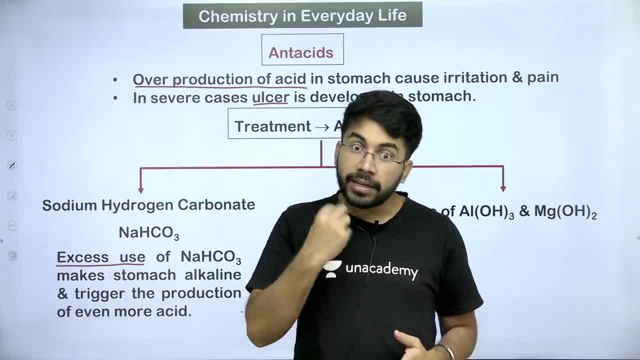 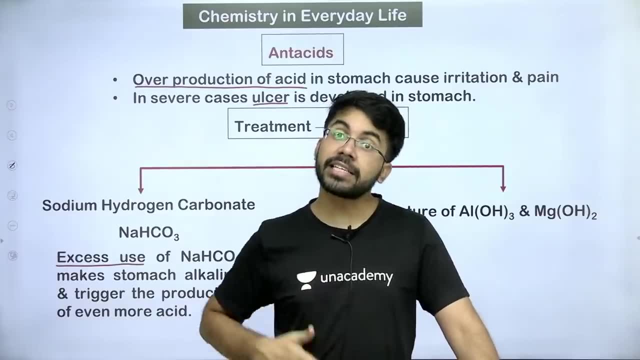 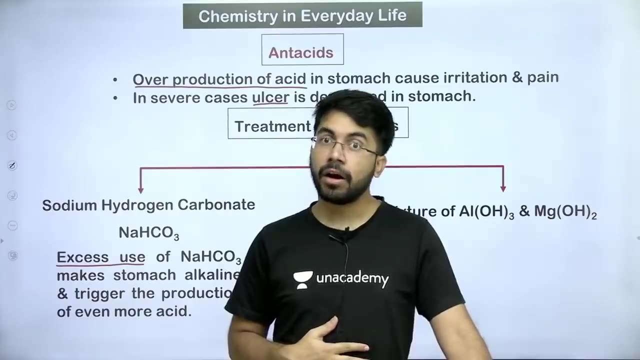 that is, it got neutralized by preparing acid plus base. but now we are taking anti-acid. so here the basic nature is increasing. the amount of acid has become neutral. but if anti- acid is taken by 1-2 tablets more then the basicity increased. because anti-acid has a basic nature now the increased acidity plus basicity is also dangerous. in this situation the basicity is increased by reducing the acidity. it is a good thing. 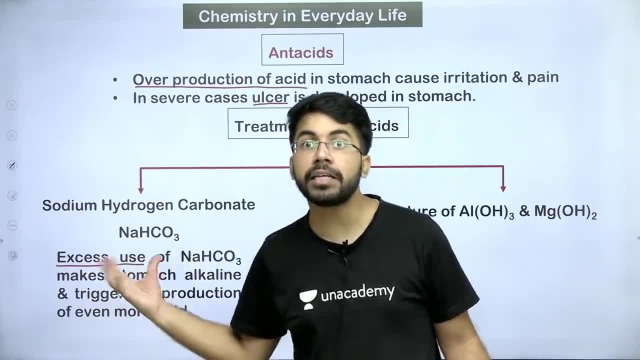 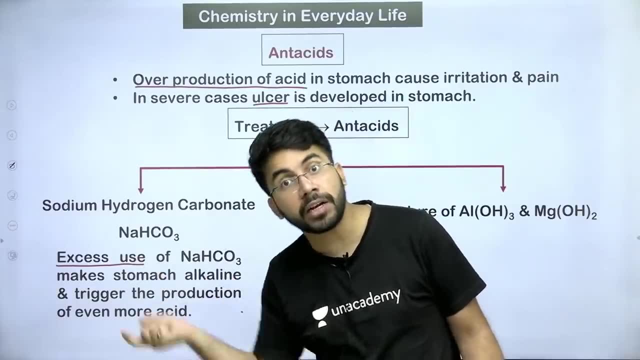 what? But it increased the basicity upside down. If you take more than one or two tablets and increase the basicity, then what will you do To finish it off again? overproduction of acidity will happen again, Do you understand? 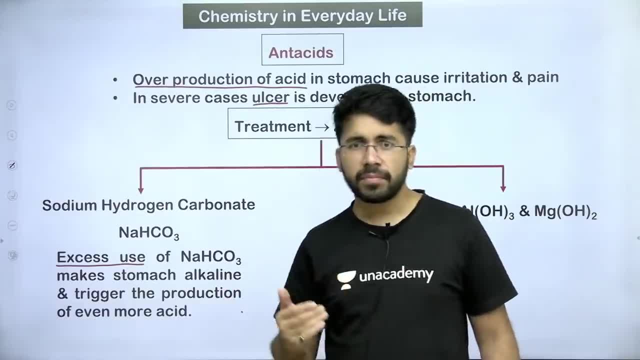 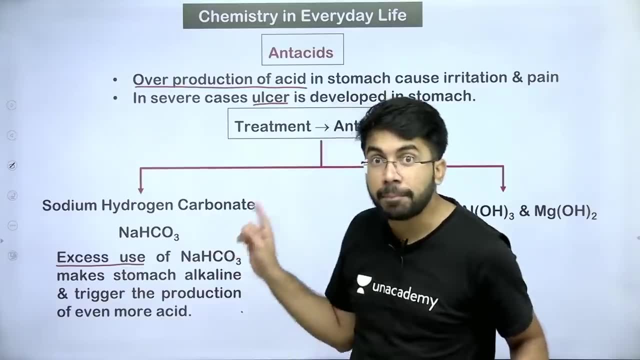 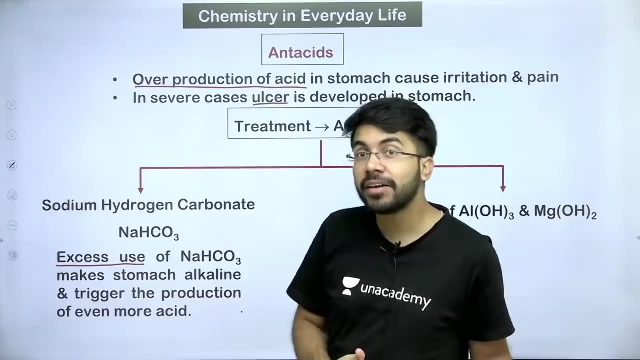 So you must have seen some acidity. that is not that good. After a few days acidity starts coming back again. Why? Because you have neutralized the acid first, But it is basic, So it is increasing the basic nature in your stomach. 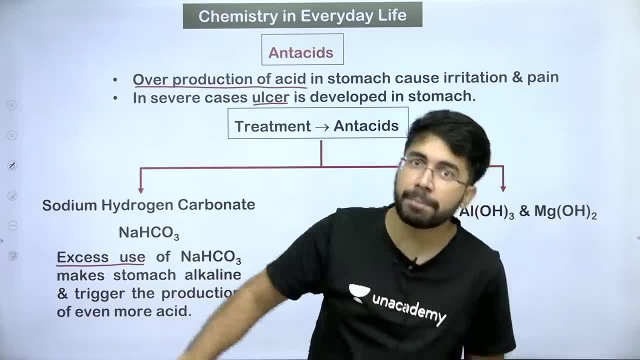 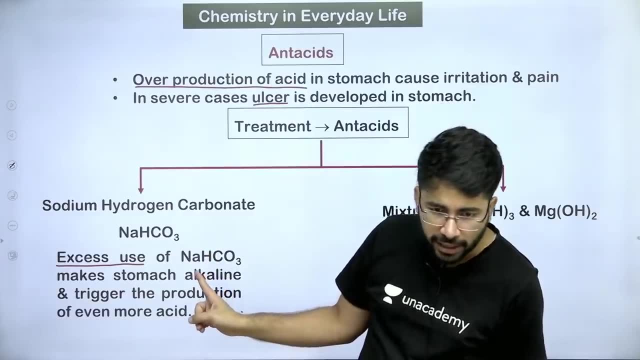 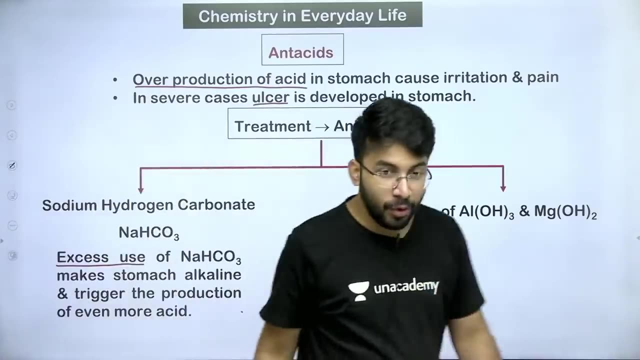 And when it increases the basic nature to control it, overproduction of acidity will happen again. So excess use of sodium bicarbonate makes the stomach alkaline. Now, if the stomach is alkaline, then again, Sorry, Sorry, Again, overproduction of acidity will happen. 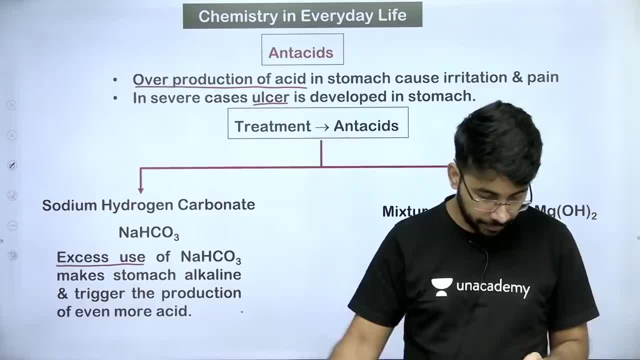 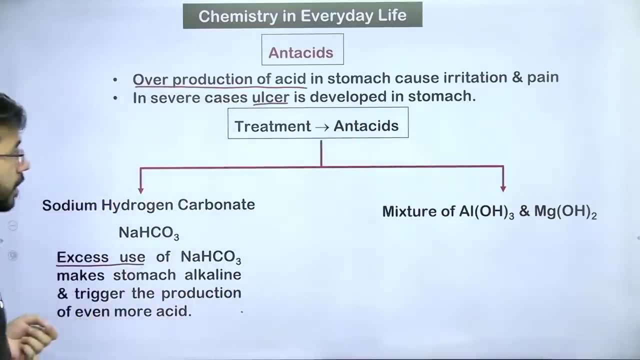 It triggers the production of even more acid. Okay, Let's go. Yes, It triggers the production of even more acid. Now comes the mixture of aluminum hydroxide and magnesium hydroxide. What is this Actually? what is this? 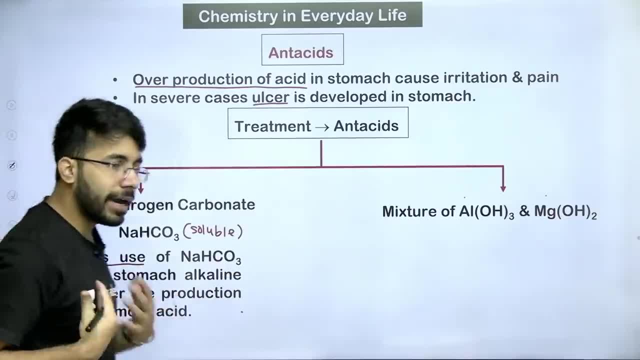 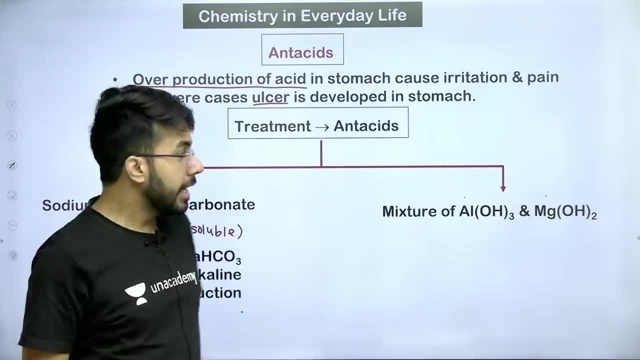 Bicarbonates are soluble. So if this is being soluble in your stomach, then my friend will increase the pH. It will increase the basicity nature. But what is this Mixture of aluminum hydroxide and magnesium hydroxide? 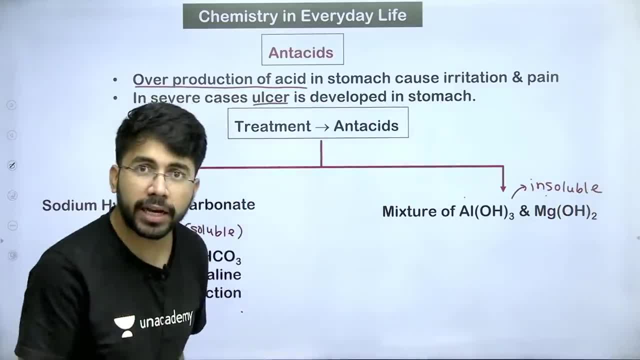 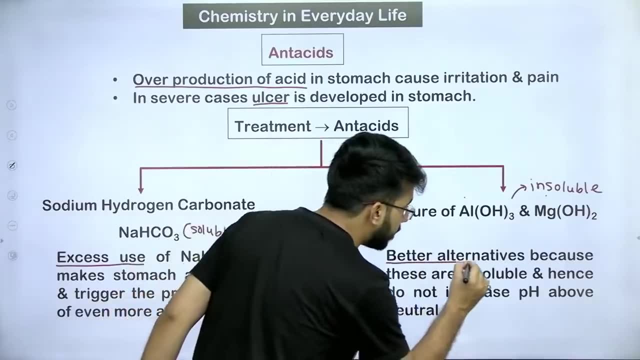 These are insoluble in nature And when it will not be found, it will not dissolve. then it will only stop the acid, It will not be soluble. This is a better alternative, friend. This is a better alternative Why? Because this is insoluble. 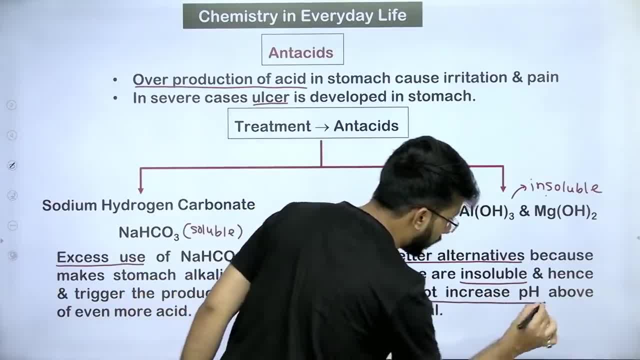 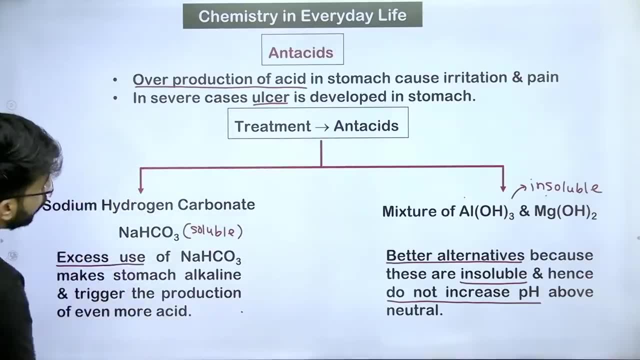 And that is why it does not increase the pH. Do not increase pH, So there is no overproduction again. So what will it do After a while? it will overproduce again Because it is soluble, it increases the basic nature. 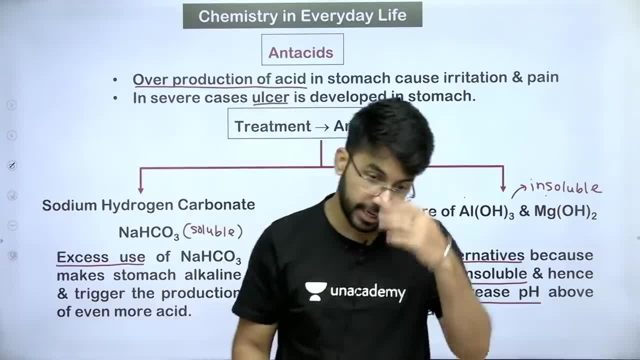 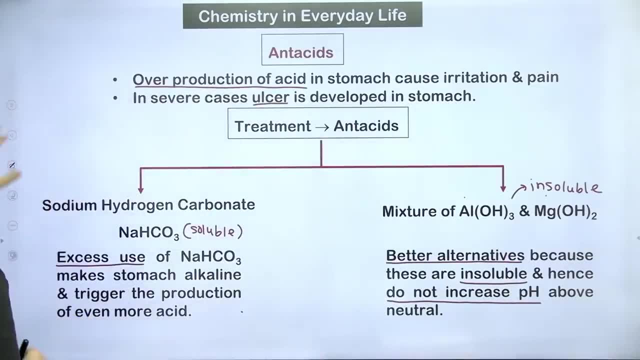 And it is not soluble. It does not increase the basic nature, And this is what anti-acid does. This is what anti-acid does. Okay, Let's go ahead. Next, Anti-acid is in front of you. What happened in anti-acid? 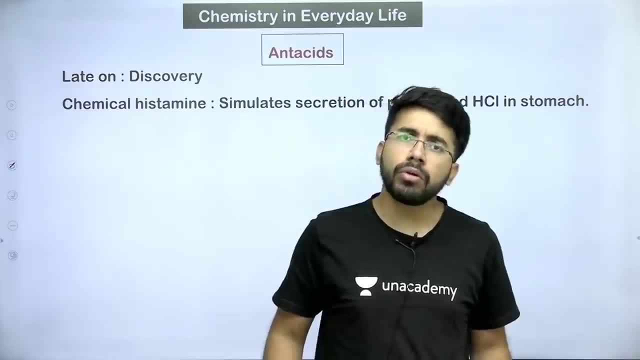 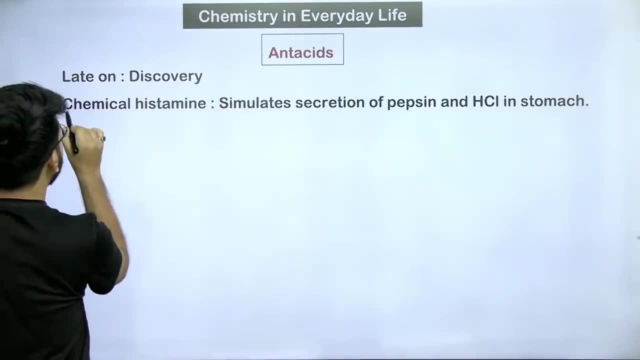 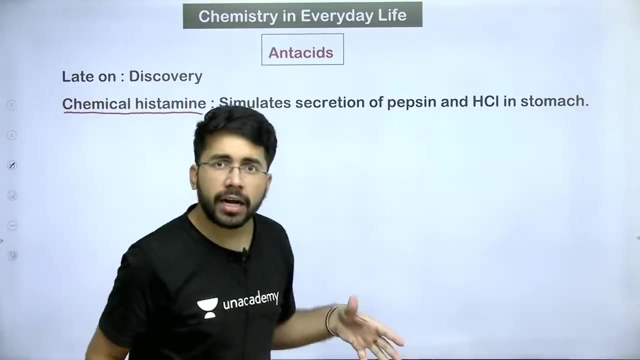 Later on. this discovery happened Later on, when many scientists went ahead with discoveries. then a friend came to know that there is chemical histamine in our body. What happens? There is histamine in our body which simulates the secretion of pepsin and HCL. 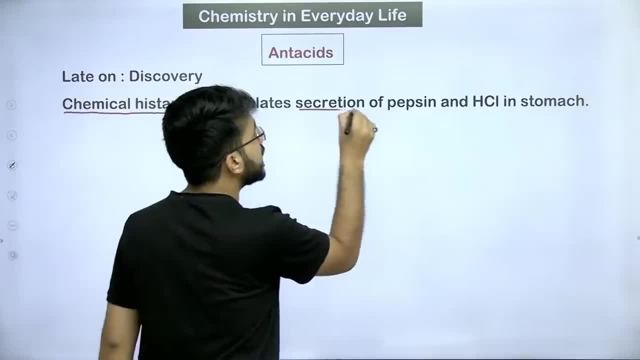 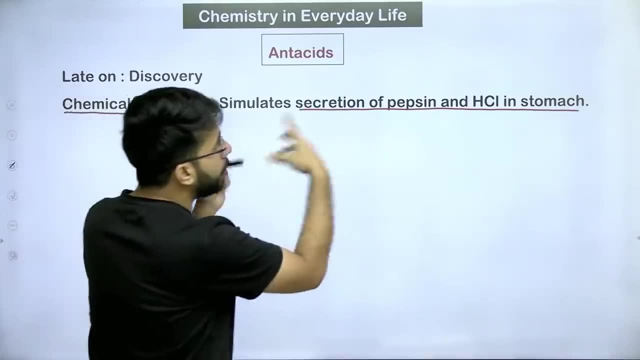 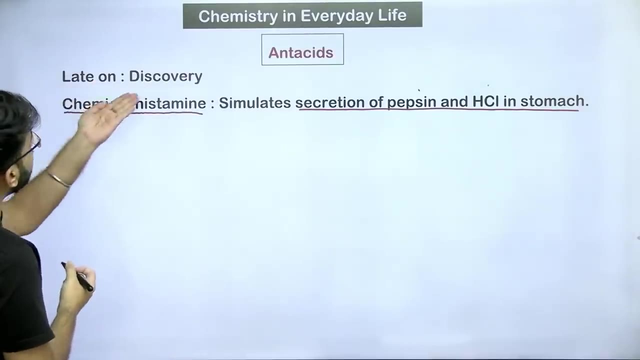 The histamine that is responsible for the secretion of pepsin and HCL in your stomach. Your histamine secretes HCL and pepsin in your stomach. So later on, the discovery was that we give an anti-histamine. 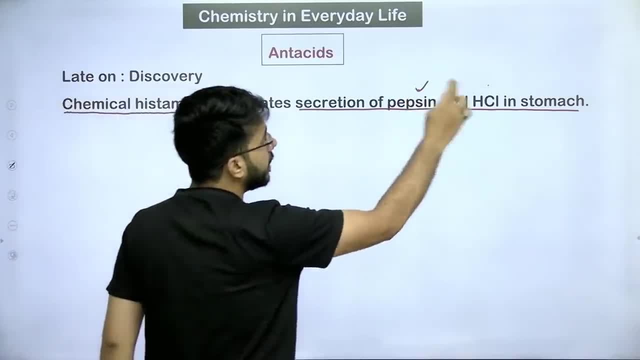 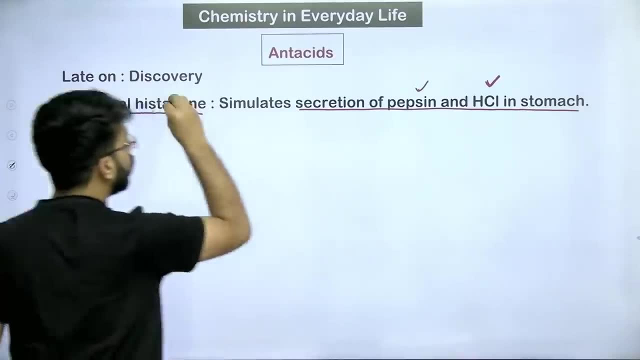 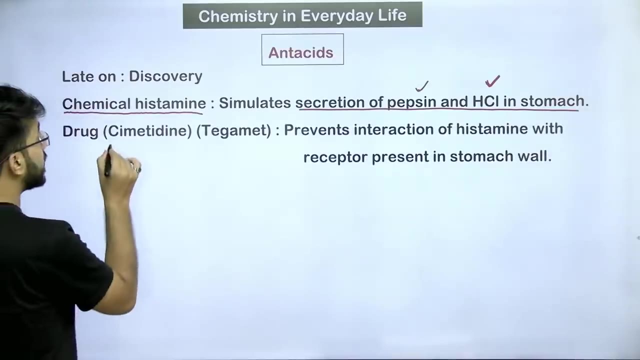 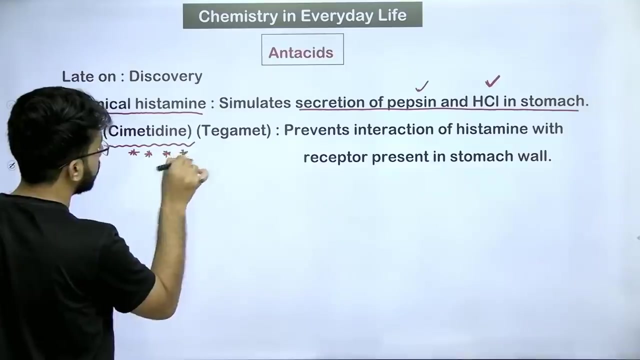 What does histamine do? HCL released in your body happens because of this. So if it is over-producing, then stop it. slow down its work, Inhibit its action. Later on, a drug named Cimitidine was found in VVIP-PYQ and its second name is Tegamate, which is sold in the market in the name of Tegamate. 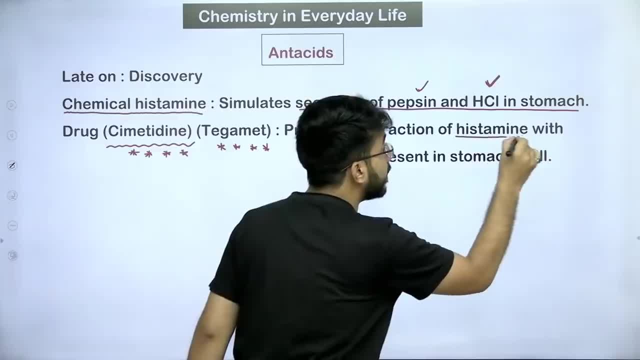 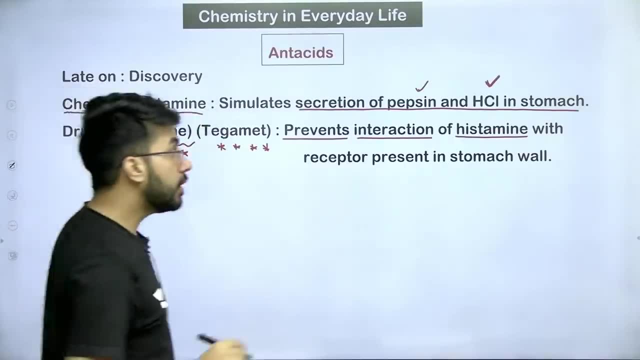 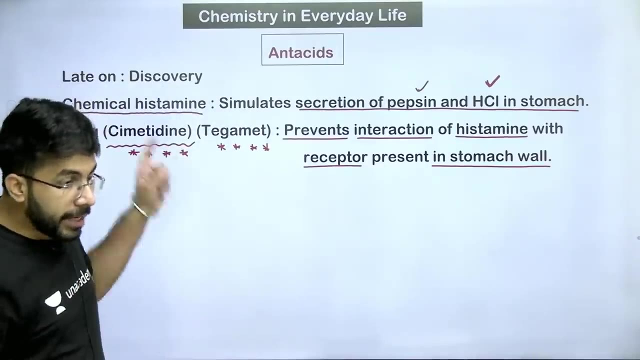 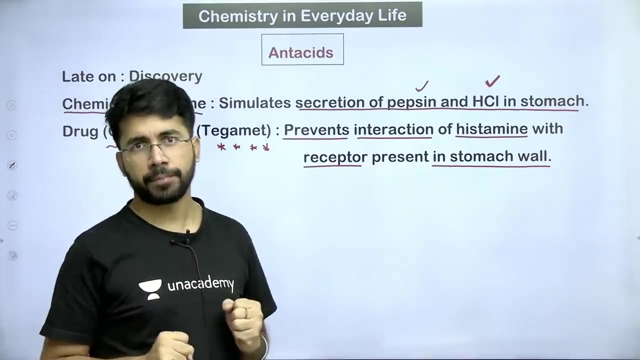 What does it do? It inhibits the interaction of histamine With the receptors in the stomach wall. This is a chemical histamine that sees the production of HCL in your body. Because of this, HCL production is triggered. Now, what will we do? We will reduce the work of the one due to which HCL is increasing. 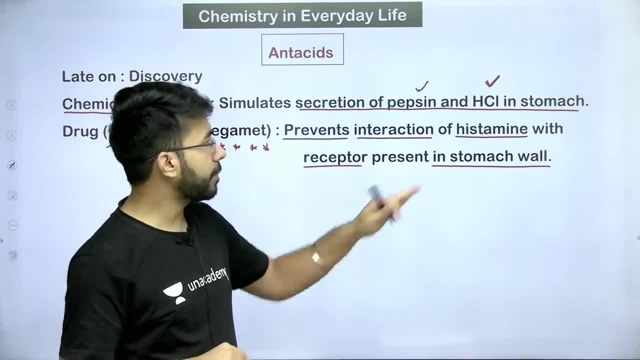 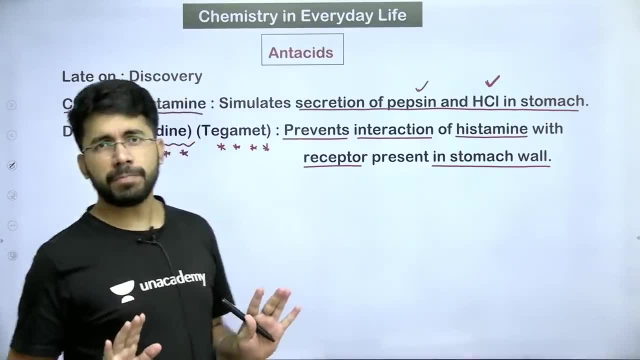 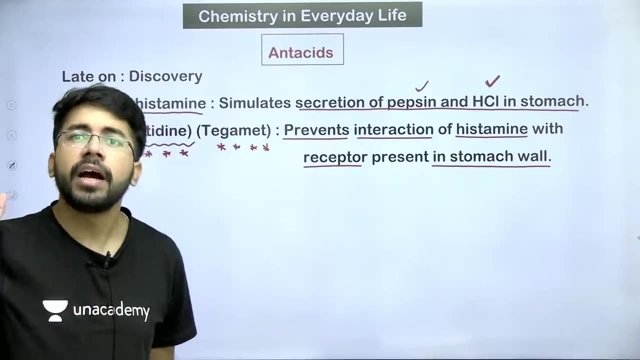 Inhibit the action of histamine. And what happens to the receptors in the stomach wall? The one who is getting the message that release HCL, Stop that message Prevents interaction of histamine with receptors. If the receptor is not given the message that you have to release HCL, then your work will be over. 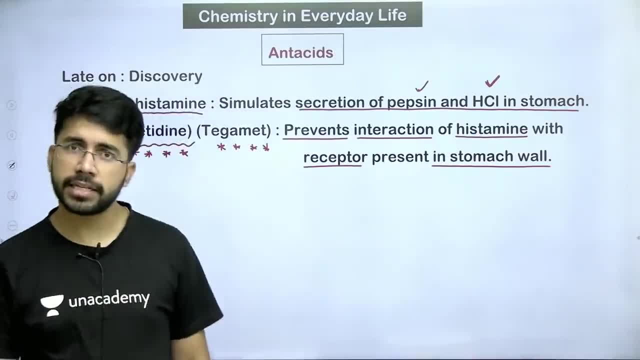 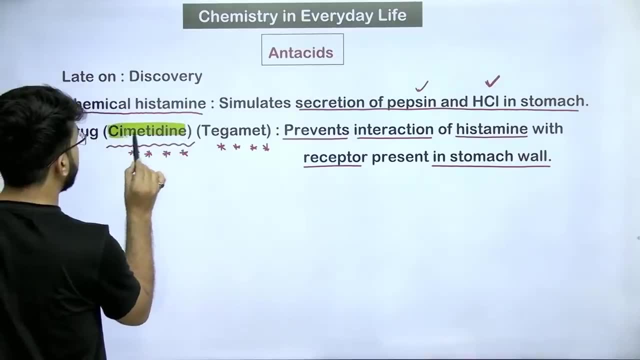 So, friends, it stops the interaction of histamine. With whom? With the receptors. So, in front of you, these two very important names have come. What is Cimitidine? It is anti-acid. Tegamate is anti-histamine. 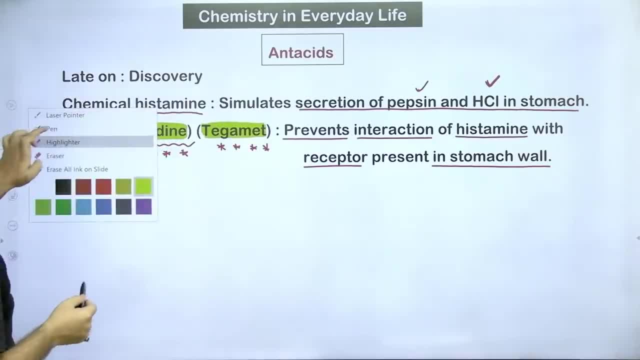 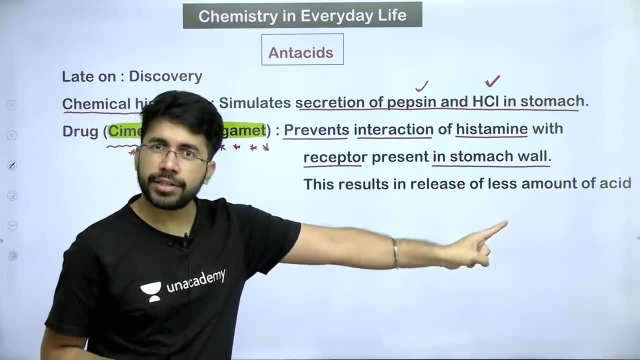 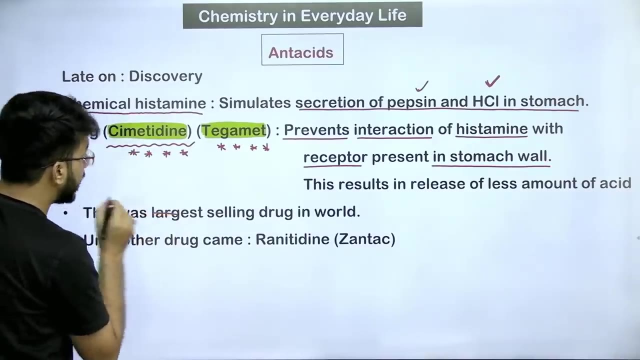 This is what anti-histamine is, And what does it do? It works as an anti-acid. It controls the acid. This results in the release of lesser amount of acid, So the production of acid will decrease. Next is this Cimitidine, and Tegamate is the largest selling drug. 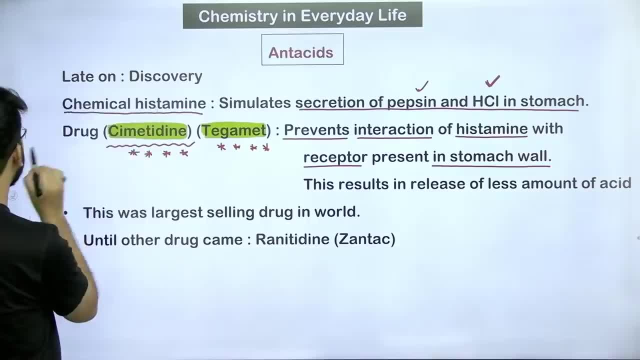 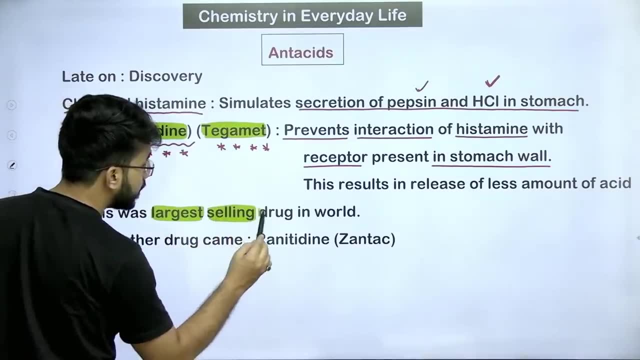 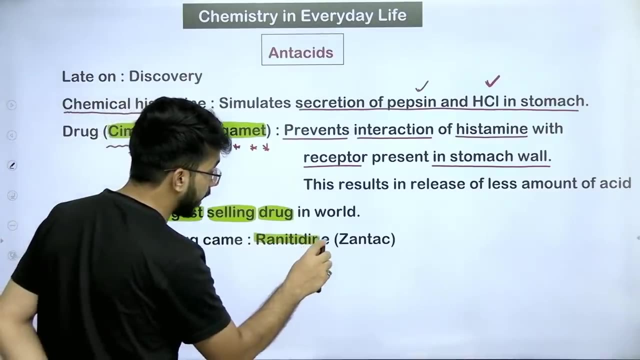 This- Cimitidine and Tegamate- is the largest selling drug. Cimitidine and Tegamate is the largest selling drug. What is Cimitidine and Tegamate? It is the largest selling drug Until Renitidine is not used. 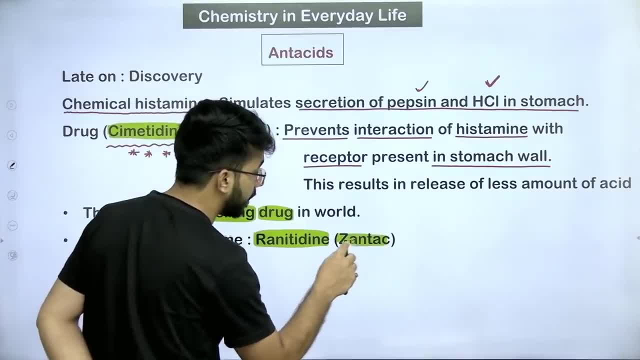 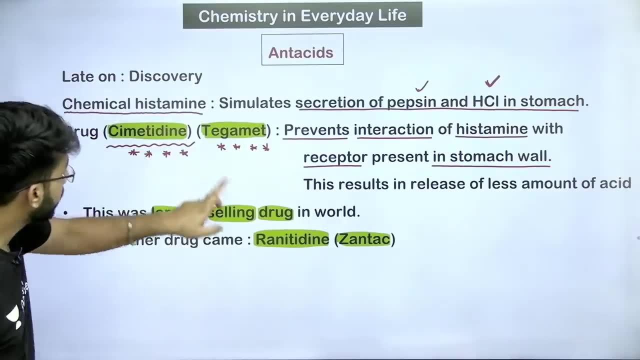 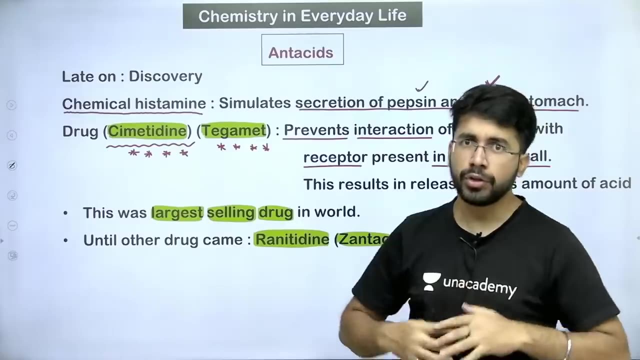 Until Renitidine is not used. Until Zantac is not used. Until Renitidine is not used. Until Zantac is not used, It means both are anti-histamine- Cimitidine and Tegamate, and Renitidine and Zantac are anti-histamine. 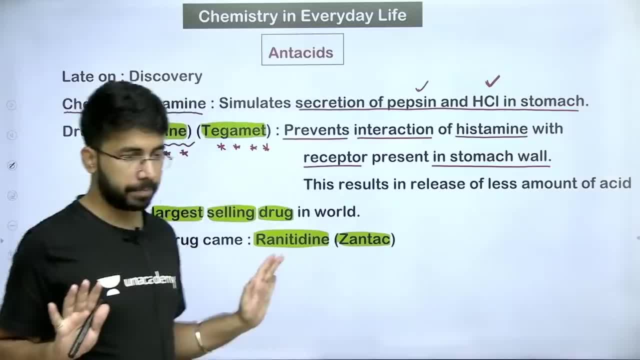 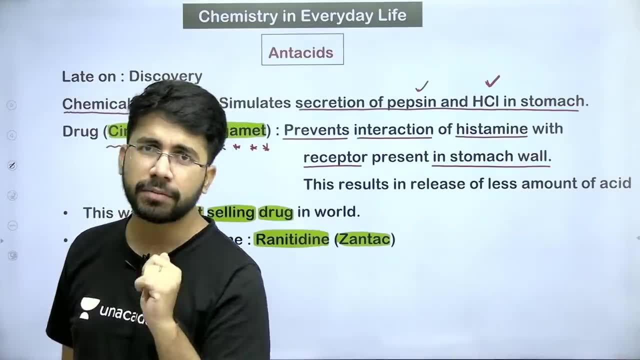 Which controls the overproduction of acid. It is a simple story Before this. what did we use? We used ALOH whole thrice and MgOH whole twice mixture. Still, it was a good solution as compared to sodium bicarbonate. 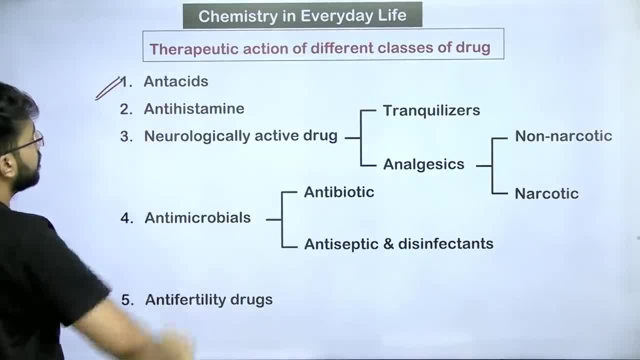 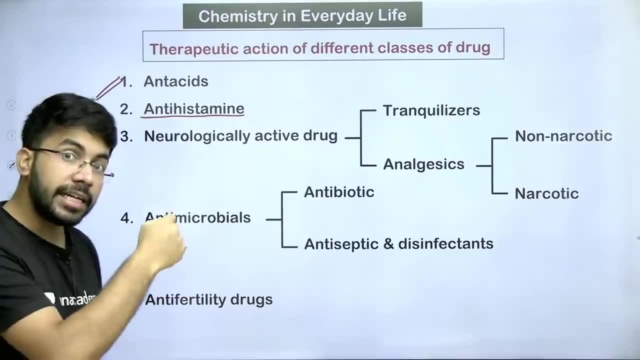 Next, my friends, anti-acid is over. Now let's come to anti-histamine. We study anti-histamine separately. We have already studied one type of anti-histamine. Now let's study the second type of anti-histamine. 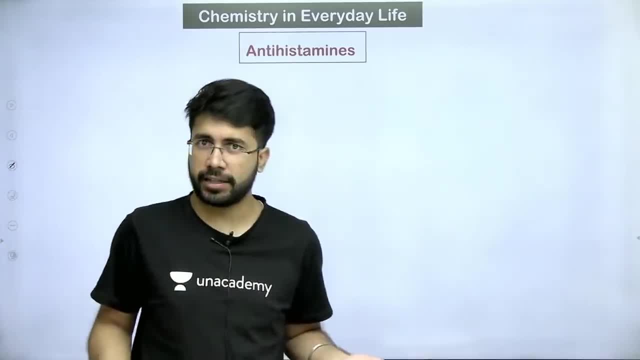 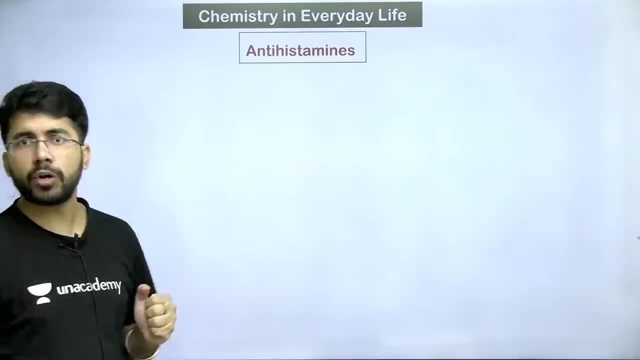 Actually, first of all, let's look at histamine. What else does histamine do? Histamine in our body? First of all, it stimulates the secretion of HCL and pepsin, And the second thing it does is that it is a potent vasodilator. 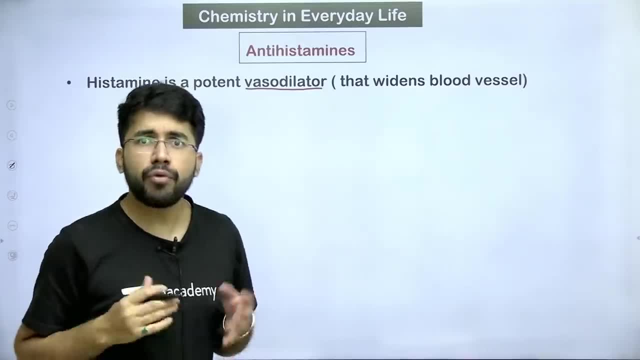 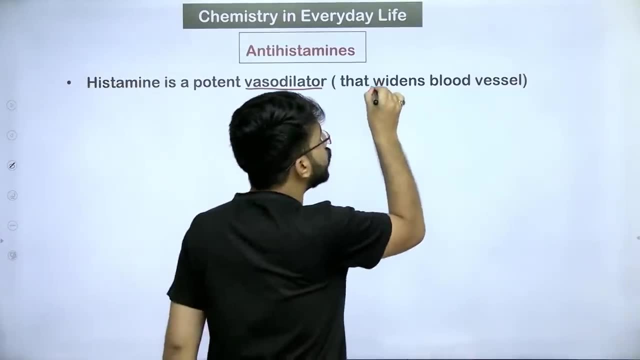 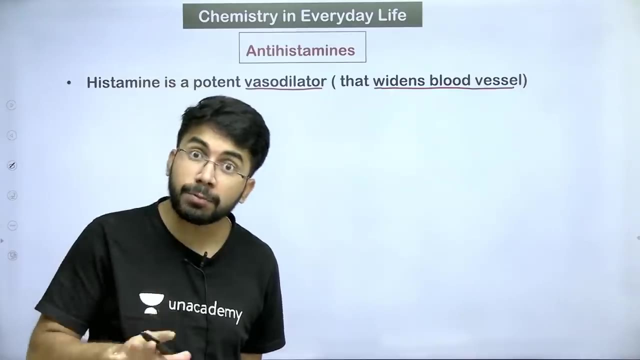 First of all, what is a vasodilator? Histamine is that chemical in your body which widens your blood vessel. Which widens your blood vessel. What does it do? It helps in maintaining the blood pressure also. It helps in maintaining the blood pressure also. 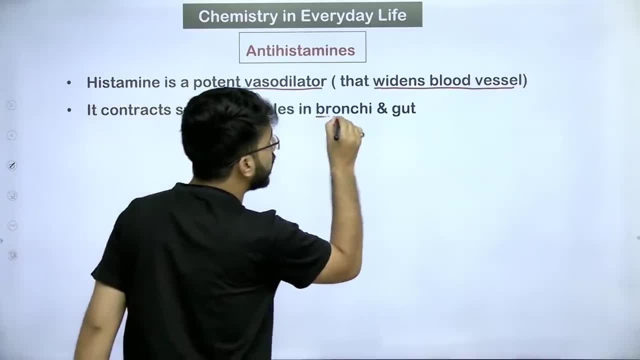 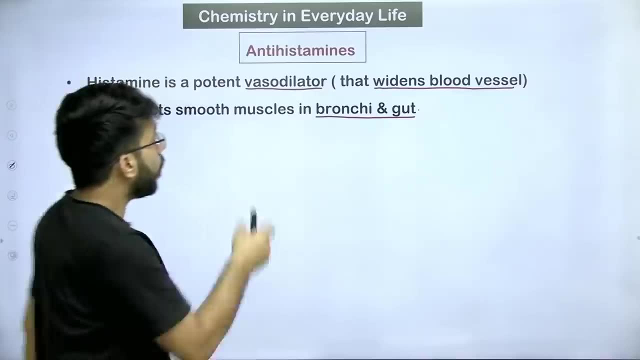 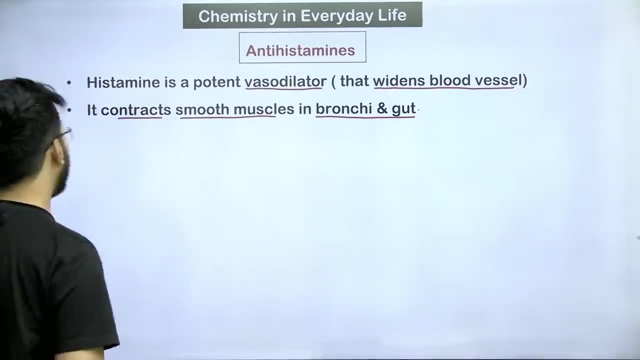 My friends. the second thing, This is your bronchi and gut. Bronchi and gut means the soft muscles in your lungs, The small muscles It contracts, the smooth muscles in the bronchi and gut. What is the third function of this? 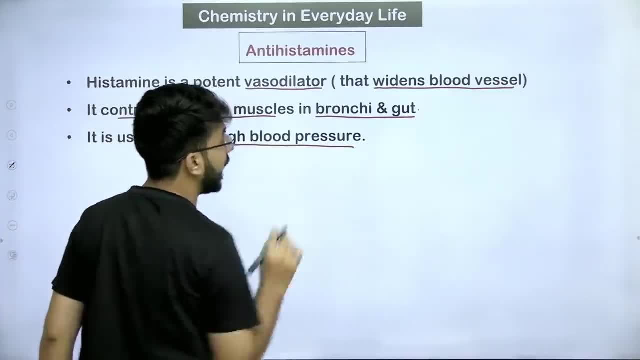 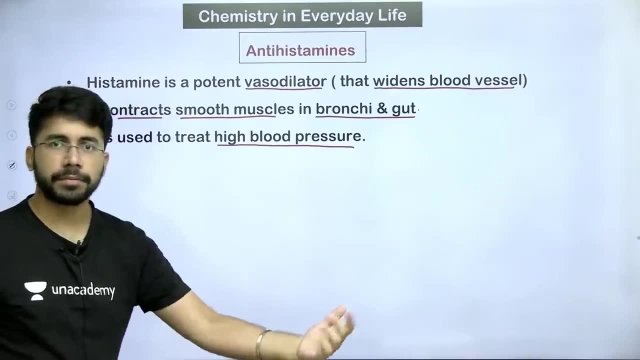 It is used to treat high blood pressure. It treats high blood pressure How? By opening the blood vessel, By widening the blood vessels So that the blood flow is easy, So that the blood pressure does not increase. Next, Let's come further. 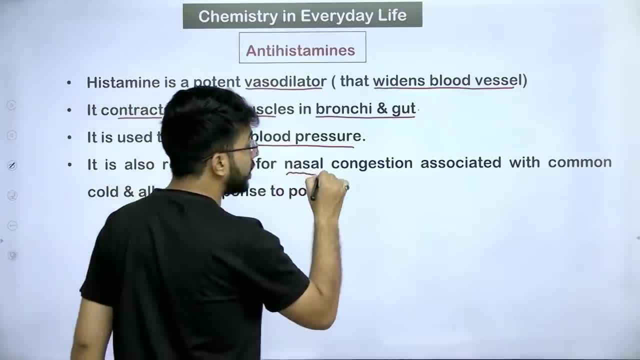 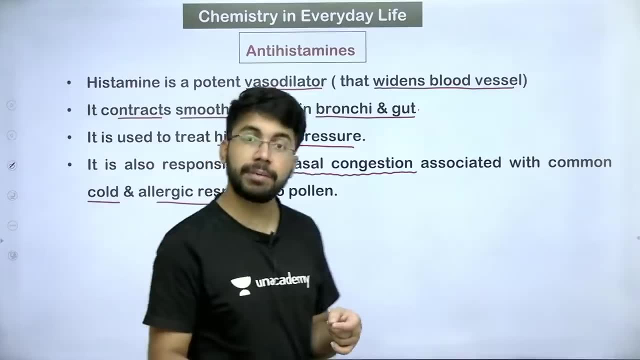 It is also responsible for nasal congestion When your nose is jammed, When, When you have common cold and allergic response For that also histamine comes. These all are histamines. These all are what we are talking about. We are talking about histamines. 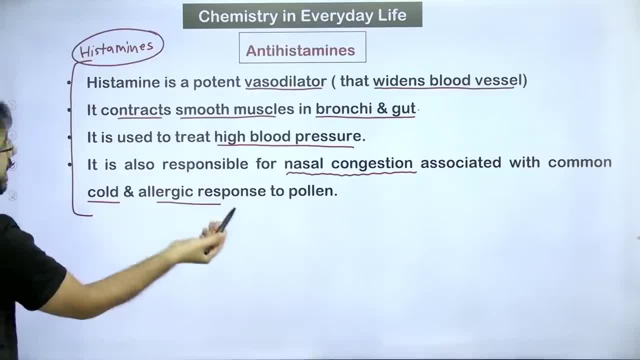 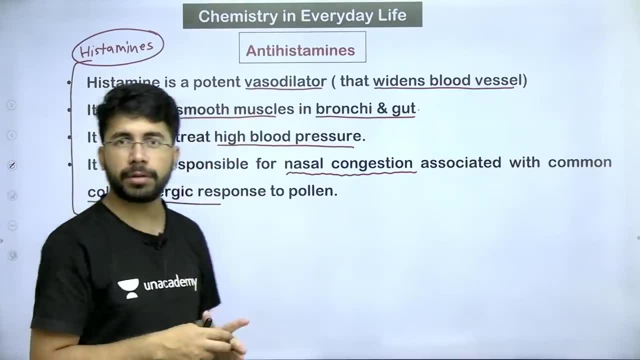 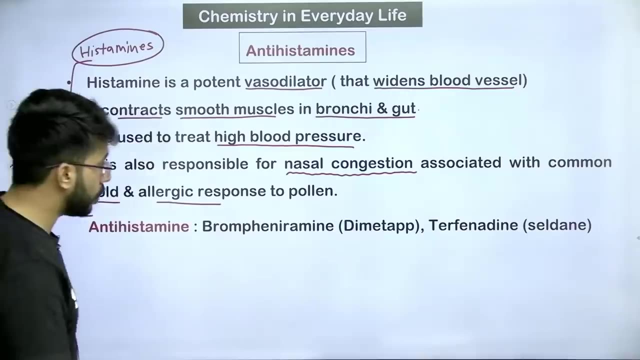 Who is working? Histamines are working: Nasal congestion, High blood pressure, To contract the smooth muscles in the bronchi and gut. It works as a vasodilator. Okay, Then we come to anti-histamine. What are our anti-histamines? 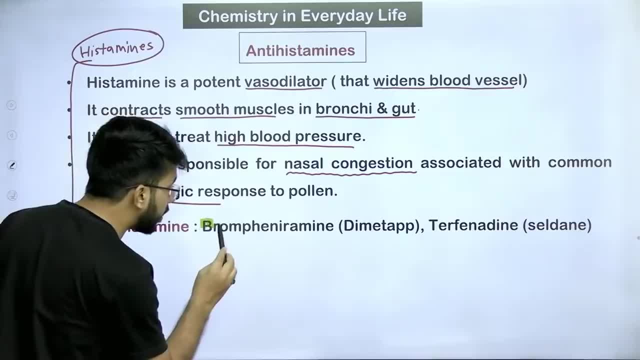 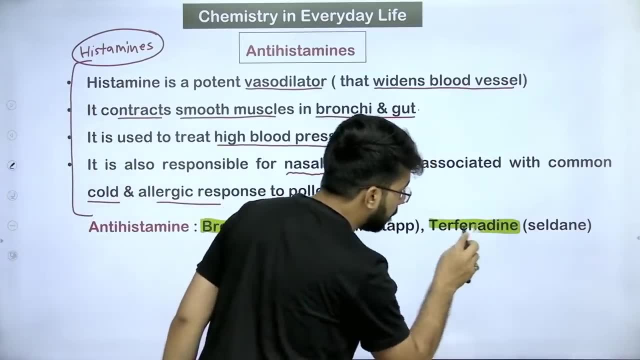 So again, anti-histamine has been asked. The name of the drug has been directly mentioned in front of you. What are the anti-histamines? Bromfenaridine And then terfenadine. Bromfenaridine and terfenadine. 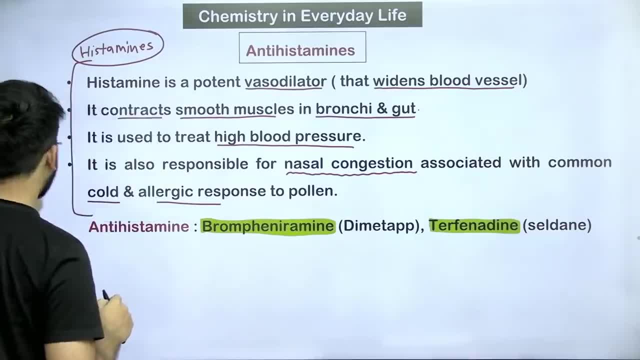 And it is also called Dimetap and Seldane. It is also known by another name: Dimetap and Seldane. It is also known by the name Seldane. So these two will work as anti-histamines. They will give the opposite response. Okay, Now it comes that we have read two types of anti-histamines: One will work as an anti-acid, One will correct high blood pressure, nasal congestion, etc. Now it comes When you have both anti-histamines. 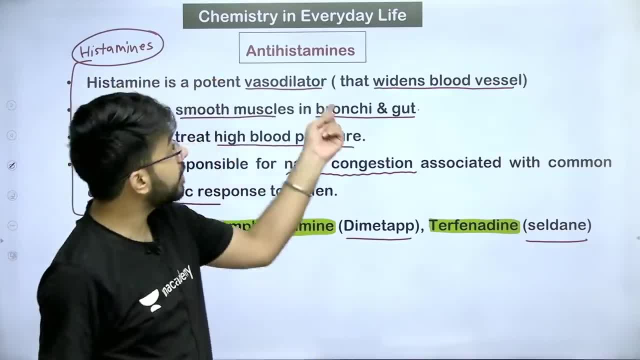 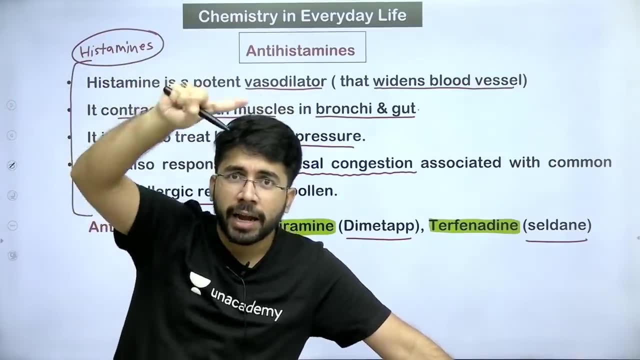 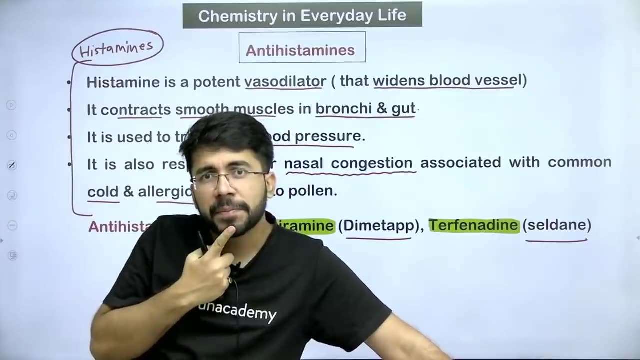 So do I have to use that anti-histamine? I can use anti-histamine with anti-acid here In blood pressure. Can your acidity medicine work in blood pressure, Or can your blood pressure medicine work in acidity? But both of them are anti-histamines. 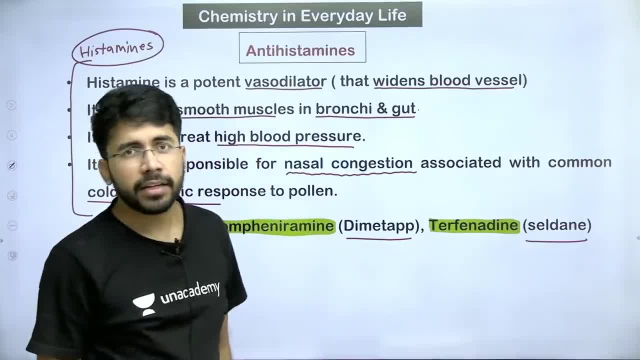 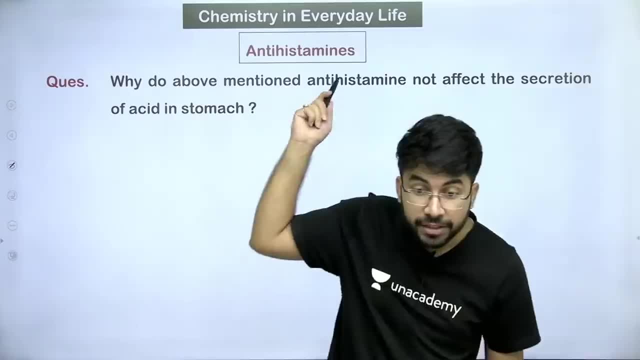 We have read anti-histamine there as well, And we have read anti-histamine here as well. This question came from IMS. I gave it in question form. Why do above mentioned anti-histamines not affect anti-acid? Why don't we use the current anti-acid? 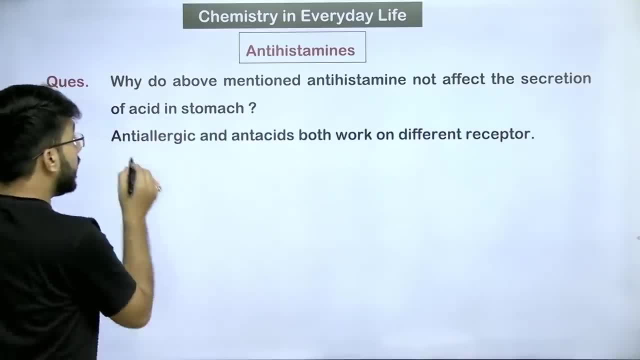 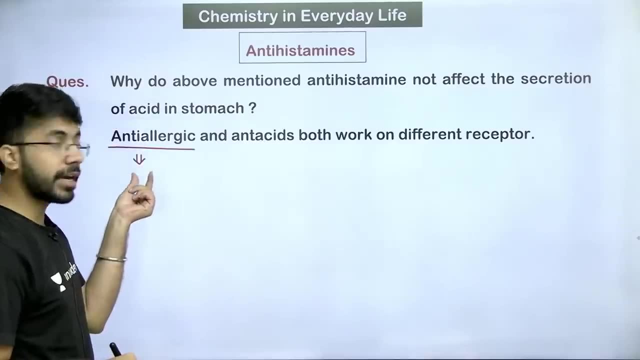 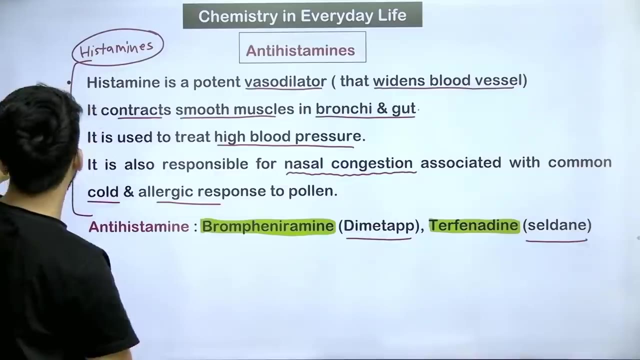 So I will explain it to you in simple language. This nasal congestion, high blood pressure, is anti-allergic. This bromfenaridine and terfenadine. What are they? Cimetidine and celdane. This dimetapine and celdane. 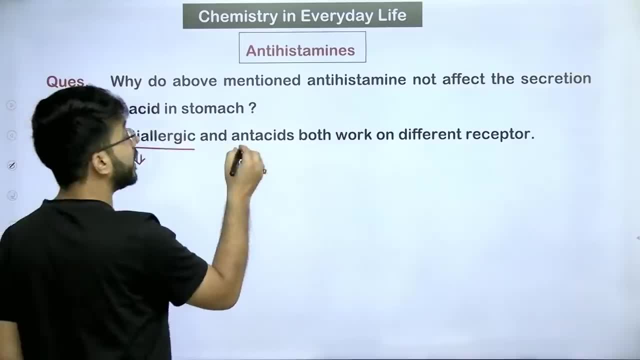 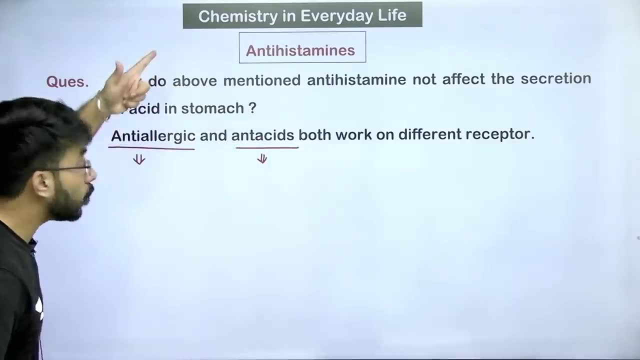 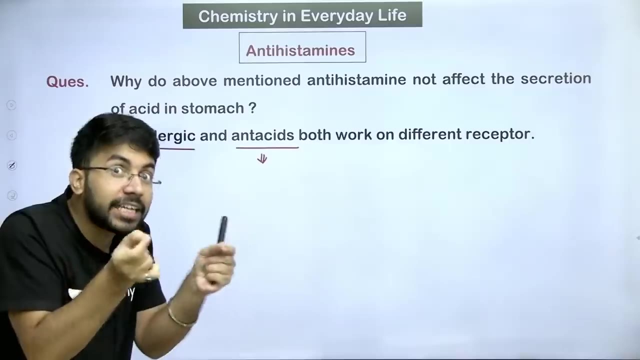 My friend, it is anti-allergic. And what we have read earlier- Tegamet, That is your anti-acid. This allergic receptor is different And this anti-acid receptor is different And the shape of the binding site of both receptors is different. 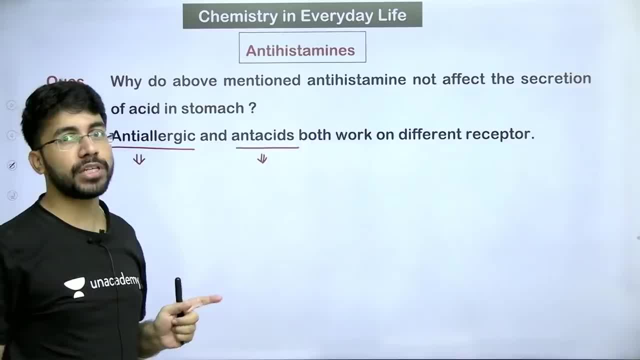 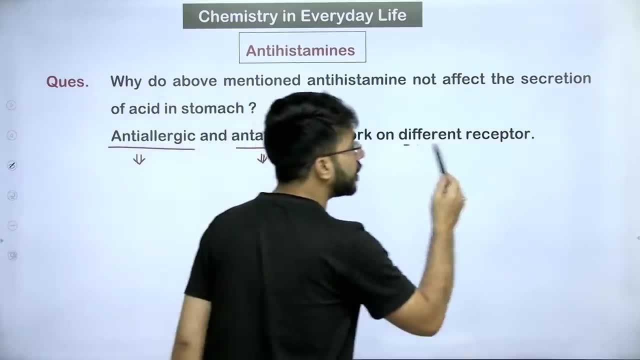 So if the shape of binding site is different, Then the shape of the drug should also be according to that. It is not that every drug will work in every disease. No, Its receptor is different. They work on different receptors. And what is the problem with different receptors? 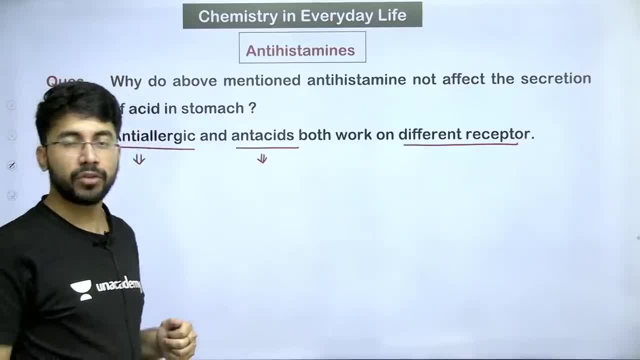 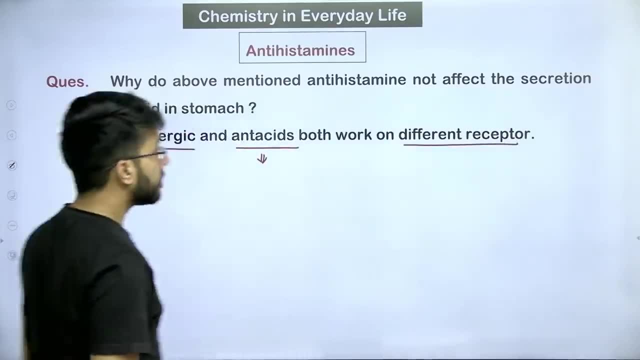 The shape of the active site of different receptors is different, So every drug's shape is also different. So every drug's shape is also different. Okay, Now it is clear, Okay. Okay, Now let's come In front of you: anti-acid and anti-histamine. 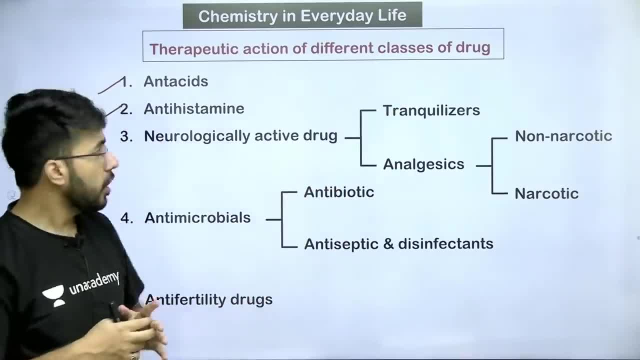 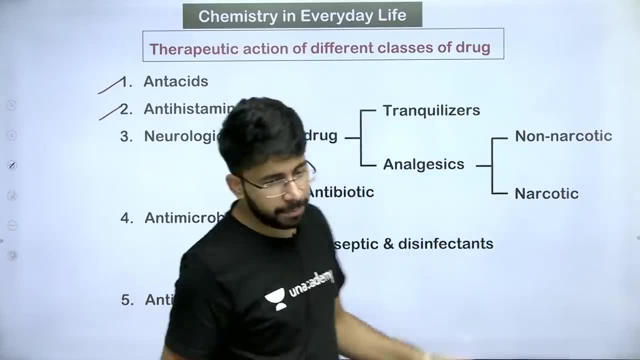 Now let's come to what is tranquilizers and what is analgesics, The neurologically active drug, Like you call anxiety, Which you call depression, For anxiety and depression, The medicines we use Which are of the sleepy nature, Non-narcotic, narcotic. 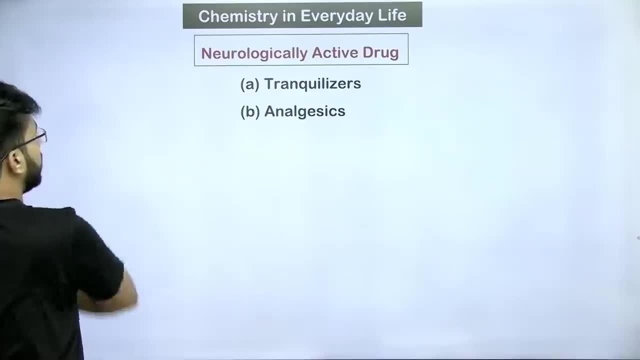 Now we are all going to see. Come first to tranquilizers. First of all, let's talk about tranquilizers. You have two neurologically active drugs: Tranquilizer and analgesics. First of all, we will read tranquilizers. 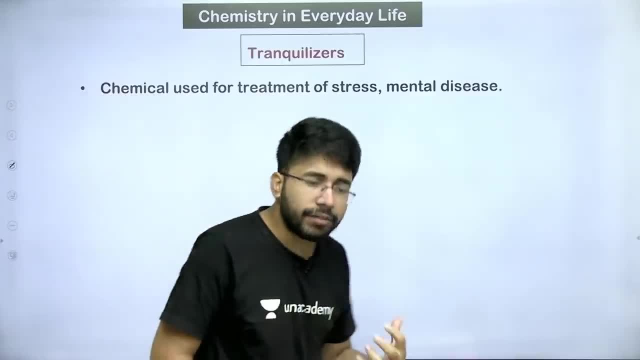 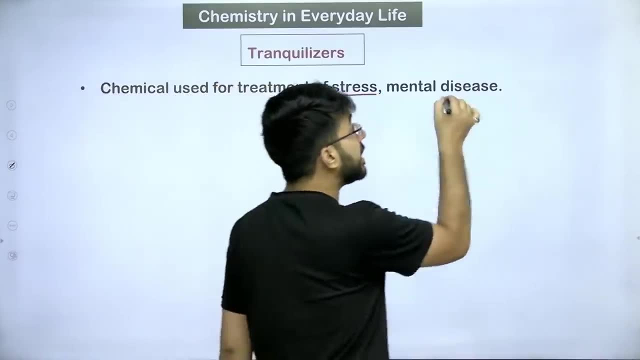 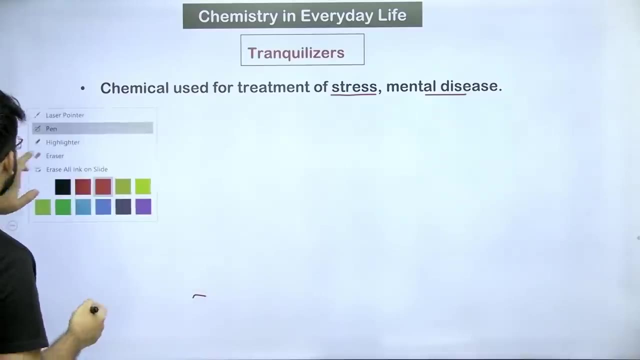 What is tranquilizers? That medicine, That chemical Which treats your stress, Which treats your mental disease. That is your tranquilizers Which reduces your stress, Removes mental disease. That is tranquilizers in front of you. Next, It relieves anxiety. 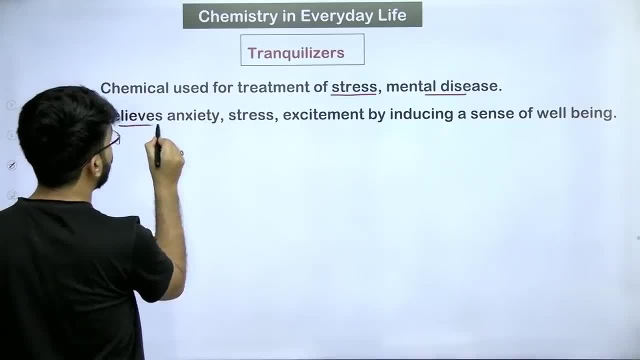 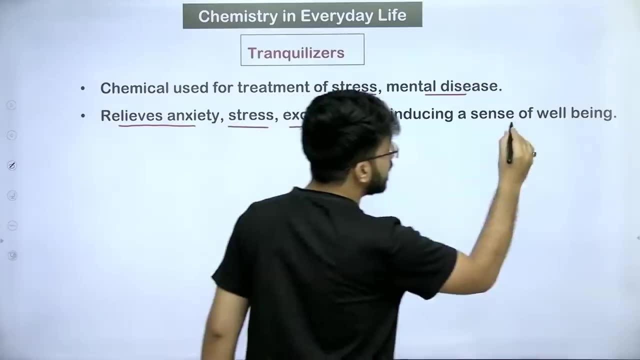 This relieves anxiety in front of you. It relieves stress. It relieves excitement by inducing cells of well-being. What happens? Reduce anxiety, Increase stress. It leads to over-excitement. Many people start to get scared due to overexcitement. 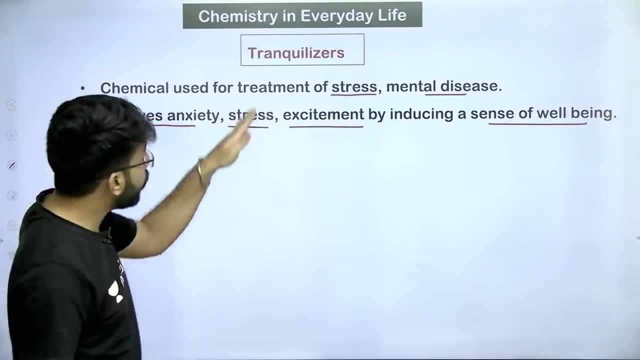 Their hands and feet start to shake. This must be in your exam days. So, my friends, In all these three you have tranquilizers. Next, It relieves anxiety. This relieves anxiety. It relieves stress. It relieves anxiety. 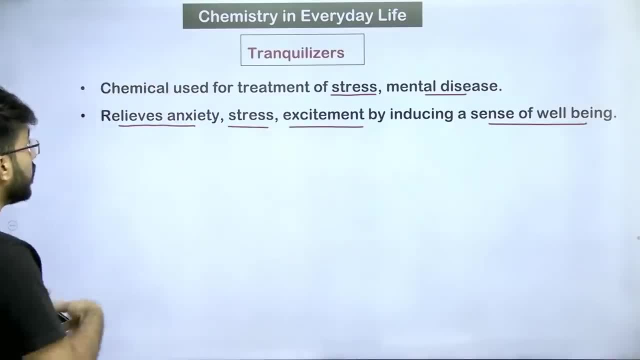 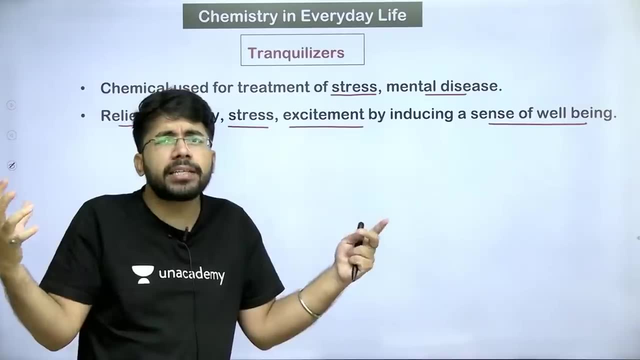 It relieves anxiety. This relieves stress. This relieves anxiety. This relieves stress. This relieves anxiety. Let's say we use a tranquilizer. The way you take the tranquilizer, it messages your receptor that all is well. 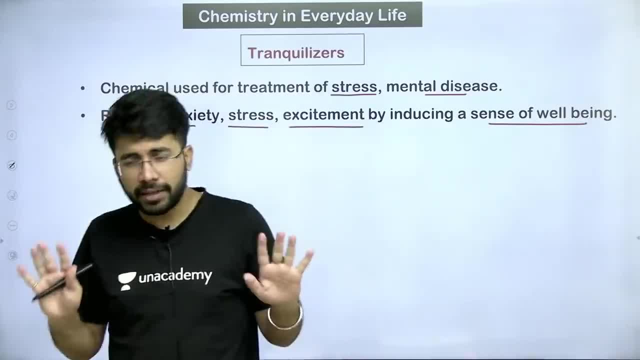 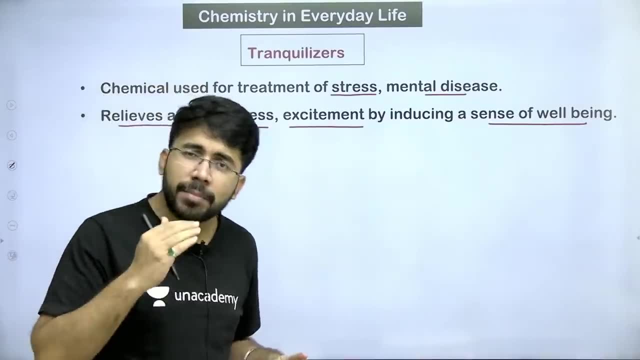 It gives a sense of well-being. So the receptor cools down- Actually, it slows down the communication system of the receptor, So you won't be able to communicate and you won't be able to feel these things. Let's move on. 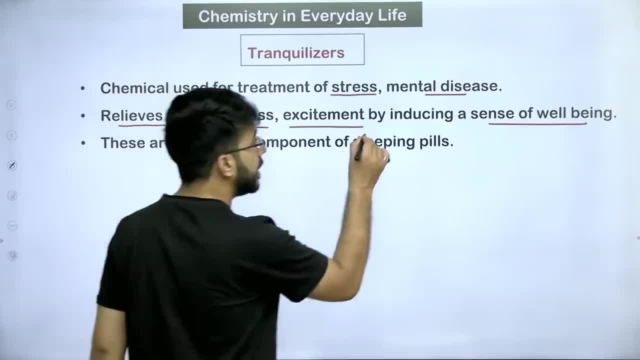 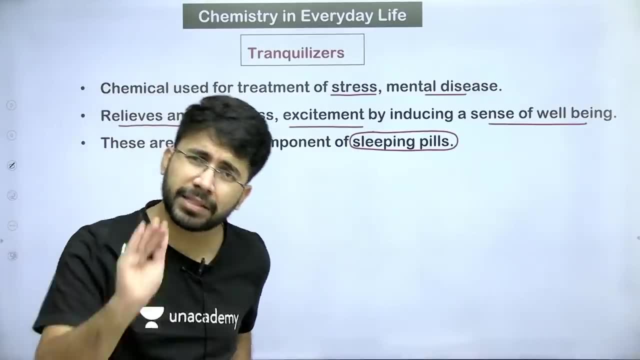 My friends, these are essential components of sleeping pills. What did I say about tranquilizers? It will make you sleep. It won't let your receptor message go. It will slow down the message of your receptor, So you will be in sleep. 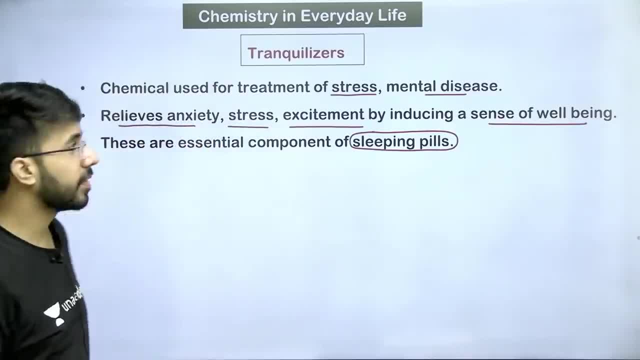 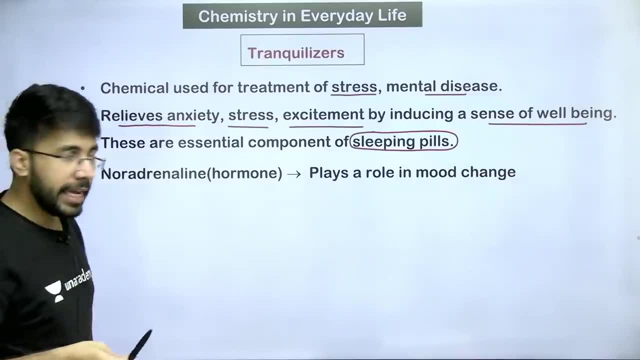 You won't be able to feel that something is happening. You will forget everything. Okay, let's move on This. my friends, in front of you is Norafatehi. There is a hormone in the body whose name is Noradrenaline. 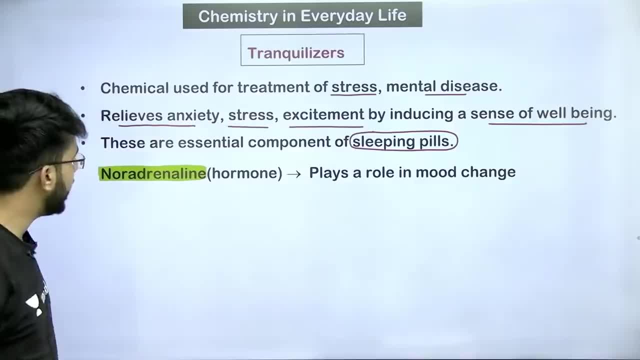 Something or the other is coming in front of you from adrenaline, Adrenaline, Noradrenaline. What is this Noradrenaline In your mood changes. Obviously, Norafatehi's songs make you change your mood. So, friends, it plays a role in mood change. 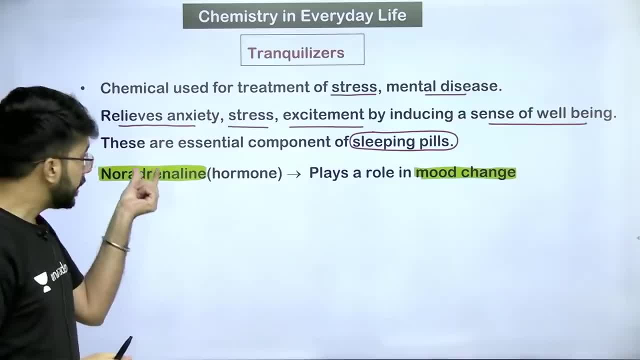 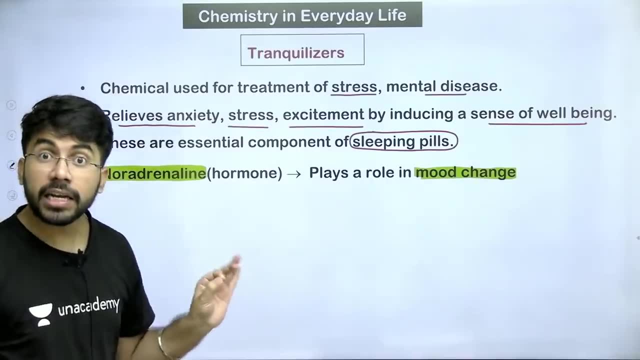 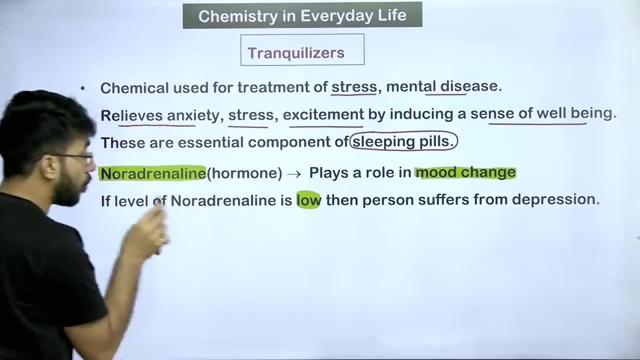 It releases hormones in your body due to which you feel anxiety, stress and excitement Because of the Noradrenaline hormone. If this hormone, if this hormone, if the level of Noradrenaline is low, if the level of this hormone is low. if it is not released properly, then you suffer from the disease of depression. Nothing else. You suffer from the disease of depression. Then the person suffers from depression. Noradrenaline is a hormone which plays a role in mood change. Let's move on. 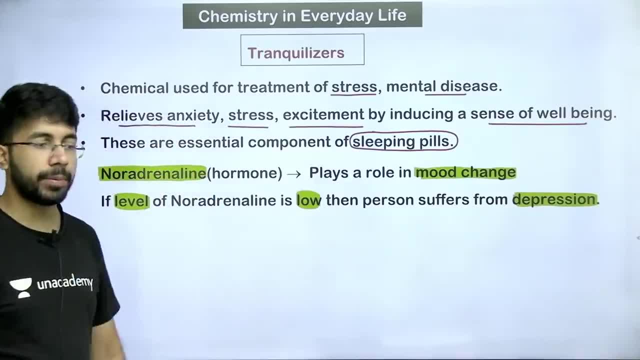 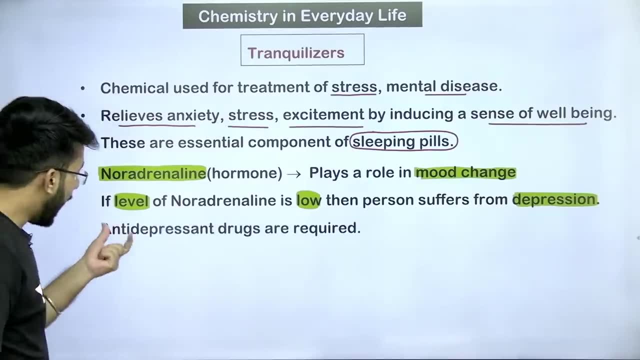 If the level of Noradrenaline is low, then the person suffers from depression. Then the person you have suffers from depression. Noradrenaline, Okay. Next, my friends, anti-depression drugs are required For this. we give anti-depression drugs. 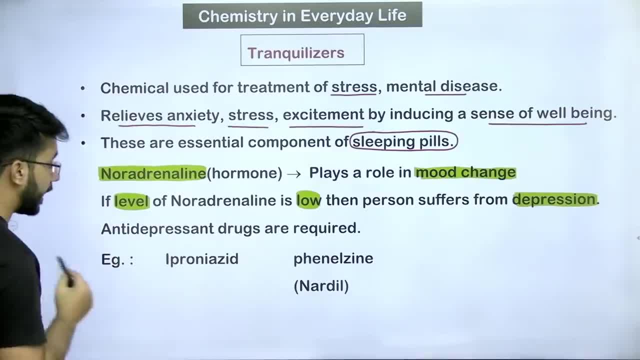 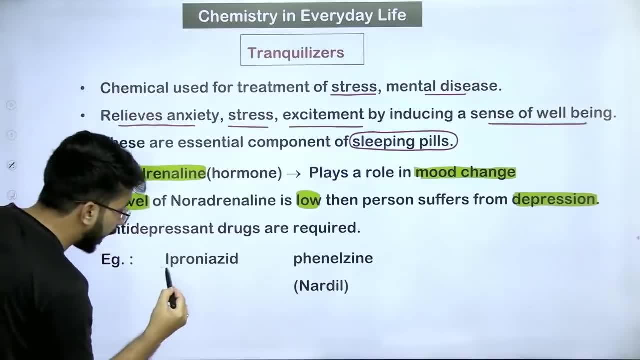 If you have depression, then we will give anti-depression. As an example, you will see ipronazide, Sorry. As an example, you will see ipronazide, which is yours. it is your anti-depressant. 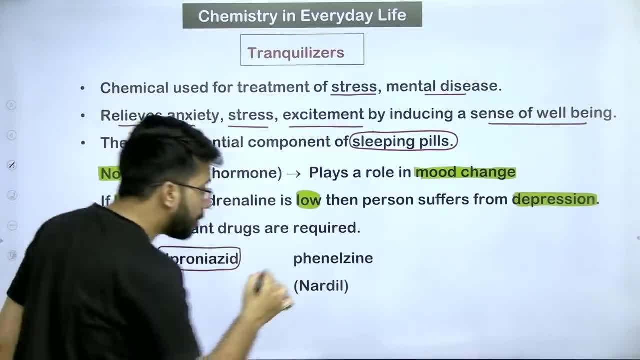 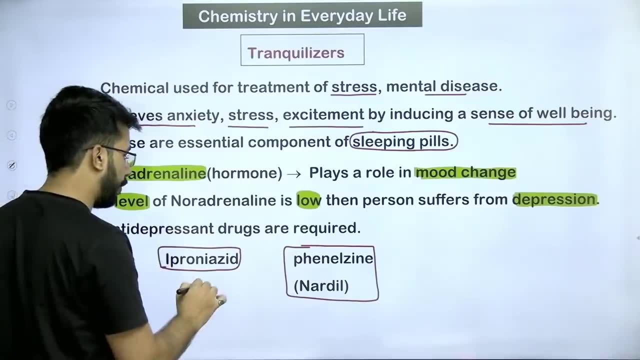 It will work in your depression. The phenylzine you get, which is called Nardil. this is your anti-depressant drug. Very, very important, Very, very important. Again, It has come in PYQ. It will come in you too. 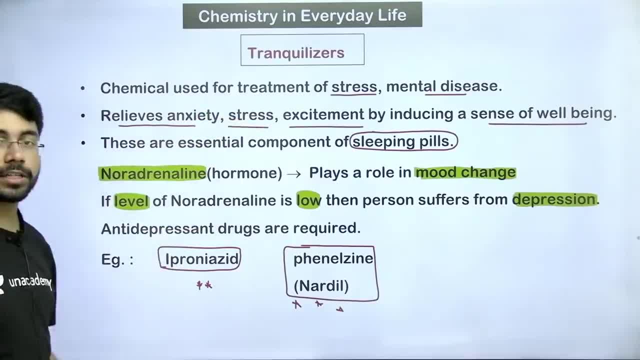 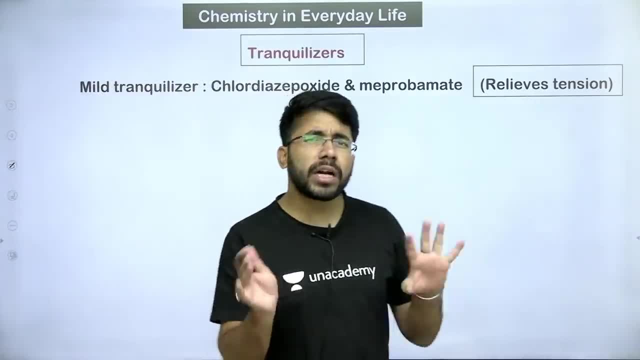 They ask the name of that drug, that what is anti-depressant? Okay, Next, my friends, come on Mild tranquilizers. Which is not a little tension? Something happened at home, Or a friend said something Or earned marks. 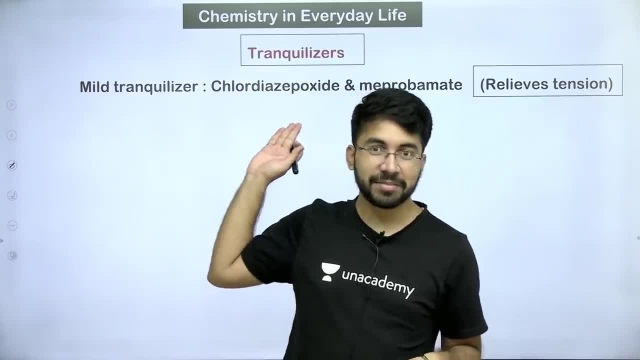 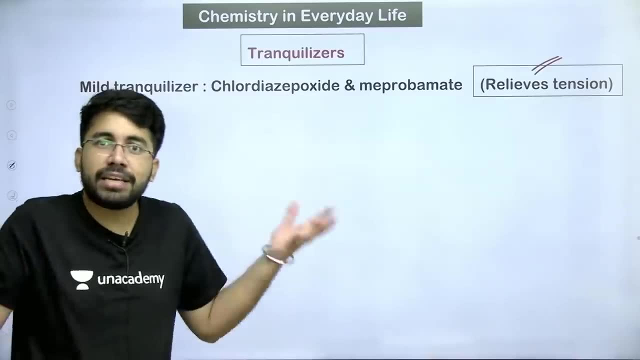 Okay, You don't have to go to the shop to buy That. give this a little, This one. So this is not A little tension. I mean you don't have a very big, severe depression victim. Then, friends, you have mild tranquilizers. 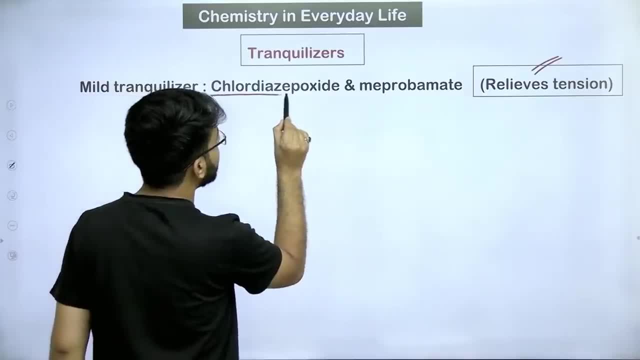 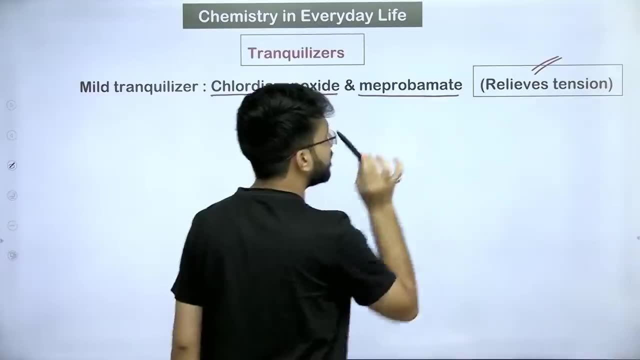 You use. This happens, friends, in front of you. Very big name is Chlordiazepoxide, First, And the second is friends Meprobemate. Chlordiazepoxide and Meprobemate are used like mild tranquilizers. 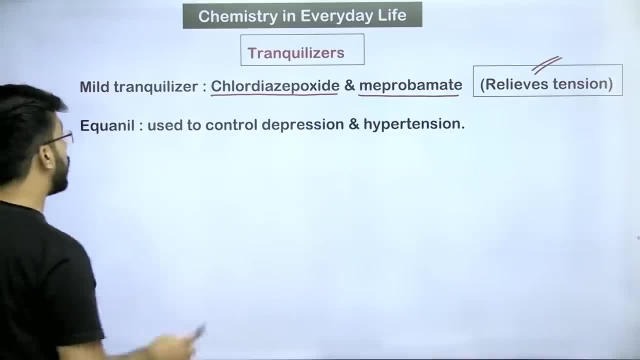 Okay. Now friends, you have Equanil. This is PYQ. What is Equanil? It is used for to control depression and hypertension. If the anti-depressant is just asking, then the last two will be Ipronazid and Nardil. If the mild tranquilizer or tension is small, then Chlordiazepoxide and Meprobemate, And if you have depression and hypertension, then you will use Equanil. Okay Next, my friends, Let's go ahead. 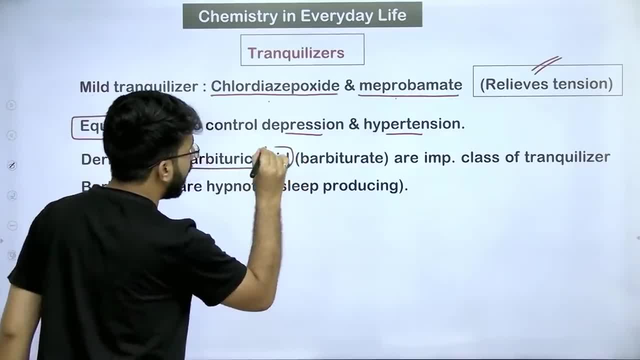 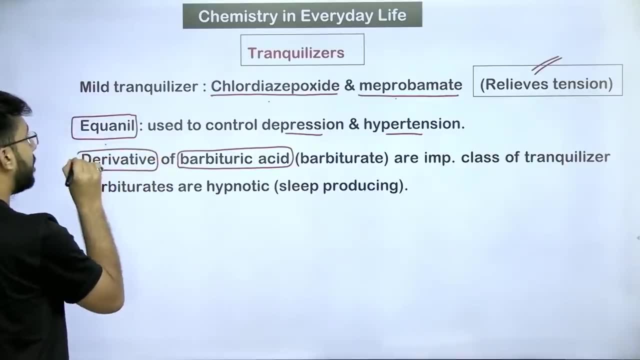 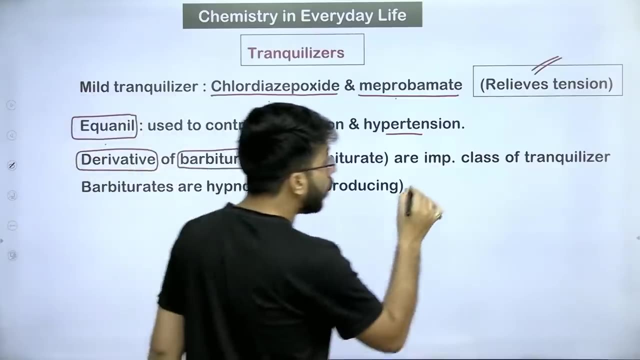 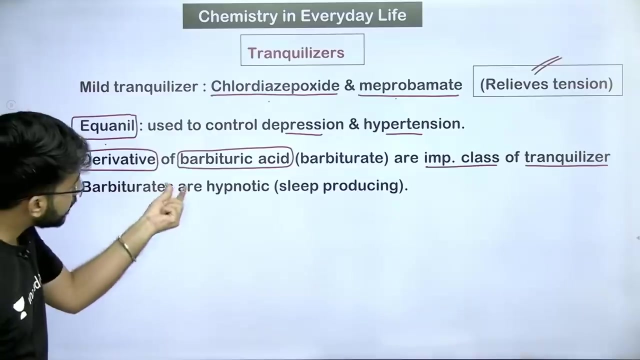 You have a barbituric acid. What happens? You have barbituric acid, Derivative of barbituric acid. You have barbituric acid. So what is the buildup? What is smokes? Either you. 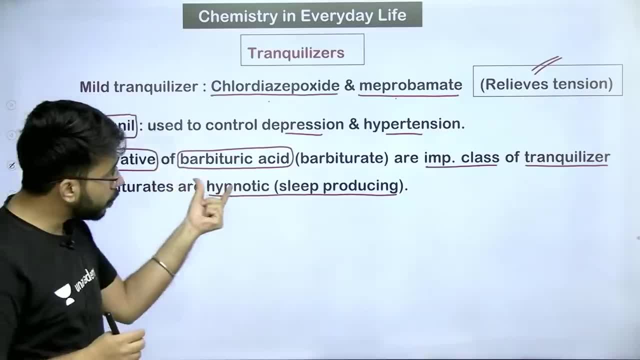 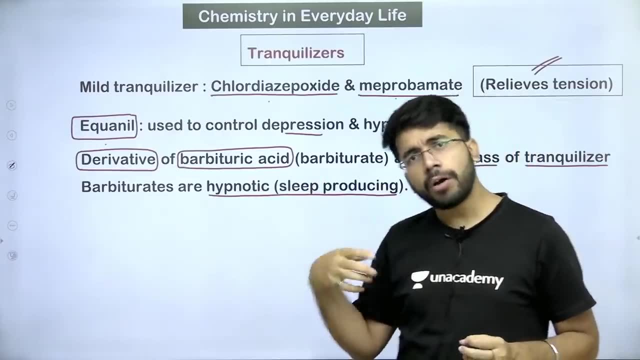 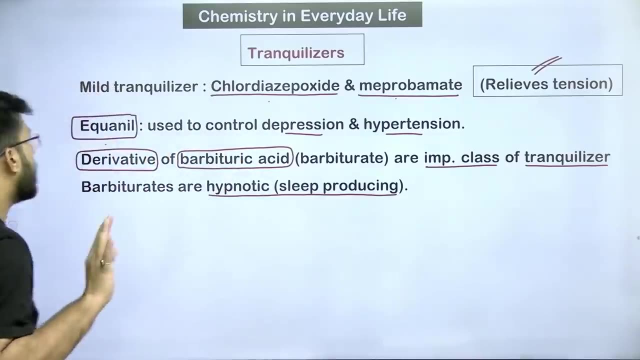 have barbituric acid, The mittlerweile. it is slimy If, according to, the Barbiturates are sleep producing. so basically, tranquilizers are made of barbituric acid and barbituric acid is of sleep producing nature. basically all the antidepressants are of sleep producing nature. they make you sleep. 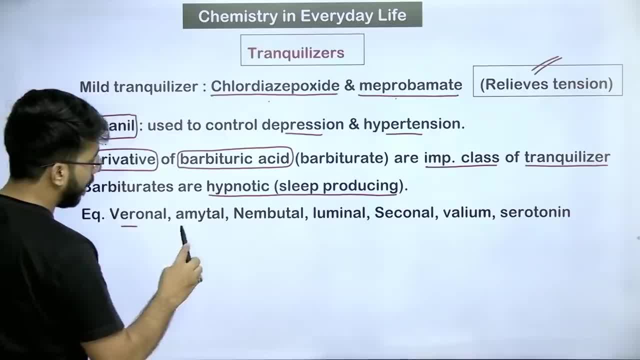 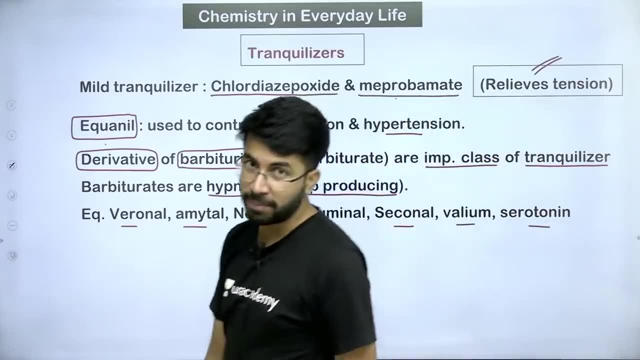 All these are tranquilizers. veronal, amytal, nebutal, luminal, seconal, valium, secrotonin- all these are tranquilizers. How can you remember so many drugs in tranquilizers? There should be a trick. 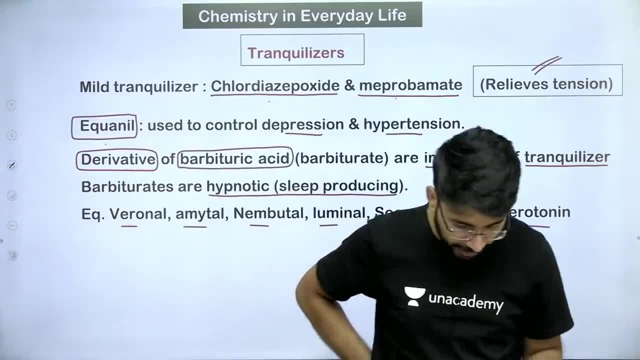 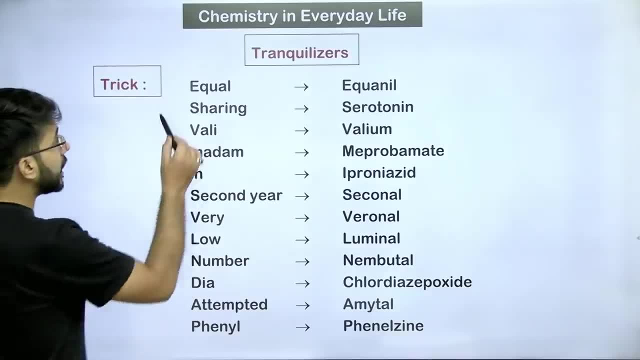 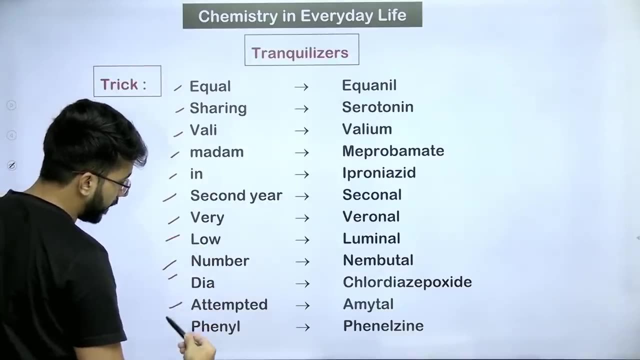 How can you remember so many drugs in tranquilizers? There should be a trick. Come, sir, I will tell you the trick of tranquilizers: Equal sharing madam in second year gave a very low number of attempted phenyl. Equal sharing madam used to give a number of equal sharing. 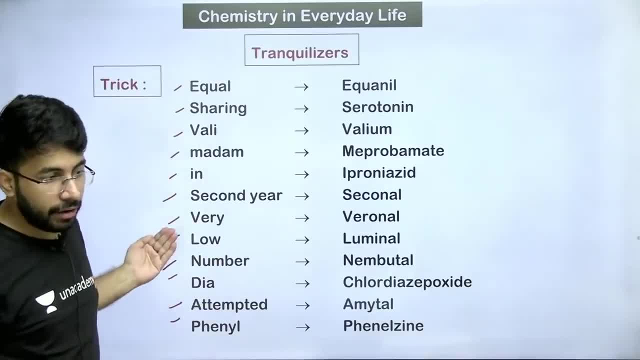 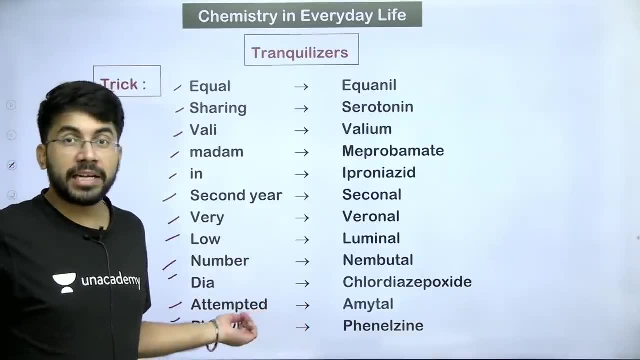 but equal sharing. madam in second year gave a very low number and when she gave a very low number, she tried to drink. phenyl tried to sacrifice her life for madam, which is completely wrong. Next, this is a little funny trick- now come. 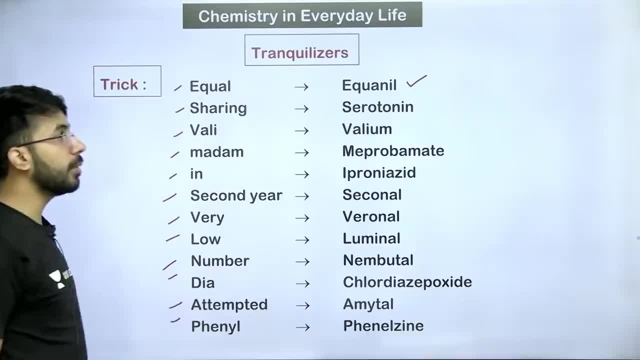 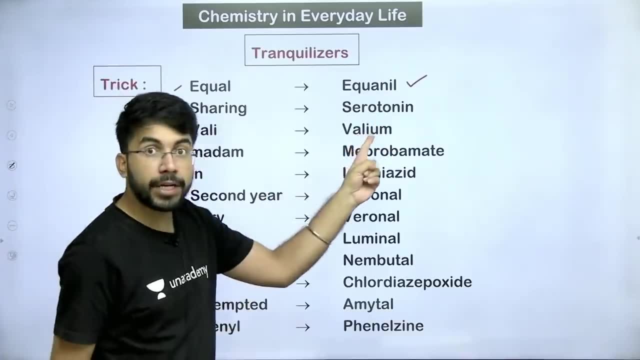 Equal means equanil. it is found in both hypertension and depression. Equal sharing means secrotonin. this is the derivative of barbituric acid. Friends valium is the derivative of barbituric acid. Meprobamate, my friend, you have a mild tranquilizer. 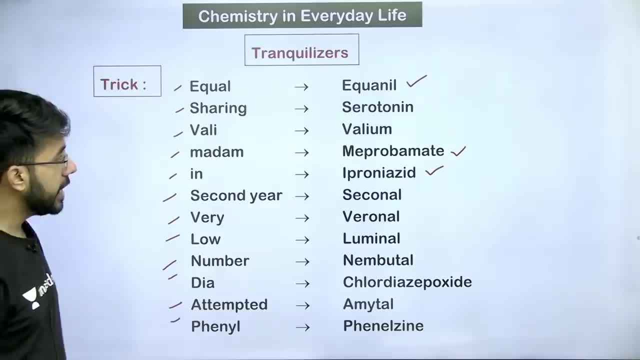 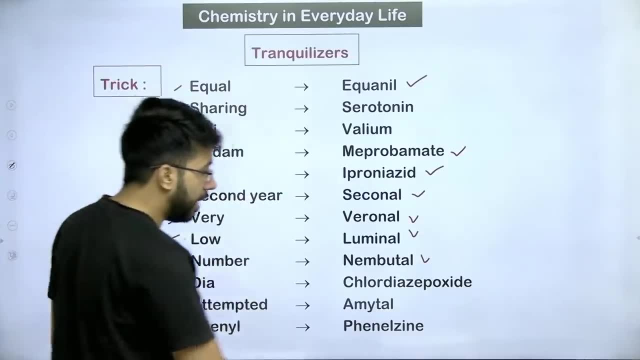 Epronazide. you have a simple anti-depression drug: Seconal, veronal, luminal and nebutal. what are these in front of you? These are all the derivatives of barbituric acid, Amytal and phenylzine. what are these in front of you? 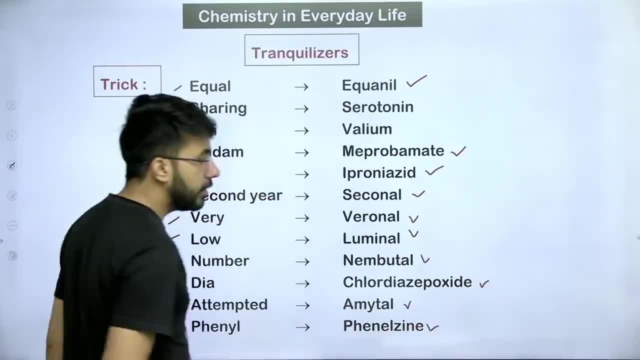 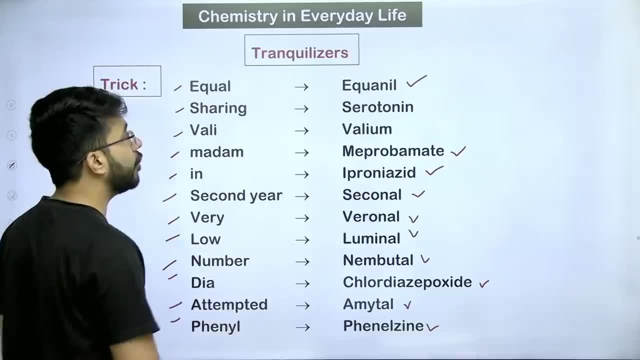 Barbituric chlordiazepoxide. what are these in front of you? These are mild tranquilizers, So all the tranquilizers will be remembered from here And in front of you. in PYQ, this has been asked- equanil right. 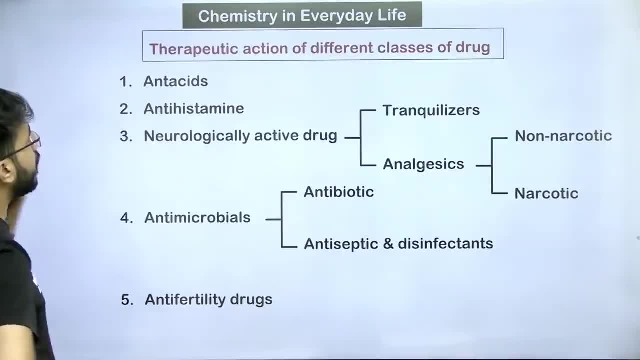 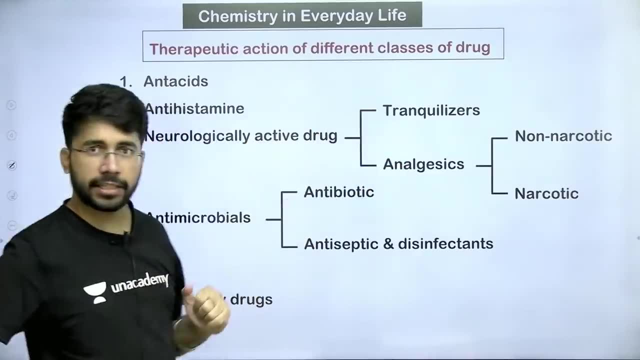 No problem. next, You have come after tranquilizers. you come to analgesics, right, Neurologically active tranquilizers and analgesics. What is analgesics? Let's understand: Analgesics are basically painkillers. 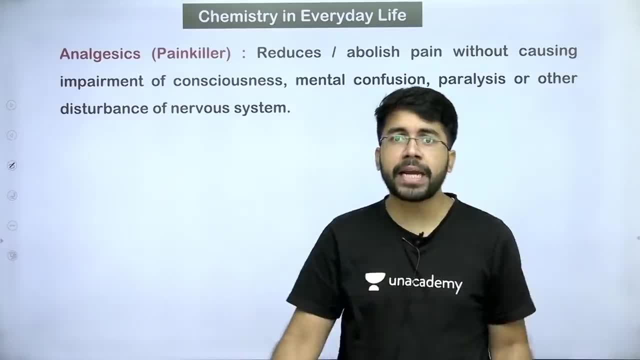 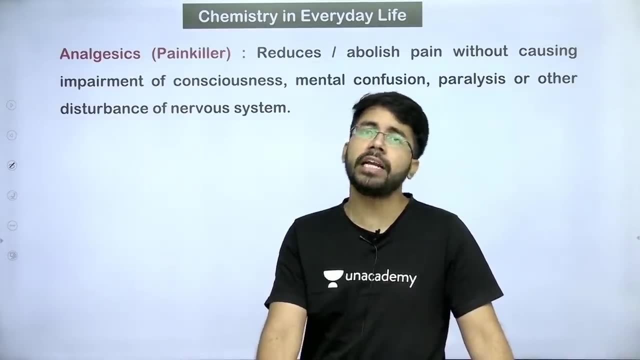 Like your operation etc. happens. So we make that part pain. what do we do? We make it zero. It is said to make that part zero That whatever you operate bring phenyl Or you are made unconscious. 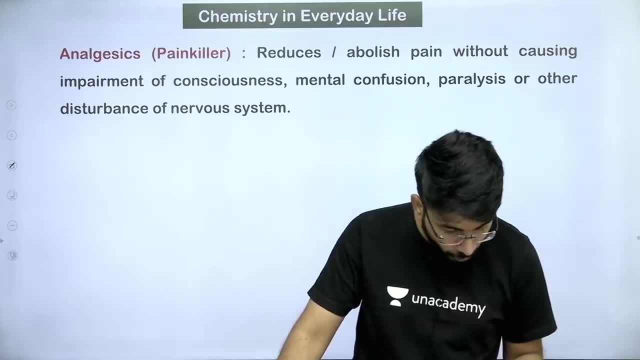 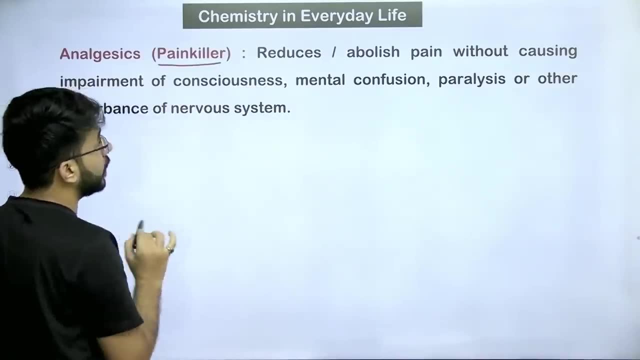 Okay, By giving chloroform, etc. you are made unconscious. So what is that for you, friends? Neurologically active drug? analgesics, Let's come. What is analgesics? We have the category of painkillers. 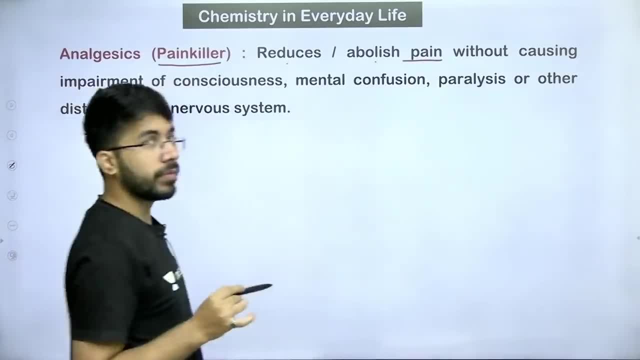 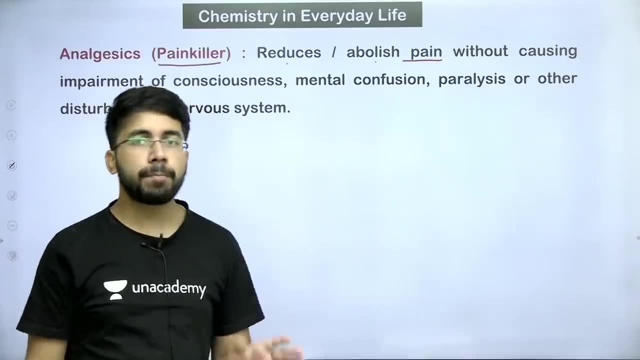 It reduces or abolishes pain. Now it is not that pain is killing you. Now it is not that pain is killing you, But when the pain is killing you, then somewhere or other nervous system See how the pain can be TERMINATED. 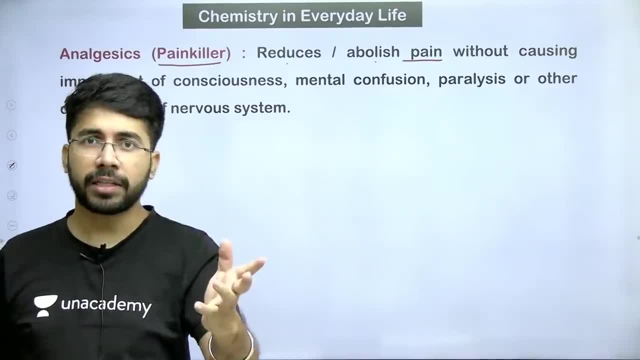 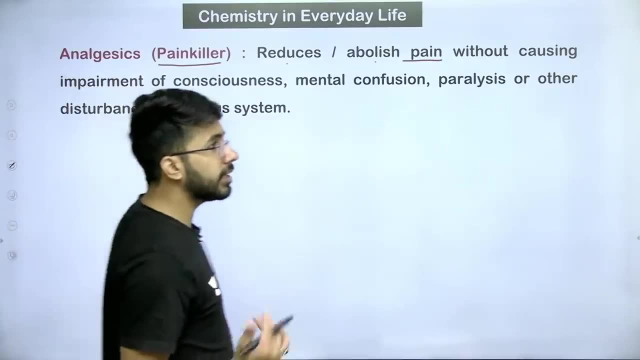 If your nervous system does not receive a message, if the nervous system is spoiled, you will not feel the pain, Because when the brain does not receive any message, you will know what is happening. Like some people- alcoholics- you see that when they are high in intoxication. 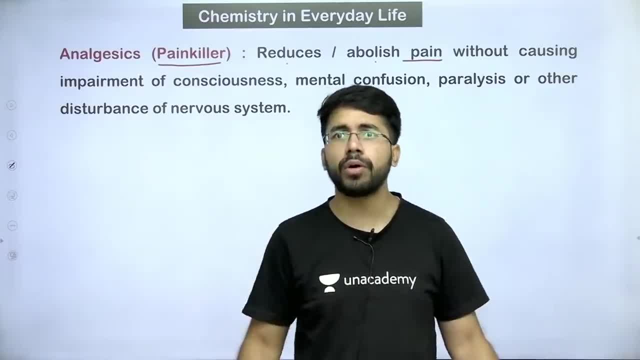 their cut is hurt, hand is broken or leg is broken, It does not matter, and at that time they do not feel any response. Why so? Because their brain does not receive any message at that time, Because their brain does not receive any response at that time. 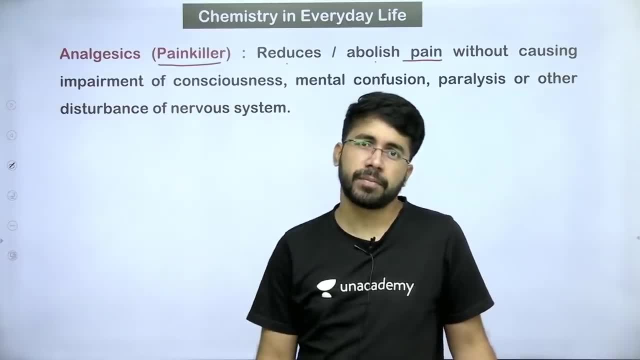 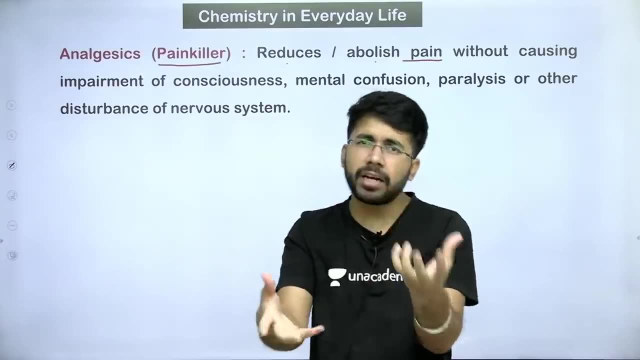 At that time the brain's receptor is very slow down. They are not thinking about anything in the present. So if they don't message their brain, then there will be no difference in cutting. breaking of hands and legs. Yes, but let it happen in the next morning. 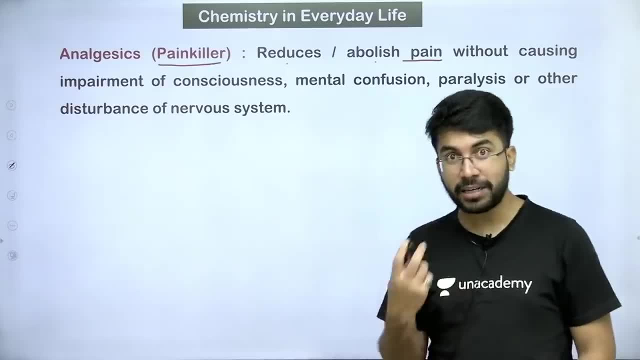 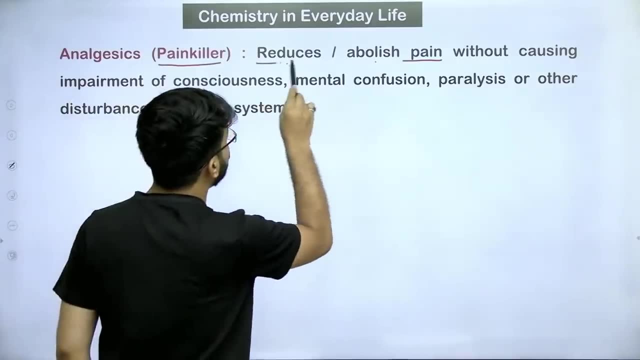 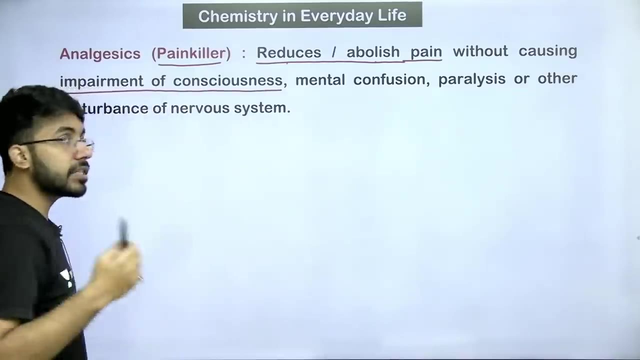 When your brain's receptors are ready, then they shout loudly. So this is the thing, my friends: that analgesics are painkillers which reduces an abolished pain without causing impairment of consciousness, Without disturbing your consciousness, Without disturbing your consciousness. 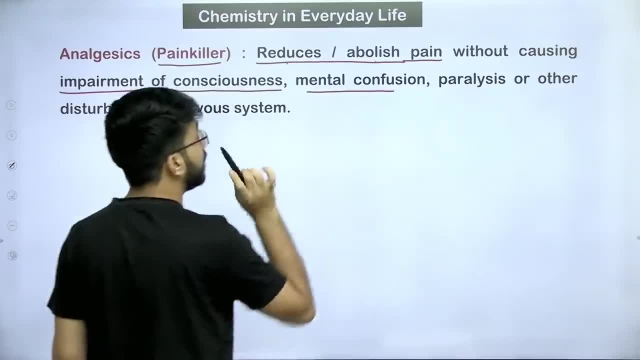 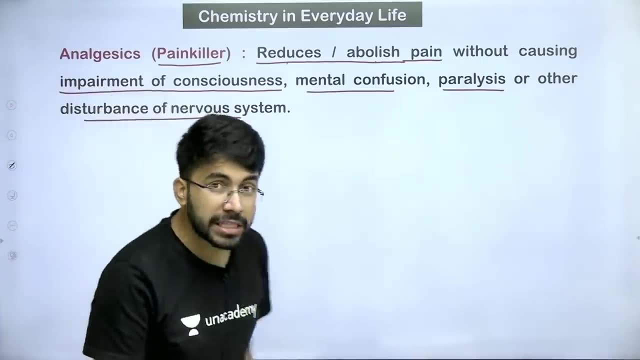 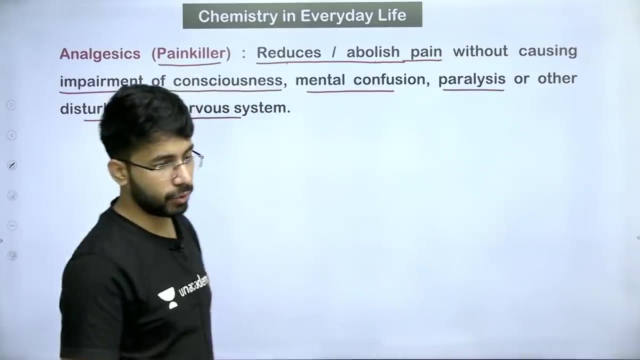 Second, without causing mental confusion, Without causing any paralysis or other disturbance of the nervous system. Basically, without disturbing the nervous system. analgesics is a painkiller that reduces or removes your pain. Yes, Without disturbing the nervous system. Next, 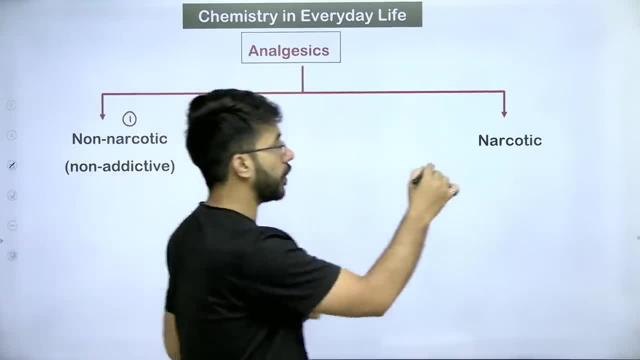 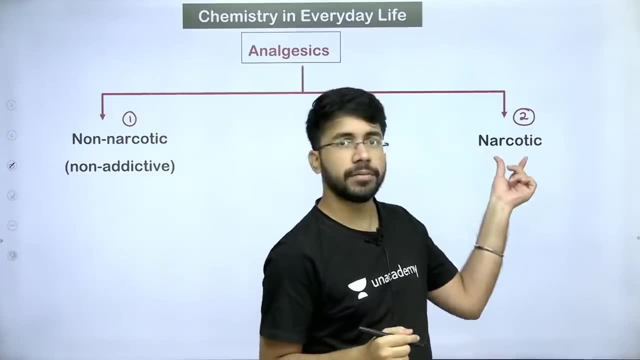 Analgesics is of two types: One is non-narcotic and the other is narcotic. Non-narcotic is that which is addictive, Sorry, that which is not addictive. Narcotic is addictive. This will not be addictive, But this will be addictive. 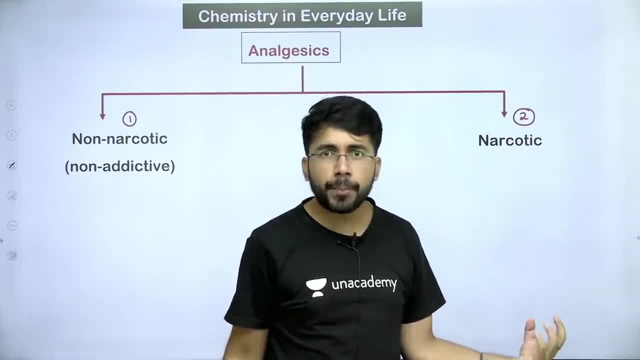 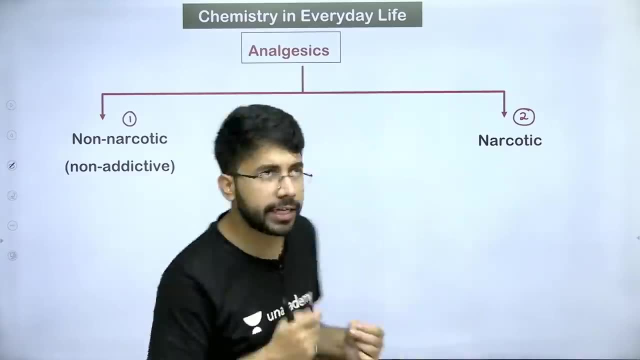 Okay, Now we will show that it is made of aphene, Opium poppy. It is made of the flower of opium. It will be made of aphene. Okay, That is why it is addictive, Obviously. And, friends, these will be non-addictive and non-narcotic. 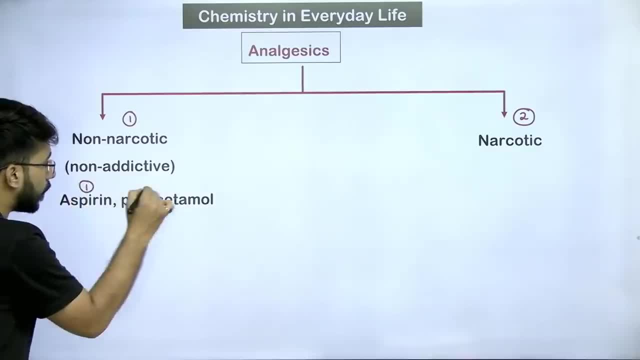 I will tell you one by one The aspirin and paracetamol that you take. The question has come PYQ, Aspirin and paracetamol. These are non-narcotic drugs. Aspirin and paracetamol. 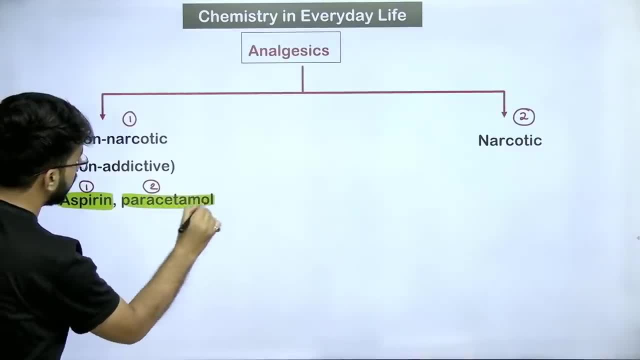 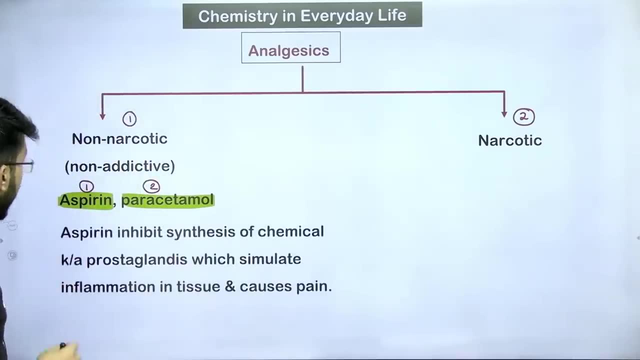 These are non-narcotic drugs. These are analgesics that reduce your pain. Okay, Come Next. You will come to know what aspirin does. Understand Aspirin: What does aspirin do? It inhibits, It stops. 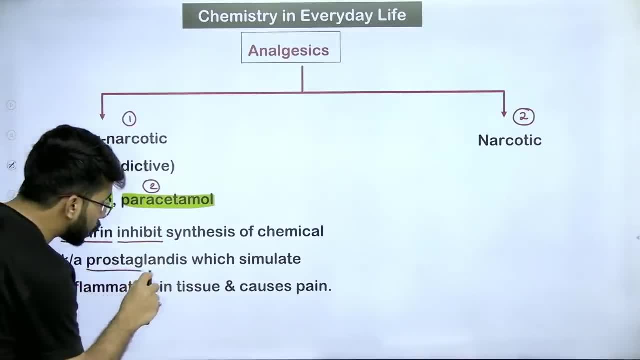 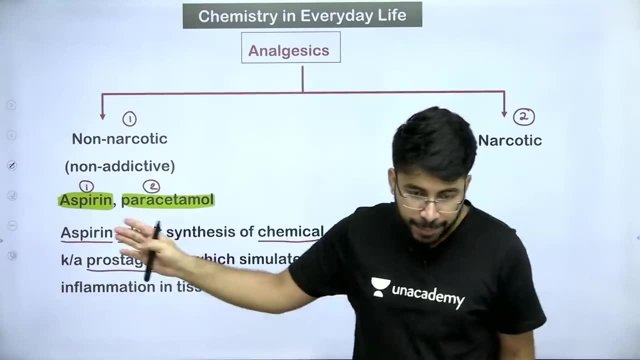 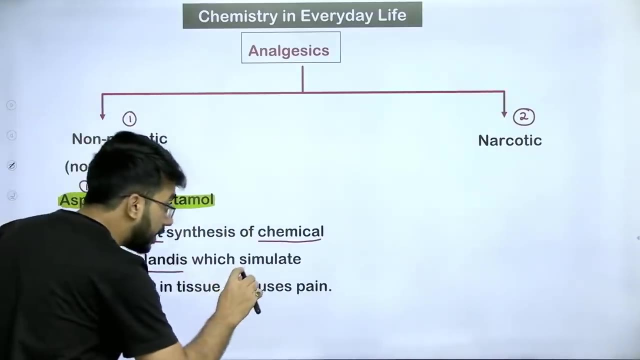 What is that? It is a chemical posta-glandis. It is a chemical posta-glandis. Aspirin inhibits chemicals known as pasta-glandis. It simulates inflammation inux and causes pain. What does posta-glandis mean? 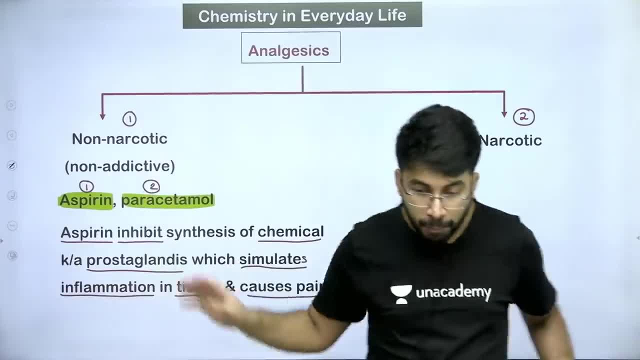 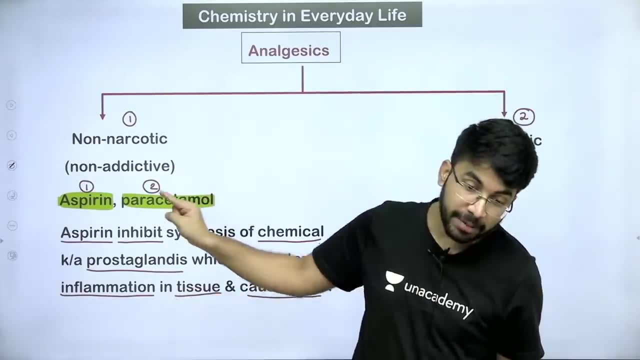 Your tissues begin to expecting inflammation, Cinghan jane. It causes swelling in your tissues which causes pain, And to reduce that pain we give aspirin. And what does aspirin do? It stops the synthesis of the posta glandis. 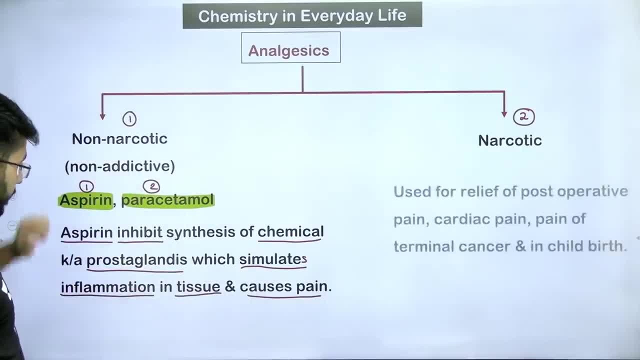 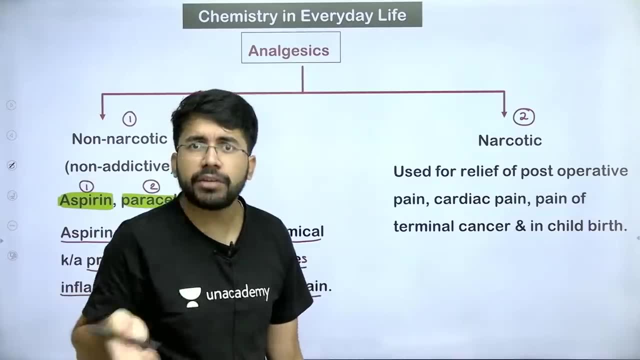 Okay, Let's move ahead. What is narcotic Like? post-operative pain. Even after the operation, there is a lot of pain. You have been irritated in many places. So the post-operative pain. For its relief, you use narcotic drugs. 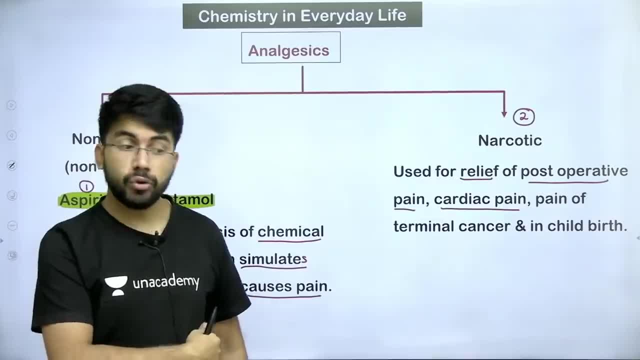 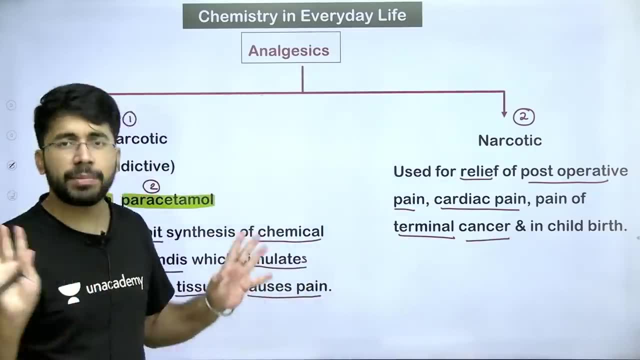 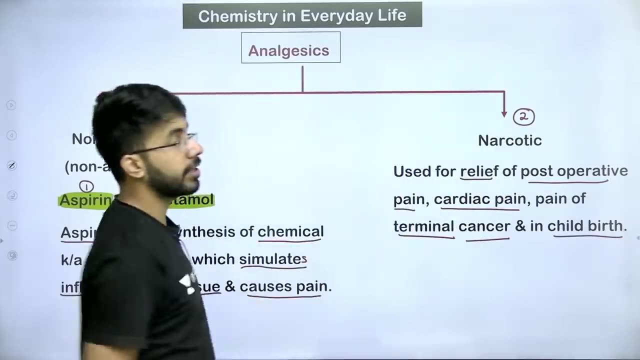 Or Cardiac pain. For that what do you use? Narcotic drugs, Pain of cancer, terminal cancer. I have no idea about terminal cancer, But I have written it in NCERT To relieve the pain of terminal cancer And even in childbirth we use these narcotic drugs. 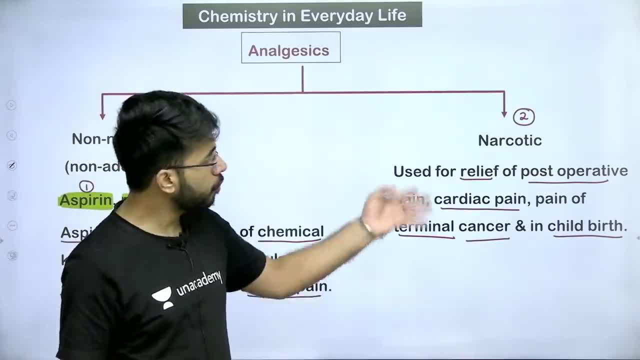 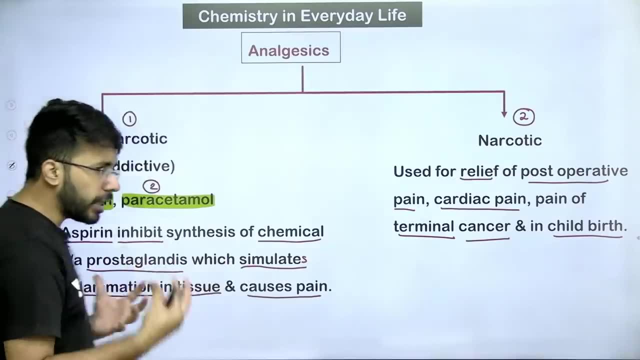 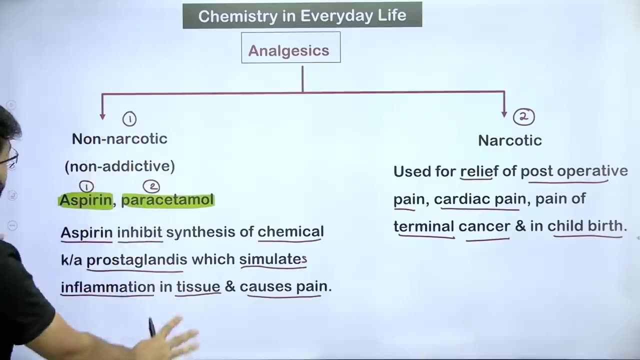 Even at that time, Wherever you are seeing unbearable pains, They are narcotic drugs. in all places, Okay, And in tissues There is not much pain. If there is heavy pain, Then you can use narcotic. If there is a little pain. 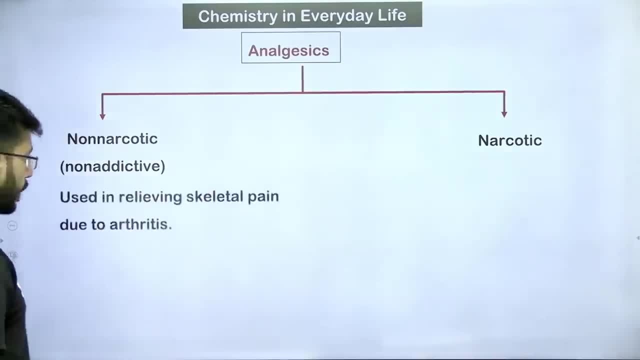 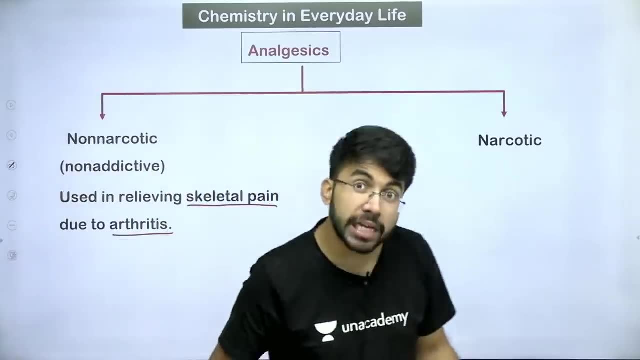 Then you can use non-narcotic drugs. Non-narcotic drugs: It is used in relieving A skeletal pain due to arthritis. Due to arthritis, A skeletal pain. To get rid of it, We use non-narcotic drugs. 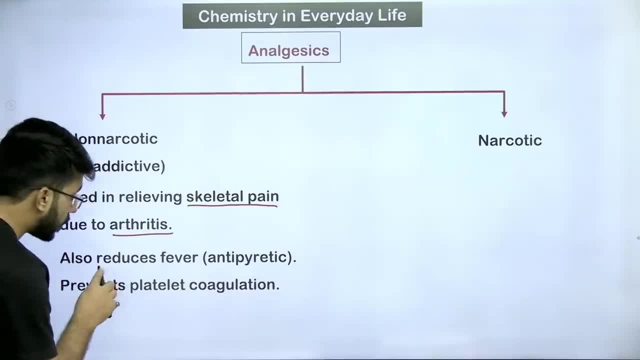 Okay, Next, also reduces fever. Do you remember? Paracetamol is given in fever. Aspirin is also given in fever. It reduces fever. That's why it is called antipyretic. Pyro means heat, And anti-heat means to reduce fever. 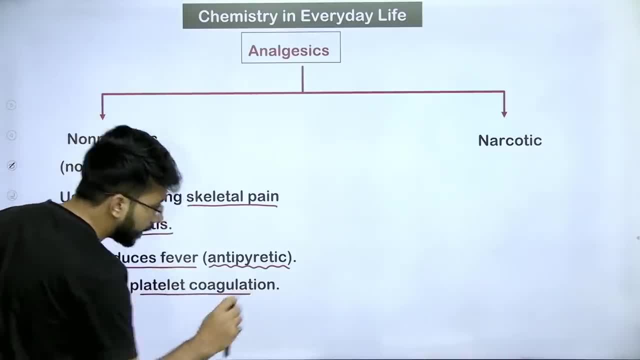 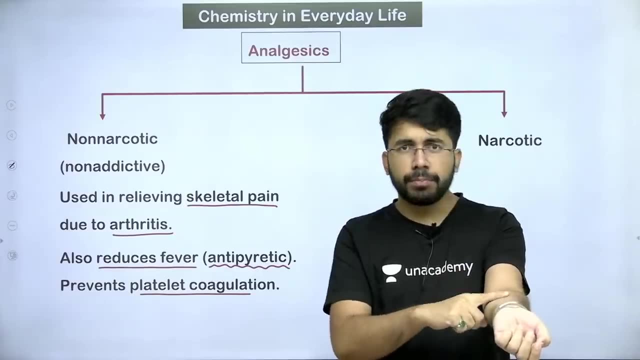 It is called antipyretic And prevents platelet coagulation, Your blood coagulation. You see, If there is a cut After a long time, The brownish gets frozen, That is because of the coagulation. 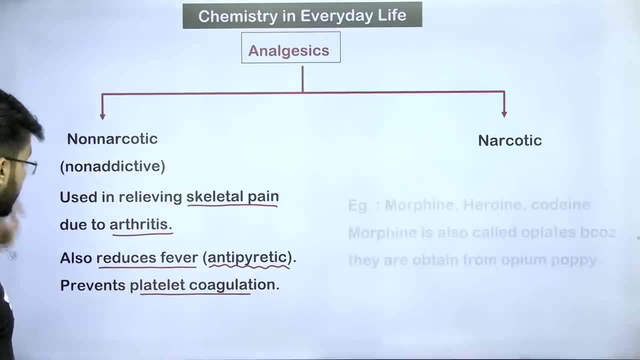 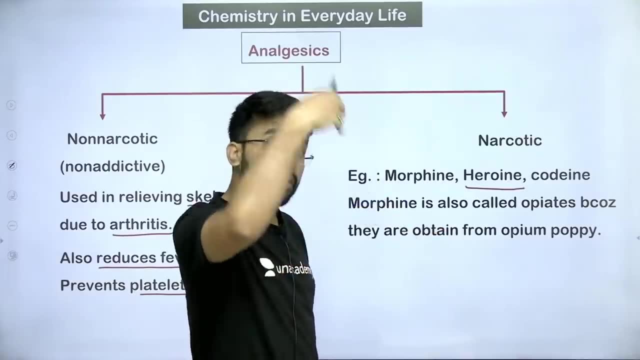 So it also reduces platelet coagulation. Now let's come to the next In narcotic drugs. You see heroin. You see heroin. This is a drug. Codine, Codine is also a narcotic drug. 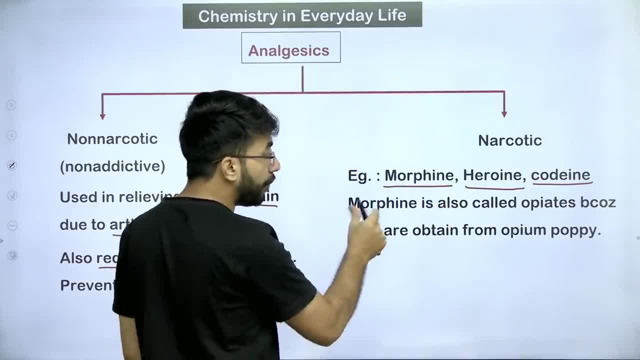 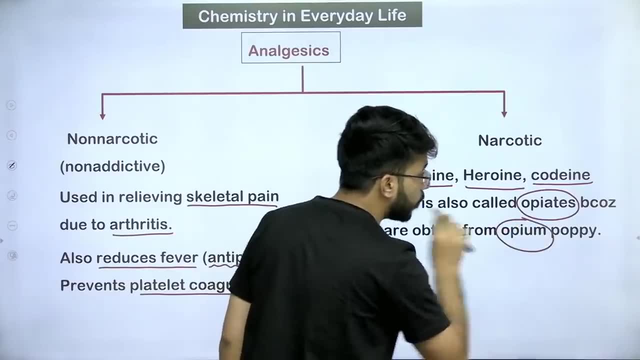 Morphine is also a narcotic drug. Morphine is also a narcotic drug. Morphine is also called opiates. Opiates are called opiates because It is made from opium. Opium poppy means It is made from opium. 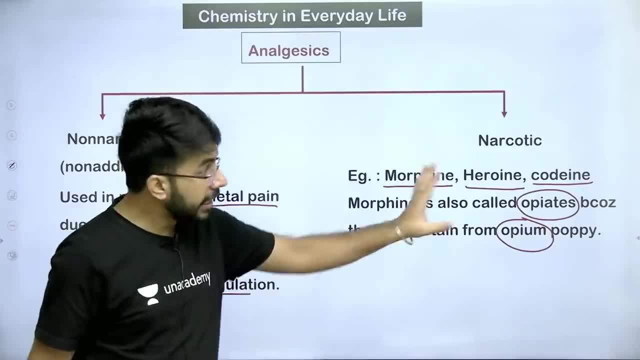 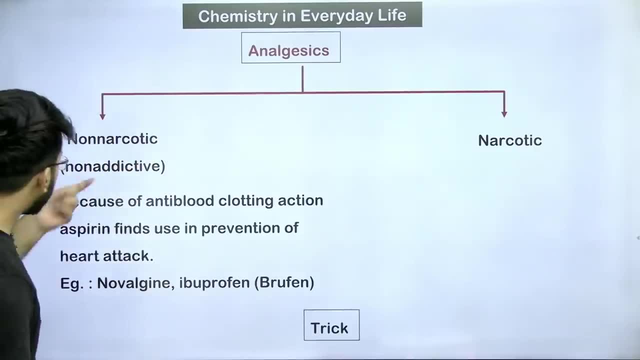 That's why it is addictive. That's why it is sleep-causing. It is used in heavy, unbearable pain. It is used in heavy, unbearable pain. Next, You will get it in non-narcotic, Because it has anti-blood clotting action. 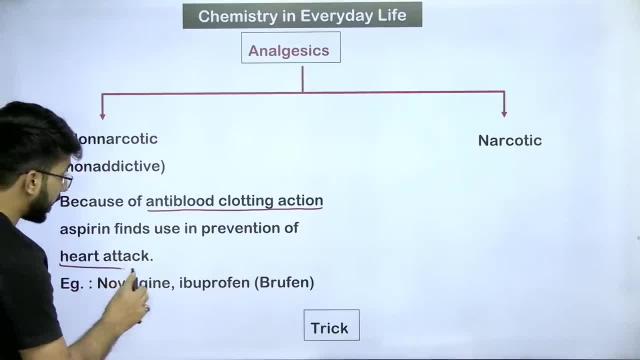 Because it has anti-blood clotting action. So what it does is It is also used in heart attack. Aspirin is used in heart attack. Aspirin is used in heart attack. Now let's come to Novalgine and ibuprofen. 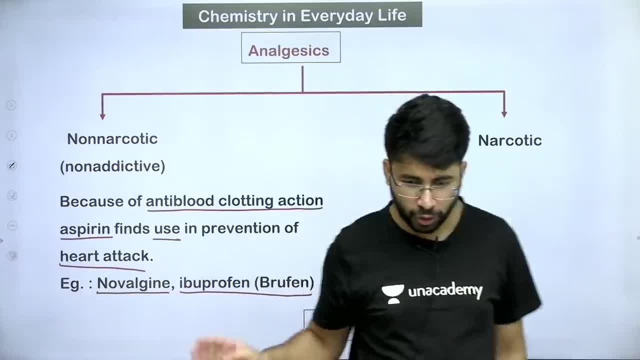 Ibuprofen is also taken in fever. I mean, the doctor has suggested this to me many times. So ibuprofen is also used in fever. So ibuprofen is also used in fever. So ibuprofen is also used in fever. 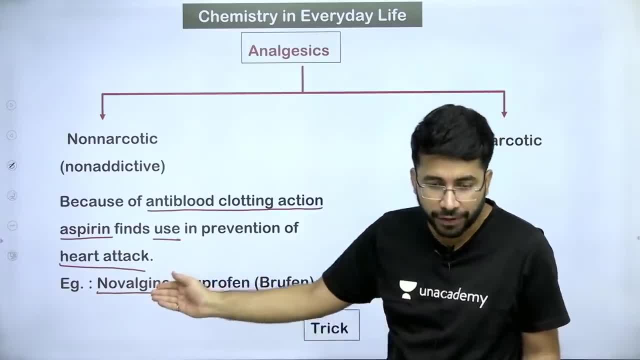 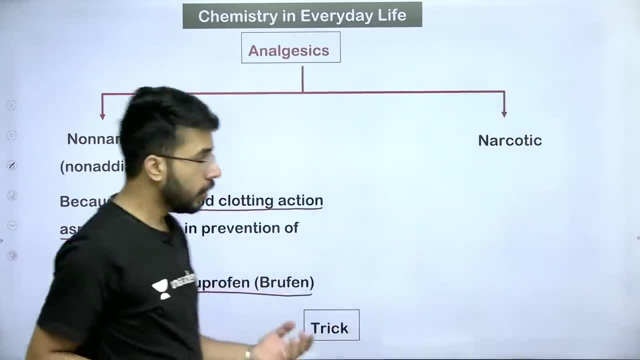 Aspirin, paracetamol, ibuprofen. Aspirin, paracetamol, ibuprofen or Novalgine- All these are analgesics. All these are analgesics. And what about narcotics? 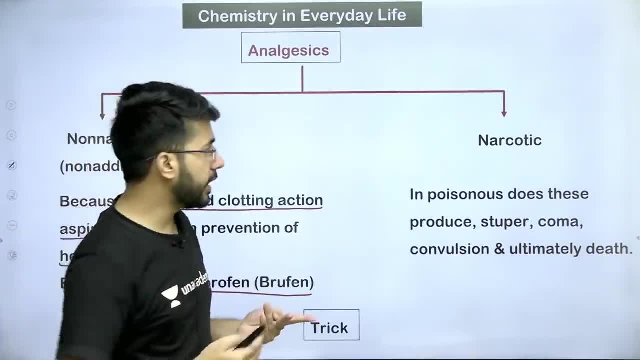 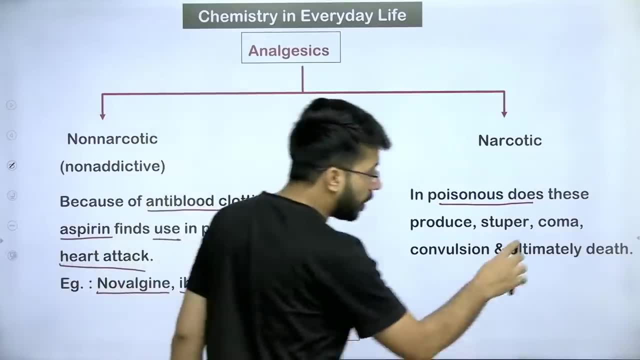 And what about narcotics? Codine, morphine heroin, Codine, morphine, heroin. These are poisonous doses. If I use too much of heroin, you will go into coma. You will become stupor. Stupor means you will become unconscious. 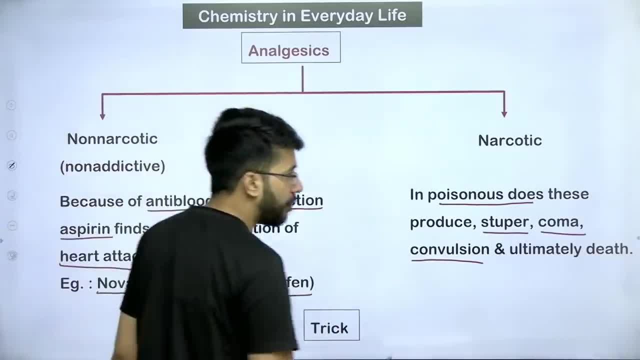 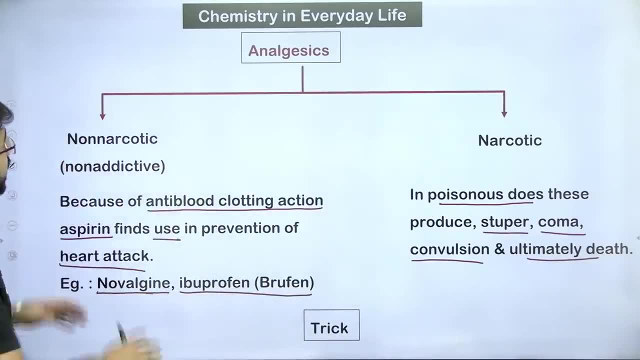 Convulsion means it is a case of unconsciousness only Or paralyzed unconsciousness, And finally you can love Ram. And finally you can love Ram. So this was the story of analgesics. If you have small pain, use aspirin, paracetamol. 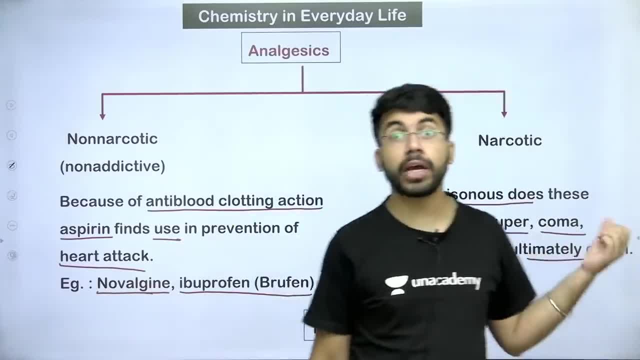 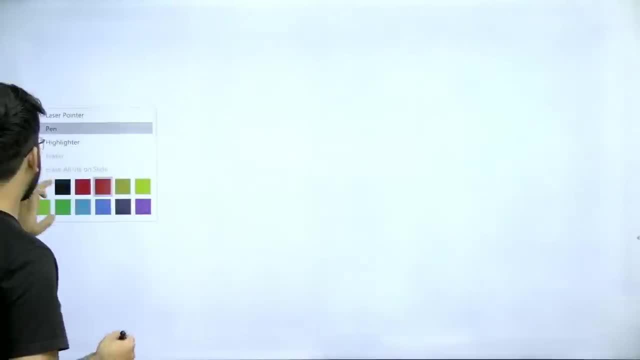 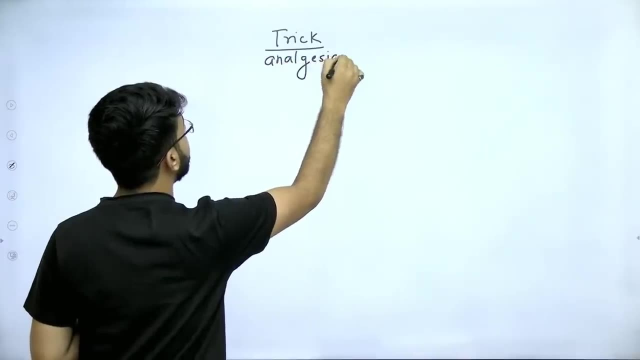 ibuprofen or Novalgine. Otherwise you will have to use heroin, codine, morphine. Next, you can see that it has a trick. It has a trick: It is about analgesics. I will tell you what is the trick of analgesics. 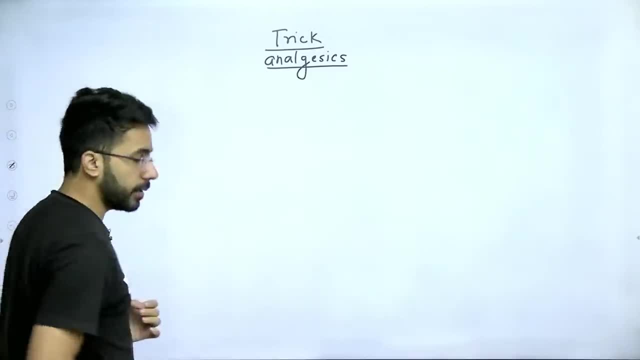 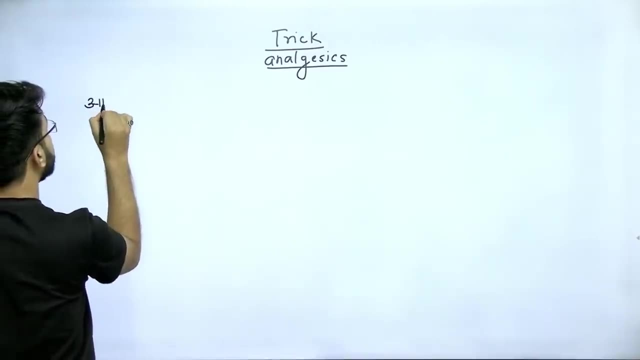 I will tell you what is the trick of analgesics. You will understand the trick of analgesics with love. You will understand the trick of analgesics with love. We have Asha Friends. what is Asha? I am writing Non Narcotic here. 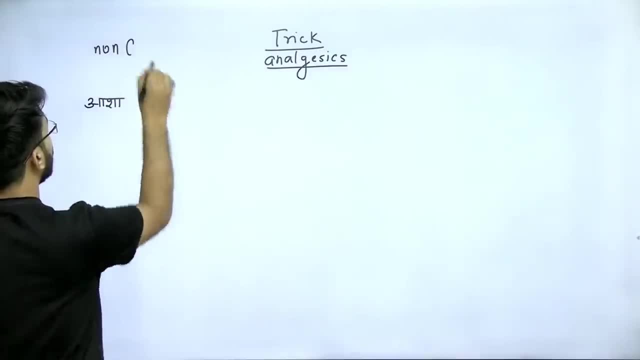 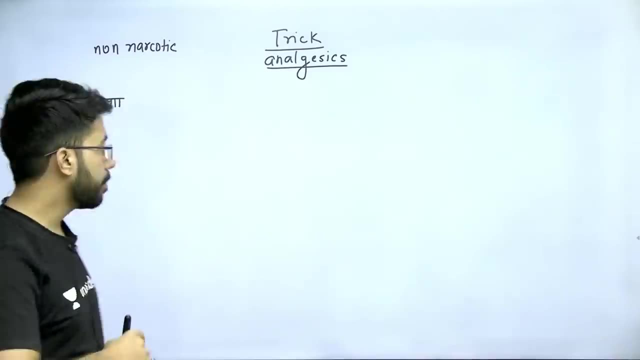 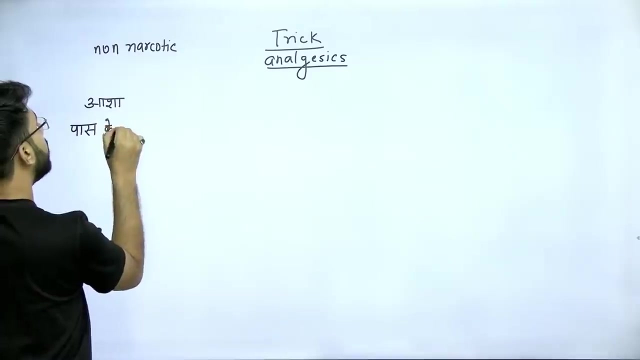 Non Narcotic. On the left hand side I am writing Non Narcotic, Non Narcotic, narcotic Asha. Asha is a pass mall. Asha pass mall, Novel brush lai. Asha pass mall, Nobel brush lai. 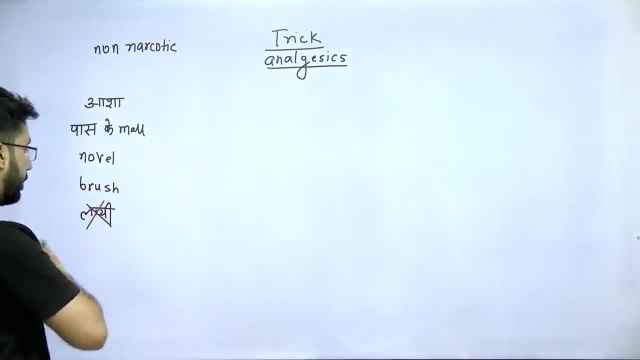 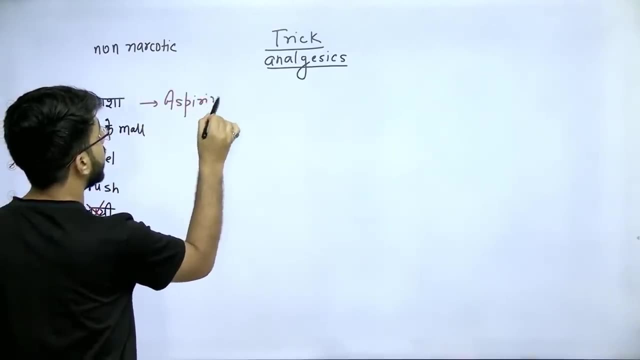 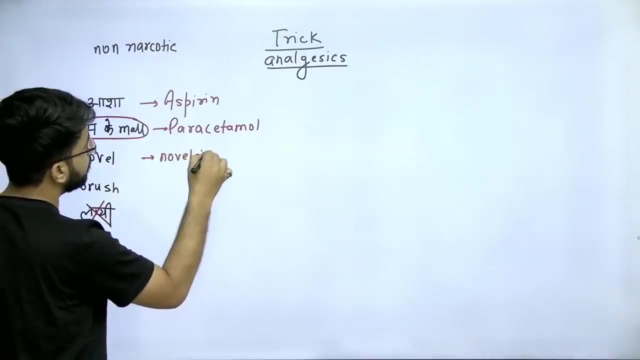 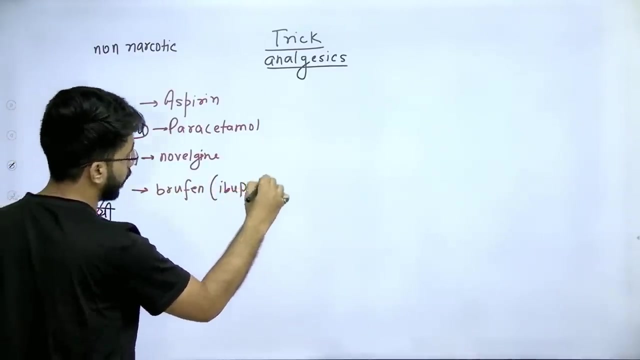 Novel and brush Novel brush lai Asha means espireal Pass mall. means paracetamol Pass mall, Paracetamol. Paracetamol Novel means novel. gene Brush means brofen or ibuprofen- Ibuprofen. 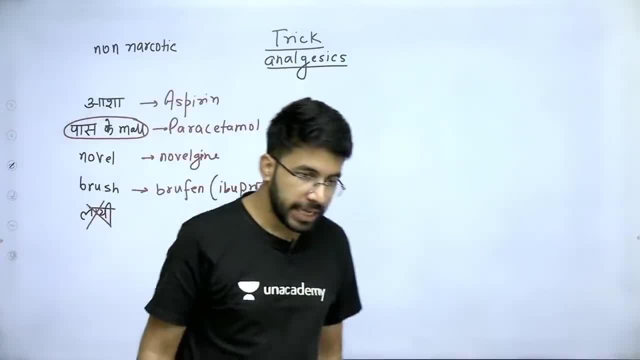 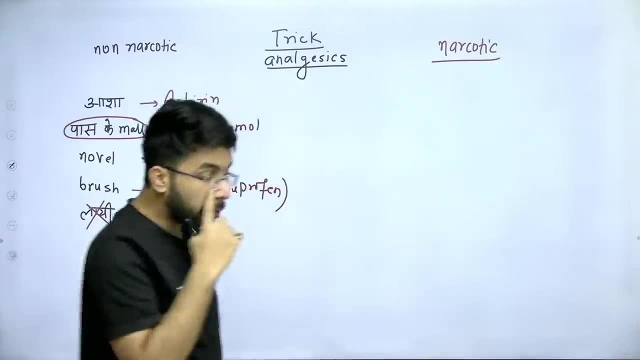 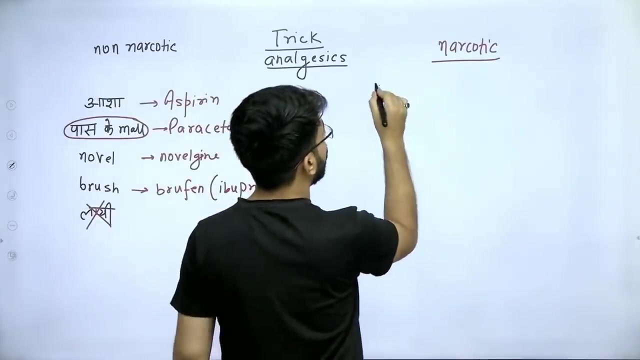 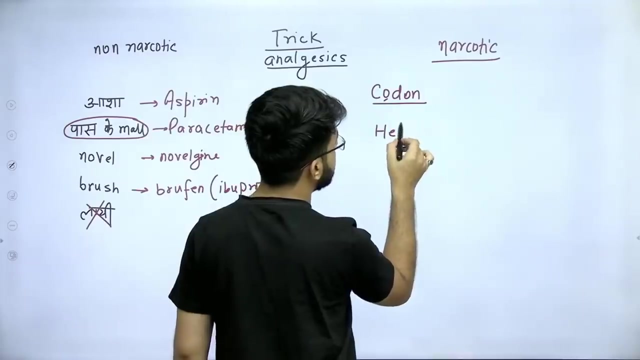 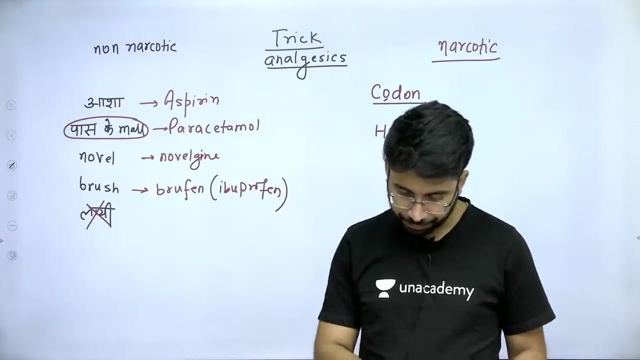 Novel means. These are non-narcotic drugs, but narcotic drugs will also come in front of you, which will produce sleep. What is narcotic drugs? In narcotic drugs, you will understand that the hero likes heroin, Morphine, codeine and analgesics. 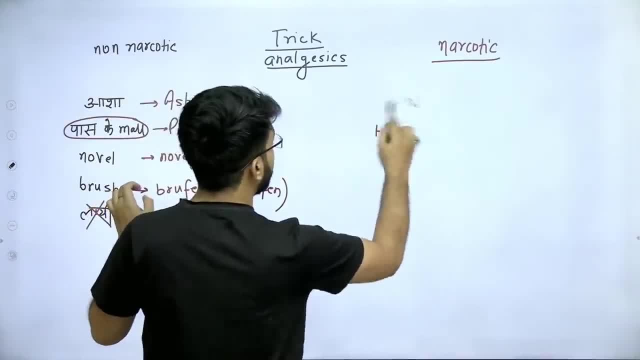 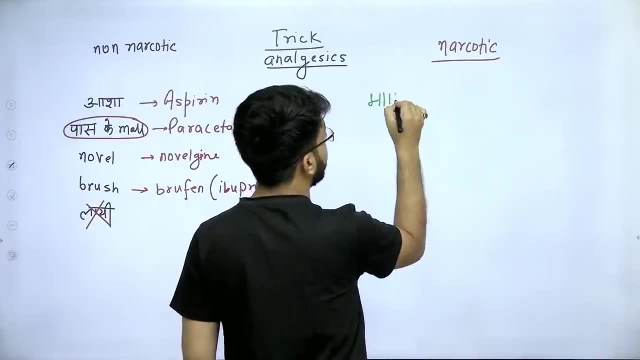 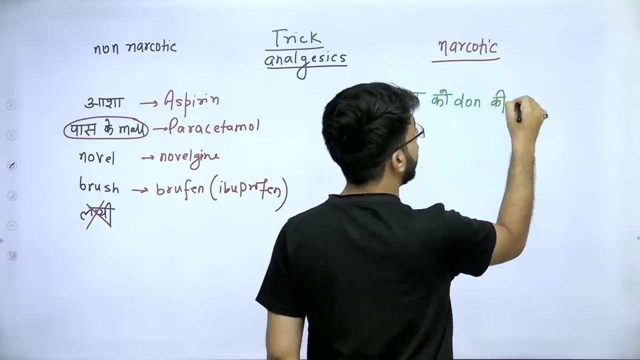 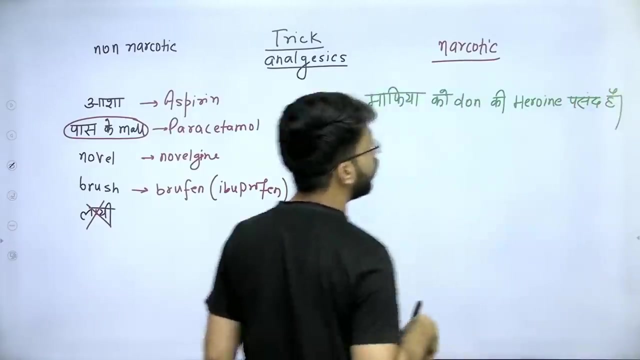 The trick here is that there is a mafia in front of you. The mafia likes the heroine of the don. What is it Now? this will be a very bad situation. The mafia likes the heroine of the don. The mafia means morphine in front of you. 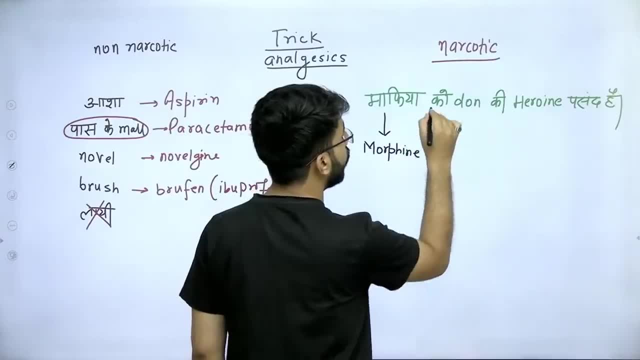 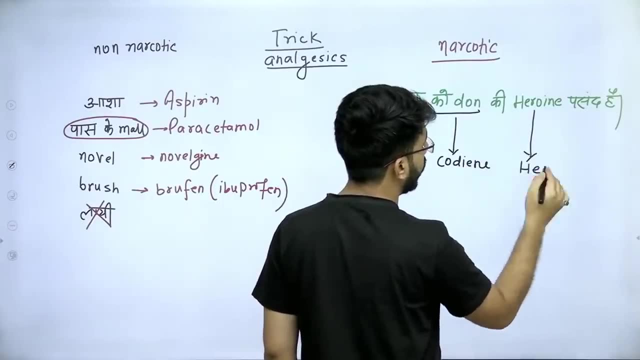 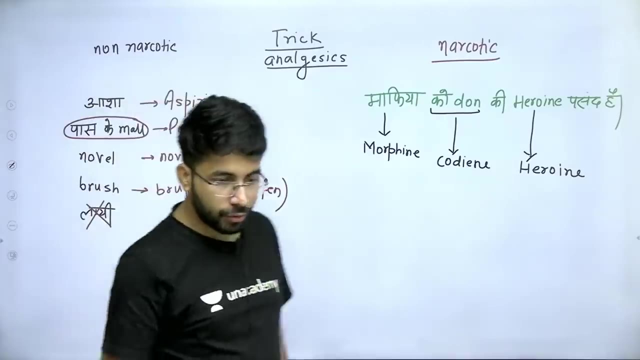 The mafia's friend is morphine in front of you, Codeine means codeine in front of you. Heroine means morphine, codeine and heroin. Morphine, codeine and heroin are narcotic drugs. The mafia likes the heroine of the don. 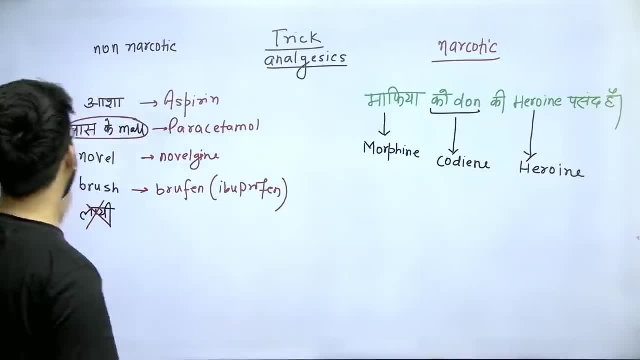 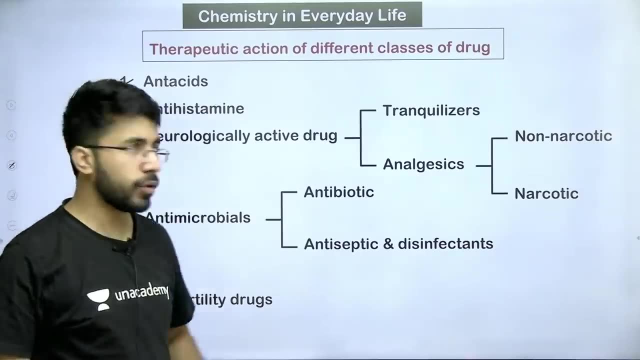 These are narcotic drugs, The drug that is addictive. Come on So in front of you. anti-acid and anti-stamina have also been done. This tranquilizer and analgesics have also been done. Non-narcotic and narcotic have come in it. 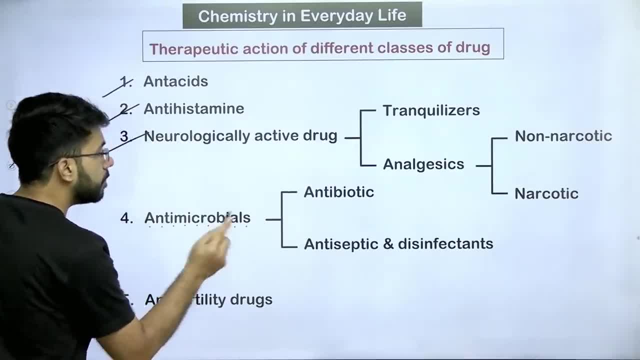 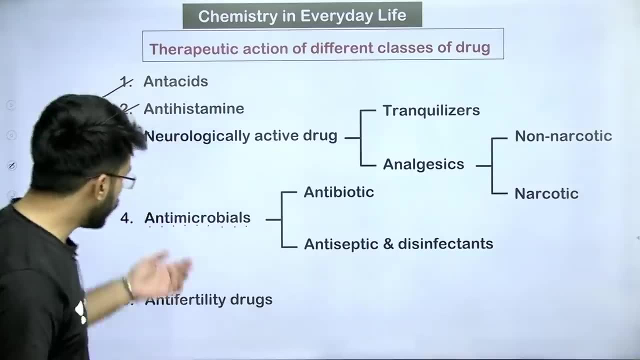 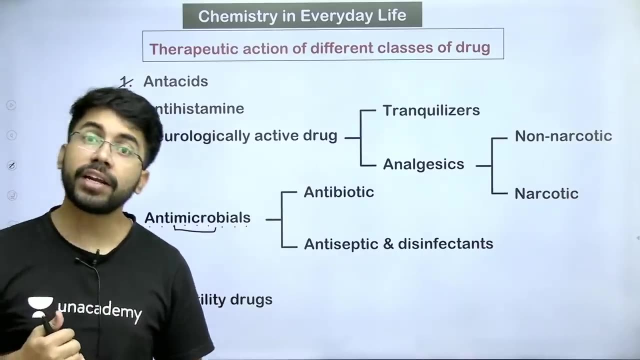 Now in front of you: antimicrobial, Like antibiotic, antifungal, antiviral, antiparasitic- All these are friends who will work on microorganisms Which will reduce microorganisms Like viral fever. So the virus is growing inside your body. 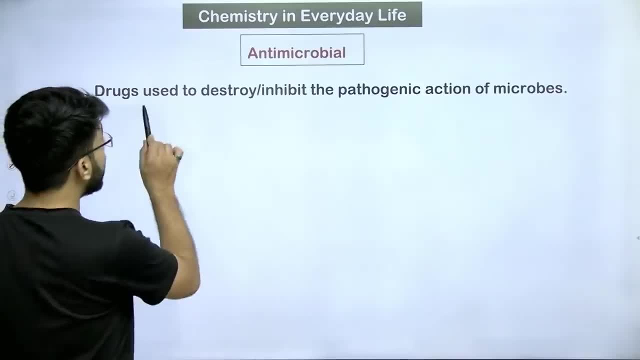 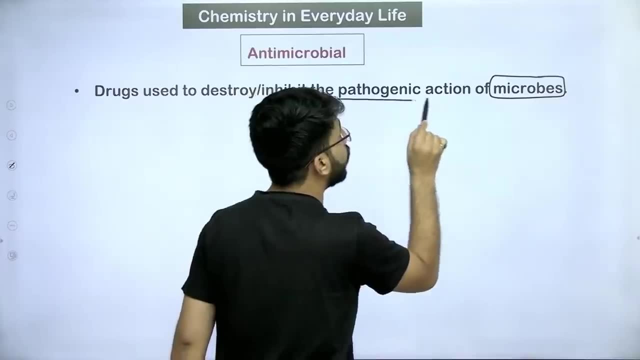 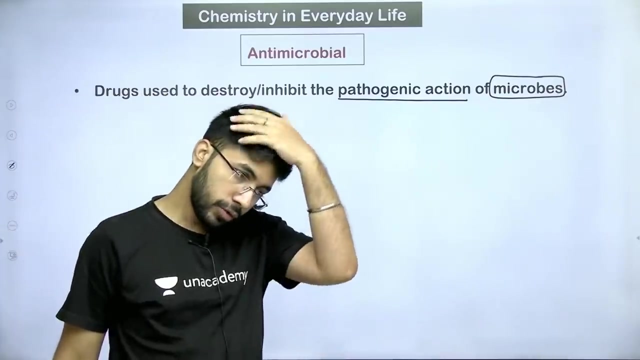 Antiviral Which will reduce microorganisms. Drugs used to destroy the pathogenic action of microbes. The pathogenic action of microbes Which will destroy. What do we call it? We call it antimicrobial drug. What do we call it? 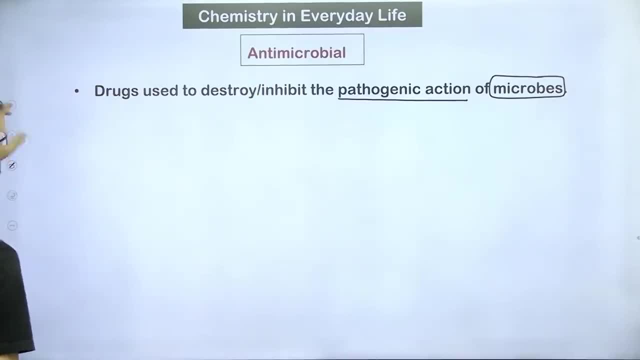 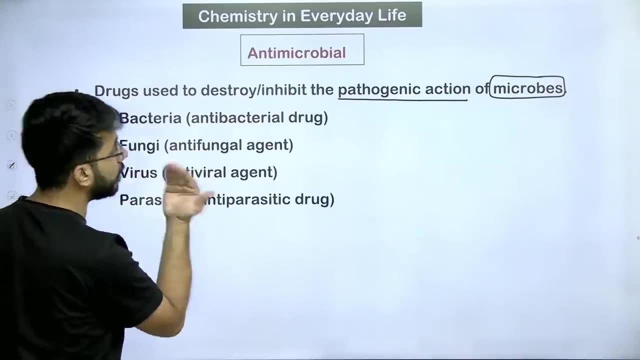 Antimicrobial drug. Okay, Come on, Let's call it antimicrobial drug Now, Like, if bacteria is growing, Then we have to give antibacterial drug. If fungi is growing, Then we have to give antifungal drug. If virus is growing, 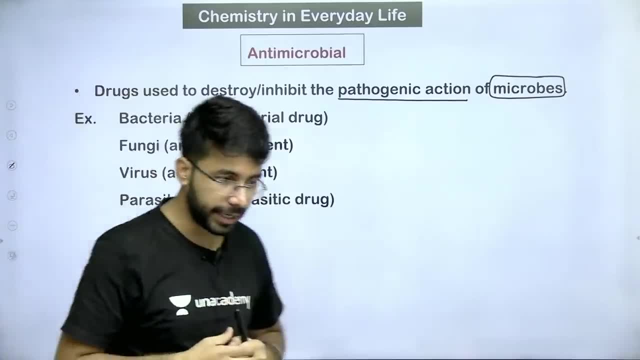 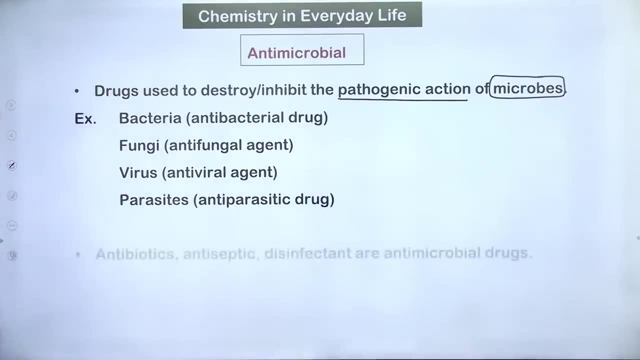 Then we have to give antiviral drug. If parasite is there, Then we have to give antiparasitic drug. I think this is clear: Antibacterial, antifungal, antiviral, antiparasitic. Next Come here. 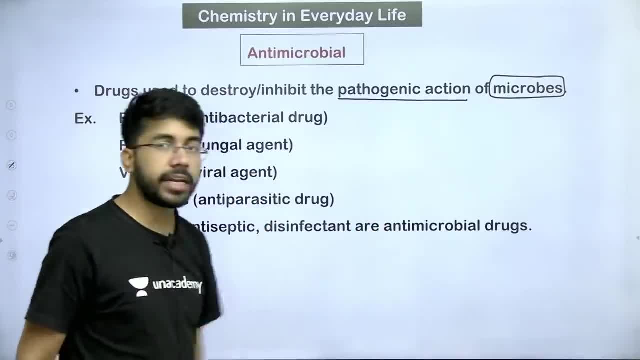 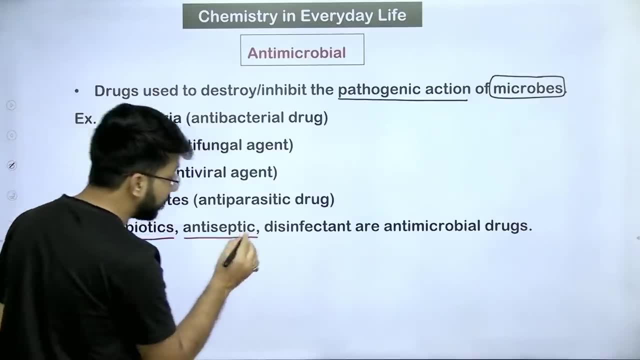 Antibiotic, antiseptic, disinfectant are antimicrobial drug. If you are giving antibiotics, They are also antimicrobial, Antiseptic In wounds. In wounds. If you are using antiseptic at the inside, You are using antiseptic at the inside. 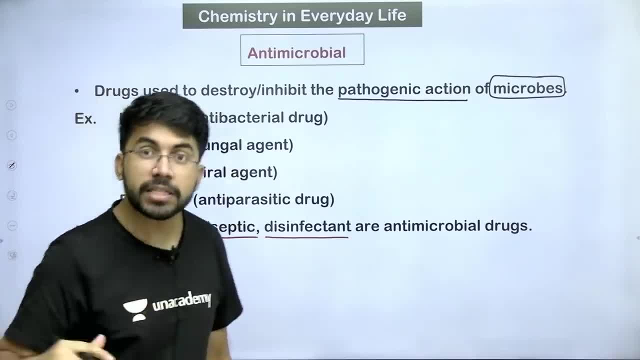 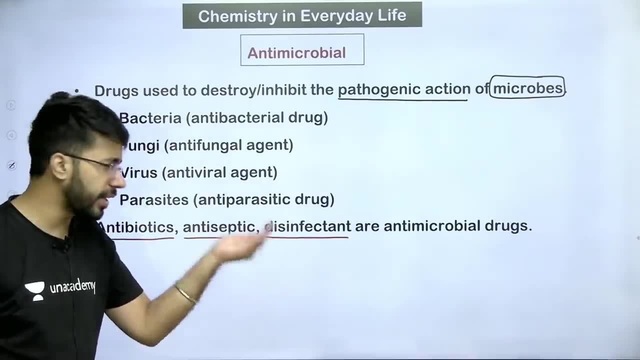 You are using antiseptic at the inside. Many times there are questions. Disinfectant also The floor on wash basis In the bathroom Where you Disinfectant means same thing. The liquid wash wim bar is your disinfectant. 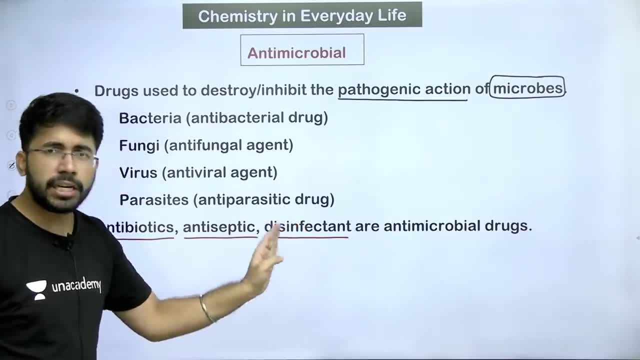 Detergent. Detergent will be in the cleaning action You have. Do you understand? disinfectant, The phenyl you use for the waxing, The one you put on non-living organisms- Non-living when you put it on floor tiles, etc. 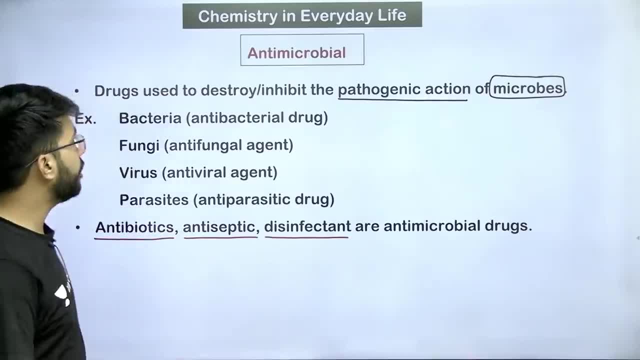 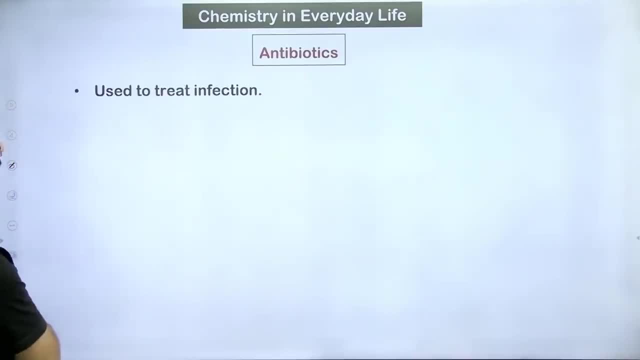 Come Antibiotic or antiseptic. Two categories: One is disinfectant, Two disinfectant, Second one is disinfectant, This one is disinfectant- Antiseptic. Two categories are given. Antibiotics are the first to be studied. 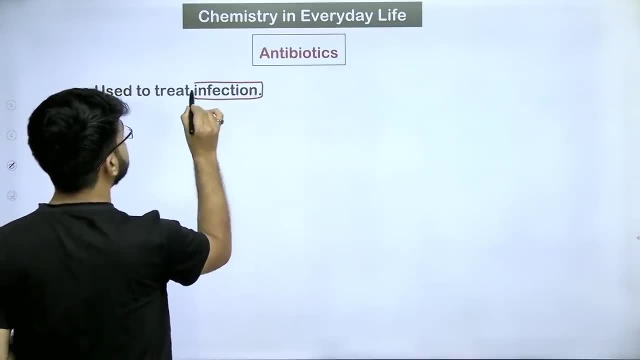 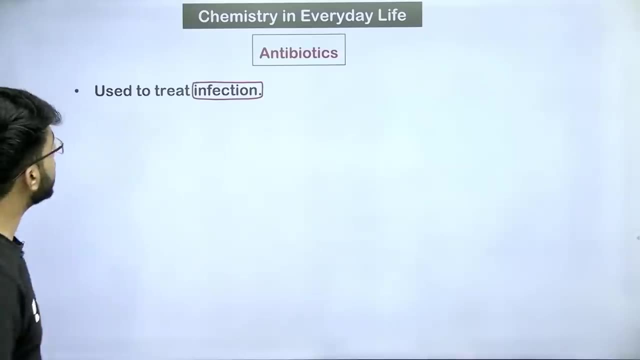 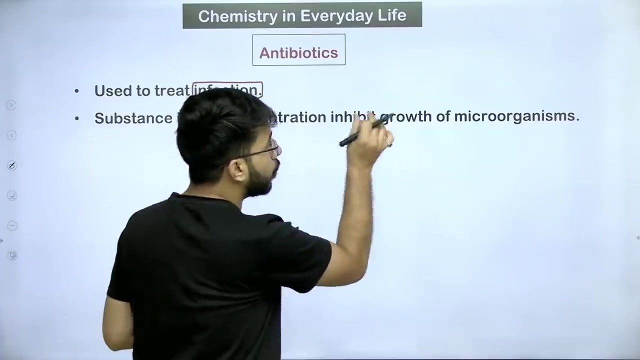 To treat this infection we give antibiotics. Any kind of infection can be there: Bacterial infection, viral infection, parasitic infection. So basically, what do we use for the infection of microorganisms? Antibiotics, Substance in low concentration inhibit growth of microorganism. 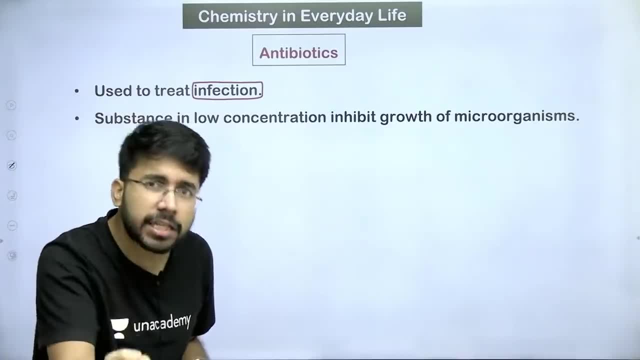 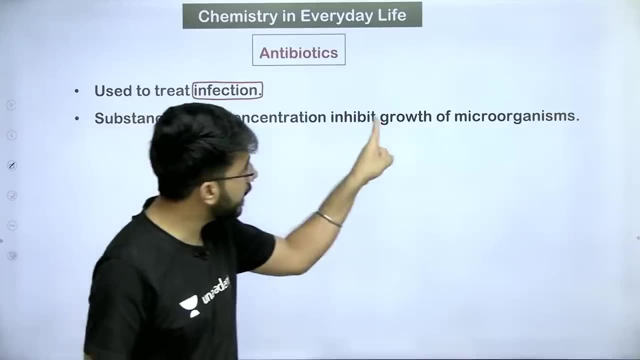 Antibiotic: what is it? Take low concentration, A substance in which micro-organism reduces growth in low concentration. Substance in low concentration inhibit growth of microorganism. So what will happen? Antibiotic Next, you will come to know what is it. 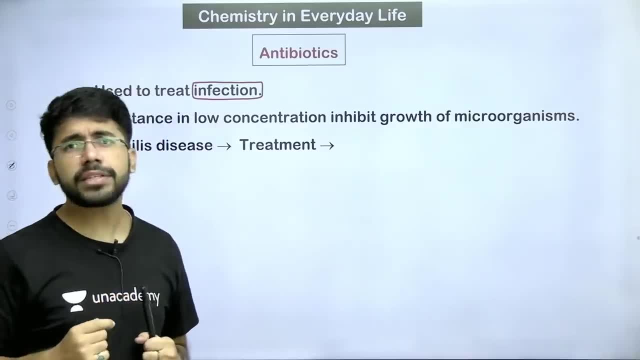 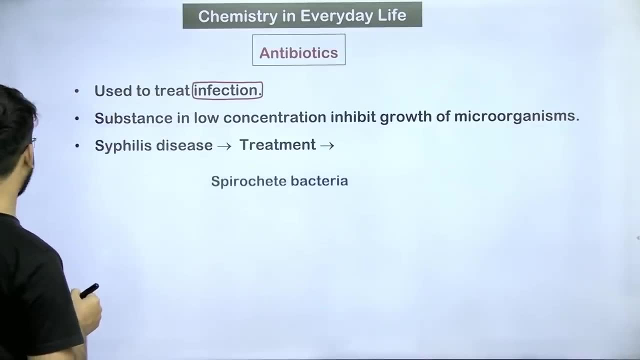 Syphilis disease. Syphilis disease, This syphilis disease is actually caused by bacteriocet bacteria And- mark this VVIP- This syphilis is syphilis disease. You must have heard, You will see syphilis. 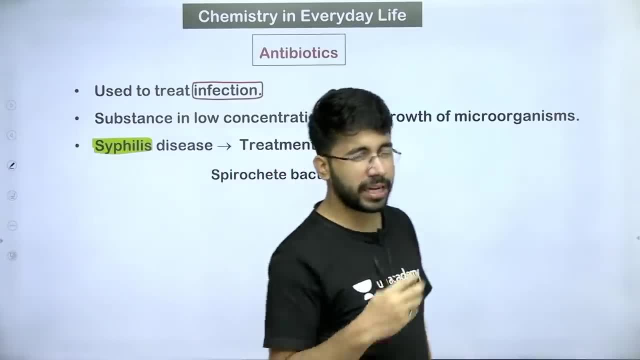 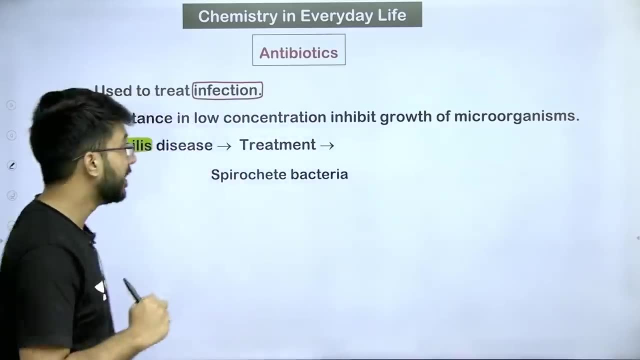 It is very strange. I searched syphilis disease on Google and went to images I was not able to see. It is very strange. Here some things happen like this. Doctors can see it. I am an engineer, Friends. syphilis disease is caused by asphyrosite bacteria. 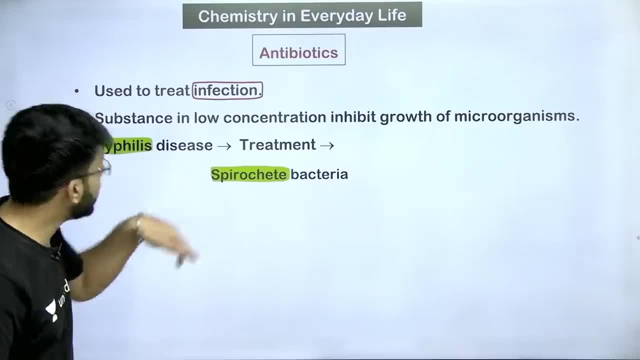 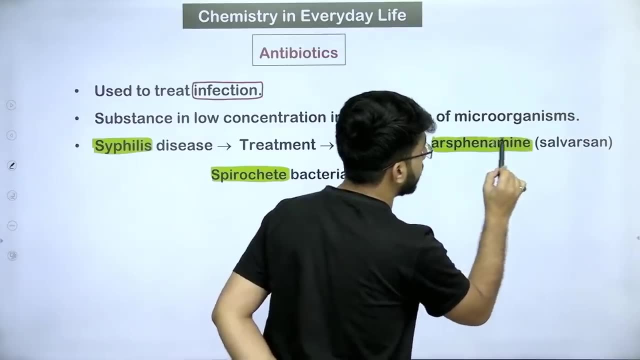 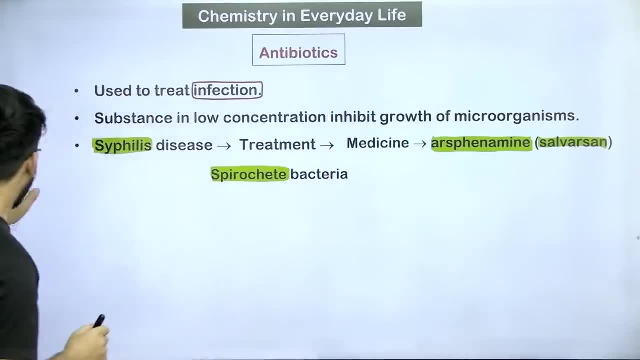 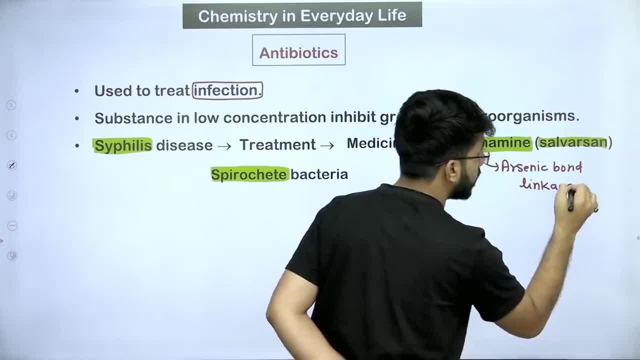 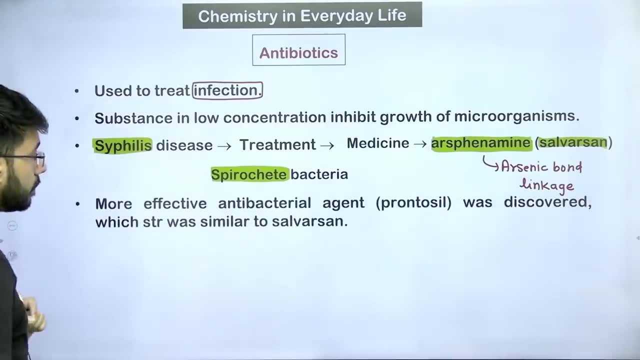 There will be linkage of arsenic bond. There will be linkage of arsenic bond In Arsphenamine. there will be linkage of arsenic bond. Next, More effective antibacterial agent, Prontosil, was discovered. Now what happens is that 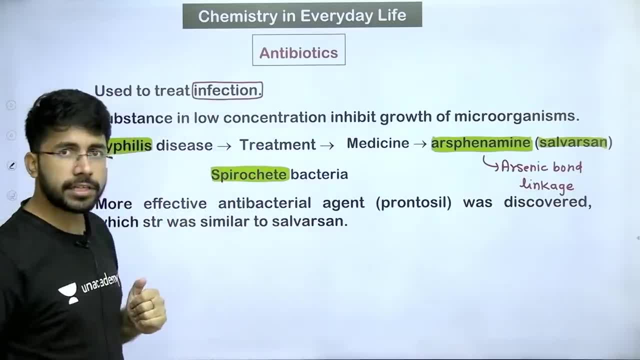 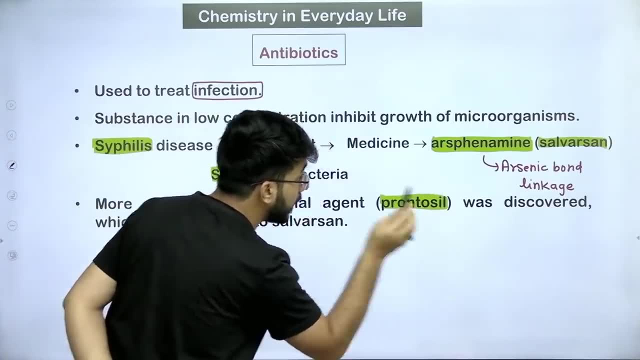 for many days. for many days they were giving Dr Salverson's medicine In it in syphilis disease you will see many times more effective antibacterial drug which is Prontosil. Prontosil was given which structure was similar to Salverson actually in Prontosil. 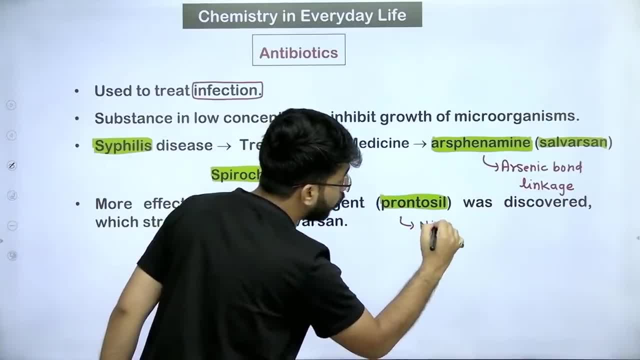 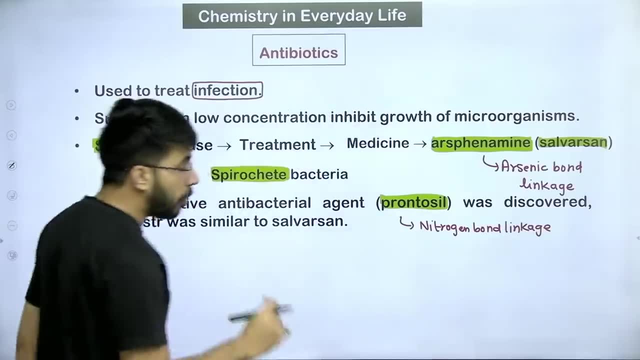 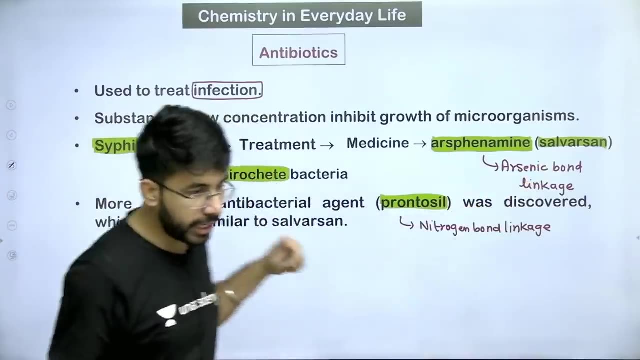 instead of arsenic bond linkage here. nitrogen bond linkage is there. nitrogen bond linkage is there instead of arsenic bond linkage? nitrogen bond linkage is there in syphilis disease, spirochete, arsferamine and salverson. is there more effective antibacterial drug? 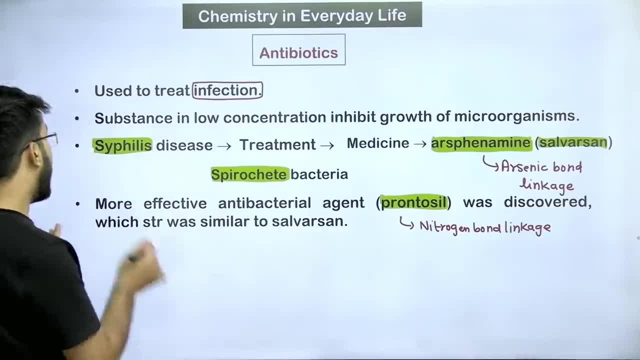 Prontosil is given in this case, in the case of syphilis, and this is VVIP. ok, VVIP, these come in the category of antibiotics. next come on discovery of sulphur drug and from. 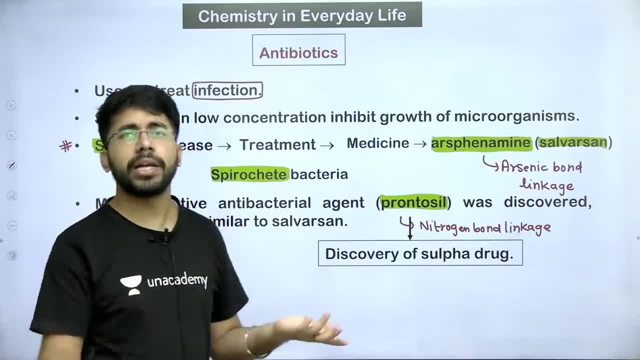 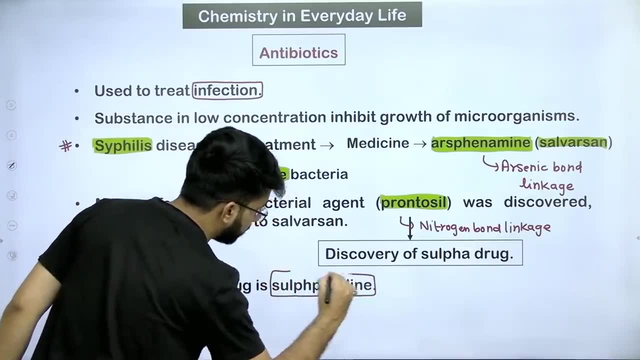 here only the discovery of sulphur drug was done. sulphur drug means drugs with double bond. S were discovered. the name of the effective sulphur drug is Sulphyridine. Sulphyridine- ok, use the name of a sulphur drug. if you tell the name of a sulphur drug, then Sulphyridine. 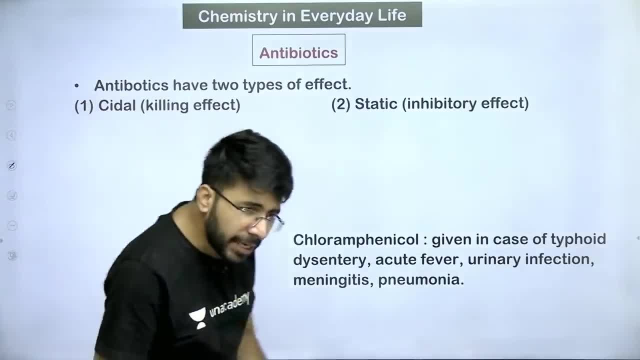 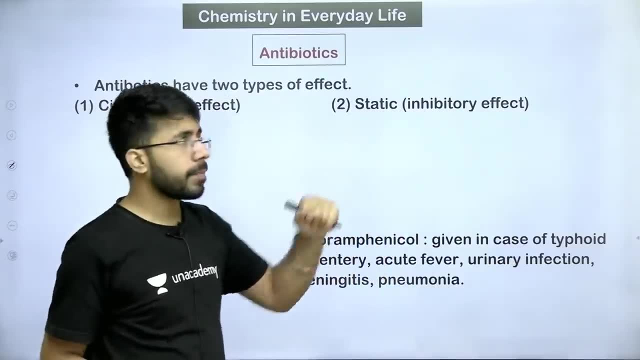 next, the antibiotic is in front of you. now let's come. antibiotics basically have two types of effects. either they kill the microorganisms or they reduce the microorganisms. those who kill, we call it a sidal effect, and those who reduce it, we call it a static effect. 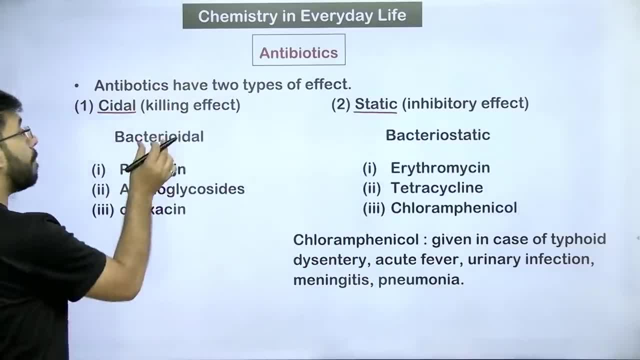 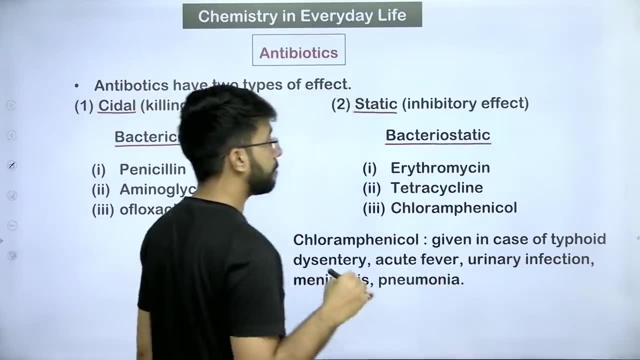 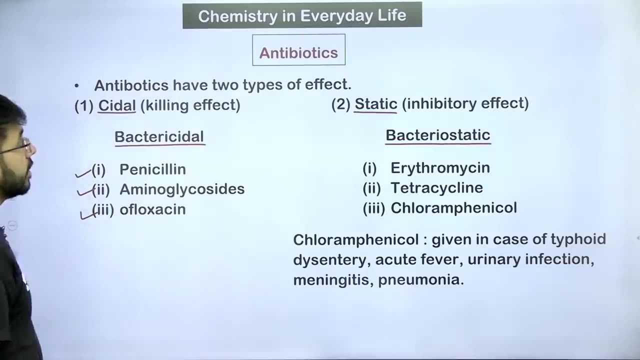 so the sidal effect is that the bacteria becomes sidal, killing the bacteria, and the static effect is that the bacteria becomes static bacteria. how does the bacteria become sidal then? only penicillin, aminoglycis and, in front of it, afloxacin, all these antibiotics that you have. 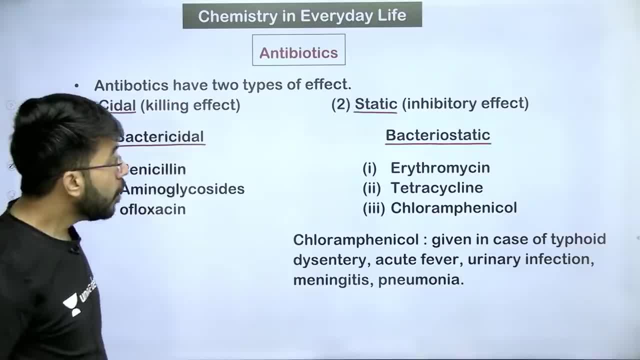 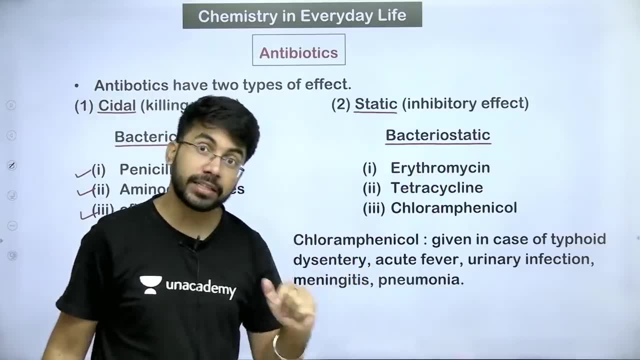 that is a sidal effect. it kills the bacteria directly, like erythromycin. if you have gone through covid then you will remember erythromycin. what does erythromycin do? it reduces it. it is an inhibitory effect of it. that means it will reduce the bacteria. 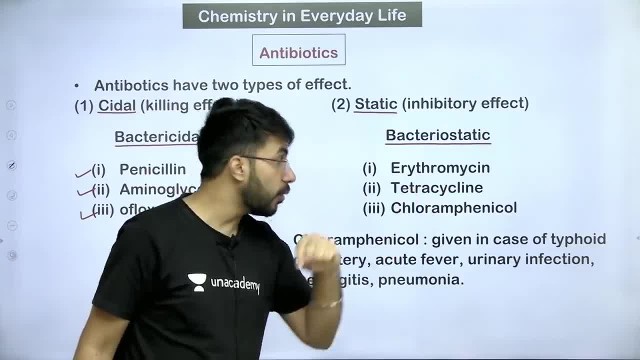 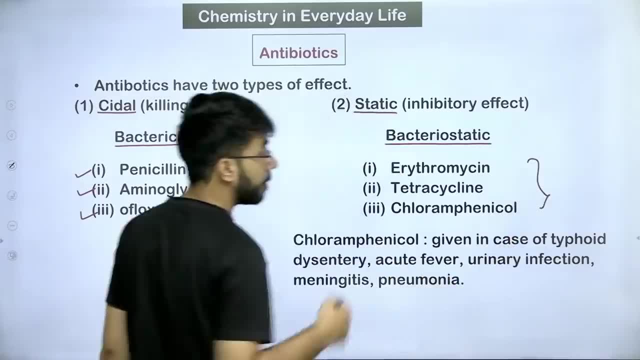 tetracycline- this has also been used in many rural areas- chloramphenicol- these all are bacteriostatic effects. what they do? they reduce the effect of bacteria and they will kill all the effects of bacteria. okay, so there is a lot of fear in giving it. 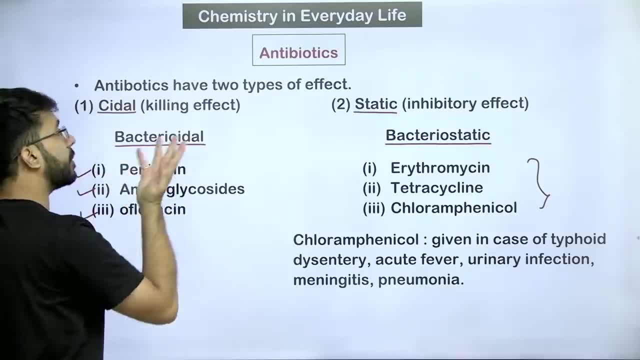 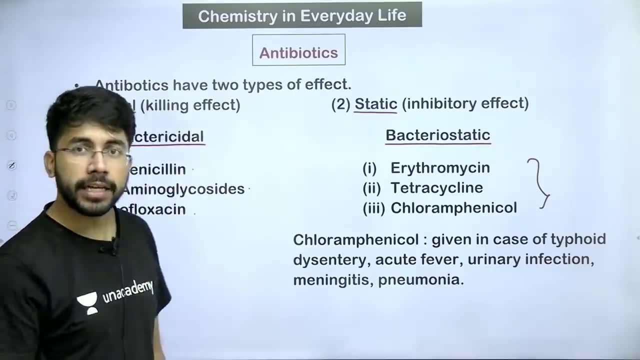 do you know why? because what happens is that many useful will also die from it. many bacteria will also die, useful for you. so penicillin, aminoglycosides and, in front of you, afloxacin, what are these? these are sidal effects, bactericidal and bacteriostatic. 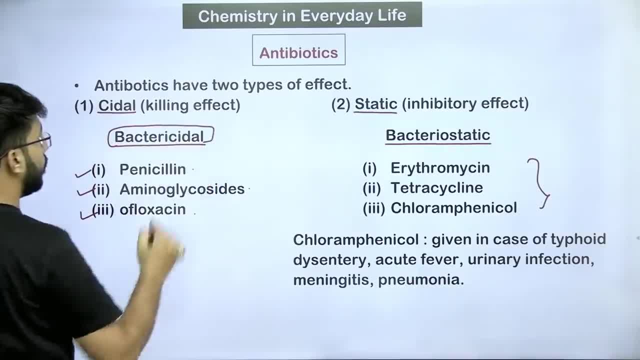 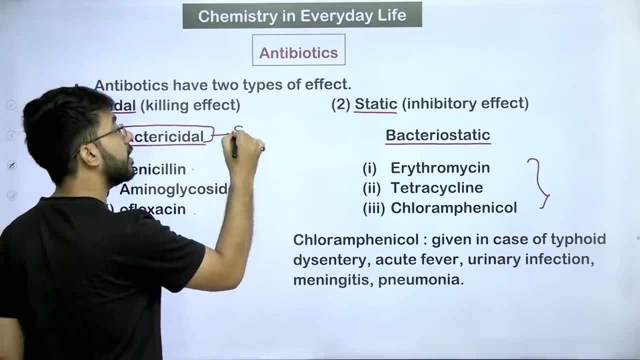 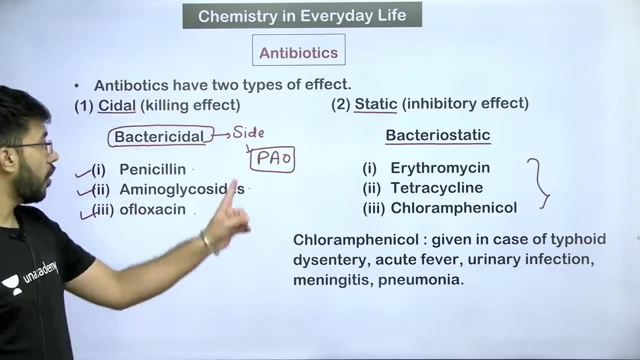 again, son, give side. what does it mean here? sidal means the side is coming. in the roadside there is a shop of pav bhaji, very beautiful, in the roadside. sidal means the side is coming. side means friend, you have the mind of pav bhaji, pav bhaji shop. P for penicillin, A for aminoglycoside. 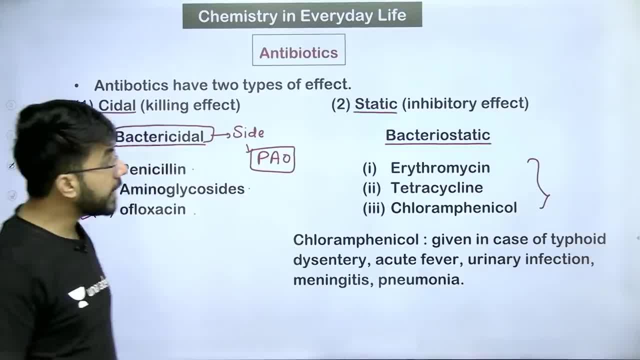 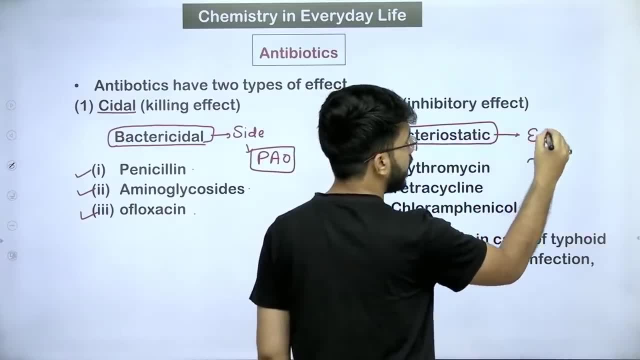 and O for afloxacin: okay, bacteriostatic. bacteriostatic, here you have to keep in mind, like there, remember, from pav pav bhaji shop. here you have to keep in mind, etc. etc. E for erythromycin: 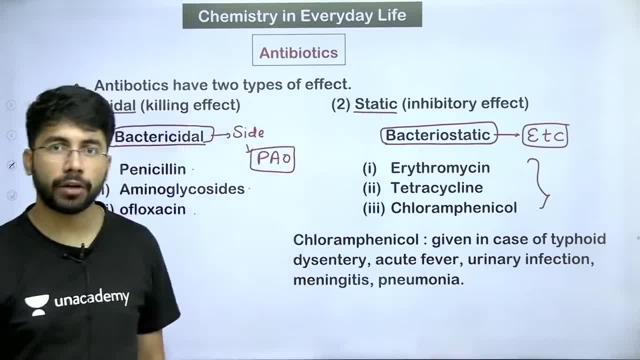 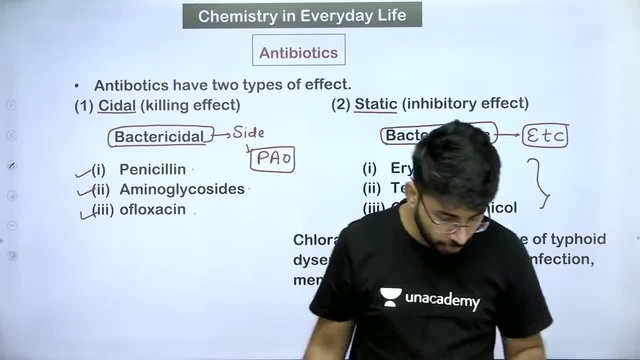 T for tetracycline and C for chloramfenicol, and these three medicines have been used a lot in covid. in fact, first and third have been used a lot. okay, you must have read the first one in the paper. 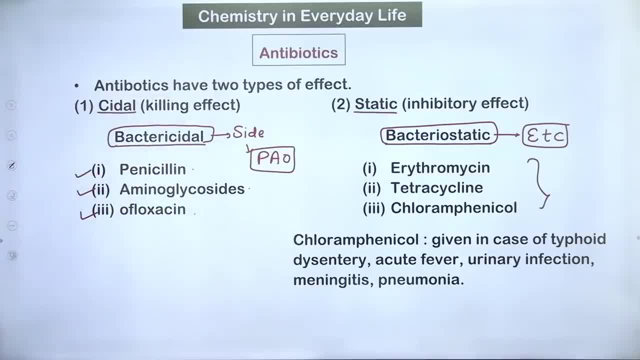 chloramfenicol, etc. sorry, erythromycin, etc. okay, where do we give chloramfenicol? so, friends, when typhoid happens to you, at that time chloramfenicol medicine will be written. it will be written. 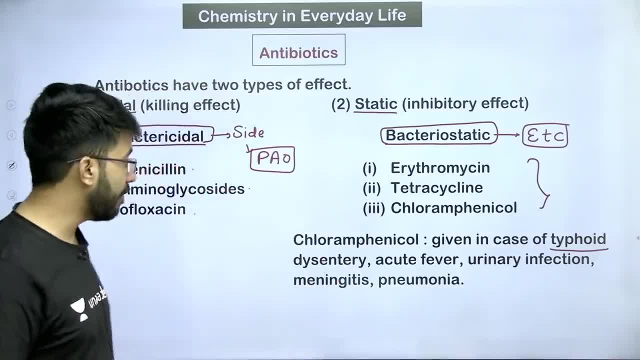 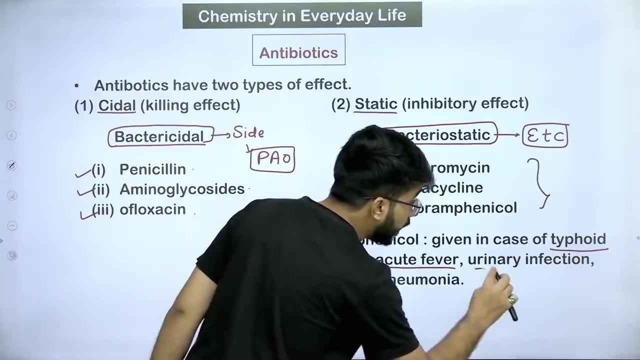 so take that of a small typhoid. look at the prescription there: chloramfenicol. you are given a time for dysentery. you will also be given in small fevers. you will also be given in urinary infection. meningitis will also be given to you and pneumonia will also be given. then a single medicine. 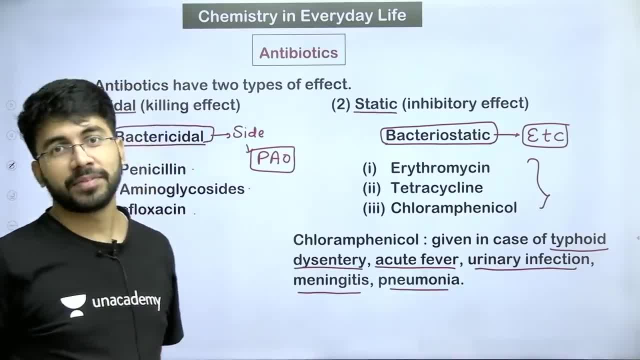 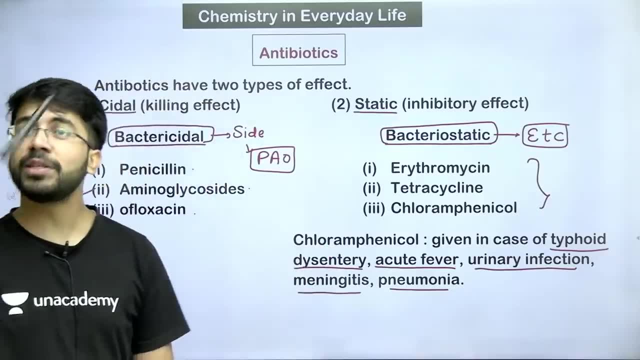 is the cure for so many diseases- chloramfenicol, okay. typhoid happened, meningitis happened, urinary infection happened, pneumonia happened, acute fever happened, dysentery happened. should I start teaching biology? There is nothing wrong in biology, but I can try this way. 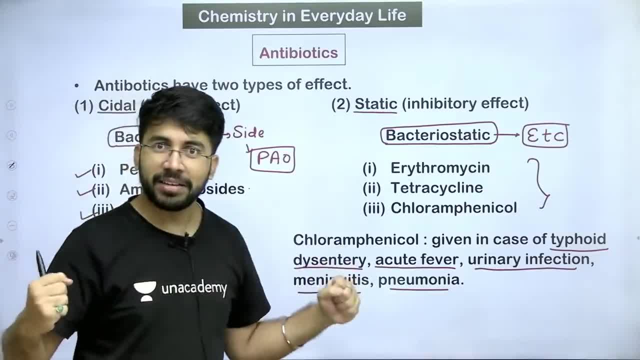 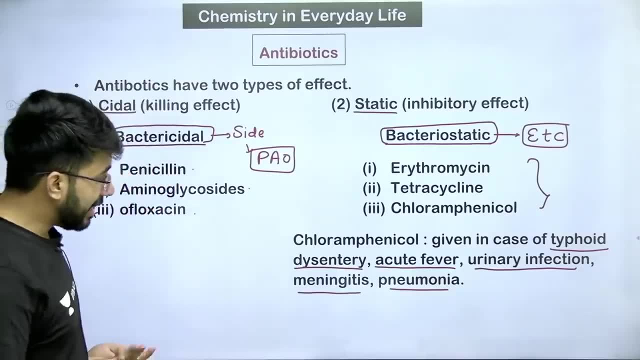 It feels good, It feels like a little attitude. I am telling the name of the medicine. I am a doctor. There is a different attitude. I think it happens in doctors. It will happen in you too. in a few days, Half of the attitude will come in you. 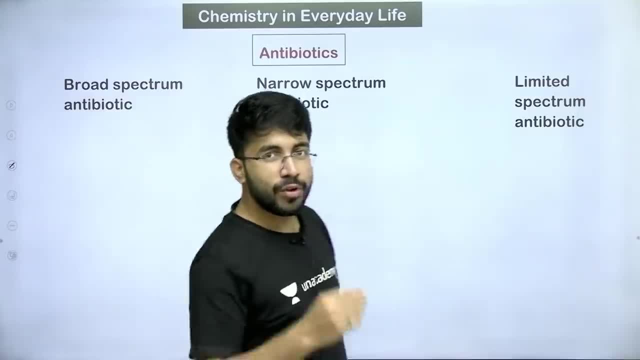 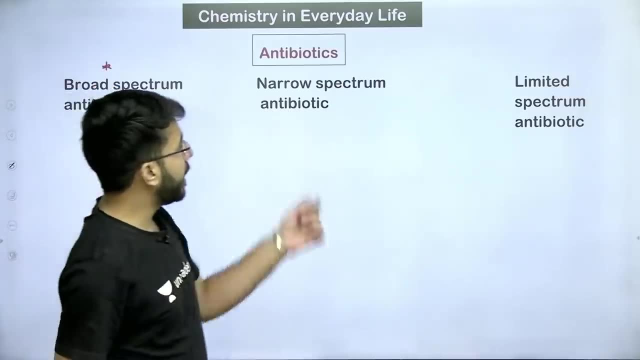 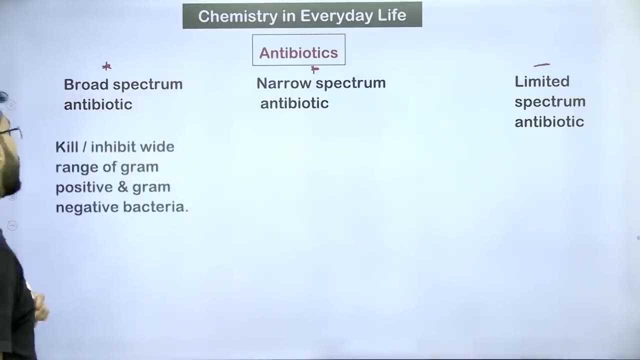 It will be complete in a few days. Antibiotics are of three types. Broad spectrum antibiotic is asked in PYQ. Narrow spectrum antibiotic is asked in PYQ. Limited spectrum antibiotic is not asked in PYQ. What is broad spectrum If it kills a wide range of bacteria? 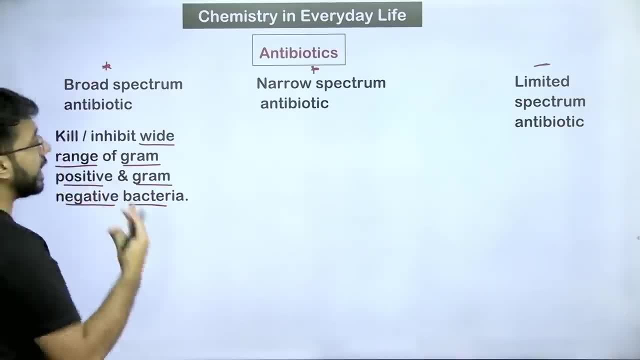 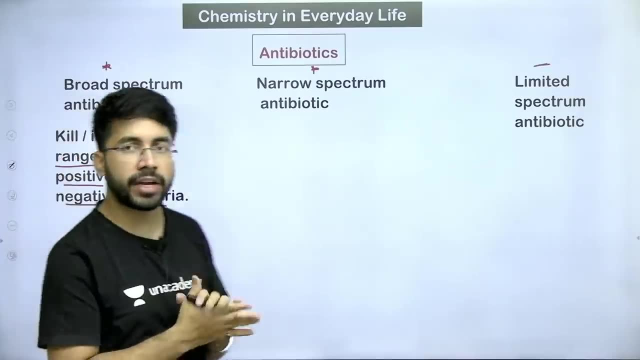 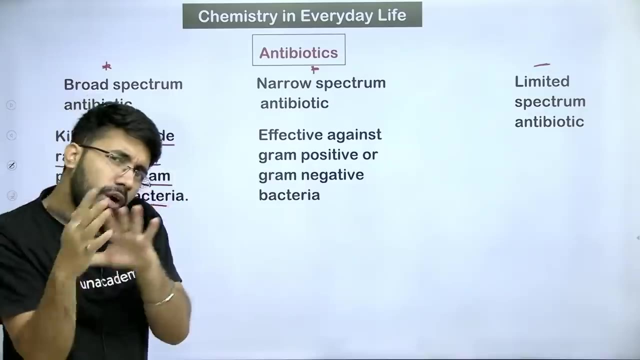 If it kills gram positive and gram negative bacteria, What will happen in front of you? Kill or inhibit wide range of gram positive and gram negative bacteria. Ok, Now comes narrow spectrum antibiotic. What happens in narrow spectrum? Either gram positive or gram negative. 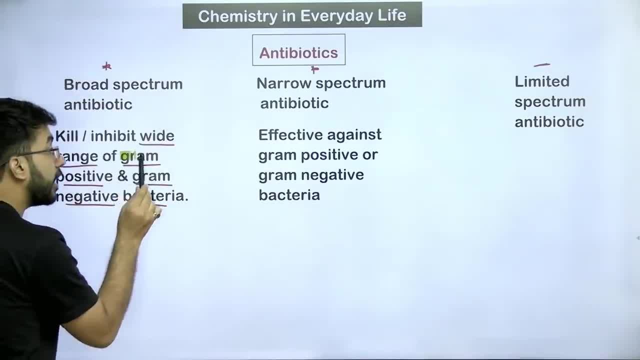 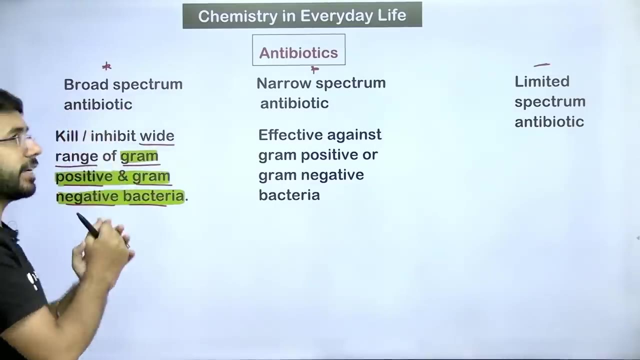 What was there? Look carefully. Gram positive and gram negative works great on both the bacteria. What does it do to both the bacteria? Will it inhibit or kill Gram positive and gram negative bacteria of both the types? What are gram positive and gram negative bacteria? 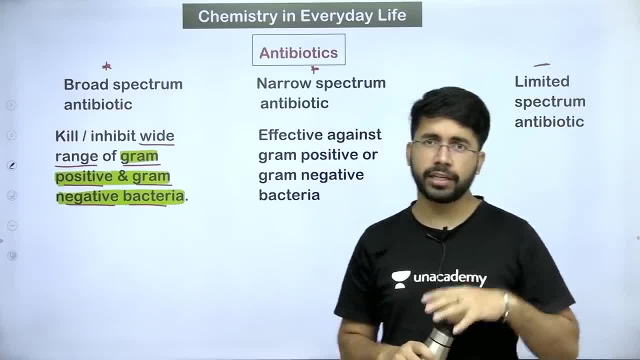 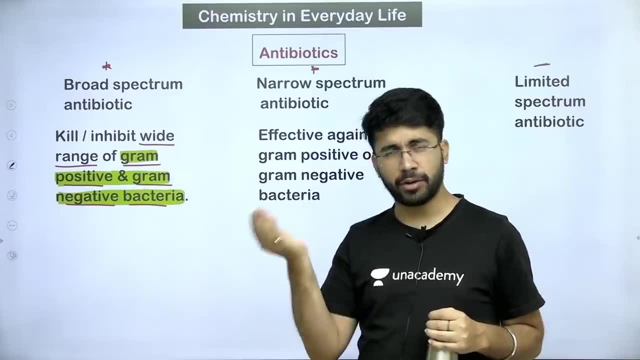 You must have read it. It is mentioned in your biology. I give you a small one. Gram positive bacteria is one of the single layered bacteria and one of the multi layered bacteria. I have also done Google. I don't have much idea about it. 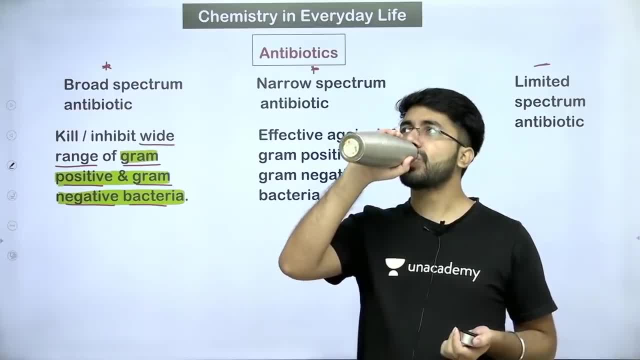 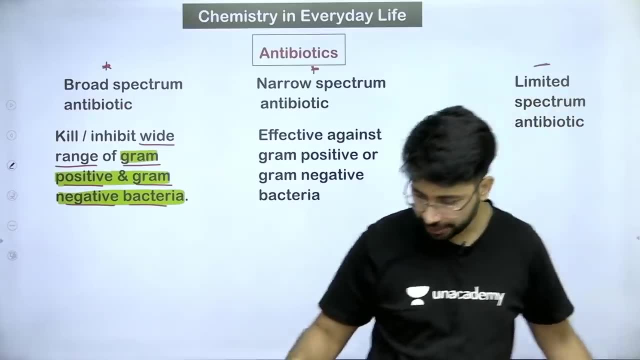 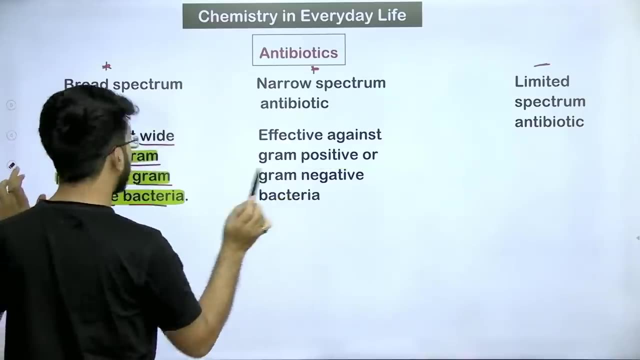 But I don't have that much information in NCIT, So your NCIT is not out of this chapter. You don't have to do much mastery in it. Come on, What is there in narrow spectrum? Yatogram-positive and Yatogram-negative. 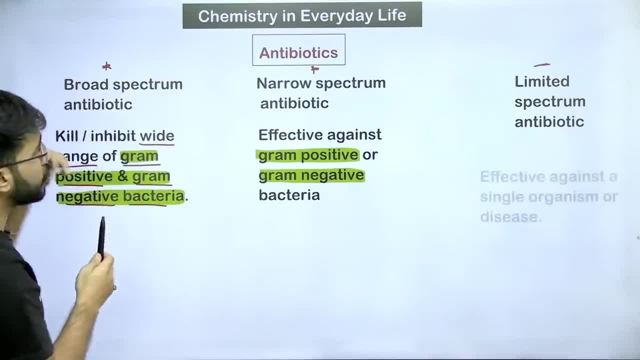 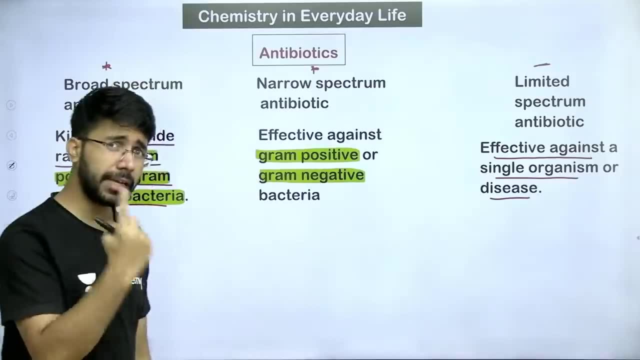 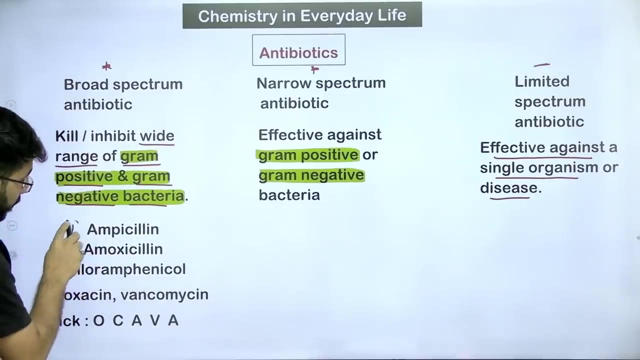 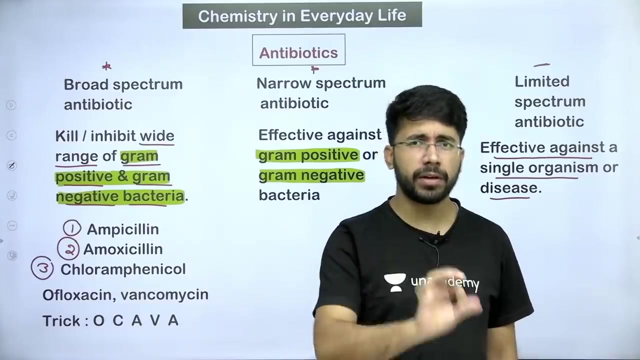 So it is narrow now. It is effective only for a single organism or a disease: Ampicillin, Amoxicillin, Chloramfenicol, Typhoid, Dysentery, Meningitis, Acute Fever, Unitary Infection. 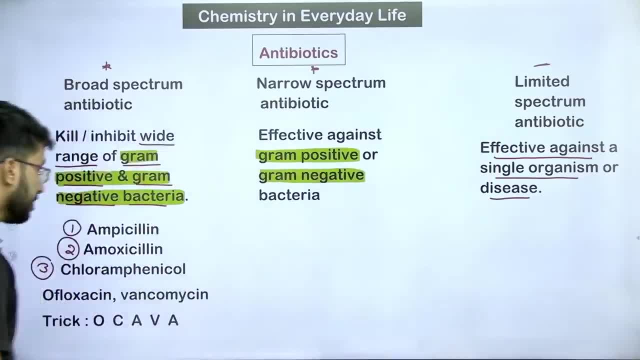 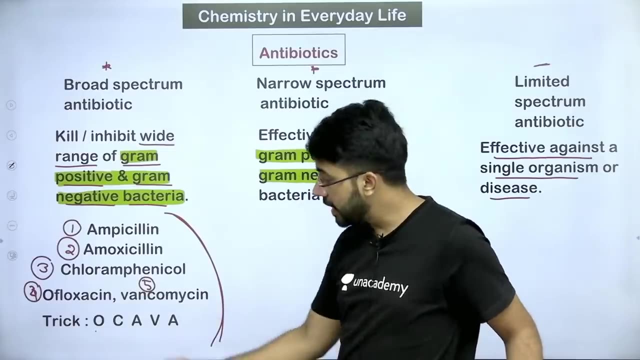 Afloxacin and Vancomycin. These are very important. These are VVIP. These are VVIP. Don't miss it. Look at its title: It is Okava. Okava means Afloxacin, C means Chloramfenicol. 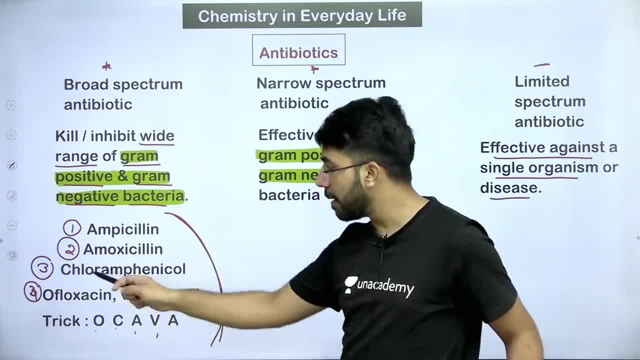 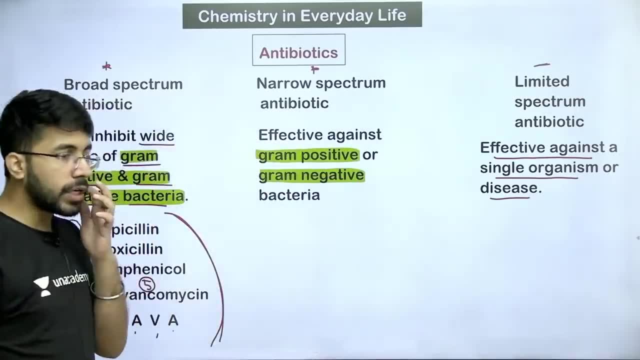 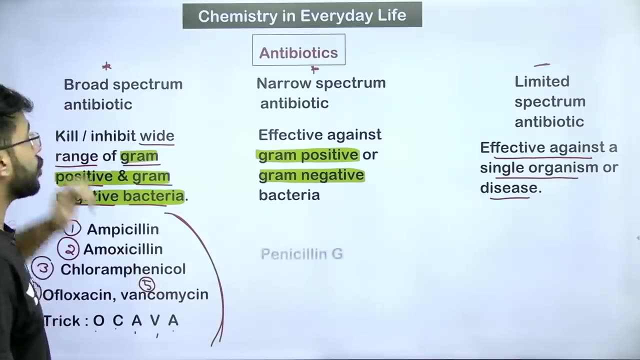 A means Ampicillin, V means Vancomycin And again A is Amoxicillin. Okava will come in front of you. That is Broad Spectrum Antibiotic. Okava is Broad Spectrum Antibiotic. Now let's come to Narrow Spectrum Antibiotic. 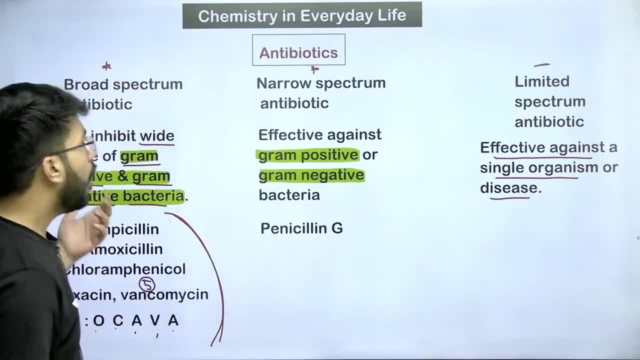 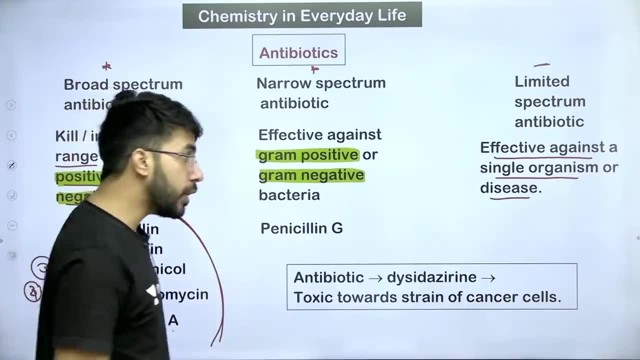 Penicillin G, The derivative of Penicillin, Penicillin G, And there is no drug of Limited Spectrum. That is why there are no questions. Next come in front of you. Antibiotic is one which is used in the treatment of Cancer Cells. 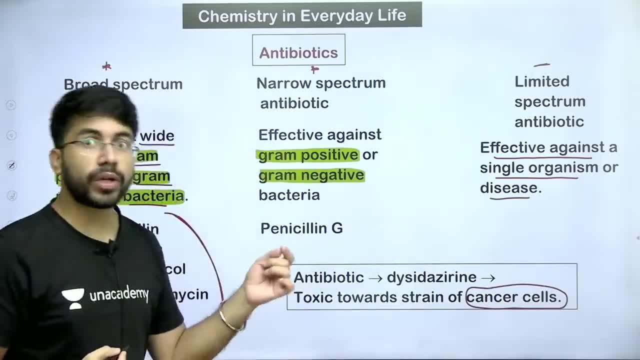 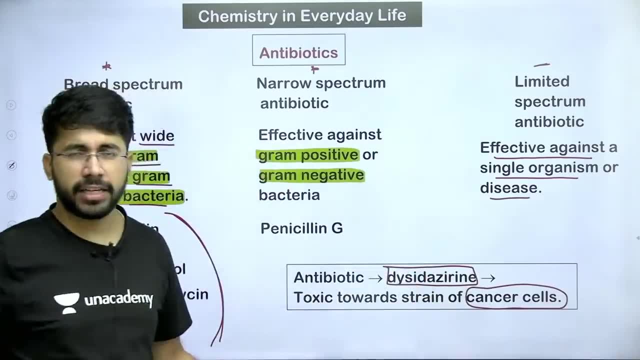 Again, since we are talking about Cancer, it becomes important That is Dicidazirine- Dicidazirine or Dicidazirine, Ok, Dicidazirine is used in Cancer Cells And this thing 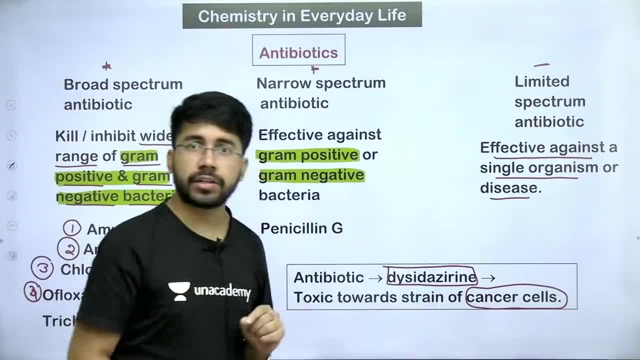 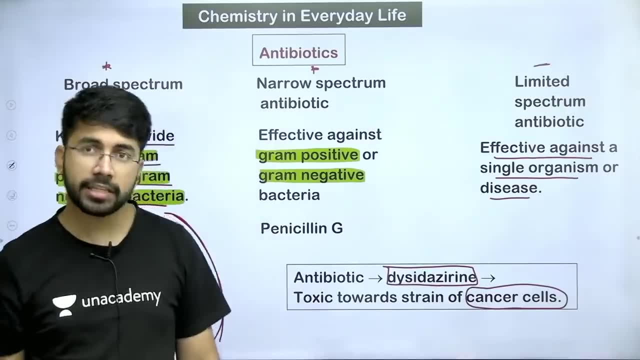 Toxic towards Strain of Cancer. It is dangerous for the Strain of Cancer Cells. So when Cancer Cells are produced in your body, So this is given: Dicidazirine, Ok, Dicidazirine. 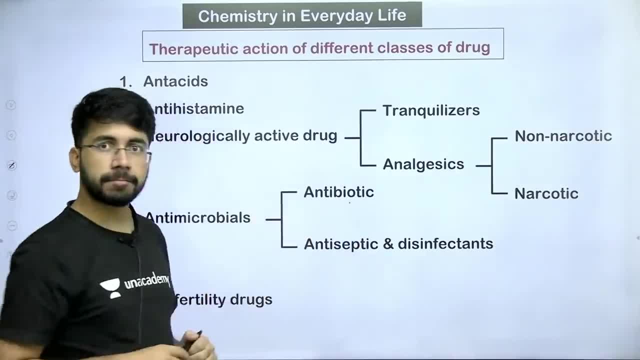 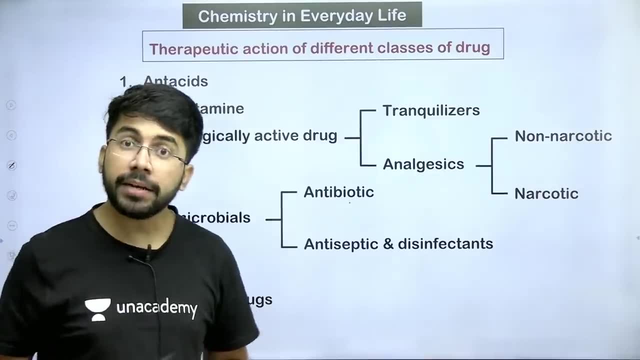 Next. Now you have read the Antibiotic in front of you. Okava is a very good one. We have also read in that: Ok, Now is Antiseptic and Disinfectant. Have you seen Antiseptic Dettol and Cevlon. 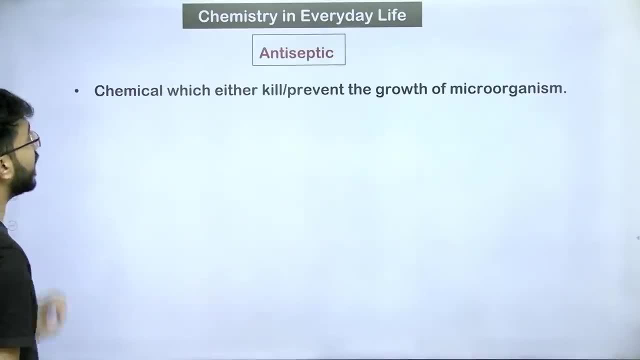 Bunty is your soap slow. That is the same. Antiseptic, my friends. Come here. Chemicals which either kill or prevent growth of microorganism. Ok, Come, I will tell you What is Antiseptic. We apply it on Living Tissues. 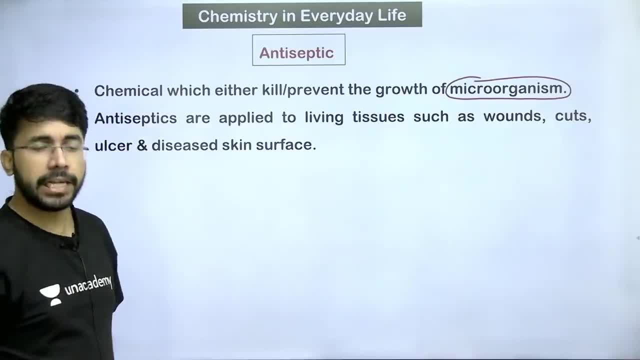 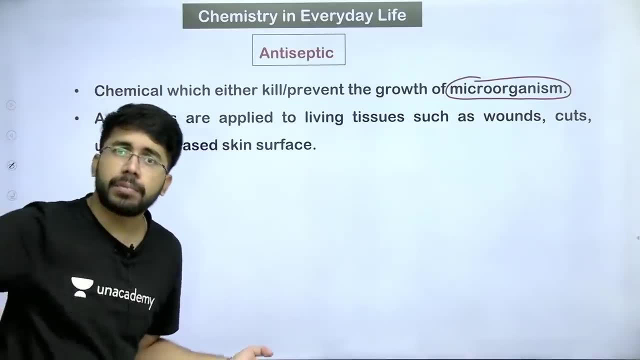 And we apply Disinfectant on Non-Living Tissues. Disinfectant is used in Basin Floor For Washing, For Cleaning Bathroom, For Cleaning Mirror- So many things. you use Disinfectant Which is used on Non-Living. 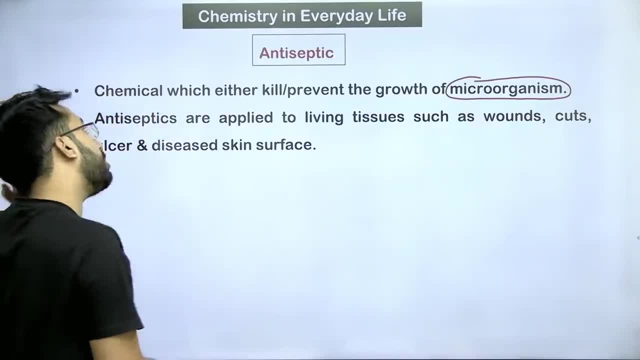 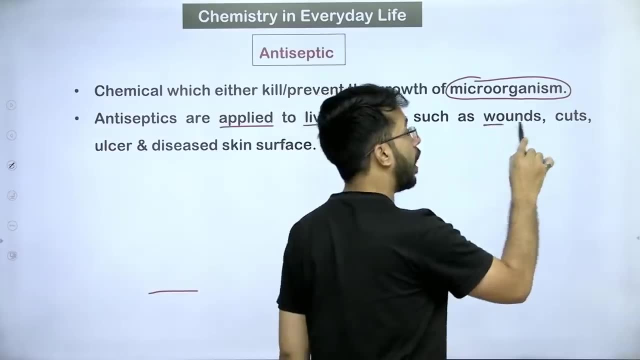 But Antiseptic Dettol and Cevlon- you use it yourself, So Antiseptic are applied to Living Tissues, Such as Where you have got wound, Where you have got cut, Where you have got Ulcer. 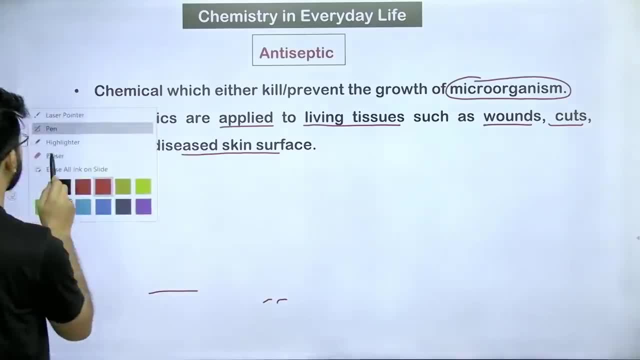 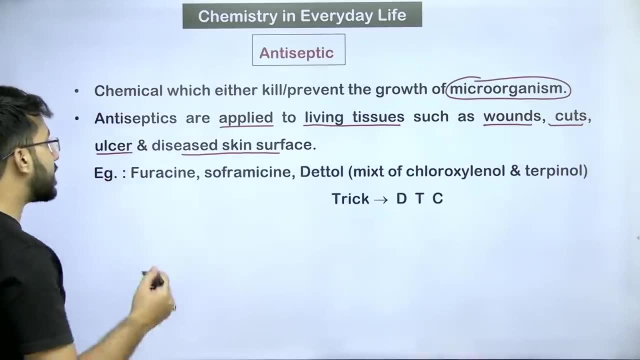 Where you have got Dizziness, Skin Surface Means. many times you have got Fungus, So we use it there also. Ok. Next is my friends As an example, Antiseptic example, Furacil Sulfuramycin. 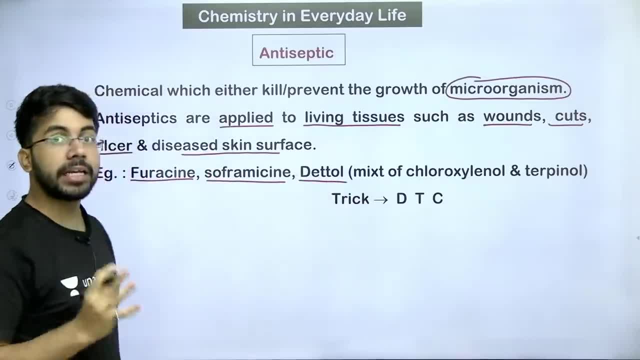 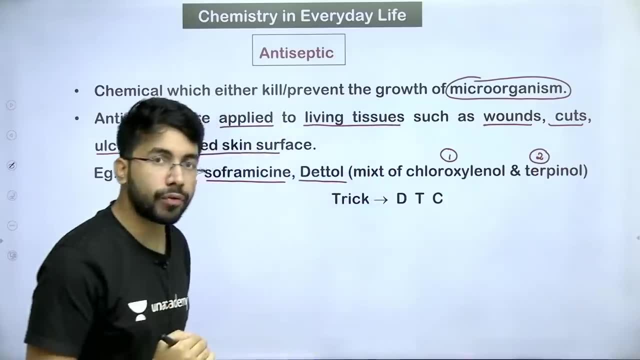 And Dettol, And how many times we have been asked about Dettol. What is Dettol? Mixture of Chloroxylenol and Terpenol. Mixture of Chloroxylenol and Terpenol DTC. 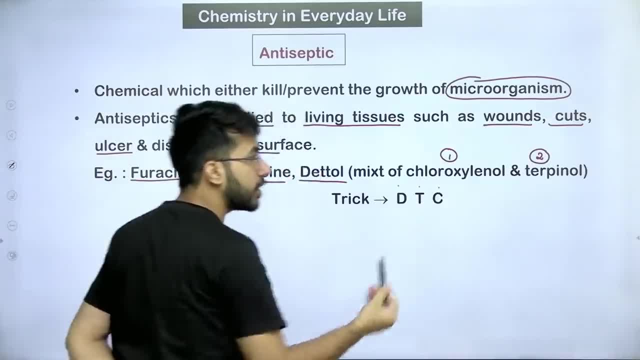 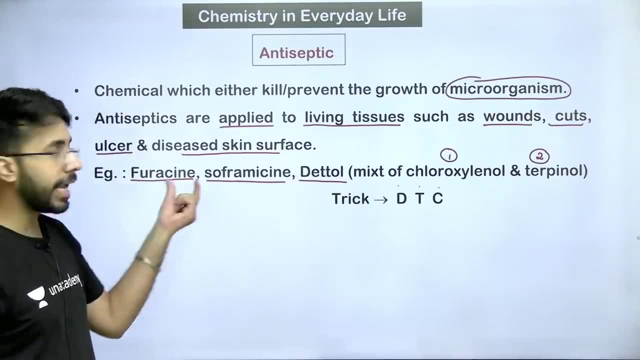 Dettol has mixture of Terpenol and Chloroxylenol. DTC Dettol is a mixture of Chloroxylenol and Terpenol And along with that Sulfuramycin and Furacil. These are: 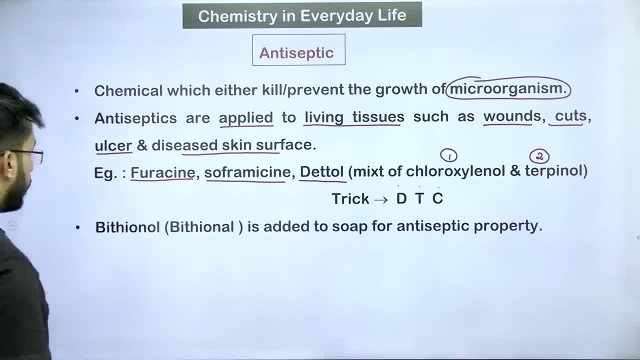 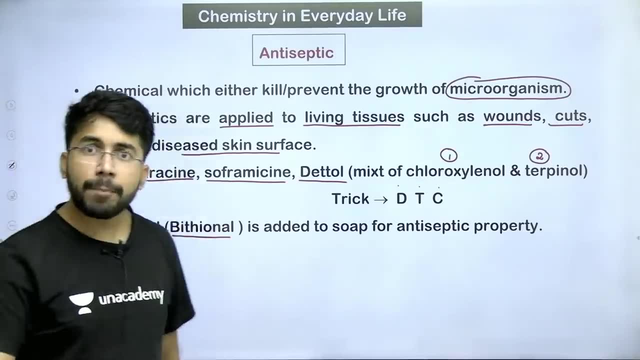 What These are Antiseptic. Now, Bithionol One is there. Either it is called Bithionol Or sometimes it is called Bithionol, Like in your soap. It kills 99% germs. 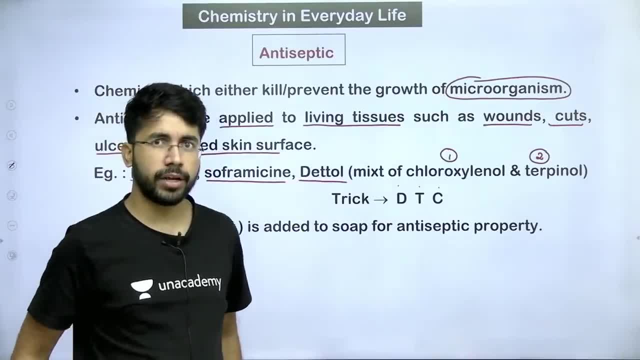 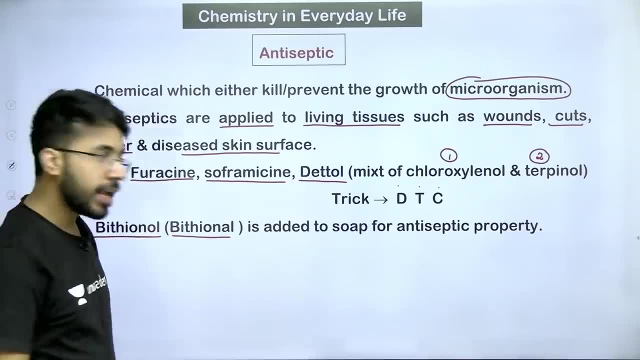 So it is a microorganism. Germs are microorganisms, So 99% is killed. How is that So, friends? in our soap We use Bithionol. In our soap, friends, We use Bithionol. 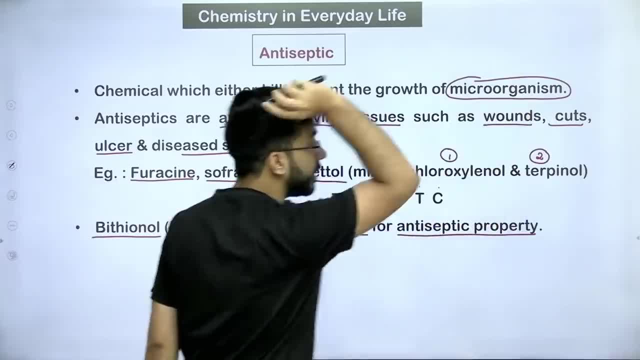 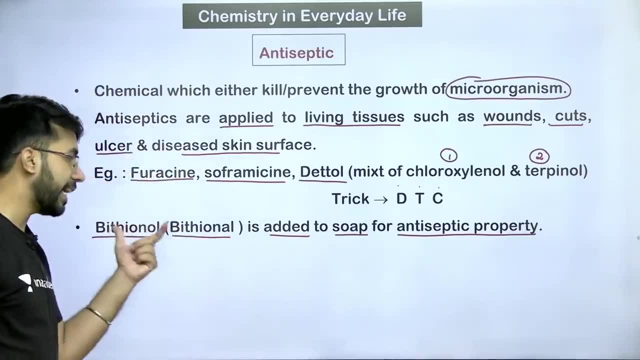 Because of which It has antiseptic properties, Because of which 99%, 99.99% of germs are killed, Right. So, whenever you see an ad, It should come in your mind That Bithionol or Bithionol 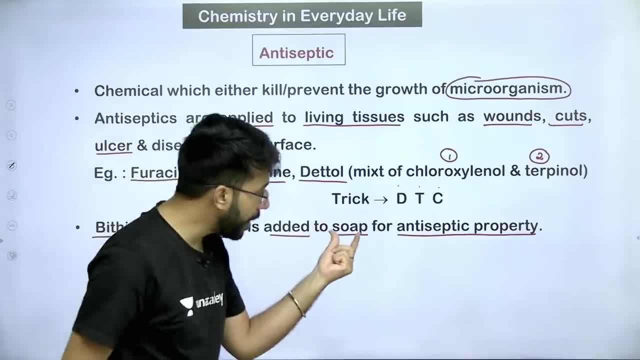 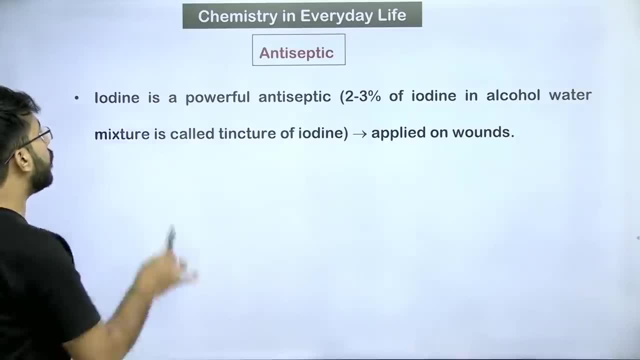 Both are the same. We add them in the soap For antiseptic properties, Right. Next, let's come in front of you. Iodine is a powerful antiseptic. PYQ has been asked. Iodine is a powerful insecticide. Sorry, it is antiseptic. 2-3% iodine in alcohol. 2-3% of iodine in alcohol water is called tincture of iodine and it is applied on wounds. 2-3% of iodine in alcohol water is called tincture of iodine and it is applied on wounds. 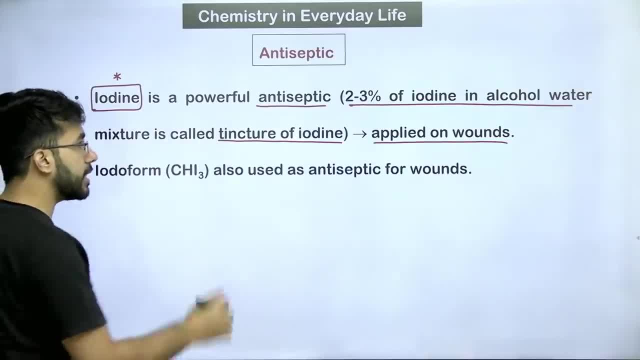 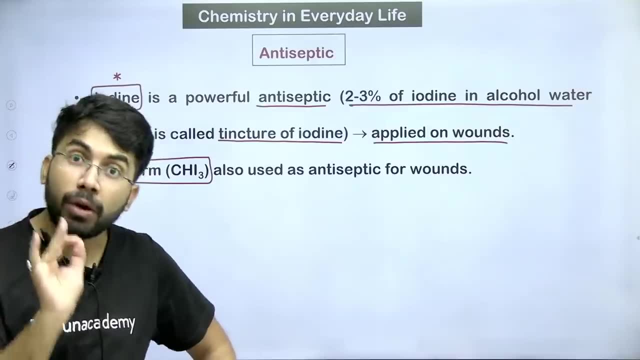 My friends come next. after iodine, Iodofoam is antiseptic for wounds Also. you have Iodofoam Antiseptic for wounds, But Iodofoam is also antiseptic for wounds. Chloroform is a medicine to make you unconscious. 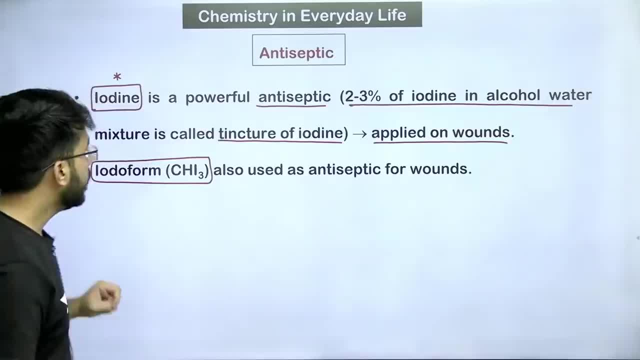 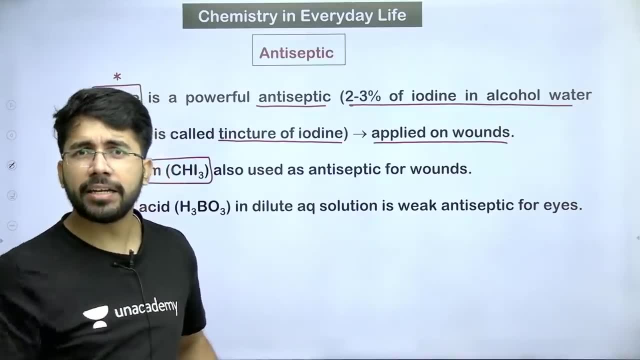 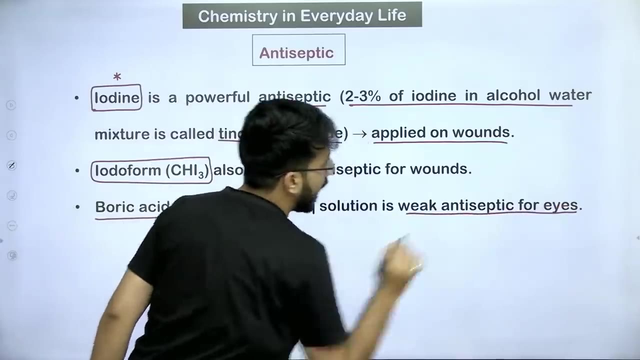 Iodoform is an antiseptic. Next, The eye cleaners that you get, The very mild eye cleaners, The eye drops that you get. It contains boric acid in front of you, So boric acid works as a weak antiseptic for eyes. 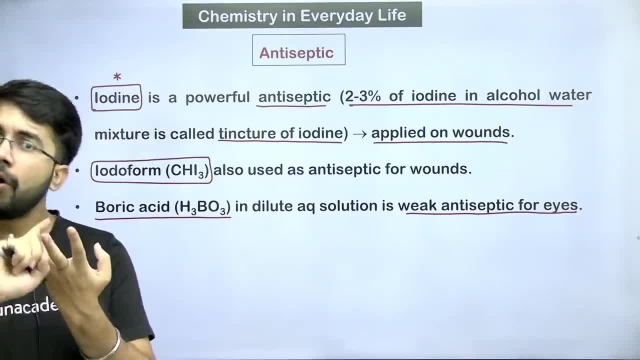 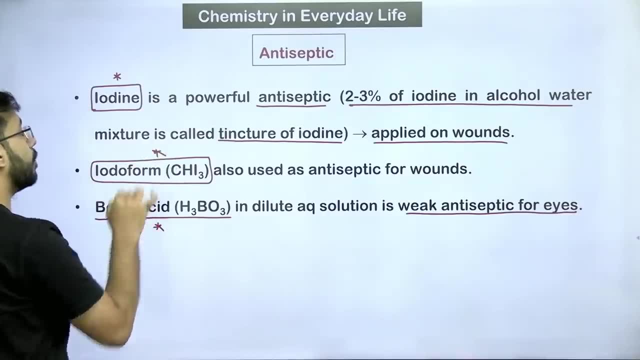 So what came in front of you? Iodine came, Iodoform came And boric acid came in front of you. These all work as antiseptic. This is the antiseptic for eyes. PYQ- This is also a PYQ. 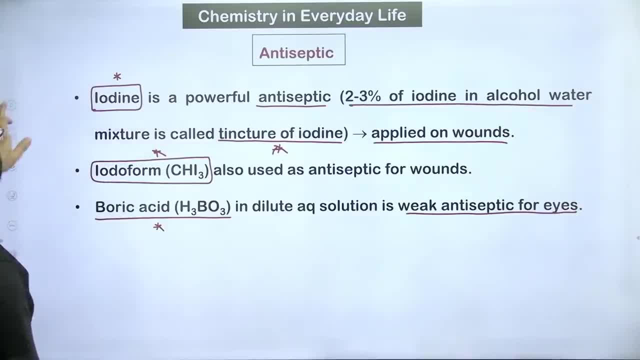 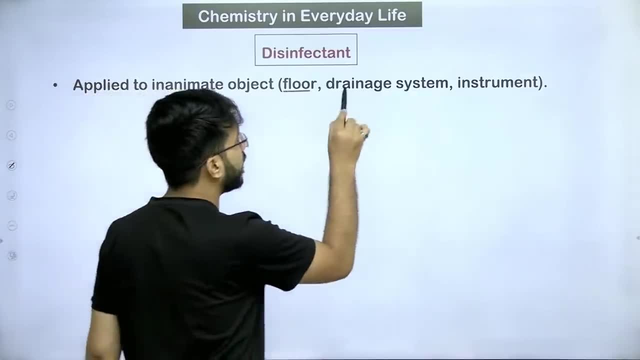 This is also a PYQ. Next, Let's come to disinfectant. Disinfectant in inanimate objects: We use it for non-living On floor, In drainage system. In instruments: We use it for sterilization. 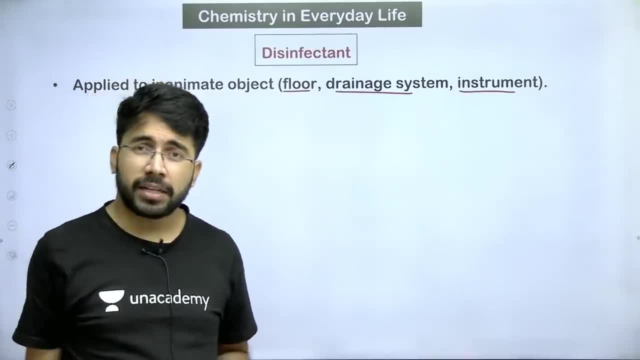 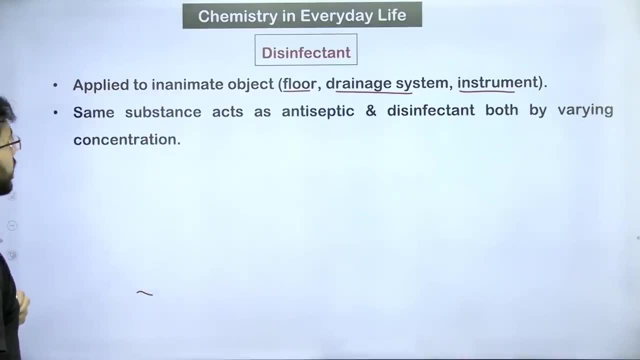 For doctors. You use Harpic, You use floor cleaners, Cleanmate- I don't know what comes. So these all are disinfectants In inanimate objects. We use it for sterilization. Same substance can be used as antiseptic. 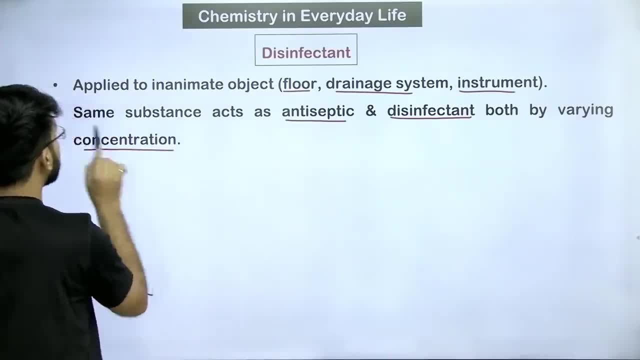 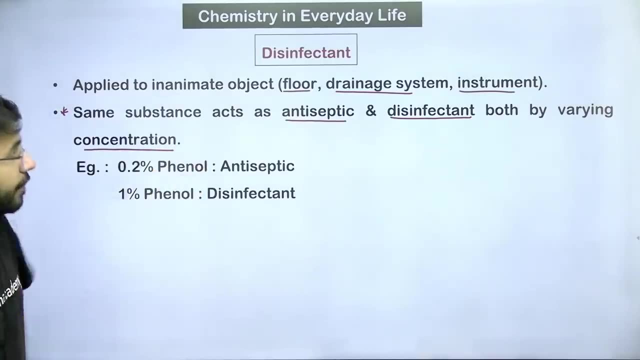 And disinfectant can also be used By varying concentration. PYQ: Same substance can be used as antiseptic And disinfectant can also be used in front of you, Like if phenol takes 0.2% concentration, Then it is antiseptic. 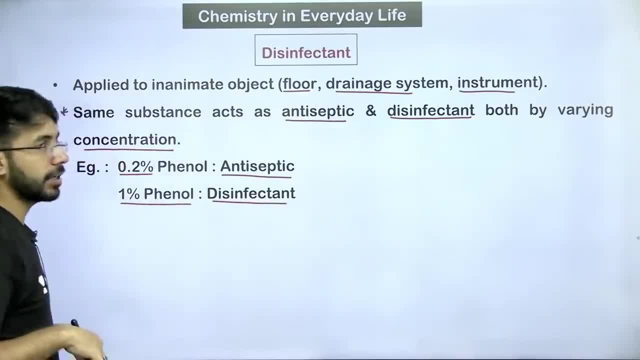 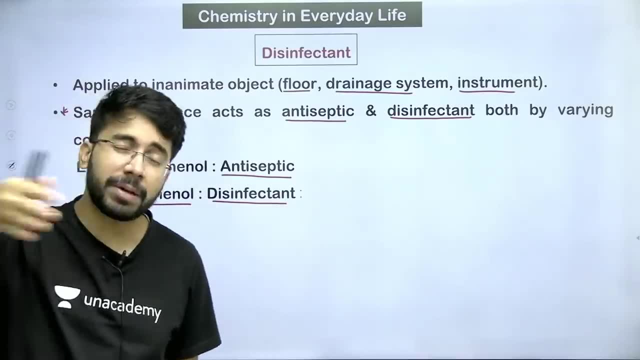 But if you take 1% phenol, Then it works as disinfectant- The phenyl that you use In it. Read the integrants. This is also 1% phenol, And there are many other chemicals, But 1% phenol is used in it. 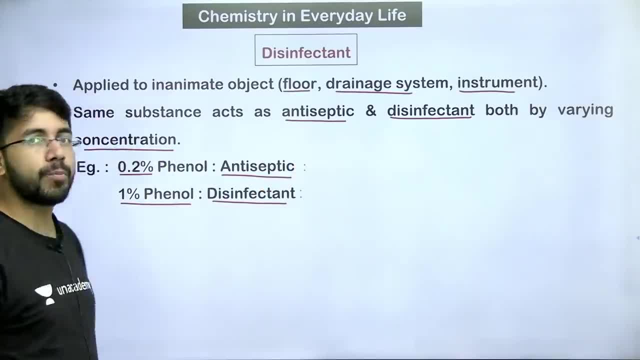 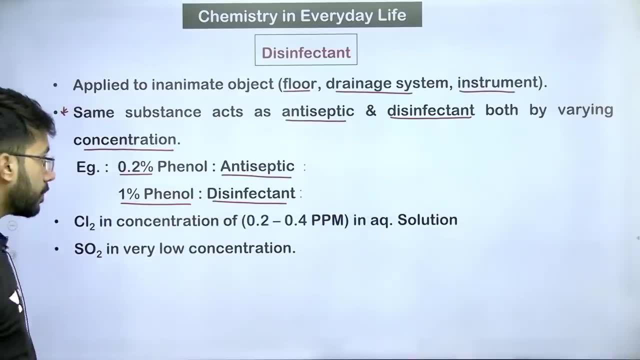 And friends, If you will study in antiseptic Dettol, Then you will also get 0.2% phenol, Savlon and Dettol. You will study in all of them. You will get it Next Now, PYQ. 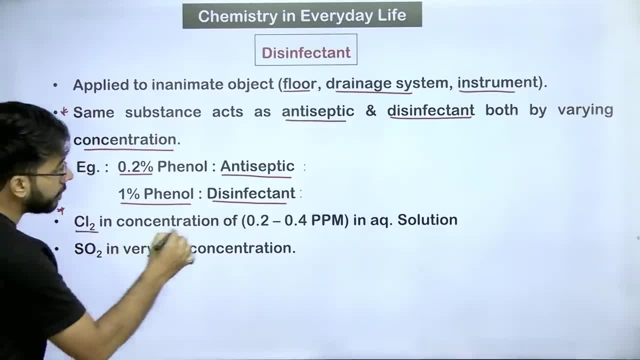 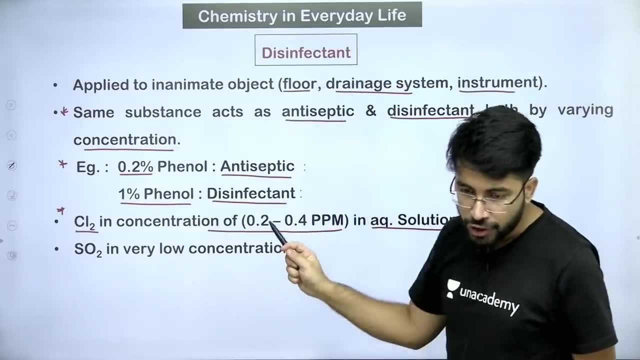 This is also your PYQ. This is also your PYQ TL2 in concentration of this much In aqueous solution. It is also a disinfectant. Chlorine is 0.2 to 0.4 ppm In aqueous solution. 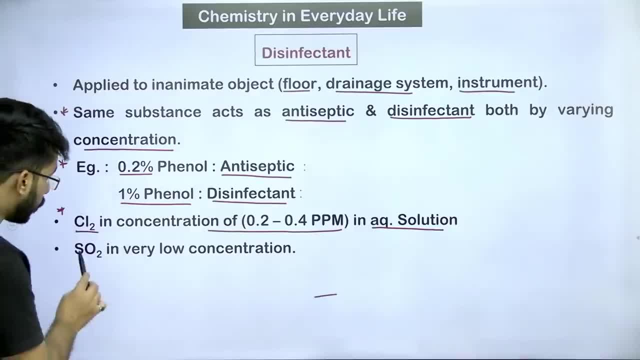 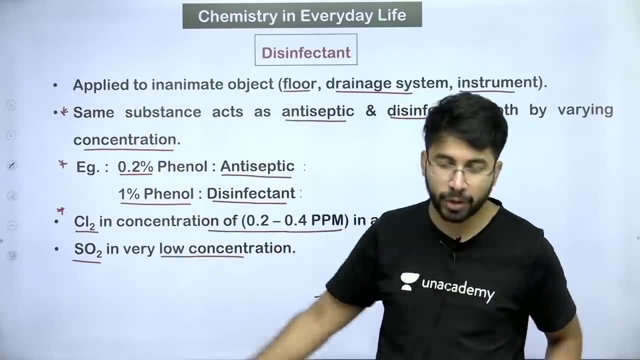 It works as a disinfectant. SO2 in very low concentration. It also works as a disinfectant. So From here, All the examples are part of your PYQ. Disinfectant is done After you have disinfectant. 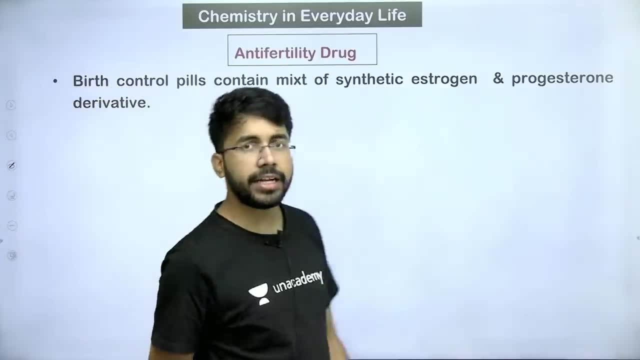 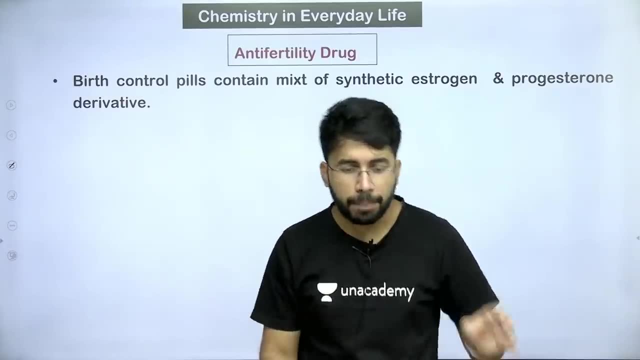 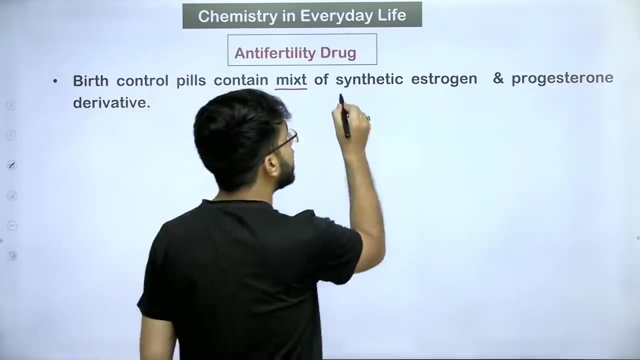 Now it is anti-fertility drug. Last is anti-fertility drug. What are these? They are called birth control pills. Okay, What happens in birth control pills? So, friends, This is a mixture of birth control pills. A mixture is used in birth control pills. 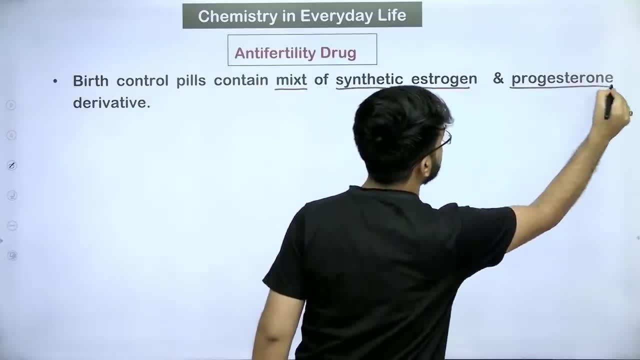 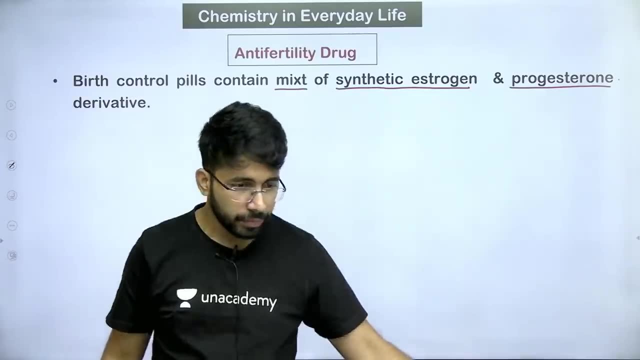 Which contains synthetic estrogen And progesterone. That is also synthetic. Okay, Progesterone derivative: Obviously that will be taken synthetic. Now, what is estrogen? what is progesterone? can you tell me Contacept? 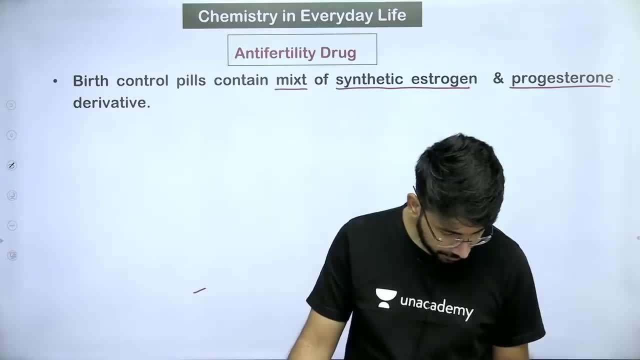 Very good, What is estrogen and progesterone in front of you, friends, can you tell me Contacept? Very good, Okay, Now in front of you, what is estrogen and what is progesterone, friends, Can you tell me? 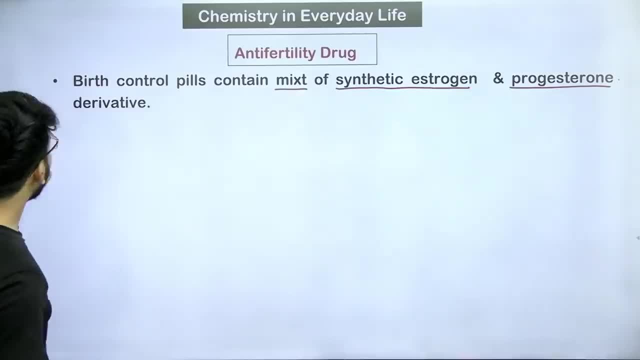 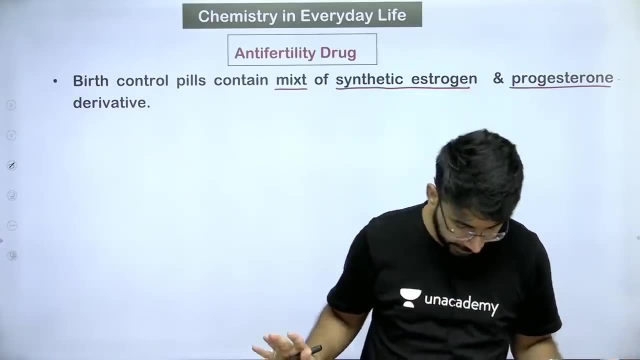 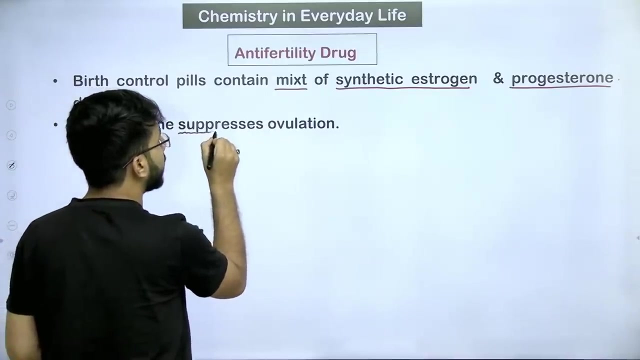 Contacept. Astrogen is a mixture of progesterone and progesterone, and antifertility is made from it. Now let me tell you that progesterone suppresses ovulation. Progesterone suppresses the ovulation in your body. 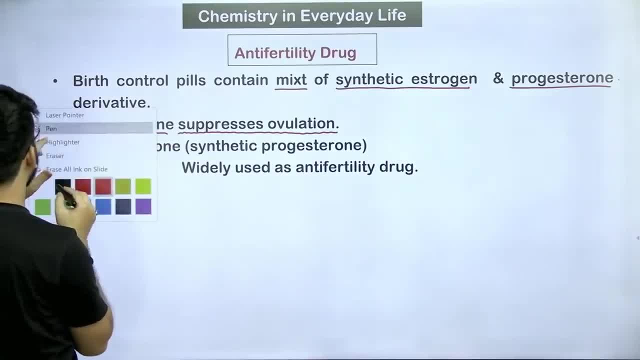 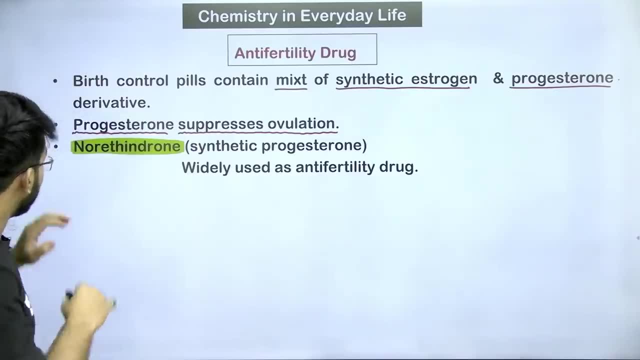 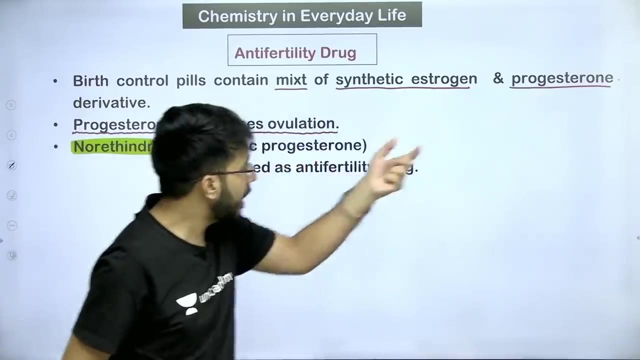 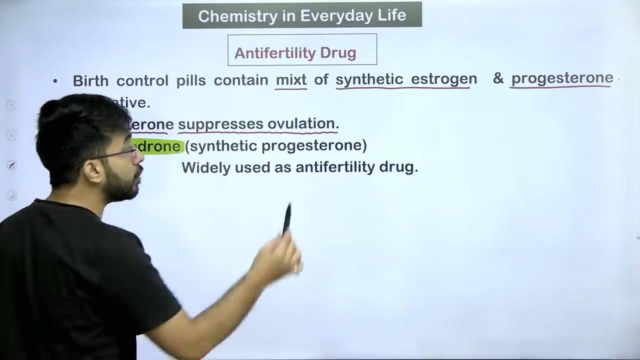 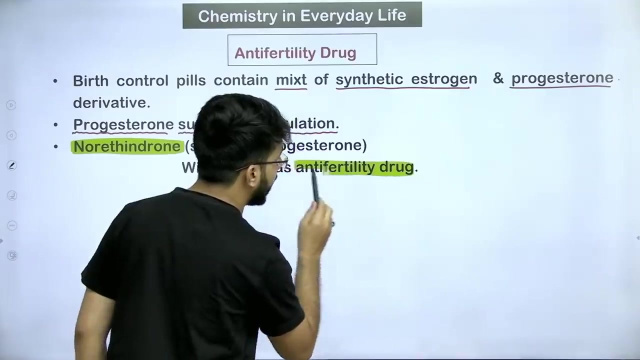 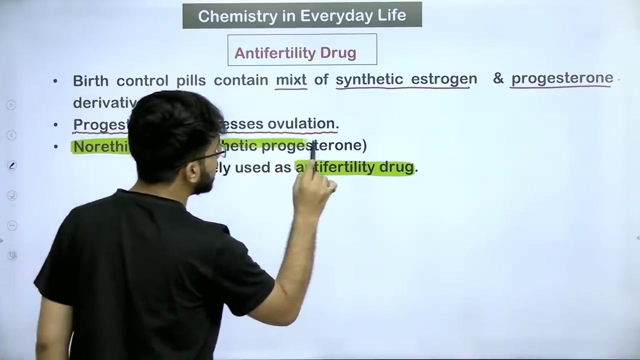 We have a drug called Northendron. Northendron is a synthetic progesterone. This synthetic progesterone is called Northendron. It is widely used as an antifertility drug. Next, it is widely used as an antifertility drug and we have a synthetic progesterone. 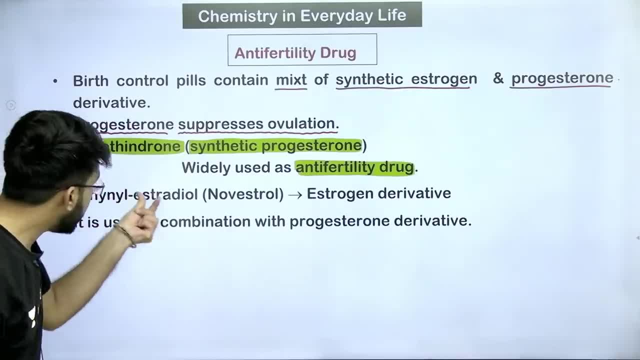 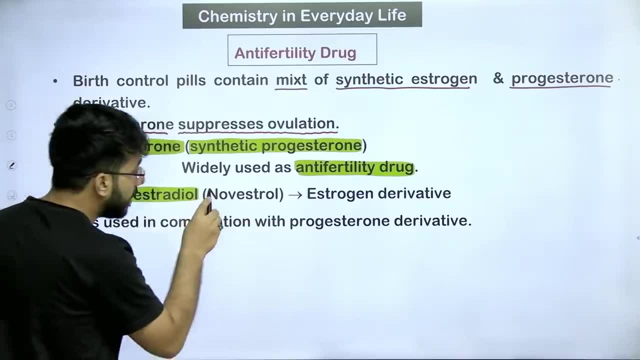 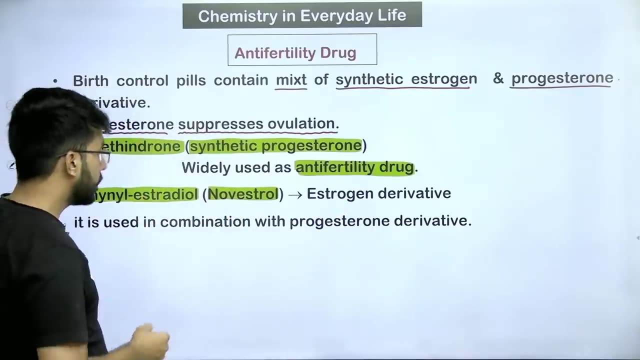 Next, Ethinyl Estradiol. You can see how complex the name is. Ethinyl Estradiol is known as Novastrol. This is an estrogen derivative. Progesterone derivative is Northendron. Novastrol is an estrogen derivative. 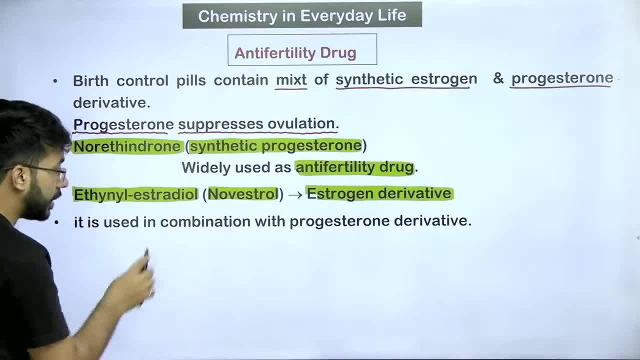 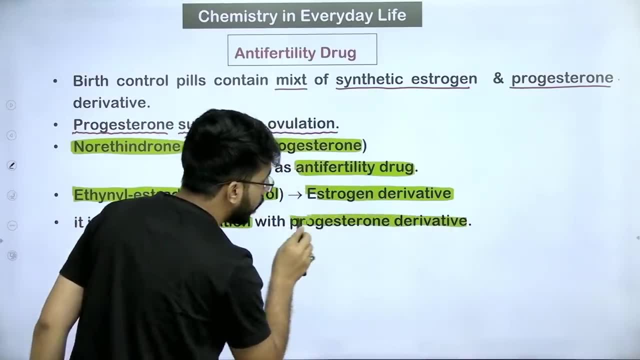 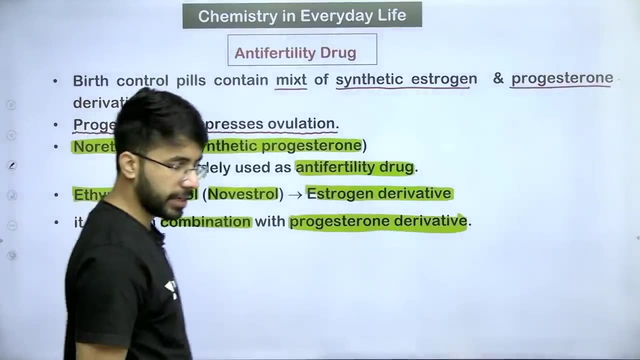 We use it with progesterone. It is used in combination. Novastrol is used in combination with progesterone. We use it as an antifertility drug. There are only two names: Northendron and Ethinyl Estradiol. 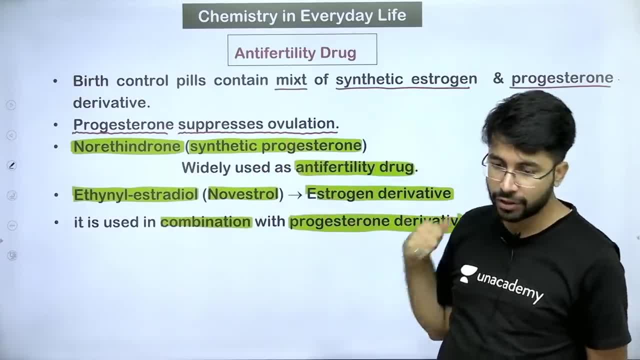 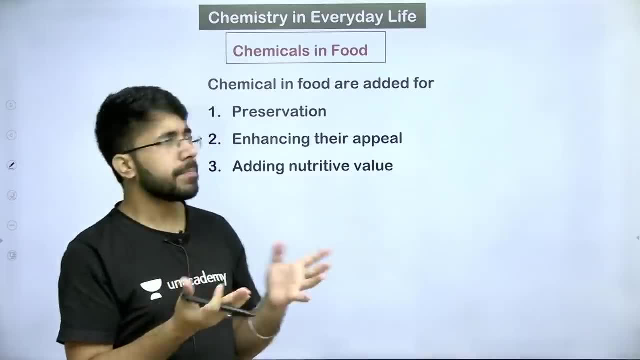 We also give the name of Novastrol. This is a synthetic progesterone. This is an estrogen derivative. Next, After antifertility drug, chemicals in food. This is the last one: Chemicals in food. What are the chemicals given to food to preserve? 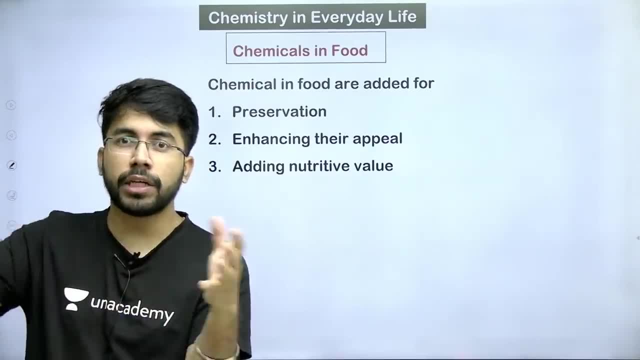 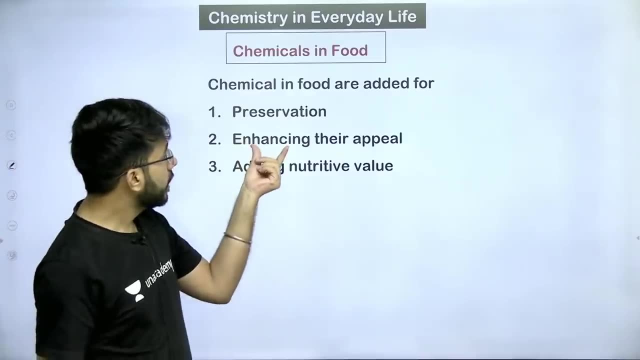 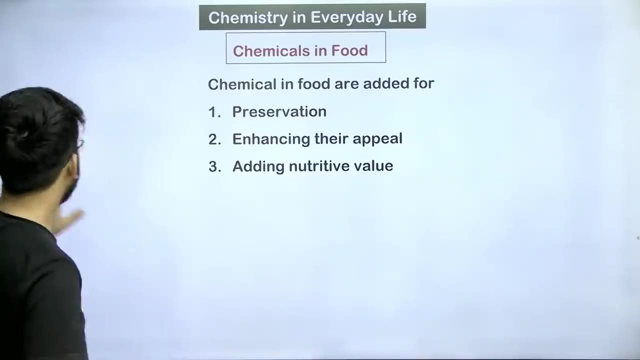 As you must have read that the shelf life of butter is 6 months, You will see that many butter are coming in the shelf life of 6 months, Enhancing their appeal To increase beauty, To increase its nutritive value. Many times we use it. 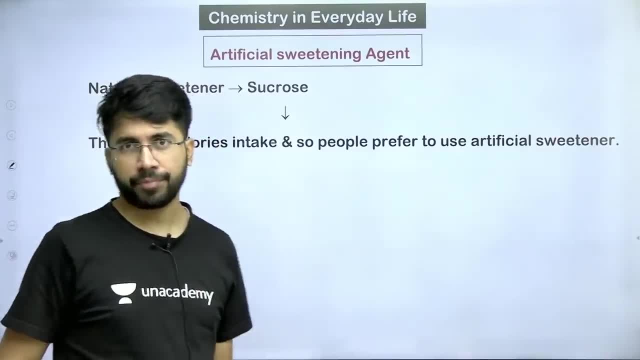 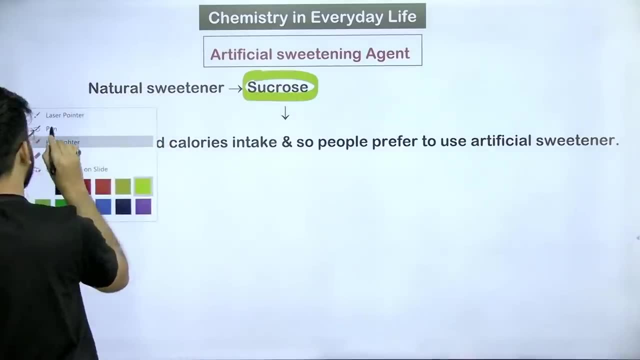 Let's come First of all. let's see which is the artificial sweetening agent. The question comes from this: Natural sweetener is sucrose. What is natural sweetener? Sucrose is in front of you, But the sucrose. 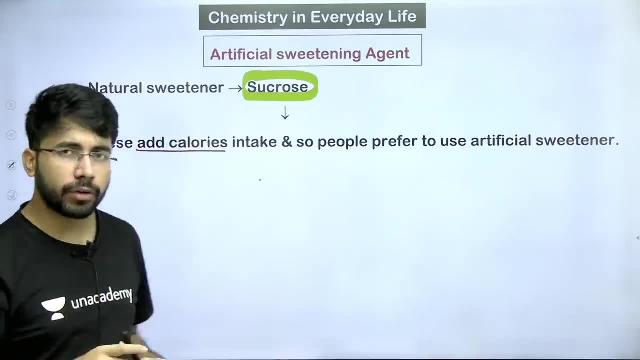 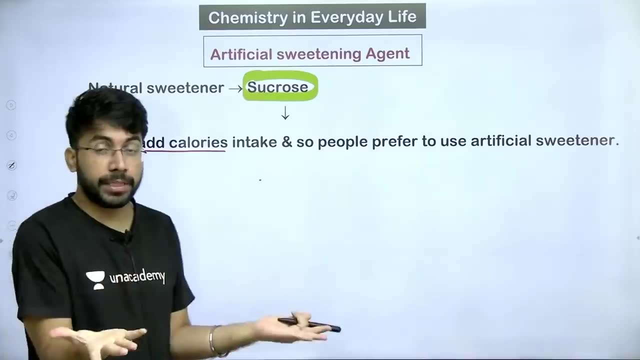 These add calories. If you add natural sweetener to sucrose, Then it increases the calorie, But nowadays we are conscious of calories. No, we have to take only this much calorie. Then we will have to burn so much in the gym. 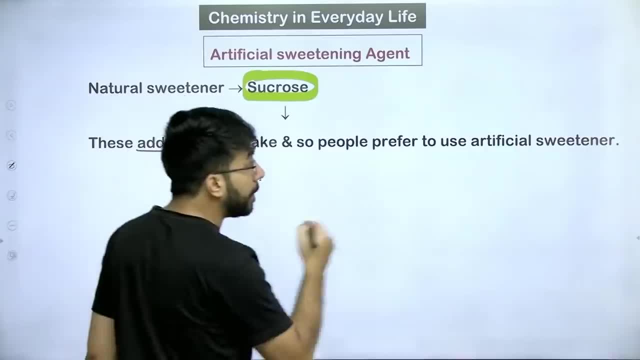 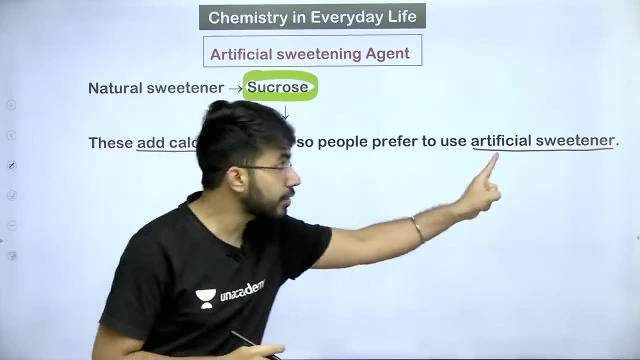 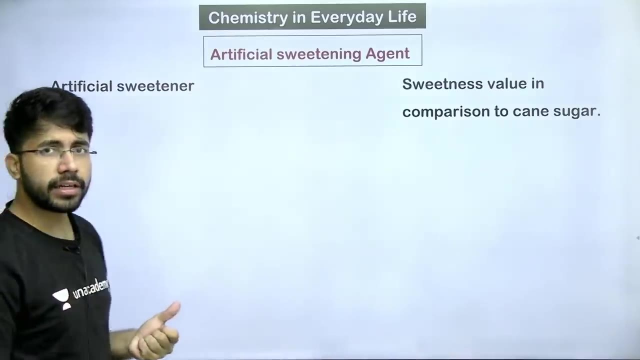 So friends, add, calorie Add. So people use artificial sweetener. Why? In natural sweetener the calorie will increase. So let's take artificial sweetener. Why? Because artificial sweetener does not add calories. Now artificial sweetener. You have four artificial sweeteners. 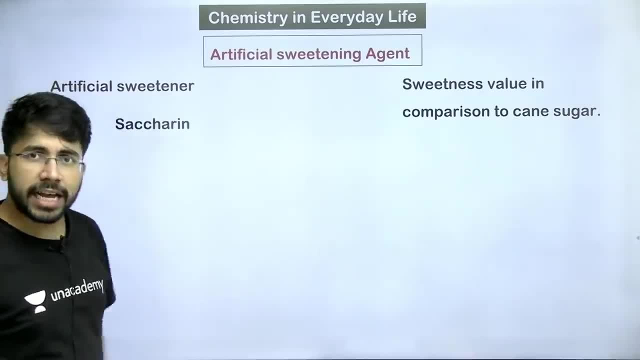 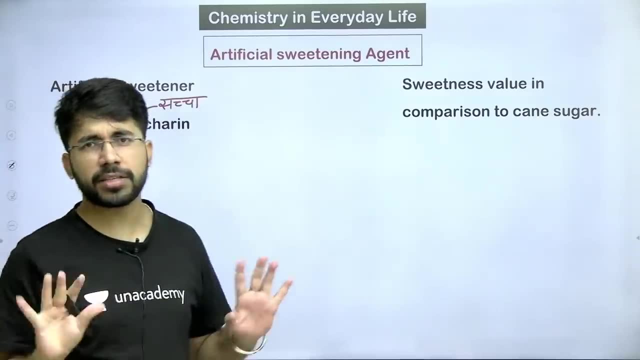 Let's read one by one. First of all, in front of you is saccharin. Saccharin will be coming to your mind here. True, It will be clear from this. It is of a very true heart. It is of a very pure heart. 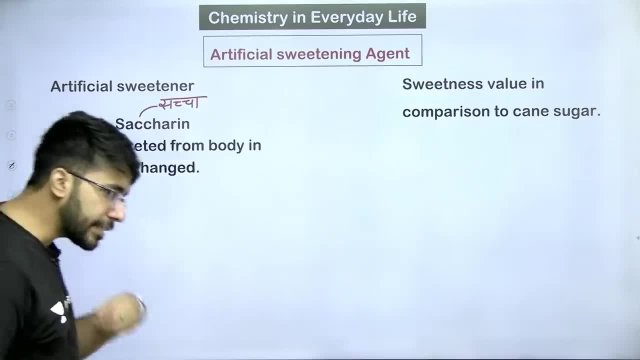 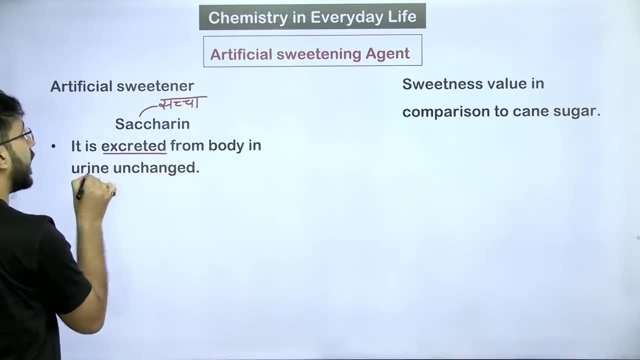 As you take it. As you take it, It will be excreted in the same way, The way you intake this body. Similarly, it is excreted in the same way, in the unchanged form, So this is not a harm to your body. 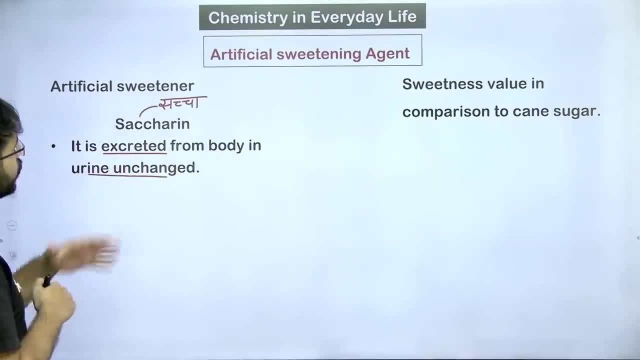 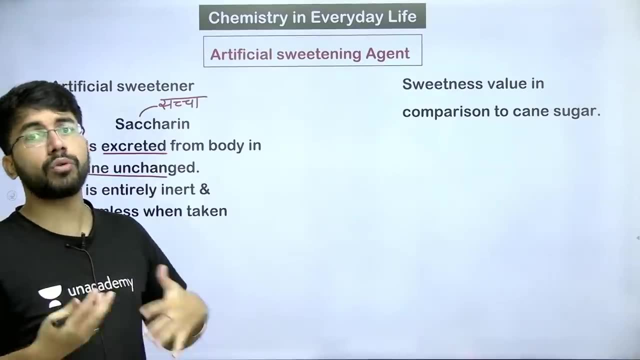 Calories have not been added. Very good person, Very good thing. This is true Saccharin. Second, It is entirely inert. No one reacts. It is not like if it goes in the body, Then do some different reaction, Then some different disease is happening. 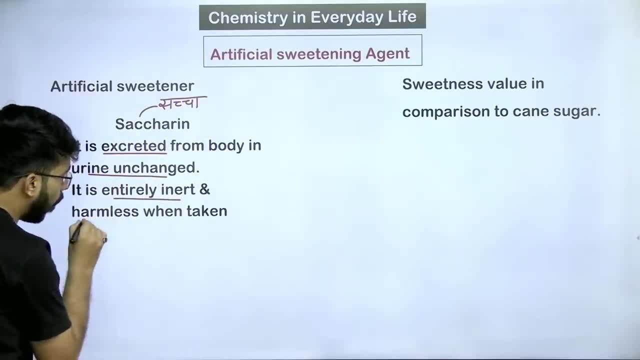 Something else is happening. So it is chemically inert And harmful And it is harmless. No harm will be done to it. Third thing: my friend comes Useful for diabetic person. This is very good for a diabetic person. Do you know why? 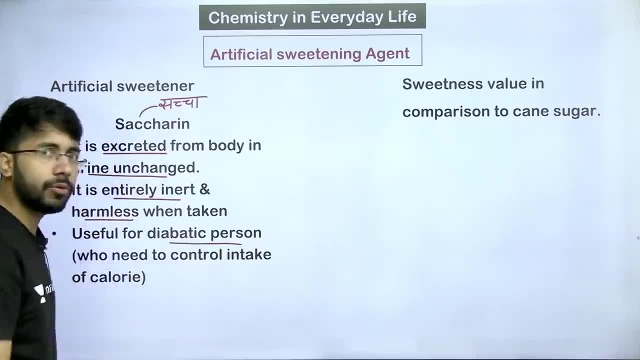 Because diabetic person has to control calories And he is not getting the calorie. So who need to control calorie? So saccharin is very beneficial. The way you intake, In the unchanged form, It comes out of the urine. Second, my friend, 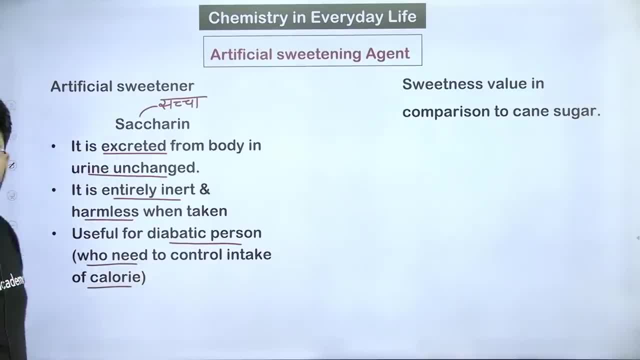 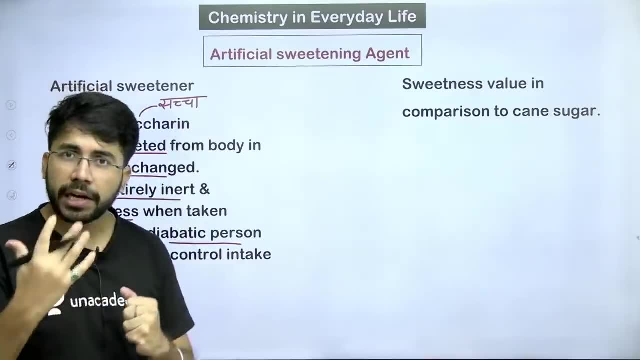 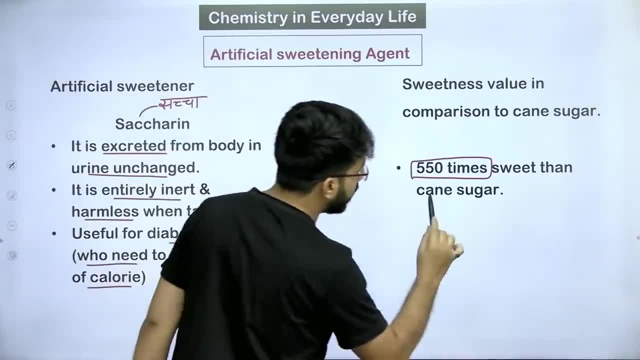 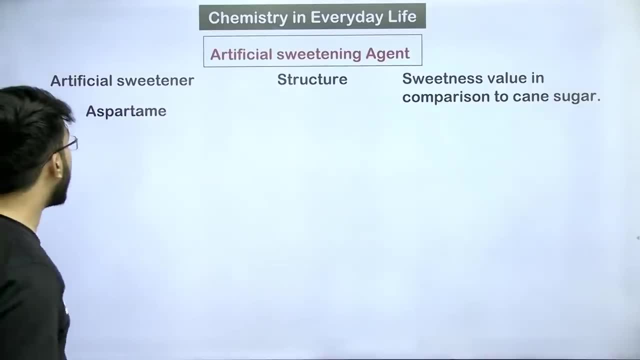 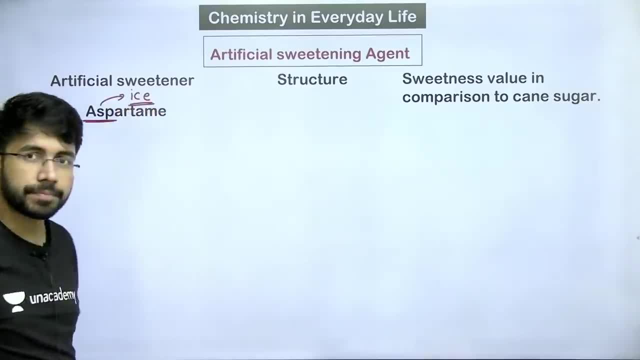 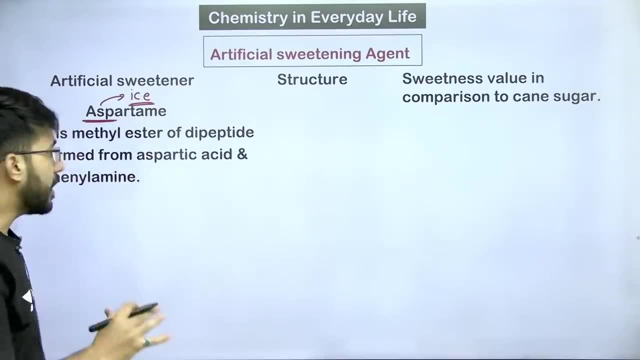 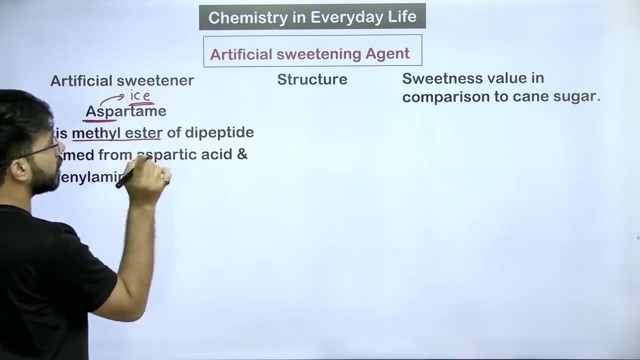 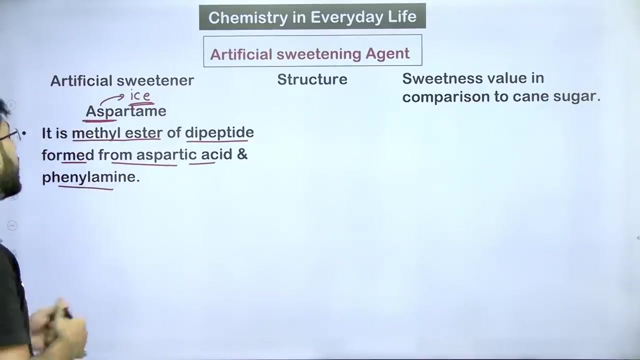 Saccharin, Saccharin, Saccharin, Saccharin, Saccharin, Saccharin, Saccharin. It is a methylester of dipeptide formed from aspartic acid and phenylamine. Aspartic acid and phenylamine makes aspartame. 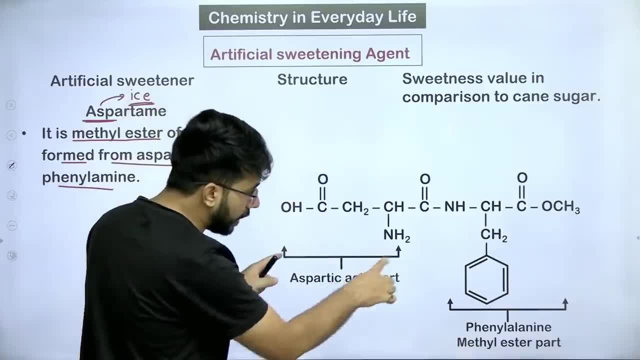 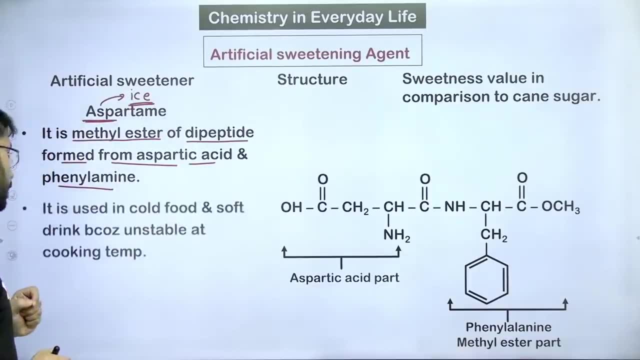 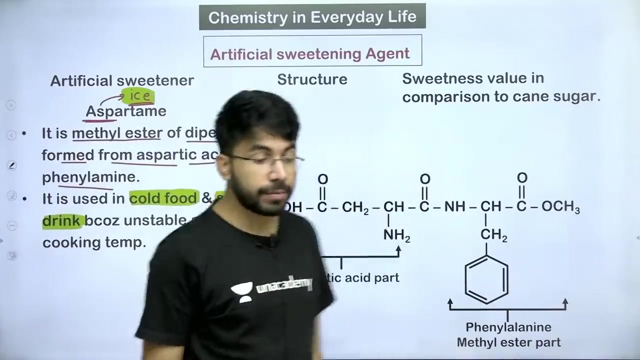 Aspartic acid and phenylamine make aspartame. Aspartame is used in cold food and soft drink. Aspartame is used in cold food and soft drink Why, As soon as it is taken to cooking temperature, it will become unstable. 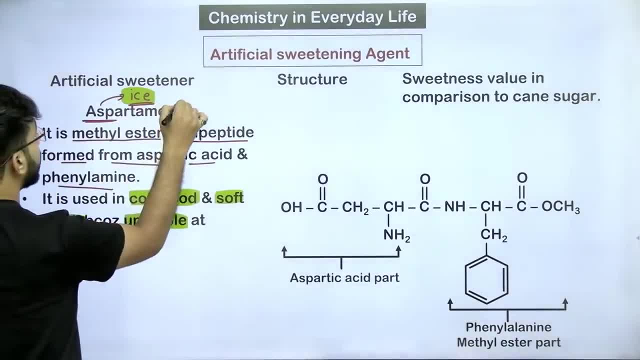 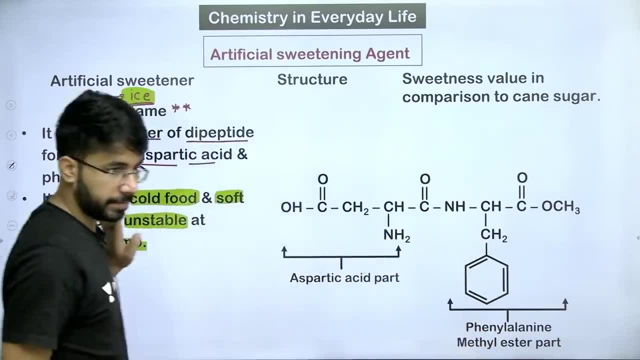 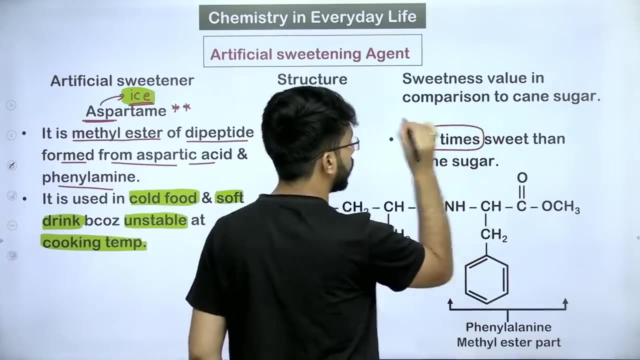 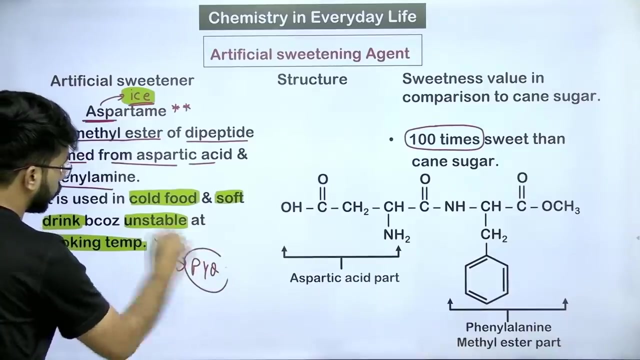 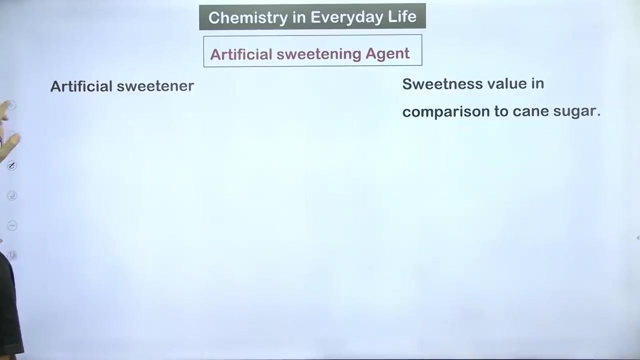 As soon as it is taken to cooking temperature it will become unstable. As soon as it is taken to cooking temperature, it will become unstable. Aspartame is used in cold-temperature ice and is unstable in cooking temperature. Aspartame ice at cold temperature. 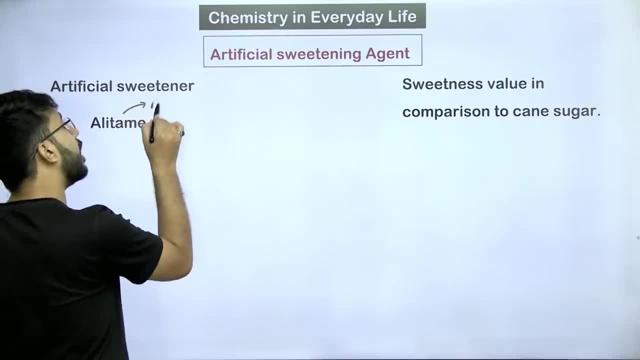 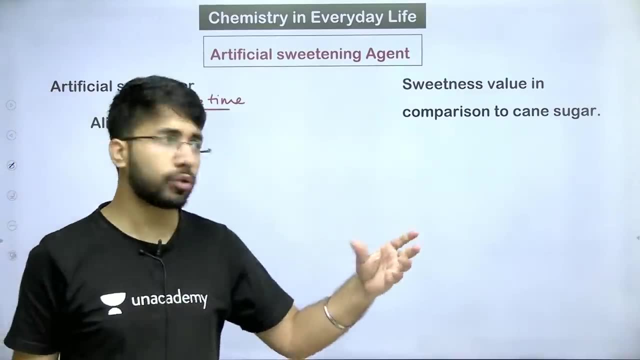 Third one is eletame. Think of eletame as all the time. Eletame is all time. All the time or all time Means it is 2000 times sweeter. It is 2000 times sweeter. It is that much sweeter. 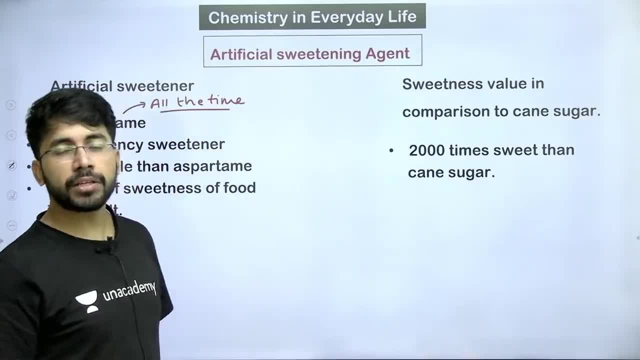 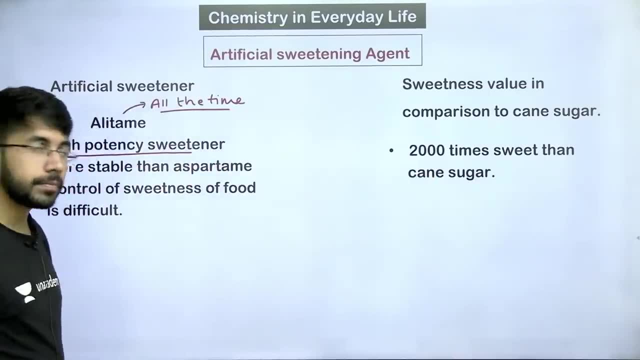 It is 550, the real one. And what is the other one in front of you, Sir? it is 100 times Here. you will see, in eletame, High potency sweetener is there. It is 2000 times sweeter. 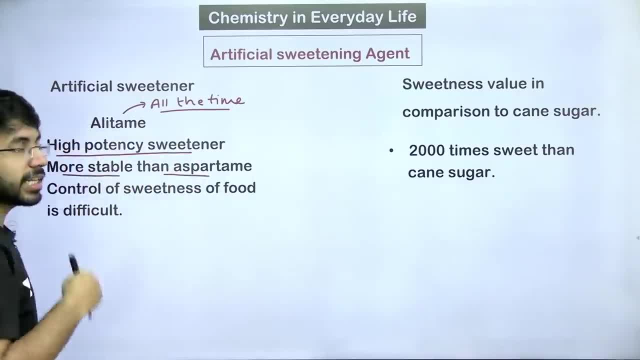 Second thing: More stable than aspartame. It is more stable than aspartame Because as it increases the temperature, it breaks and becomes unstable. The problem is that you cannot control the sweetness of the food. If you add it, it becomes very sweet. 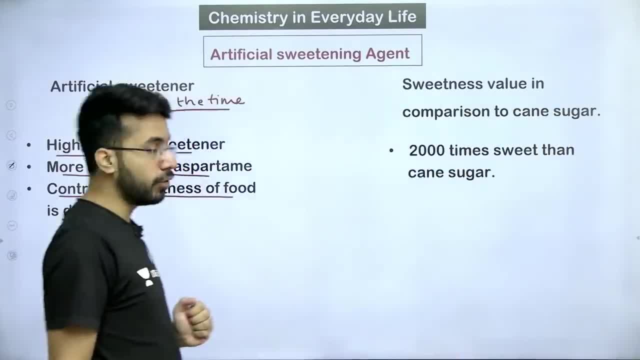 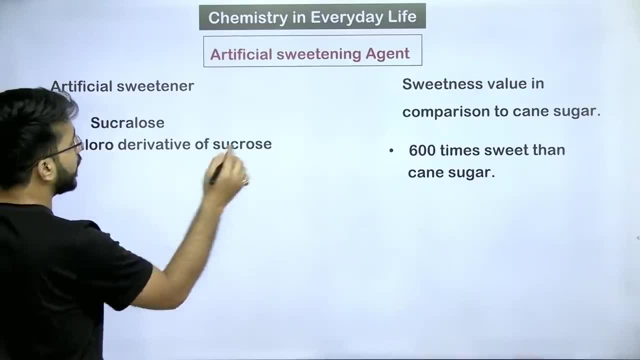 It is 2000 times sweet. It is very sweet. We use eletame for that. And last is sacralose. Sacralose is the trichloro derivative of sacrose, Sacrose's trichloro. It is the trichloro derivative. 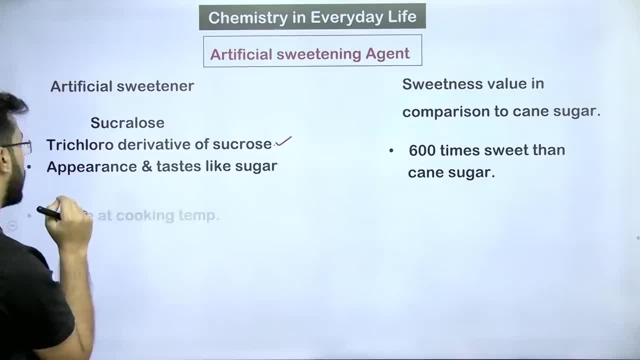 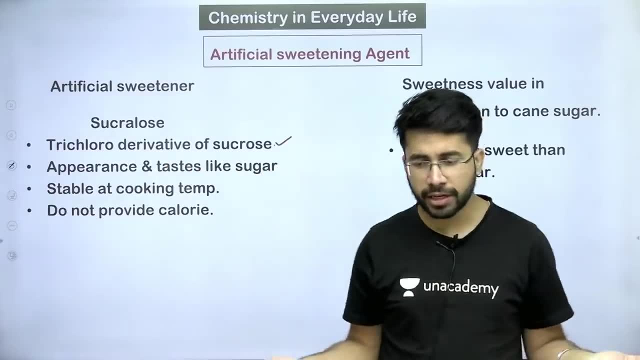 It is 600 times stable. Appearance and taste is like sugar, Stable at cooking temperature. And, last is, it does not provide any calories. No artificial sweetener provides calories. It also does not provide calories. Okay, What happens in food preservative? 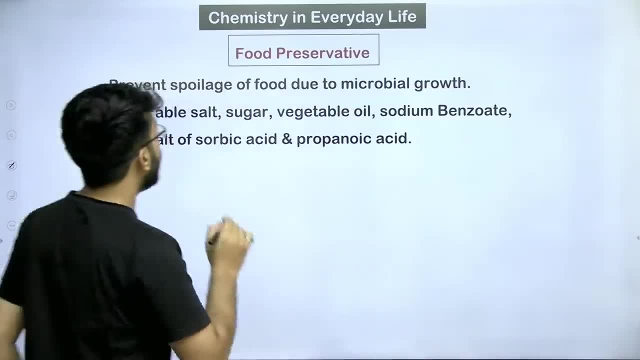 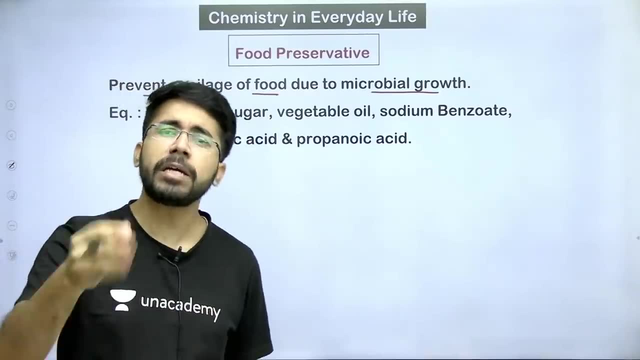 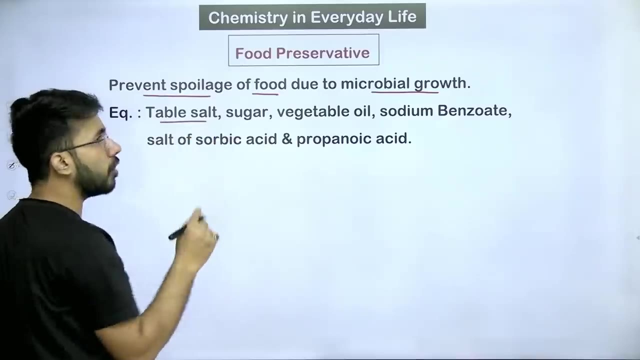 To preserve food. What do we add in it? Food preserve prevents spoiling of food due to microbial growth, Fungus, bacterial virus, any bacteria in it. Food starts spoiling. To preserve it, we use food preservative: Table salt. 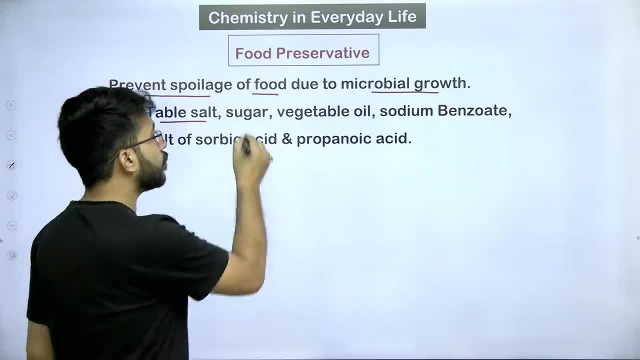 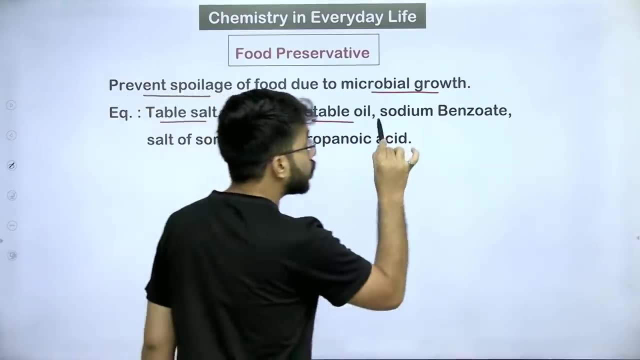 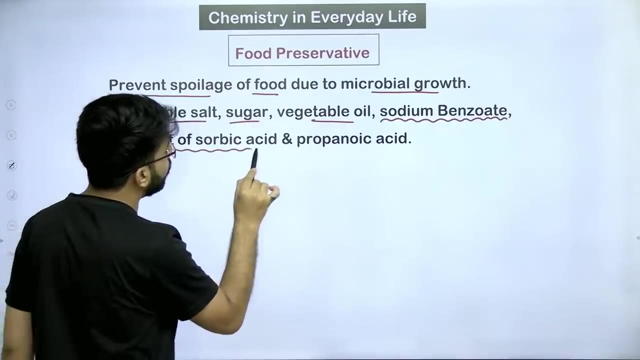 For example, we add two table salts in pickle Sugar. This also works as a preservative. We add oil in pickle, Otherwise it will spoil. Sodium benzoate acts as food preservative. Salt of sorbic acid and propanoic acid. 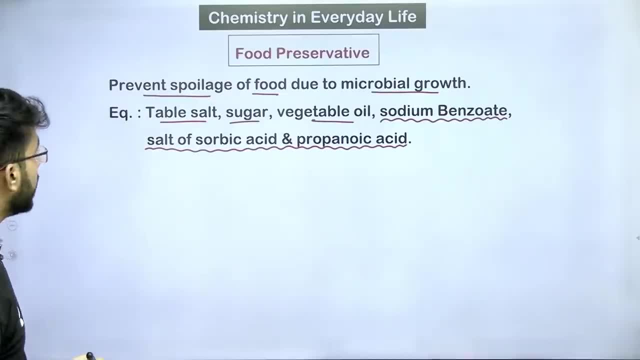 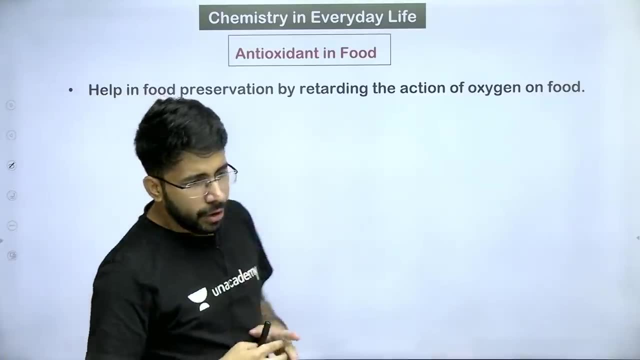 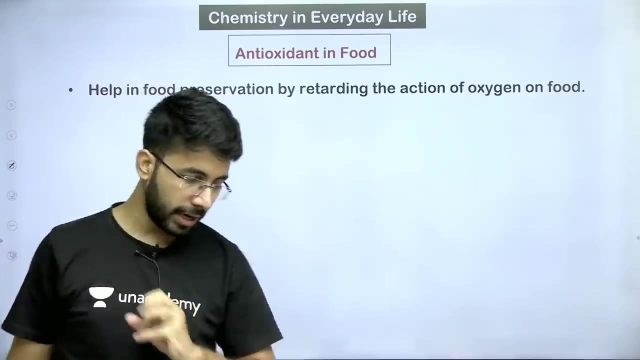 What does it use? Food preservative Salt of sorbic acid and propanoic acid Come. Antioxidant Help in food preservation by retarding the action of oxygen on food. If oxygen is added in food then food spoils. 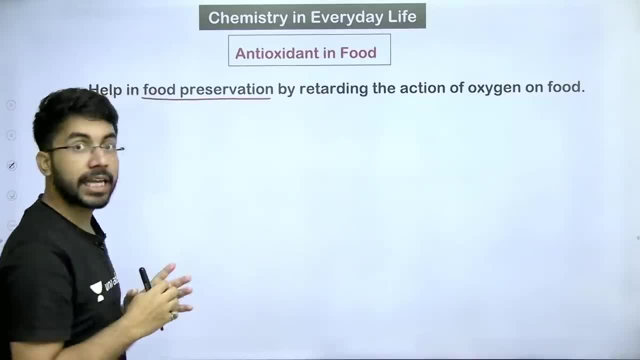 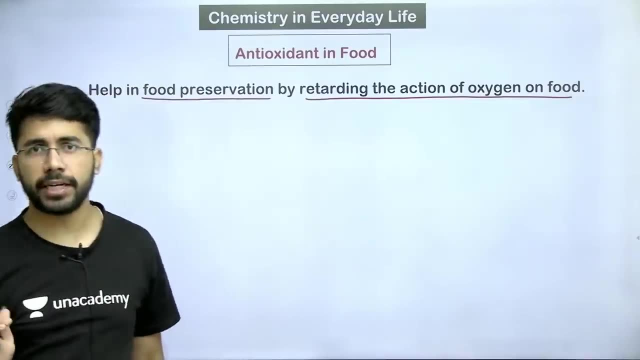 Okay, So it helps in food preservation. How, By retarding the action of oxygen on food, It reduces the action of oxygen on food. If it does not go away from oxygen, then it will not spoil, So it will not spoil. 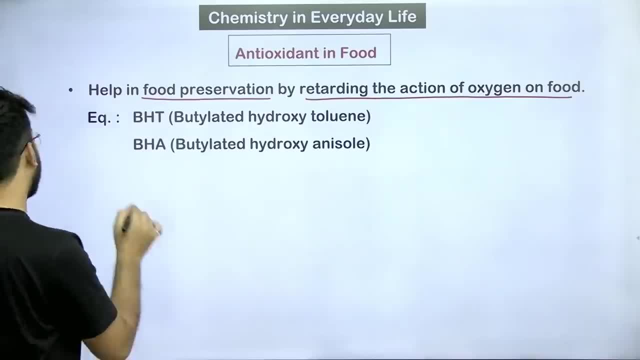 For this we use antioxidants. So it becomes VVIP from here, Because antioxidants are not given in old NCRT. But if you open new NCRT then antioxidants are added in it, And if new NCRT is added then the chances of being asked are increased. 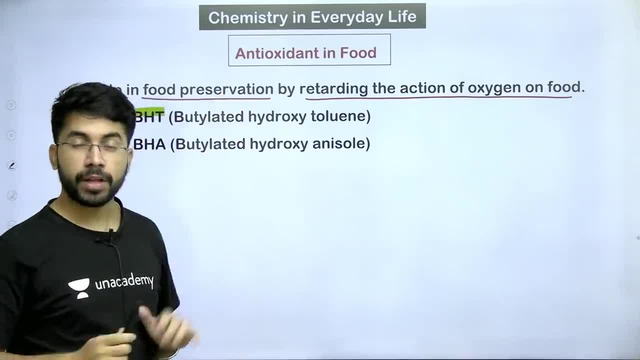 BHT and BHA. It is in new NCRT. Open old NCRT and see You will not get. So, BHT and BHA, What will happen? Butylated hydroxide. So the NCRT is added in it. 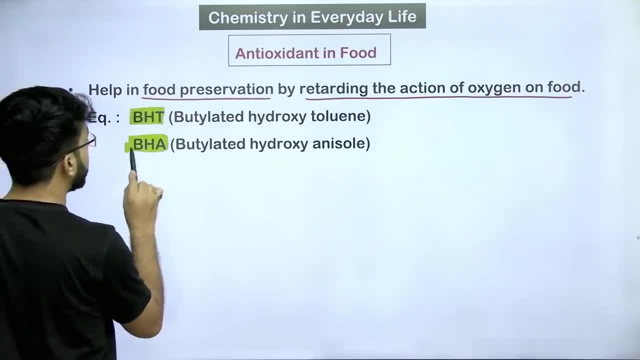 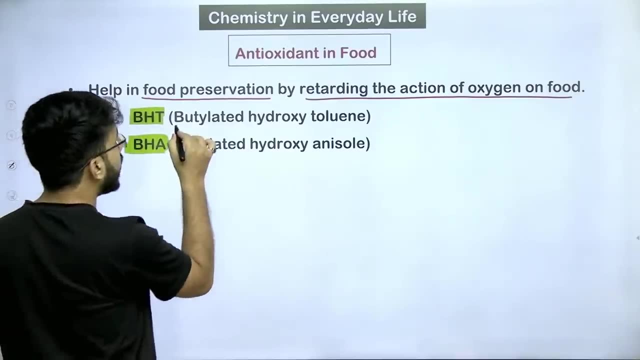 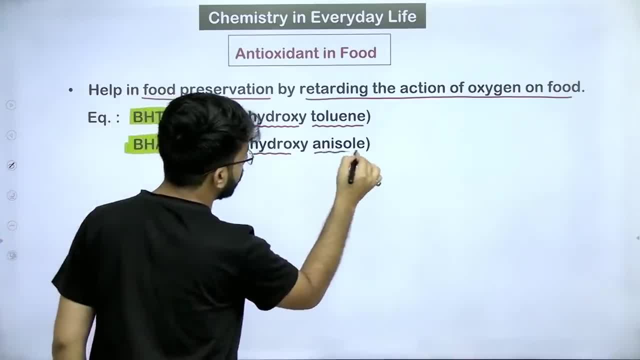 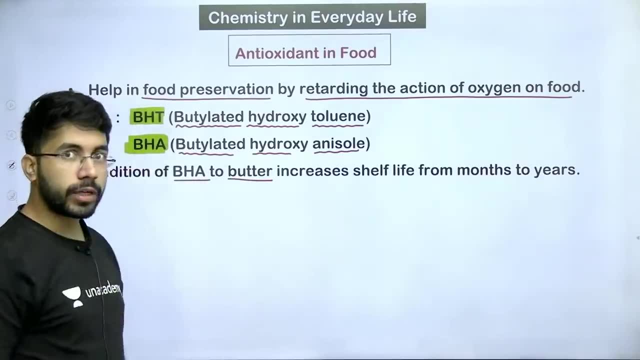 Butylated hydroxide is added along with it. These are both antioxidants. Если я far dürfen, Let's say in butter. You have put BHA inside, Which is an antioxidant. That isation of BHA. Is there any antioxidant around In butter? 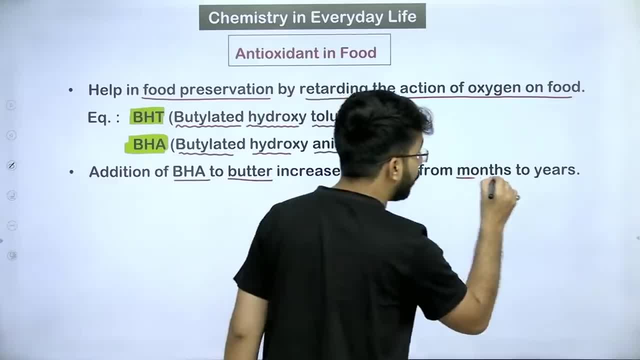 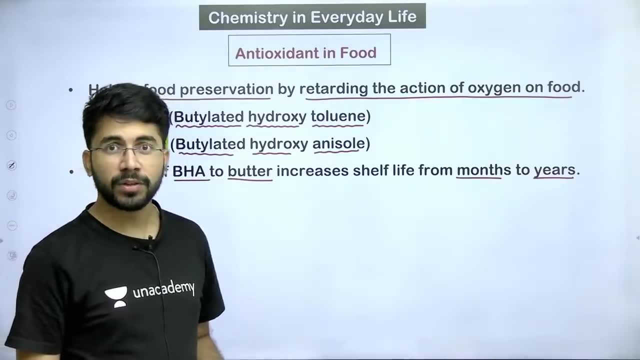 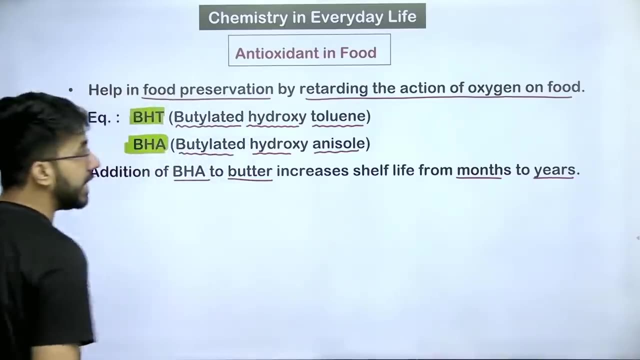 It chore consistently increases the shelf-life of your butter for six months. Well, This means few months to years. You can preserve the butter for whole year. The sell-for of it remains in the mall for years. You have to buy. But if I put BHA in butter, its shelf life changes from month to year. 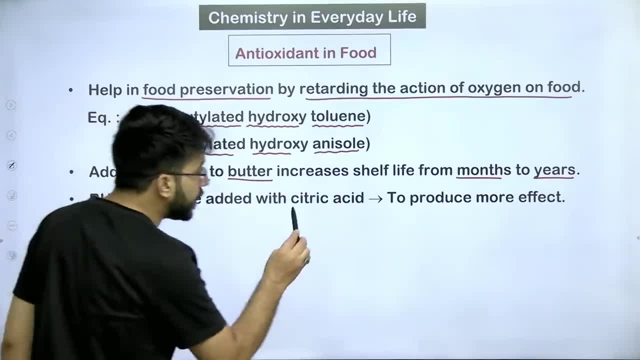 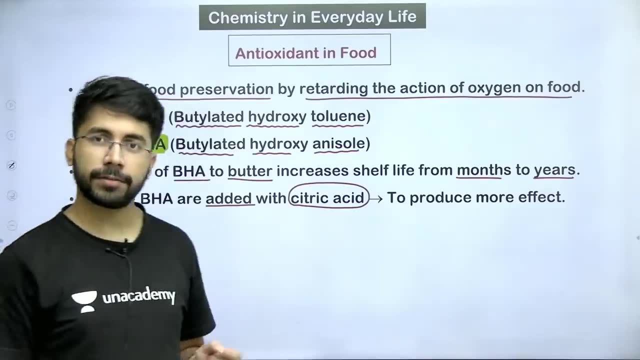 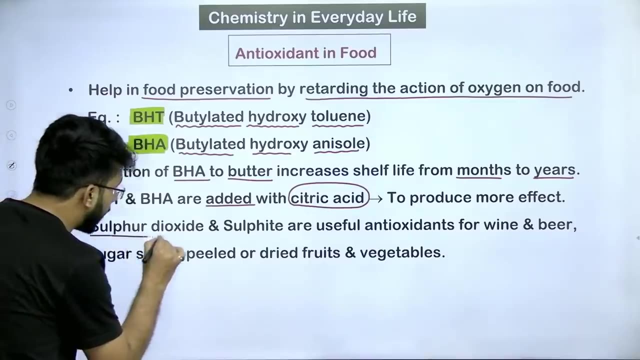 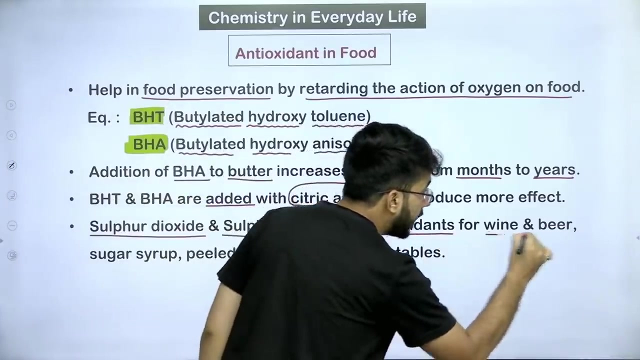 Next, BHA, and BHA are added with citric acid to produce more effect. Next, Sulphur dioxide and Sulphite. Sulphur dioxide is SO2 and Sulphite is SO3.. These are antioxidants for wine and beer. 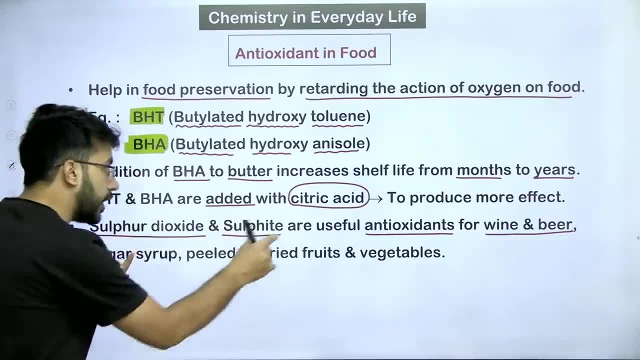 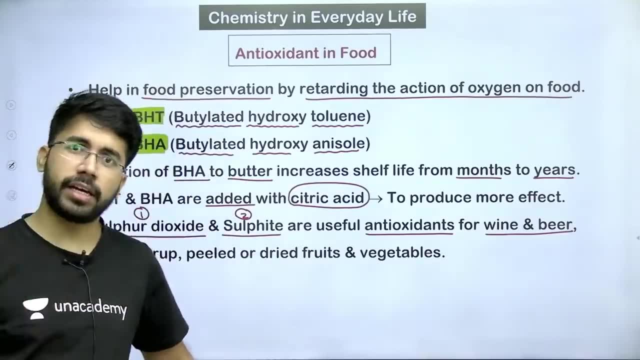 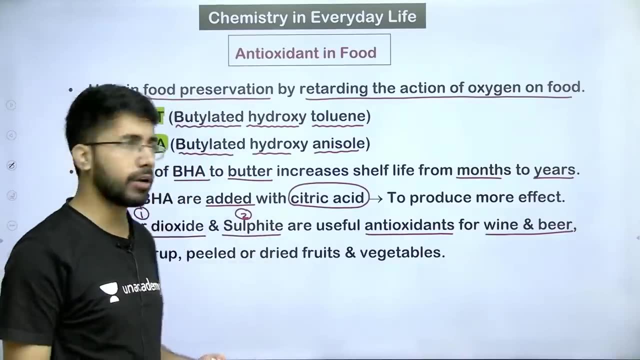 Both of these antioxidants are used for wine and beer. Wine is also preserved for a long time. Take a bottle like this. We use antioxidants in it. If it comes in contact with oxygen, its quality will deteriorate. Sugar syrup and peeled or dried fruits and vegetables. 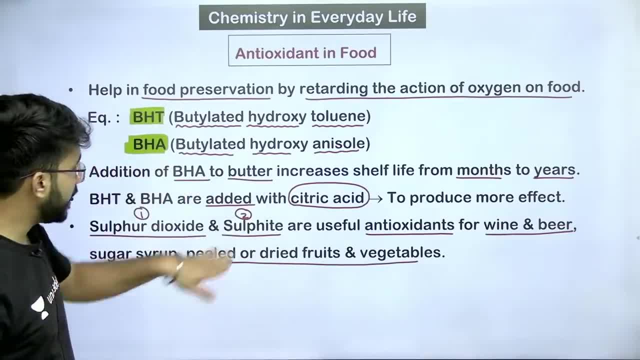 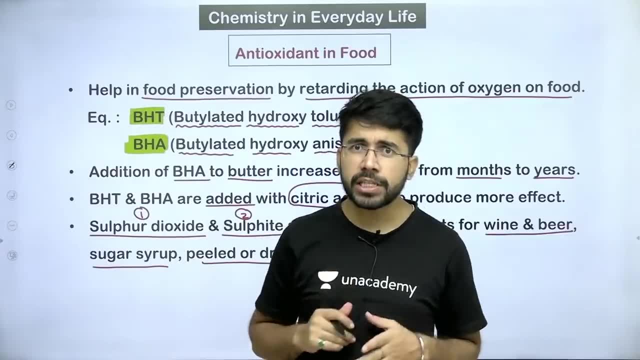 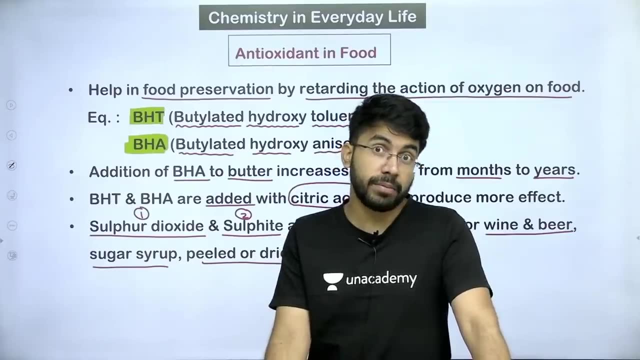 These are also used for sugar syrup. Antioxidants are used for peeled or dried fruits and vegetables. As you must have seen in the malls, they are kept in a plastic coating, Just like there are cut vegetables. they are kept in a plastic coating. 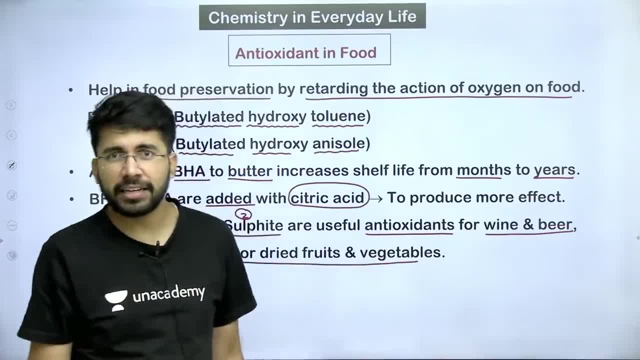 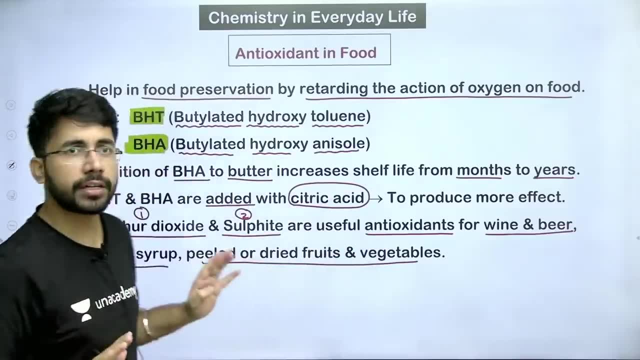 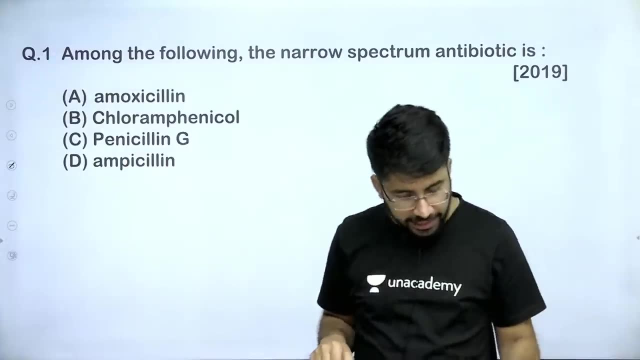 In that plastic coating, Antioxidants are put on the cover of the plastic and then they are stuck So that it gets rid of the contact with air. Next, Now, friends, you have to do PYQ Cleansing agents. do not ask questions. 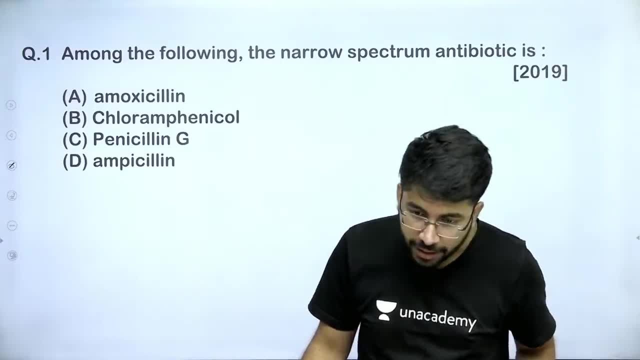 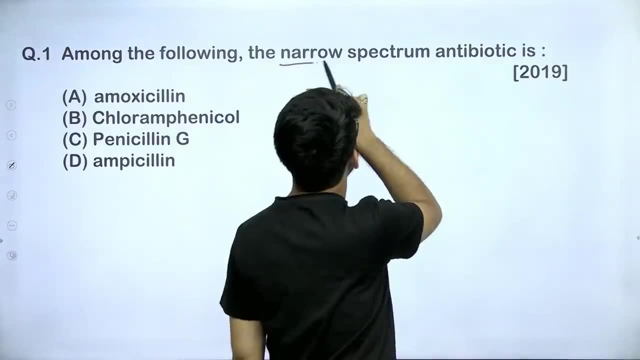 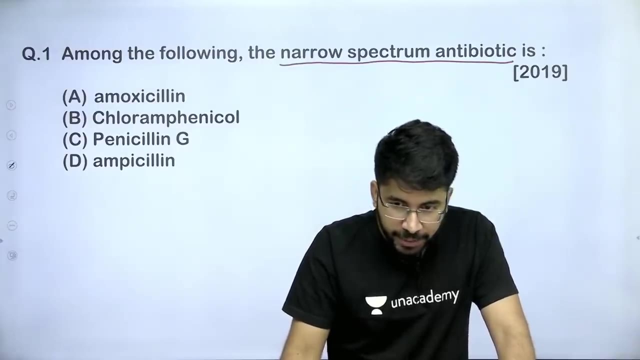 We have not come yet. Go ahead Now. who is the antibiotic? Which of the following narrow spectrum antibiotic- Narrow spectrum antibiotic. Narrow spectrum- Narrow spectrum? There was only one. Come on, Who is the narrow spectrum antibiotic? Look at the question of 2019.. 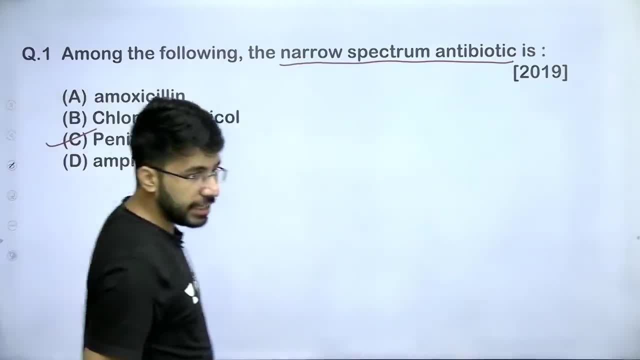 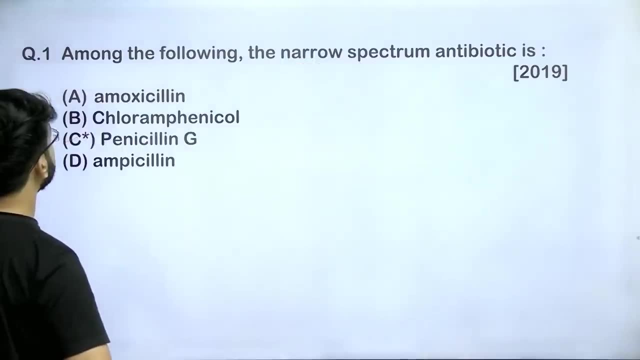 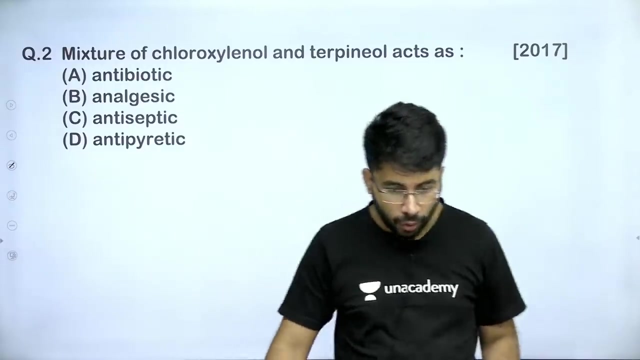 Great, Very great. Penicillin G: What was Okawa friend? It was in the broad spectrum And Penicillin G was the narrow spectrum antibiotic. Next, Mixture of What are these two called Mixture of terpenol and chlorozylenol. 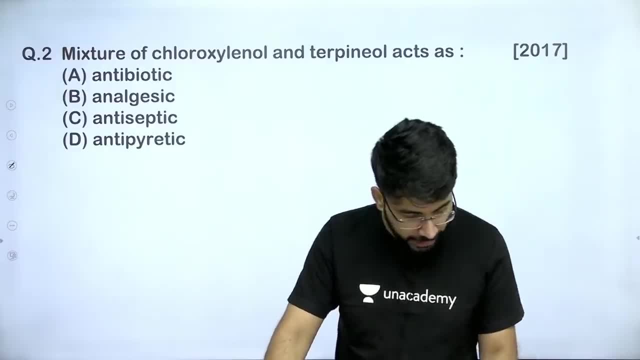 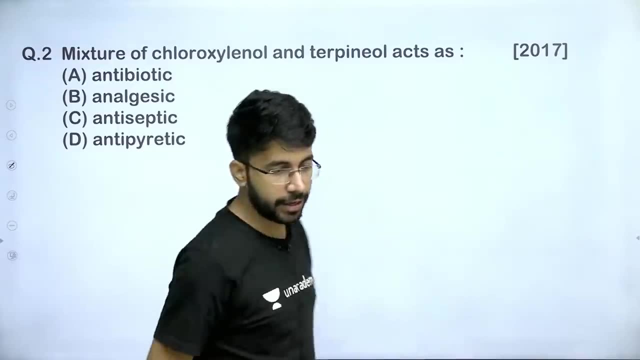 Come on, everybody. Mixture of terpenol and chlorozylenol. Mixture of terpenol and chlorozylenol- Everybody. Structures do not come. Do not see the structures of chemistry in everyday life, My friend. these two together will make detol. 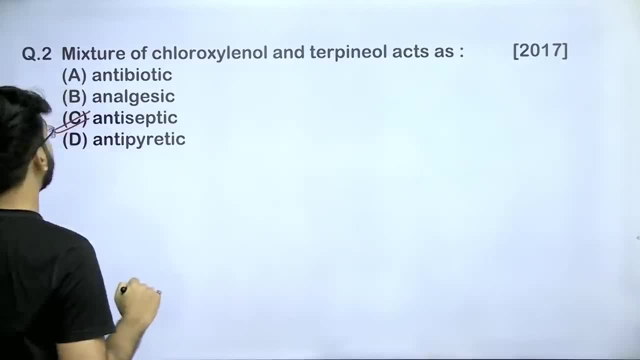 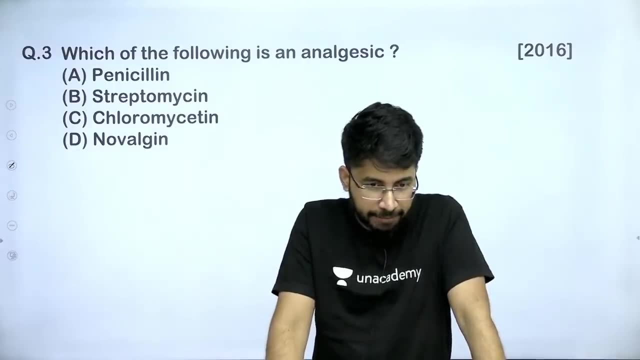 It is antiseptic. These two together make detol. It is antiseptic. Next, Which is analgesic? Which of the following is an analgesic? Who is analgesic? Who is the pain killing effect? Something like that. 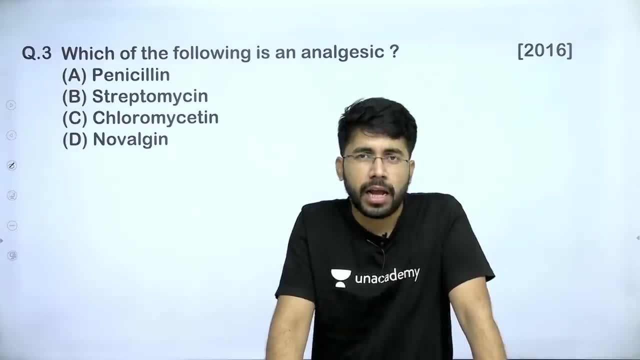 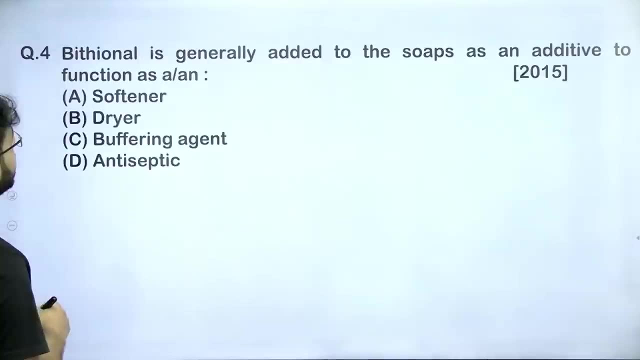 In analgesics I had told something: Asha, paracetamol, aspirin, paracetamol, ibuprofen and novelgene. So, friends, you will see novelgene. Ok, You will see novelgene in front of you. 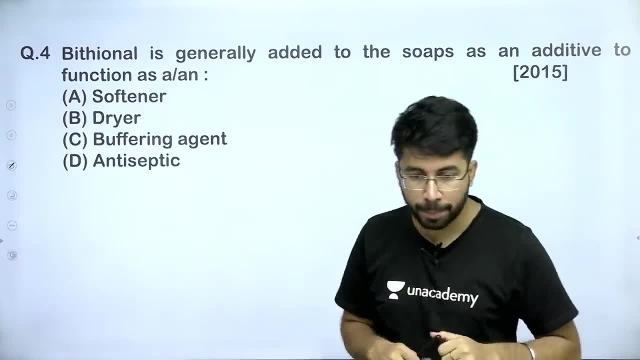 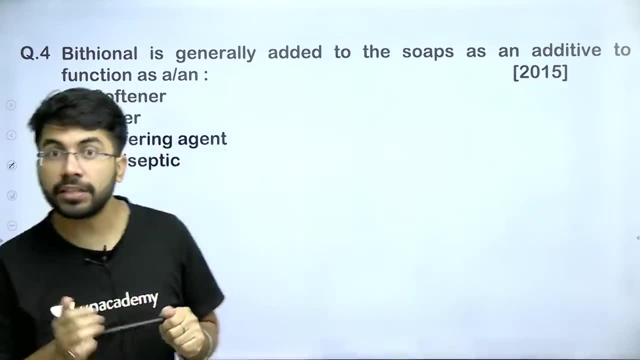 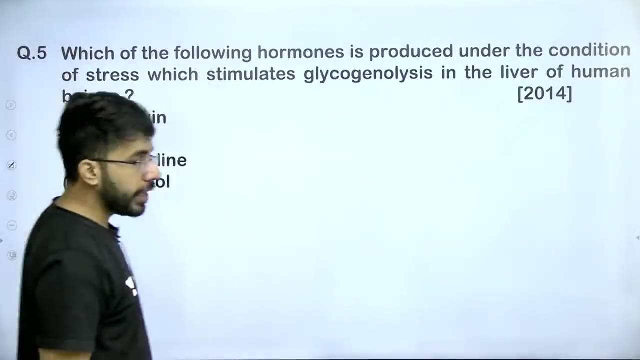 Next, We add bithionol in soap To function as. What is the function of bithionol? It is the function of killing germs up to 99%. It is the work of antiseptic. Next, Which of the following hormone is produced under the condition: 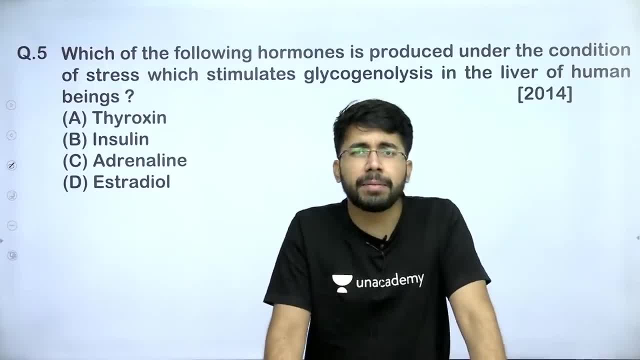 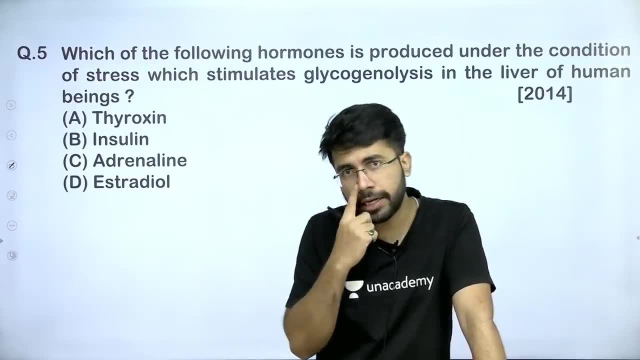 Next, Which of the following is produced under the condition of stress? When you are under stress, which of the following hormone is released? Which of the following hormone is released under the condition of stress? There is no need to read the answer You have heard about Adrenaline Rush. 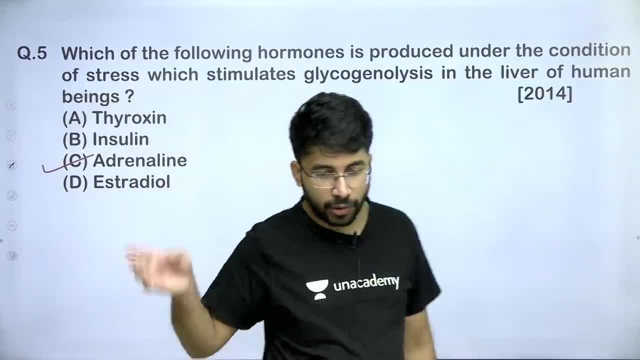 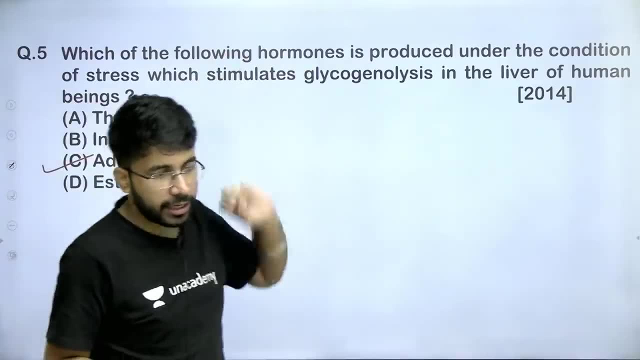 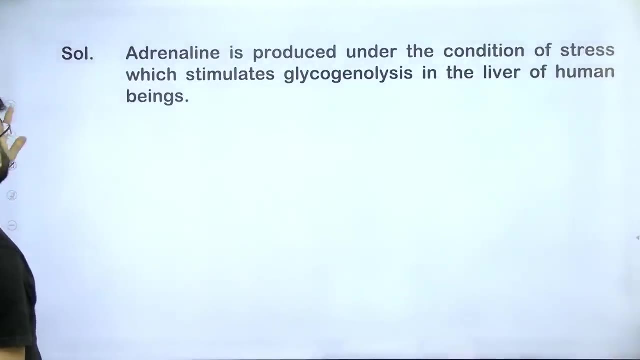 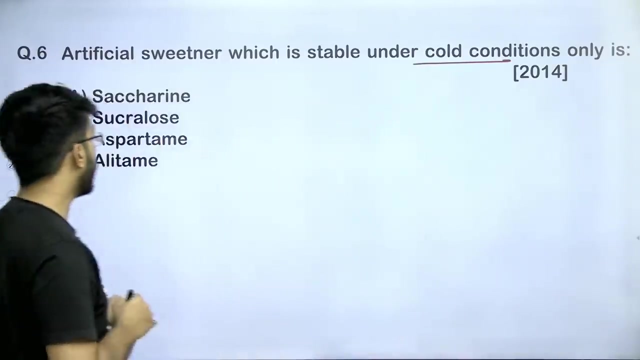 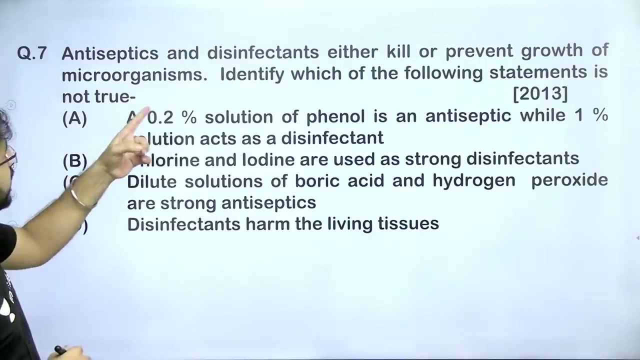 Adrenaline rush is released which is thicker than the pressure of blood. The following hormone is produced under the condition of stress. Next, artificial sweeteners in cold condition, ice or aspartame. ice or aspartame: see option. Next, antiseptic and disinfectant: either kill or prevent growth of microorganism. 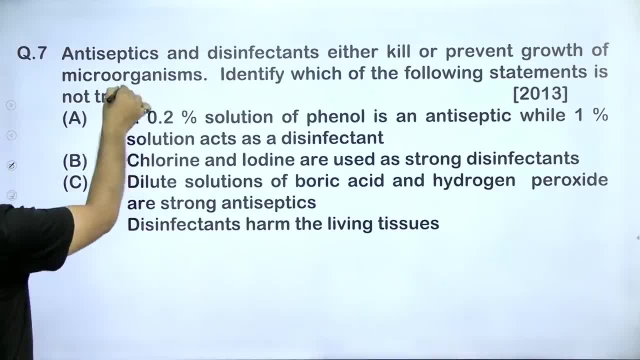 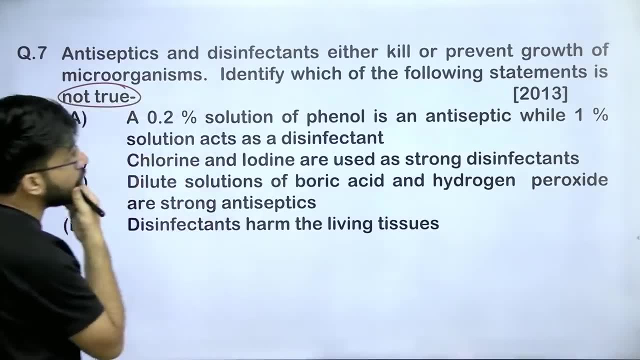 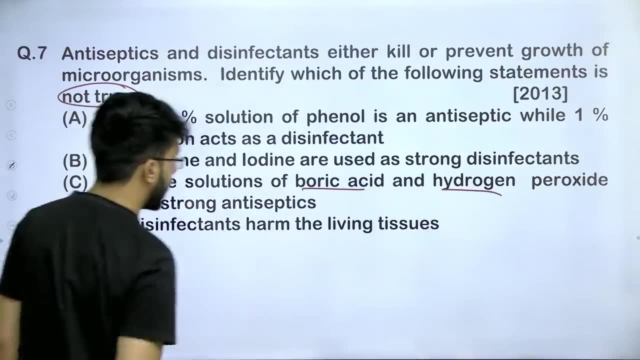 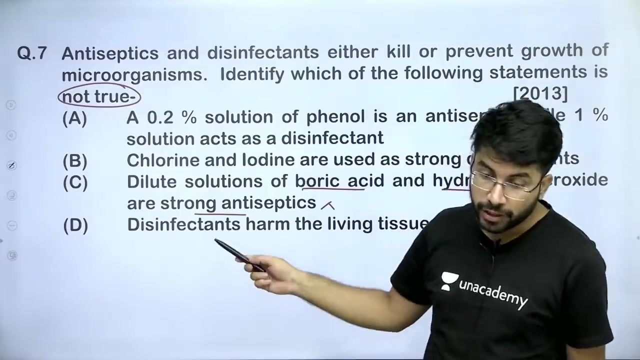 Identify not true statement. See it is saying not true. It is saying dilute solution of boric acid and hydrogen peroxide are strong antiseptic. We have not studied hydrogen peroxide. We have not studied H2O2.. And they are not strong. 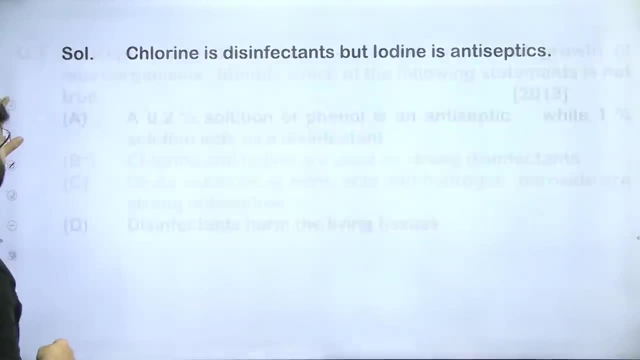 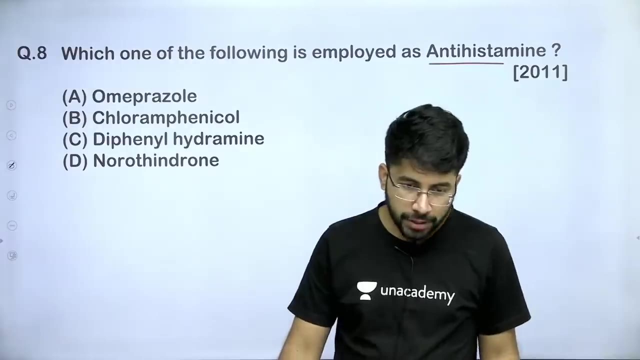 Next, Next, Which one of the following is employed as an antihistamine? Who is antihistamine? Omeprazole or chloramphenicol, or diphenylhydramine or northrindrone? What is it? 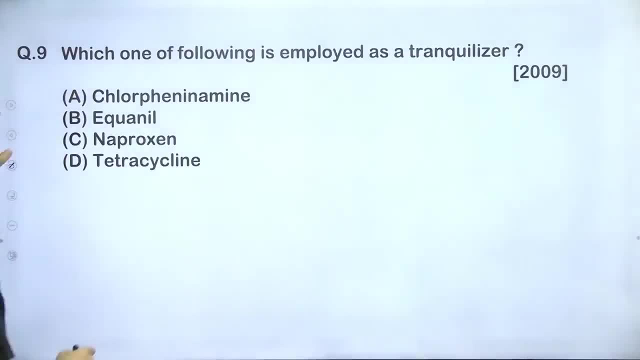 Who is it that works as antihistamine? My friend? where is antihistamine in front of you? This is omeprazole. Next, Come here, Sorry. Which is tranquilizer? I have told you the whole list of tranquilizers. 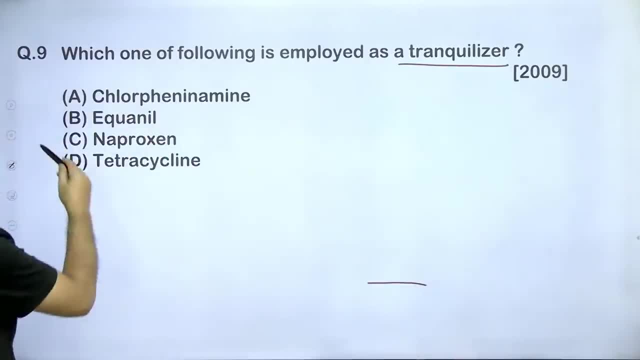 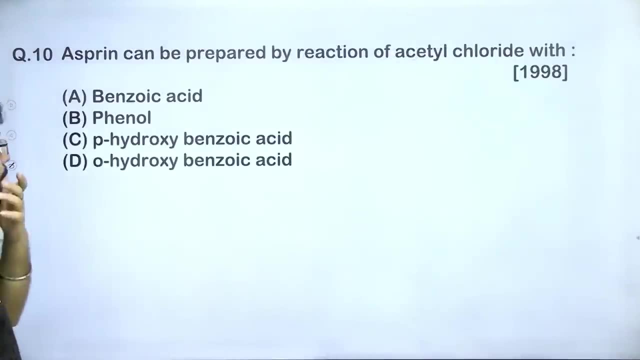 Next, Which is tranquilizer? I have told you the whole list of tranquilizers. Equal is the tranquilizer. Equally sharing, madam. Equally sharing, madam. Next, Aspirin can be prepared by the reaction of acetylchloride with 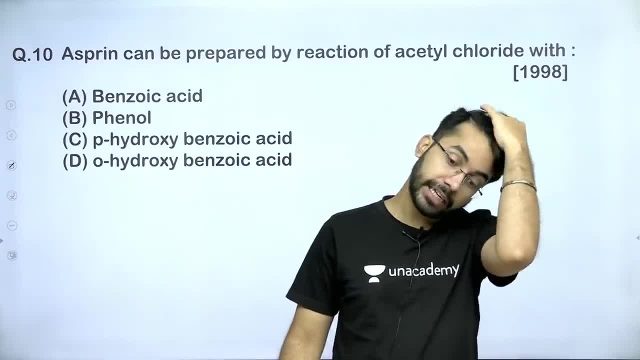 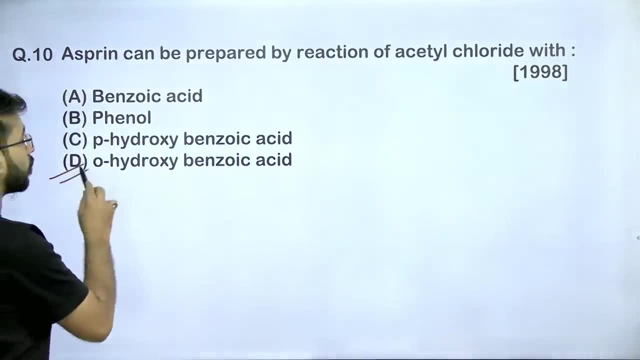 We have already studied the reaction of aspirin in carboxylic acid. Aspirin was produced in carboxylic acid. We studied there, also Friends there. we saw ortho hydroxy benzoic acid, Right Ortho hydroxy benzoic acid. 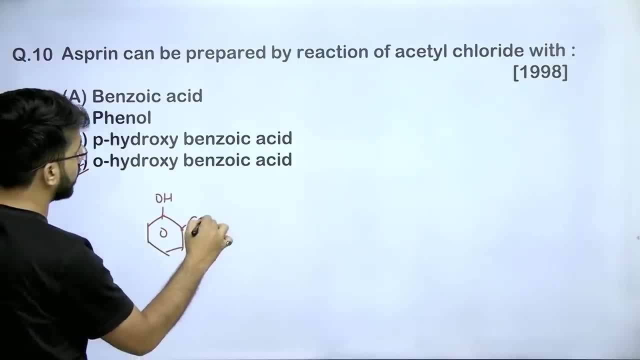 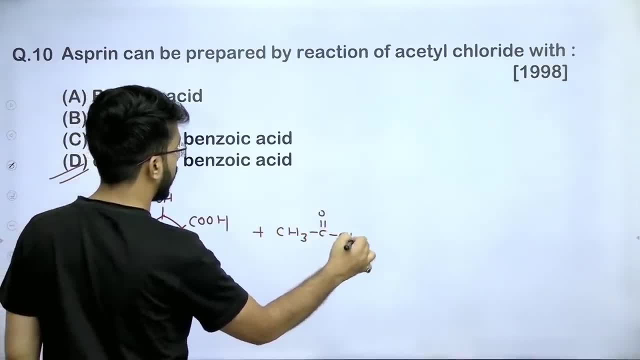 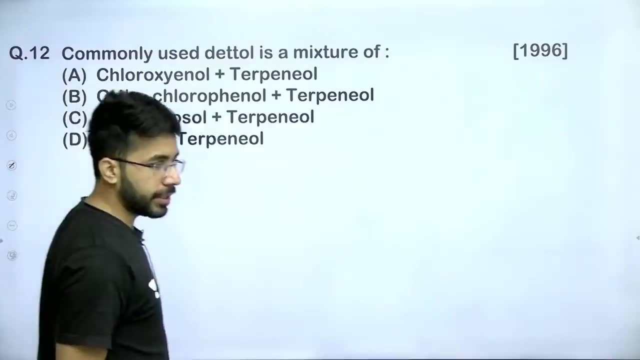 It becomes D option Right Ortho hydroxy benzoic acid. Let's go Next, Commonly used Dettol, Dettol. Dettol is whose mixture- DTC, DTC, T and C are coming somewhere. 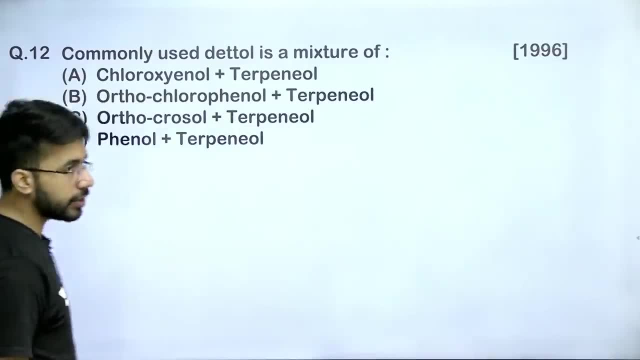 First of all, T and C are coming DTC Right. Chloroxylenol and terpenol Next. What is chloroform? What is the form of chloroform? What is chloroform? What is chloroform? 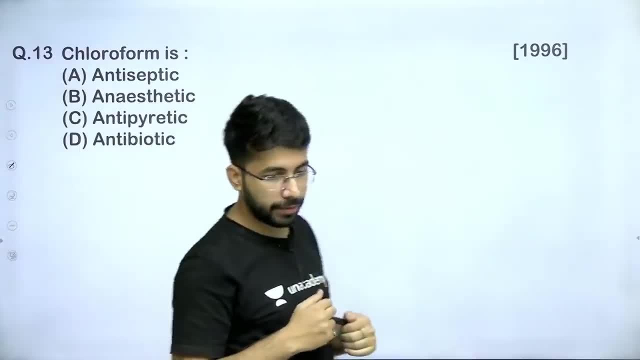 Next, What is chloroform? What is chloroform? It is used in anesthesia. It is used in de-hostage. It is useful in anesthesia of de-hostage. What is chloroform? What is chloroform? It is used in de-hostage. 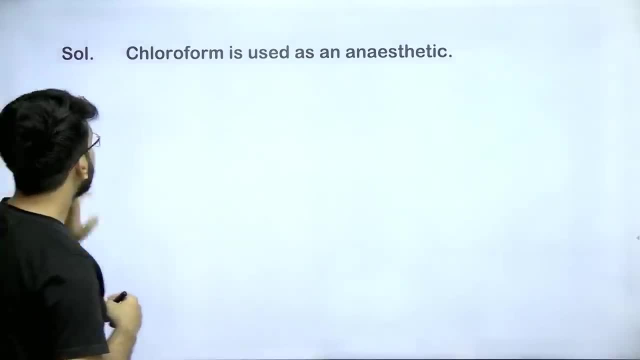 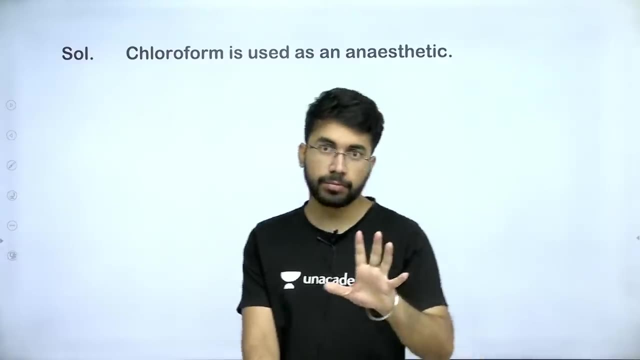 Next, Next, Next, Next, Next. Yes, Thanks, Thanks for all this. Not much has been asked since 2000.. But these days these questions have become more important. These days, the questions are coming every time and the questions are always coming on the. 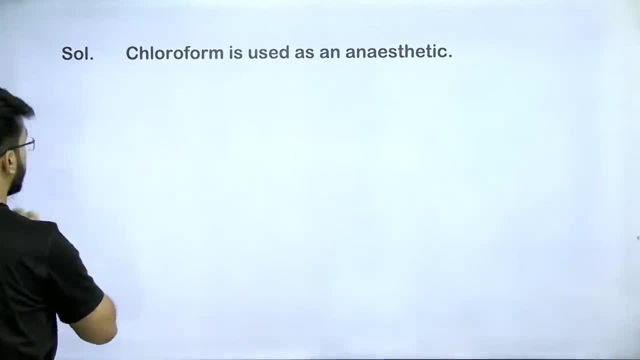 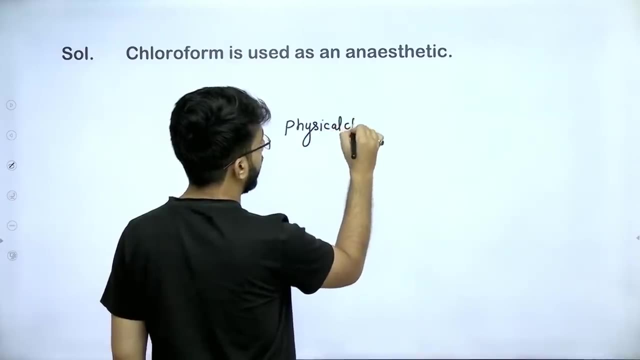 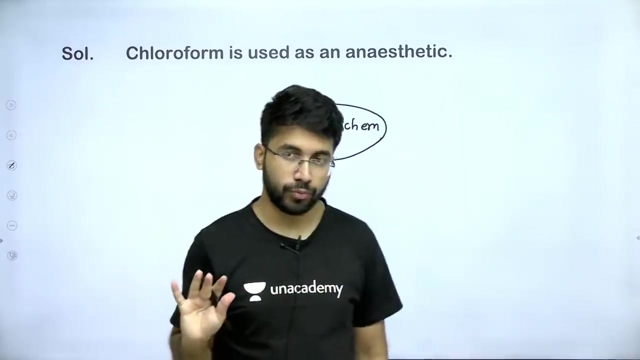 internet. My friends, I have one question from you. You have only this one thing. Next, I will upload a video of physical chemistry in 1-2 hours. I remember Biomolecule and GOC2 very well, Don't worry. 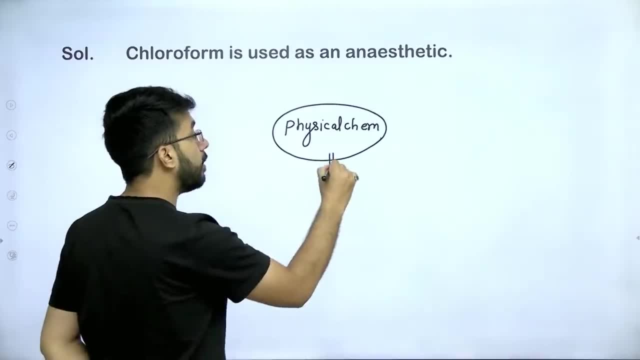 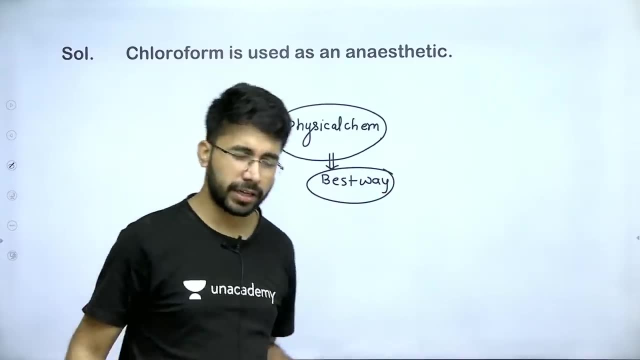 But how to make physical chemistry stronger. We will be doing in the best way. We will not do it in our mind- It's not like we have 50 questions in our mind- and we will do it in our mind. We will do proper research. 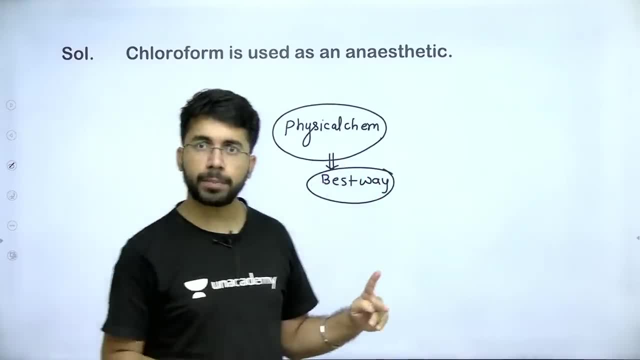 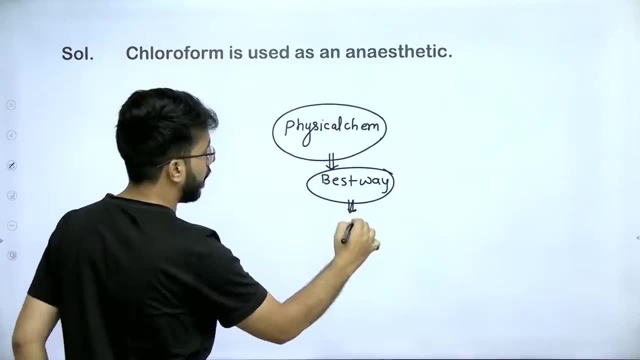 I will tell you proper PYQ, Like I tell you in every chapter. This topic has PYQ. This topic has PYQ. We are going to cover physical chemistry in the best possible way. There will be a video in the afternoon. There will be a video in the afternoon. 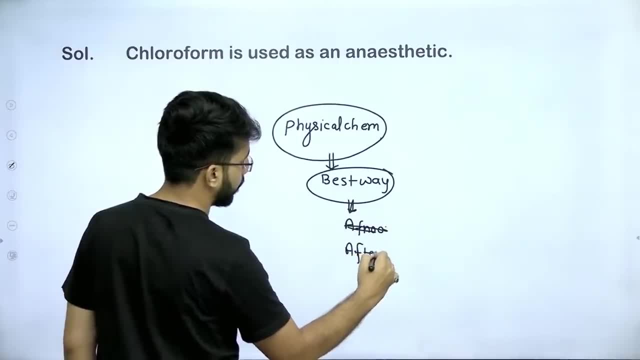 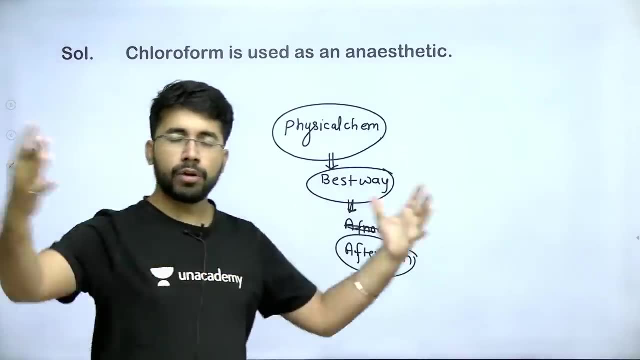 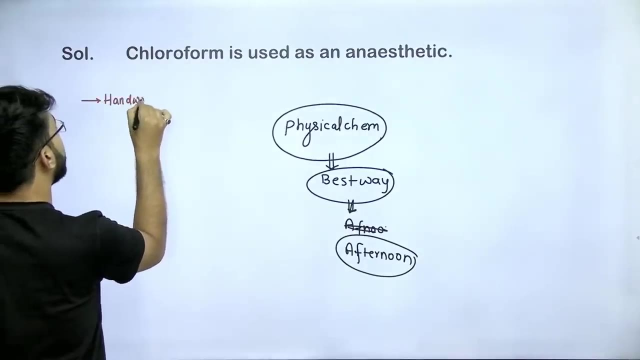 There will be a video in the afternoon And you will do that. I gave you handwritten notes. Now everyone will start giving you all over India. Don't worry, It's good that we are doing it outside. Okay, I gave you handwritten notes in telegram. 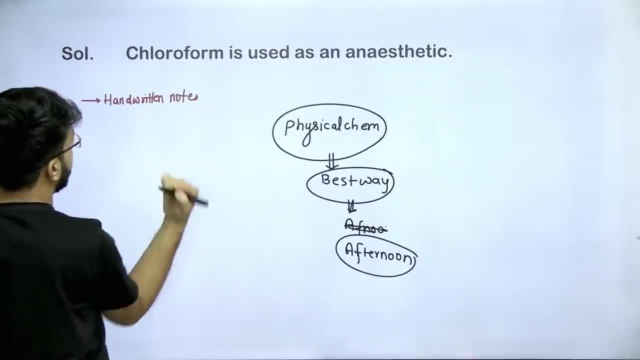 Now you will get everything. You will get everything. After that, friends, After your handwritten notes, I will start giving you the formula sheet of 11 pages. I will start giving you the formula sheet of 11 pages For physical chemistry. 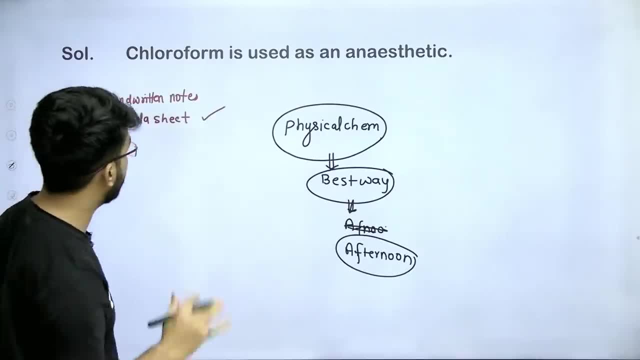 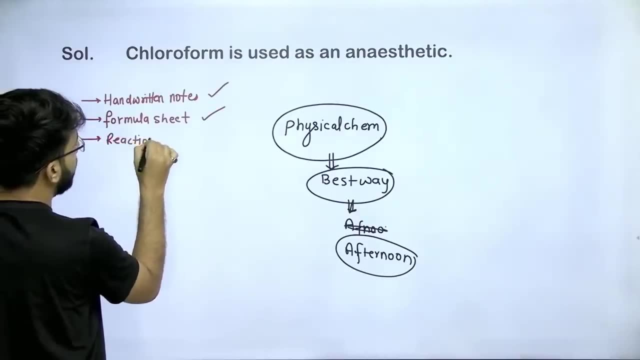 Now it will come again, Don't worry. Everything will come in physics and biology. Okay, After that, friends, It's a good thing. And our reaction chart of 11 pages? This is also being made Actually. Reaction chart. 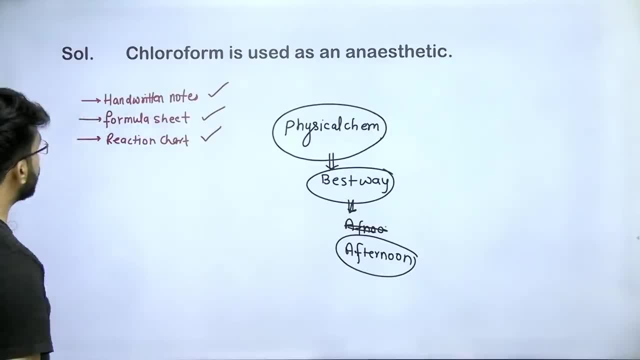 It will be made. I will give it together. Okay, It will be made. I will give it together In one or two days After that. my friends, I have What I have done to you, That if you have any aspirant. 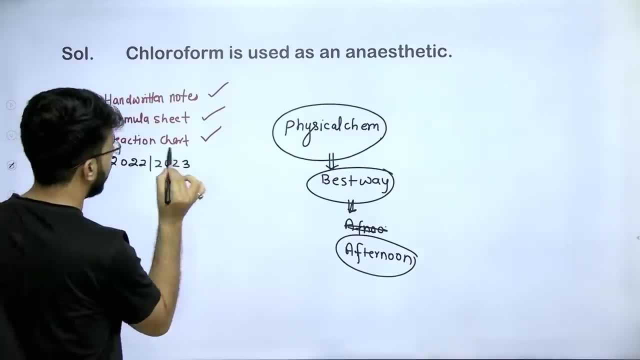 Who is preparing for 2022 or 2023. You can connect it with this education revolution And you can send it inside Bahubali sir To prepare for it. You know He puts his life on it. We can do as much as we can. 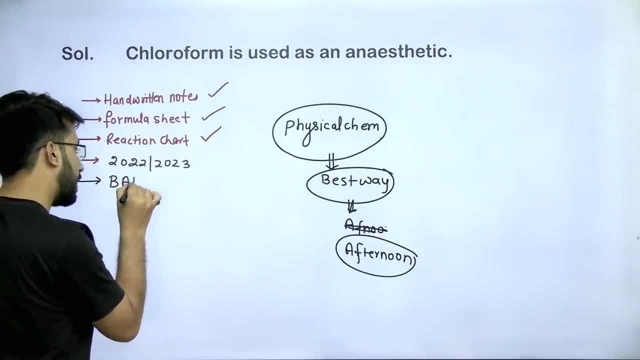 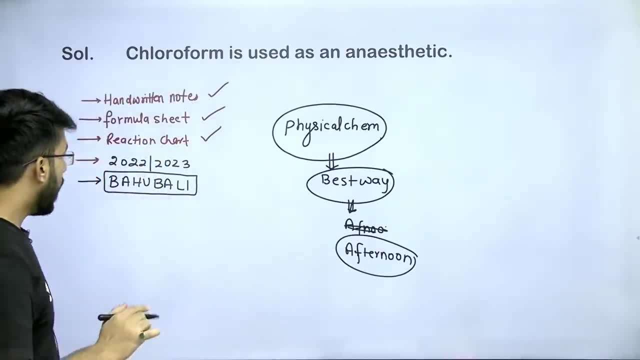 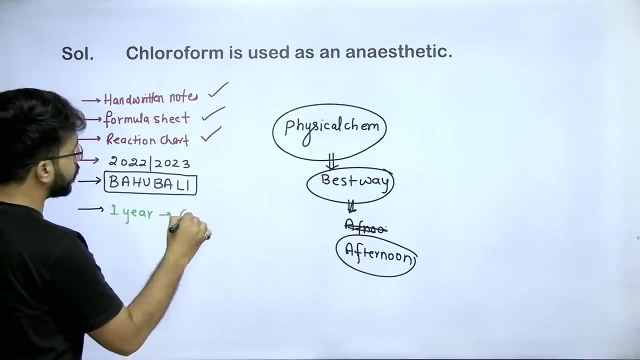 We can do it. Selection: Maximum: Maximum chances: Okay, Selection, If any student with me Prepared for 1 year, 1 year, Prepare it, I will make sure That child, His number, 680+ And for 700+. 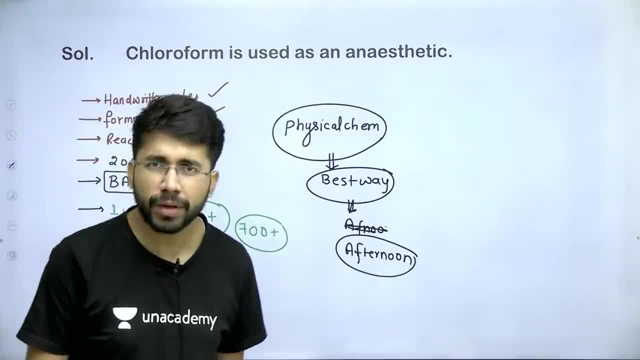 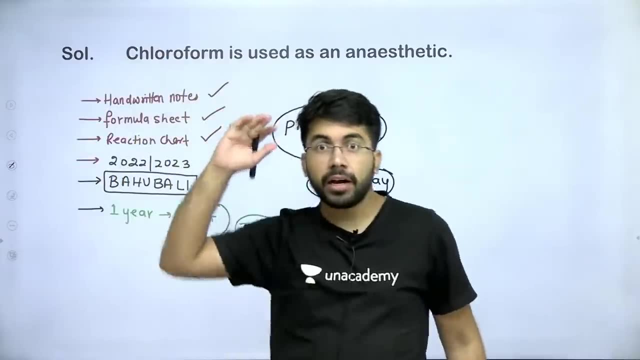 I will try, every time Your Short note, Handwritten: Read this, Read that, Do it this way, Do it this way. Read this chapter so many times. Read this chapter so many times. Do it again and again. You do not do revision. 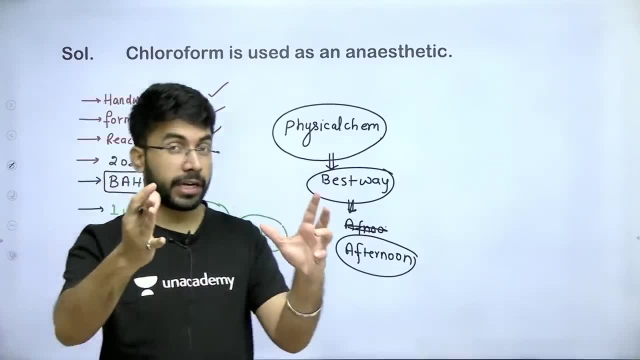 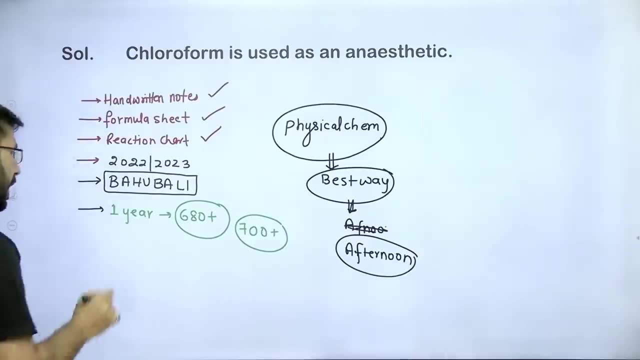 Sometimes Leave it Sometimes. If you have a good strategy, if you have a good thought, if you have enthusiasm, if you have the ability to prepare for a year, then you can apply the Bahubali code by taking a plus or iconic subscription. 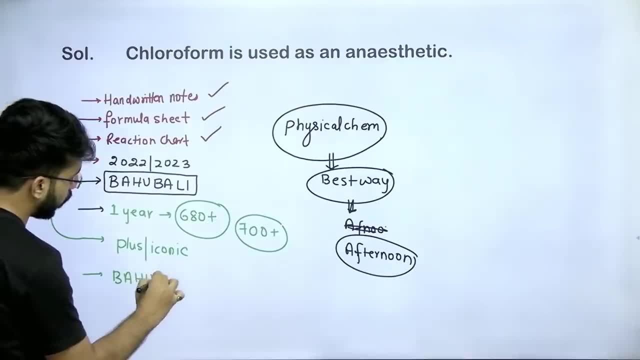 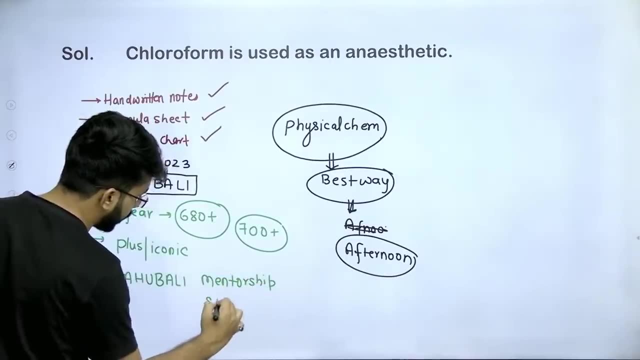 As soon as you apply the Bahubali code, the Bahubali mentorship and study material starts with the application of the Bahubali code. Bahubali mentorship, Bahubali study material, Bahubali notes- these all are the benefits. 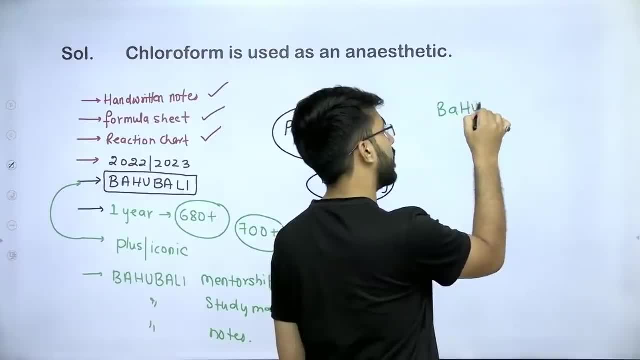 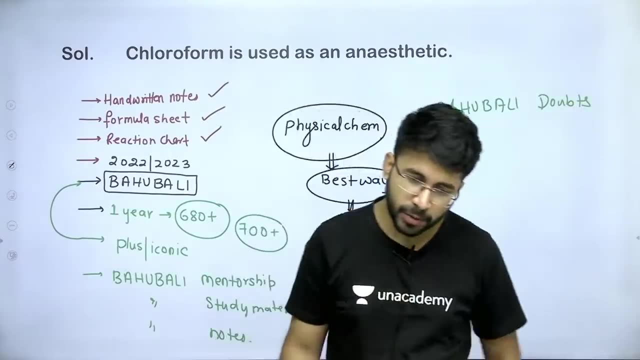 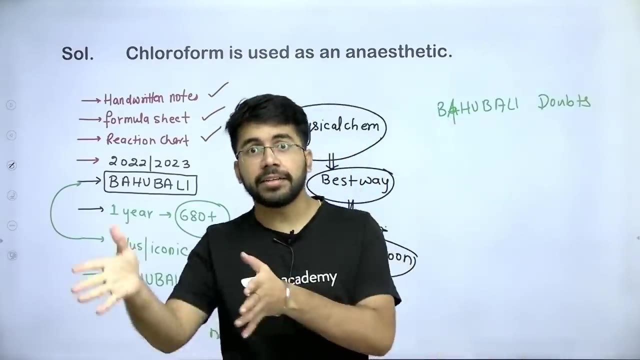 Along with that Bahubali doubts, and you get this in one place with Bahubali- Simple, The code is Bahubali. while subscribing to plus, do use the code Bahubali so that you get a proper mentorship, guidance and top batches of Bahubali. 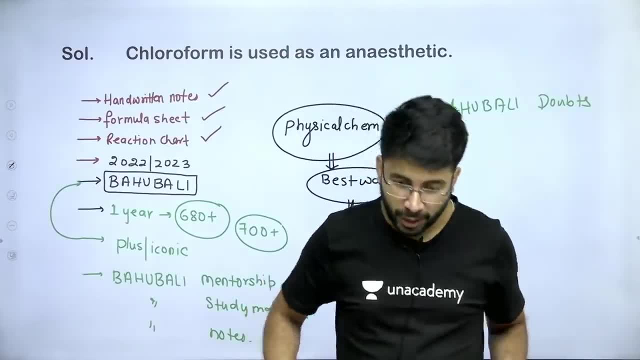 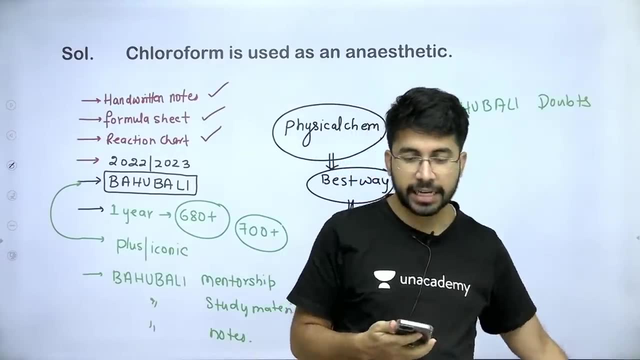 If you have any doubts, you can ask. If you have any doubts, you can ask For 2022, I will take only one batch from 13th September. I will take only one batch from 13th September and I will do mentorship in it. 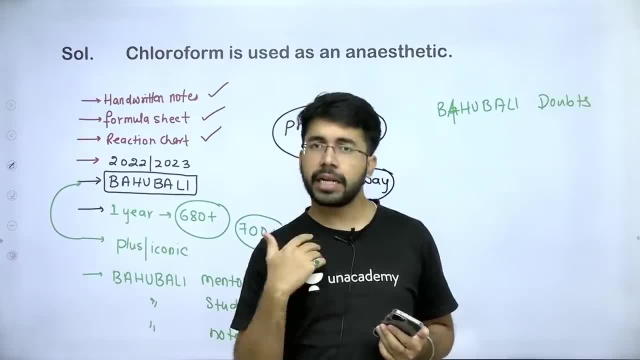 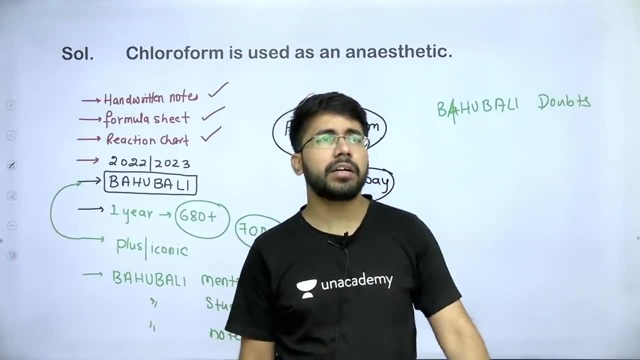 I will get the rank from it. The next year is for ranks. We have done a lot of selection. We have done a lot in the last few years, But now I want a rank in bulk, Like 5-6 people in 100.. 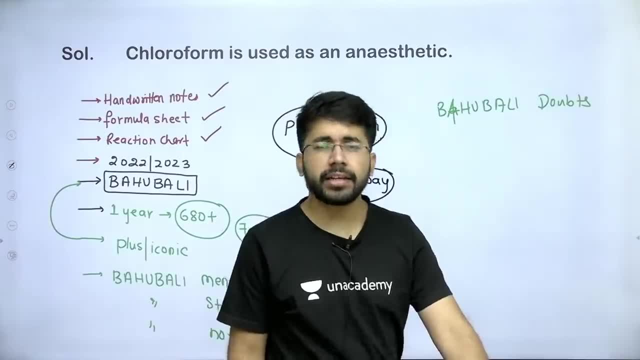 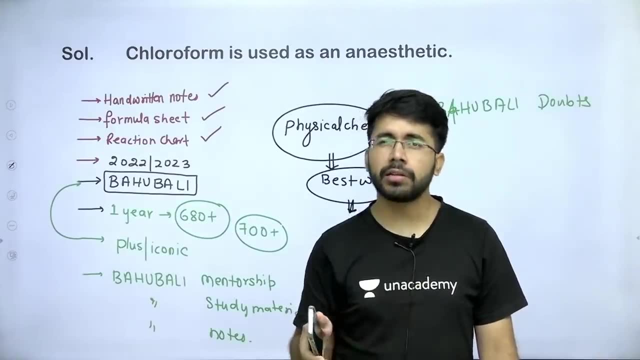 Okay, Only mine, Only mine. We will try What goes. We will try, And those who try do not lose. Okay, We will try with you And there are 5-6 people in 100.. If you are 50 people in 1000, it will not be fun.